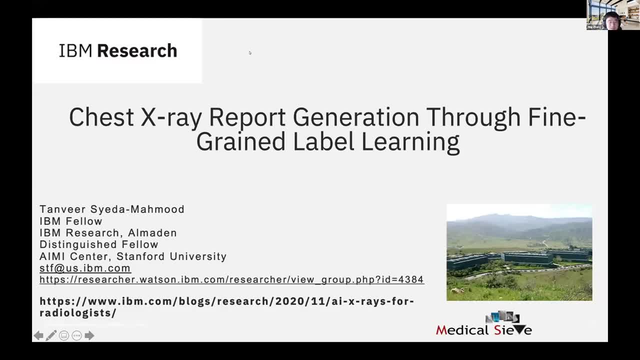 This is the section four. The topic is AI in biomedical image. The moderator is professor Kun Huang and myself. Actually, today we will have four excellent talk. If you have any question during talk, just follow what has happened in last section so you can just make your questions. 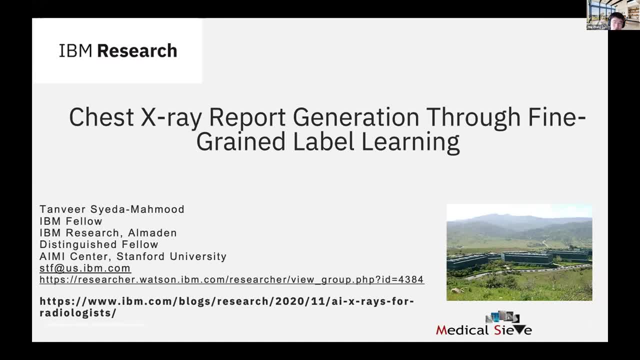 in the chat box And after the four excellent talk, we will have a panel discussion and four of the speakers will address and have a lot of discussion. So thank you so much. Firstly, it's my honor to introduce our first speaker, Dr Tanweer Syed Muhammad. 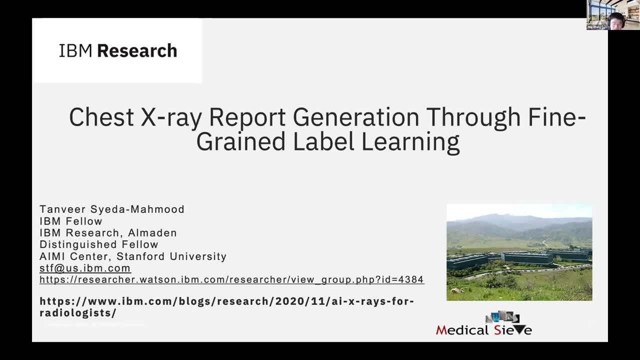 as our first speaker. So Syed is the IBM fellow and the global leader for image AI in IBM research. Syed led a lot of the initiative in IBM and worldwide in image AI. So Syed have published over 200 publications and filed over 100 issue patents. Syed has led many great excellent. 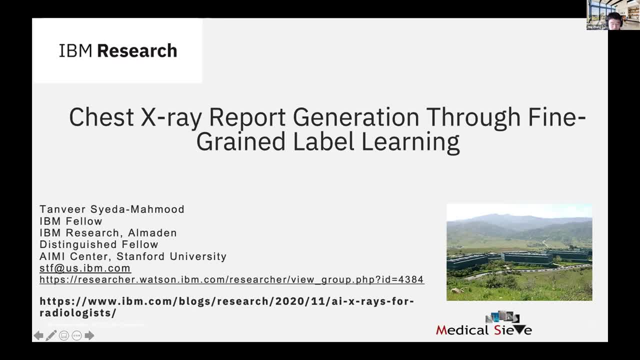 conferences in medical image and the image processing in general, like CVPR, ISBI and the McKinney. So Syed's will be the MACKINN 2023 chair. She is also a fellow of IEEE and AIMBE fellow. Thank you so much, Dr Saeed Mohammed. 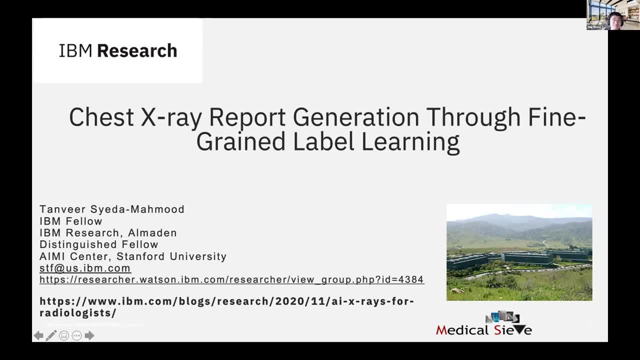 please start your talk, Thank you. Okay, thank you very much for the introduction and I'm happy to be here and talk about the work in chest x-rays that we've been doing as part of the Radiology Grand Challenge project. People can hear me, okay. 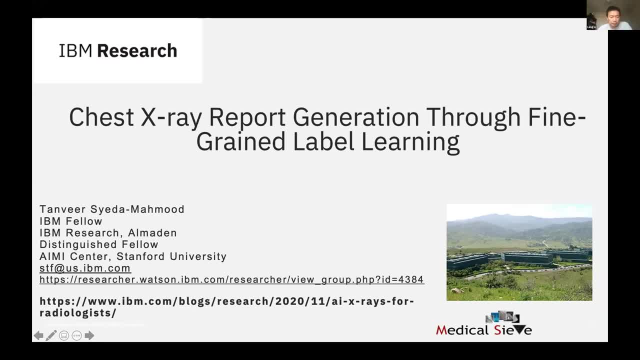 Mm-hmm. yes, Okay, okay, I am going to turn off the video so we save on bandwidth and hopefully the conversation will be clearer. So this is the work that is done at the IBM's Research Labs in Almaden, California, So you can. 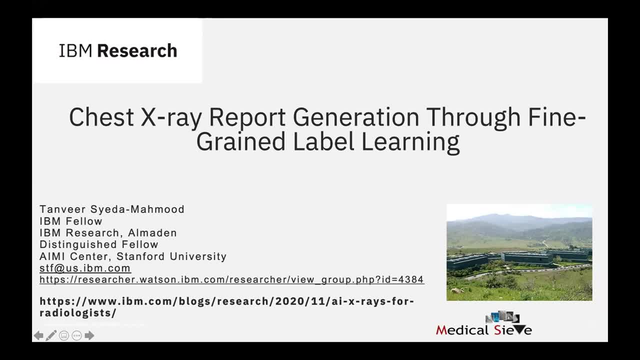 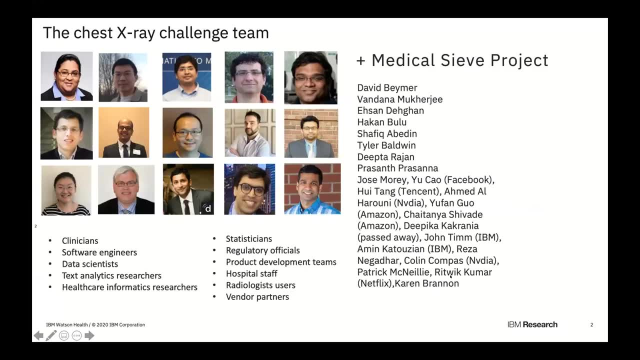 see a cool building over here that I haven't been to for a year and a half. Hopefully we'll be going there soon, So let's see. I just wanted to acknowledge my team that has contributed to this work over a number of years. The Radiology Grand Challenge. 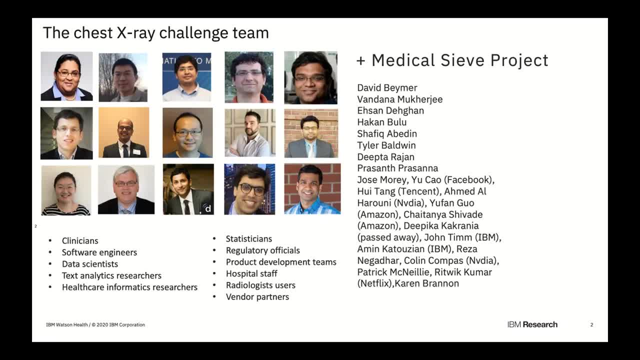 project has been running for a number of years and we just concluded it last year, And what I'm going to talk about is one of the major initiatives we took during that challenge And, as you will see from my presentation that, to pull off a challenge of that type, 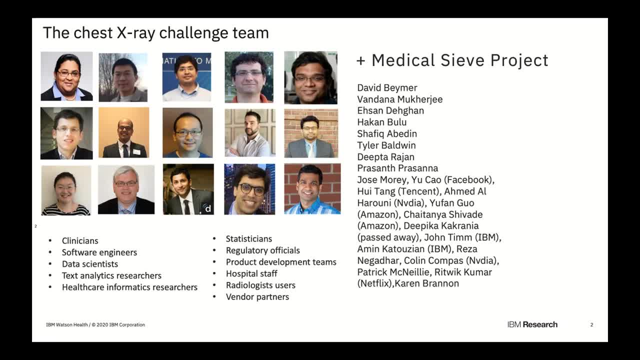 we need cooperation and collaboration from many different specialists, not only medical, imaging and clinical. So I'm going to turn it over to Dr Saeed Mohammed. Dr Saeed Mohammed is one of my colleagues in the team that has done 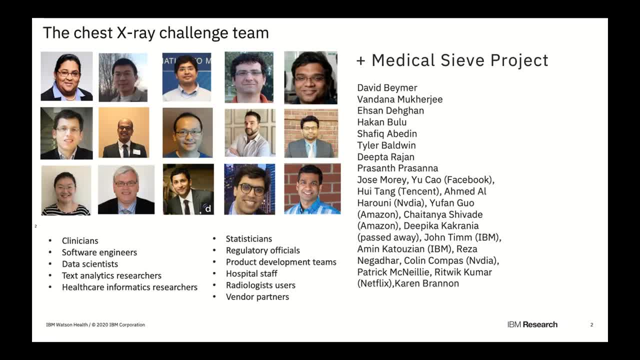 a wonderful job as one of the leading researchers, but also deep involvement of clinicians- radiologists as well as general clinicians- in our work, and software engineers and data scientists and statisticians and even regulatory personnel, as you can see. 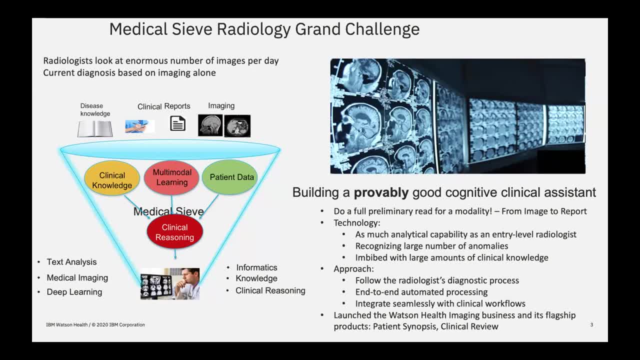 So what is the Medical Cell Radiology Grand Challenge? This was a project we started that helped kick off the field of AI in radiology And remember we did an exhibit in the called the eyes of watson in 2016 at rsna, which also helps get it exposed to radiologists from. 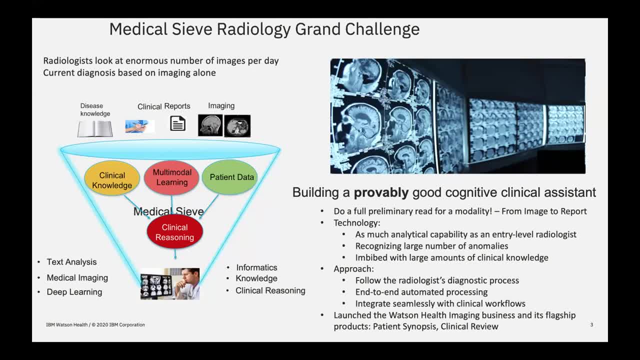 from what used to be in medical imaging as a focus area and since then rsna, holding an annual ai showcase, and sim and other radiology focus conferences have picked it up as well. so the basic idea of the radiology grand challenge was to produce cognitive assistance. 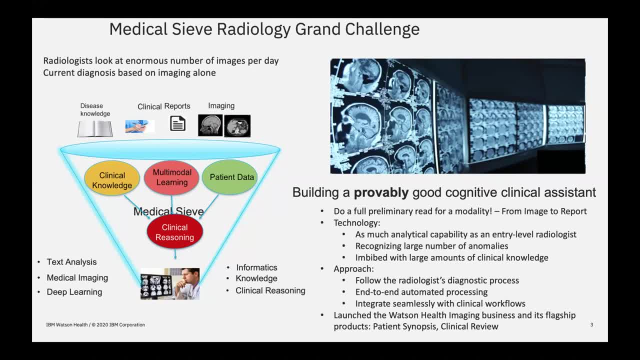 that could serve an augment radiologist workflows and and do it in such a way that they can be trusted and and and at a level that is at the level of an entry-level radiologist. so the, the, the products that came out from this work and all i think you've already seen from 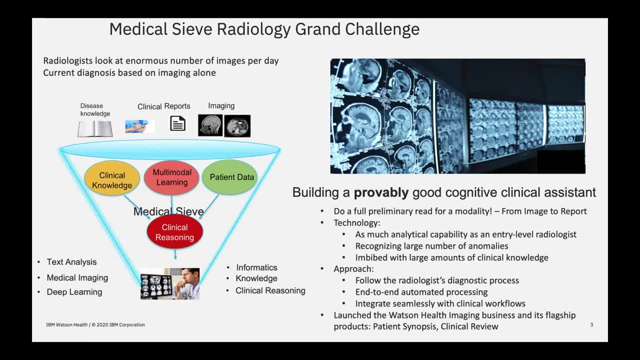 ibm, watson health imaging, has already learned some of the products that came from our research, but the challenge that we took on towards the in this particular effort was to see if a machine could do a full preliminary read of a single modality, and which means going directly from. 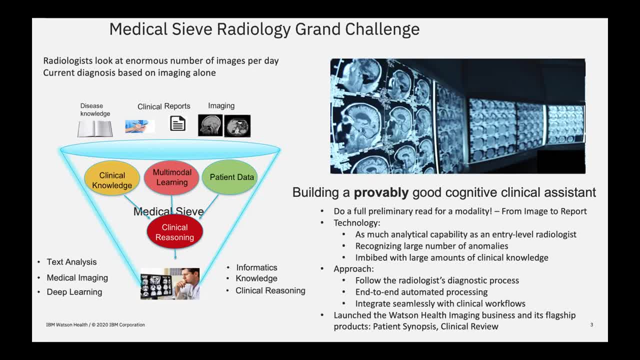 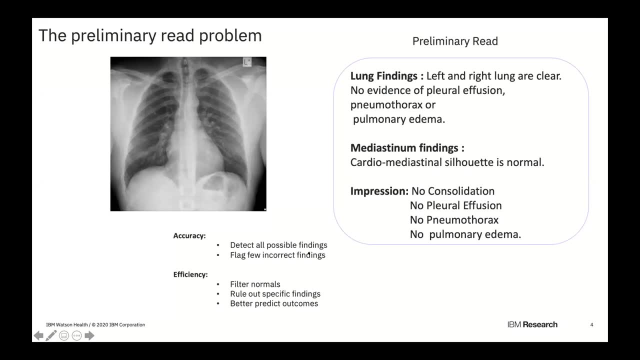 an image to a preliminary report and then show that the type of report that we've generated is as good as what could be done by an entry-level radiologist. so now you may ask: uh, what is the preliminary read problem? as i said, it is going from an image. 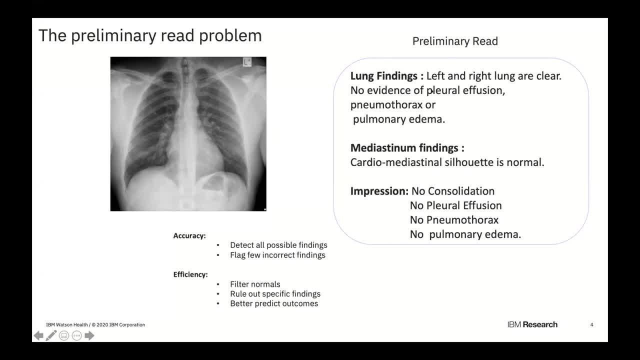 such as this to a report that documents the findings and the major structures, both positive and negative findings, uh, as well as uh non declaration of normality from which potentially could be used for filtering as such. but look at the- the- the phrasing, and the- the- the type of the. 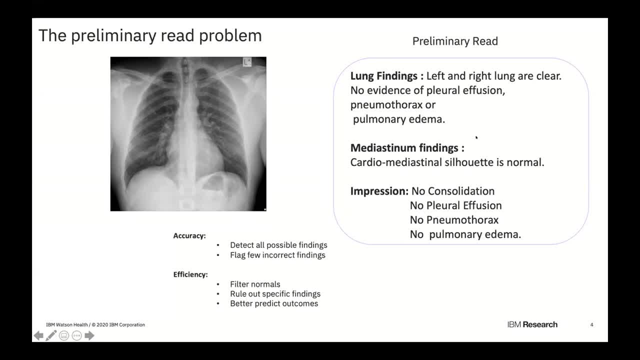 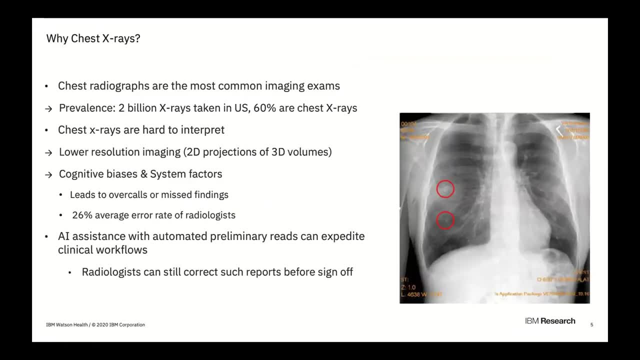 of the report that mentions the problems and in terms of where the problem is located as well, not just what the anomaly is. So we chose chest X-rays. as most of you know, it's the most common modality And it's also from a commercial standpoint that makes sense, given the prevalence. 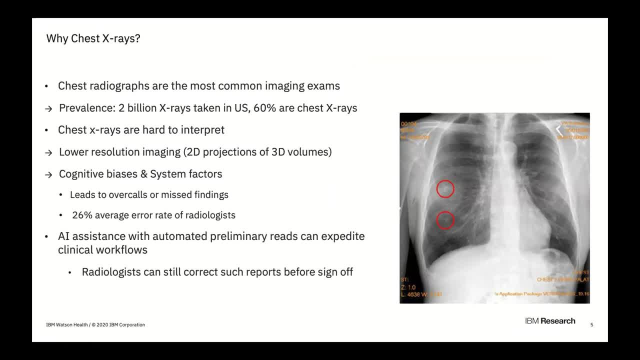 of use and the radiology practices don't make much money on chest X-rays, So having machines do much of the filtering would actually be welcomed. is the current hypothesis. There's also a lot of error: the possibilities due to the low quality of the imaging and the cognitive 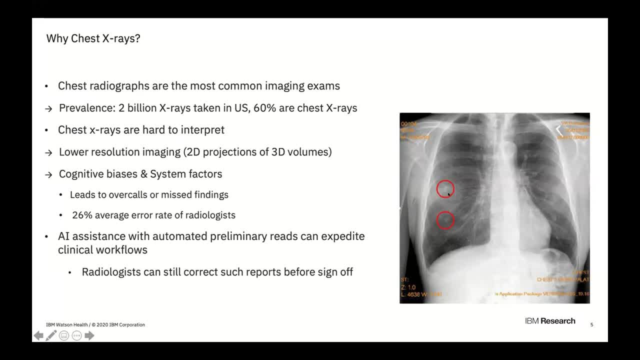 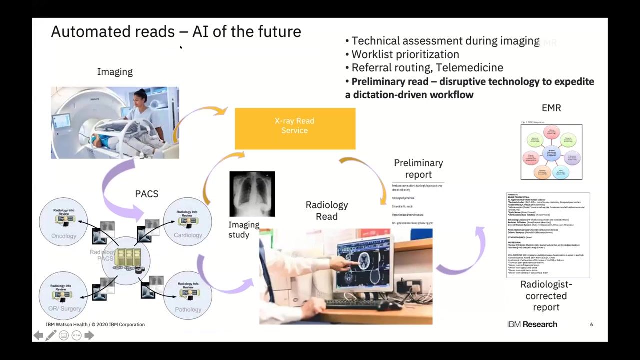 biases that hinder the interpretation of these as such. So if we could produce a report automatically from looking at chest X-rays, the machine could do that And if that was a good quality report, it can. It can help expedite workflow in many ways. We can see: sorry, I think Okay. So the idea being 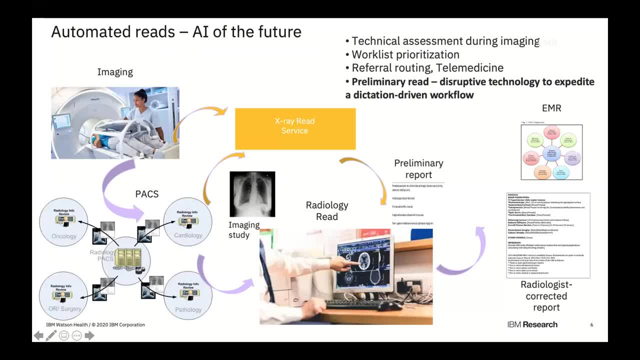 that it can be used at any steps in a clinical workflow, whether you are an imager and, at the point of imaging, determining whether the quality of the imaging is adequate. and the report would establish that, because technical assessment is one of the things that would be in the report. 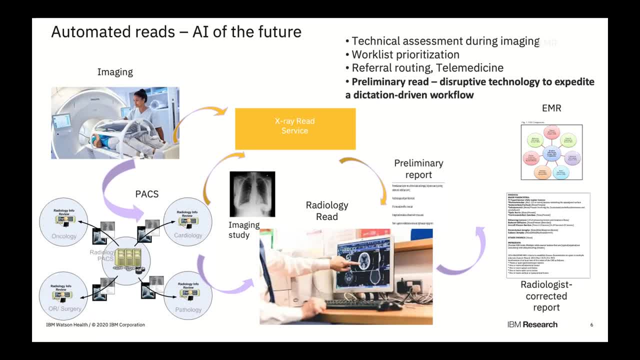 If it went into the PAC system and there was a criticality of a case, then you could reorder cases. So it helps prioritize important cases to be read ahead. If, obviously, if the preliminary report is already made, it in some sense disrupts the current. 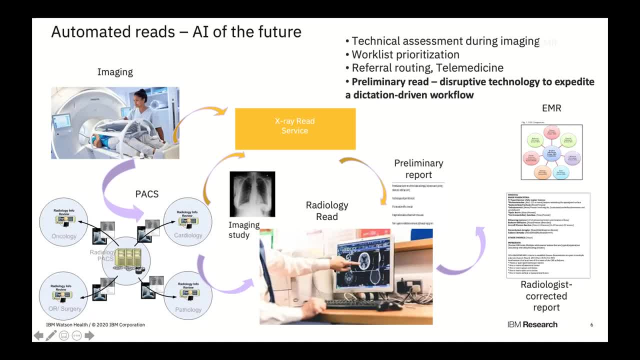 dictation-driven workflow where the clinician has to dictate and sit and correct the report or outsource it and wait for that transcribed report to come back. So in this particular case you would be able to get a preliminary report that a radiologist can quickly correct and 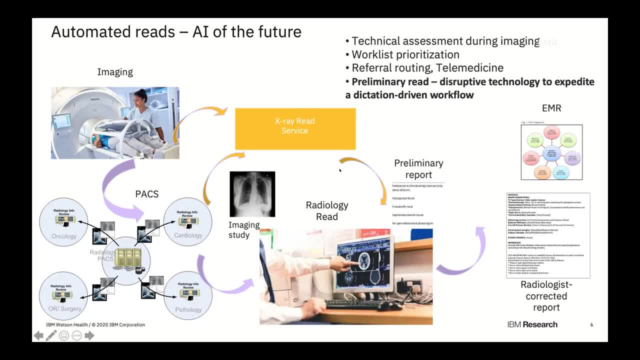 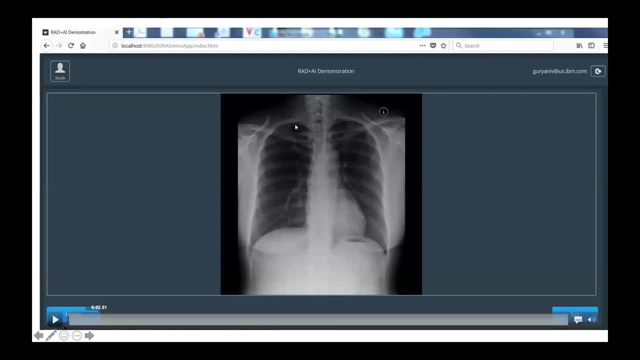 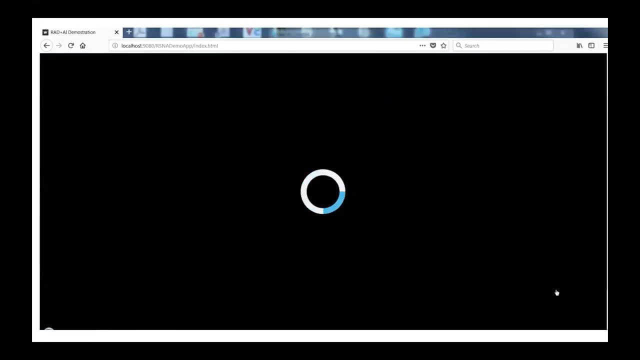 then enter it into an EMR. So overall it would expedite. that clinical workflow is the expectation. So now let me just show you what we mean by doing a report. So, given an image such as this, the system would go ahead and this is a service that is running. You submit the image to this. 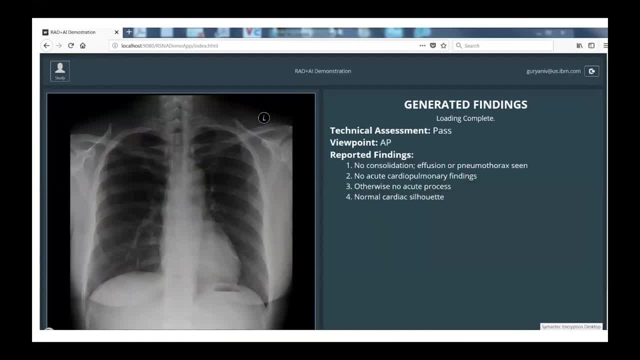 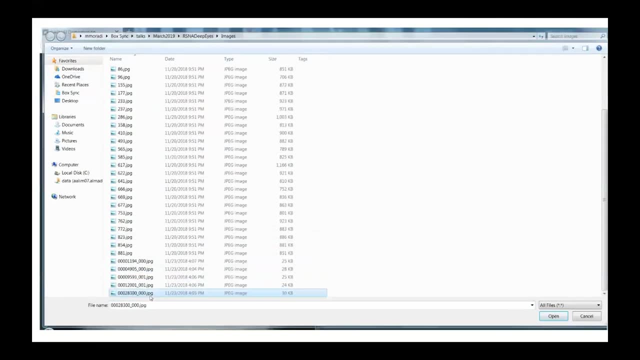 service. It analyzes the structures and then comes back with a finding report, And this is the we brought it to, and you can just select any image from your PAC system, any study, just upload it to the service and you would get back a full scale report. 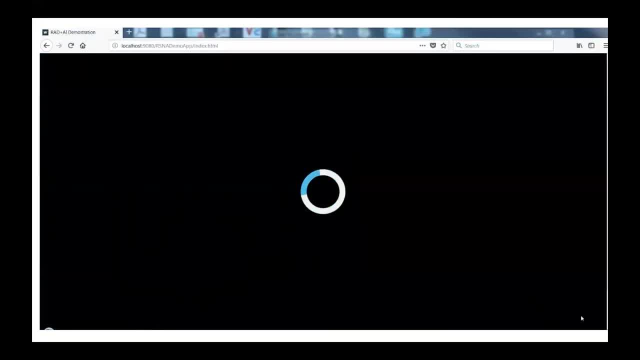 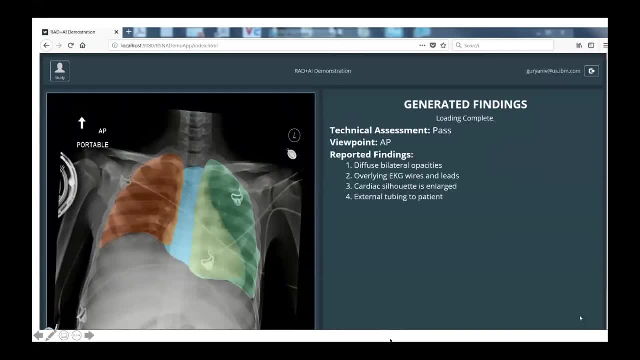 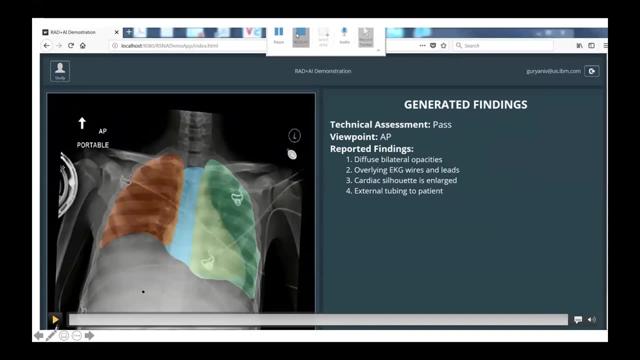 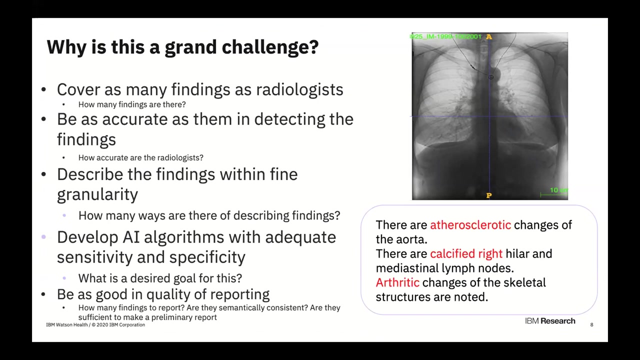 And you can see here, the image quality is pretty. there is skew and so on, but still the, the findings were detected and technical assessment was made, viewpoints established and so on, and then the report is generated. So going, so you might say, why is this a grand challenge? So the grand challenge comes from the fact that the, the imaging that we are interpreting, is, as we said, very poor quality as such, and a variety of it from various hospitals and settings. 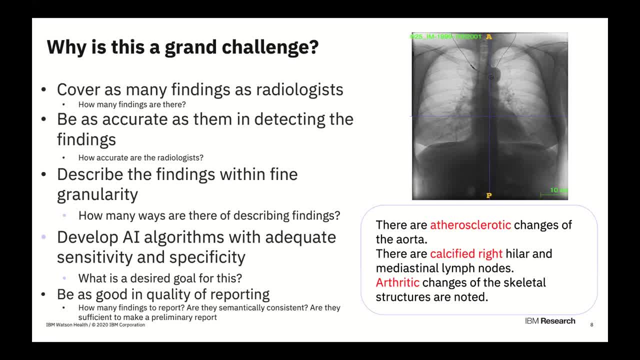 But the most important reason is that if you want to claim that the machine can actually produce a report that is at the level of the entry level radiologist, it must be Able to have a full coverage of findings. And that's the first difficulty, because we don't know how many findings are there in chest x rays. 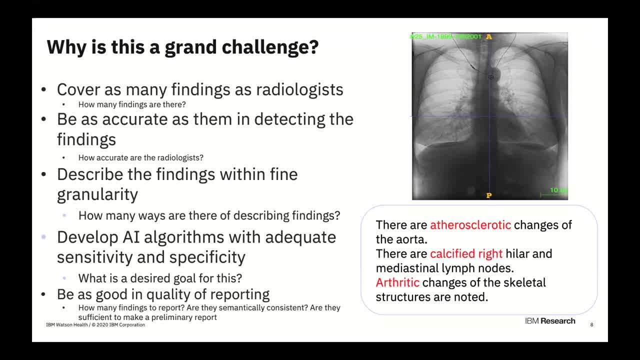 The second is to go and do them as accurately as possible, But if you're saying it should be comparable to radiologists, how good are they in detecting? and we don't have any concrete data about them, since we don't know how many findings are there. 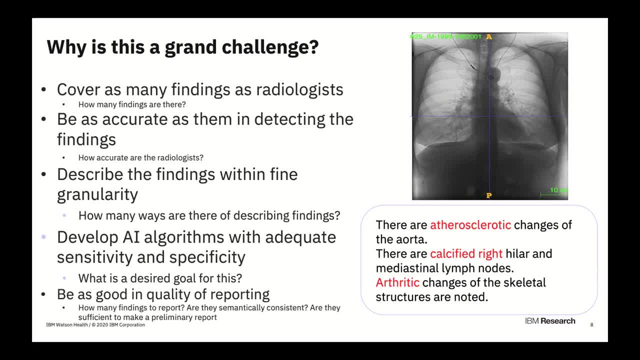 Then the last step in reducing the report form is to be able to describe the Finding, and so use terms such as these: calsified right and media style- and link notes. So this is not only describes the finding, but also where it is occurring, a neutrality location. 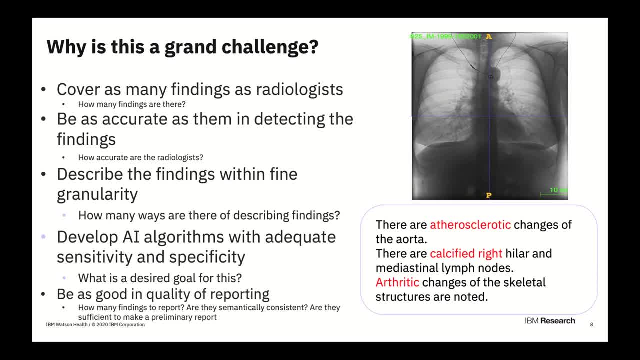 severity. all of these things need to be described as well. So, overall, how do you judge the quality of a report and and how can you actually do formal comparisons? all of these term makes it a grand challenge. So, as you can see from the description, there is work to be done, not. 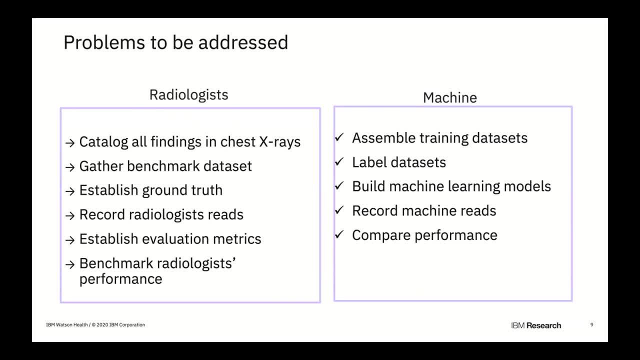 just on the machine side, but also actually establishing the benchmark itself on the radiologist side, where you need to be able to catalog all such findings first of all, and gather benchmark datasets that are agreed upon by radiologists themselves and the findings from them have been. 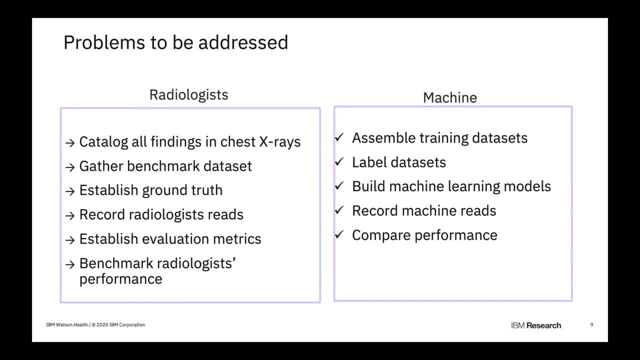 properly documented so you can have a gold standard for judging as well. And once you have that, obviously you have a lot of work to be done on the machine side in terms of assembling training datasets with different prevalence distributions, labeling such images accurately. 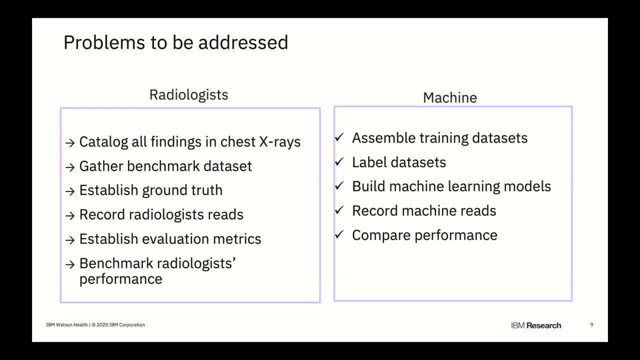 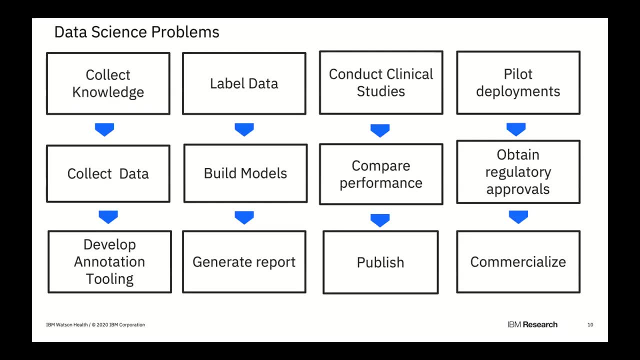 so that you can build machine learning models and then develop some comparison studies as well. So this is all we had to do in order to conduct this project, and some of the many data science problems that we had to solve along the way I'll point out, as this is a conversation that we had to have and I'll point out, as this is a conversation that we had to have, and I'll point out, as this is a conversation that we had to have, and I'll point out, as this is a. 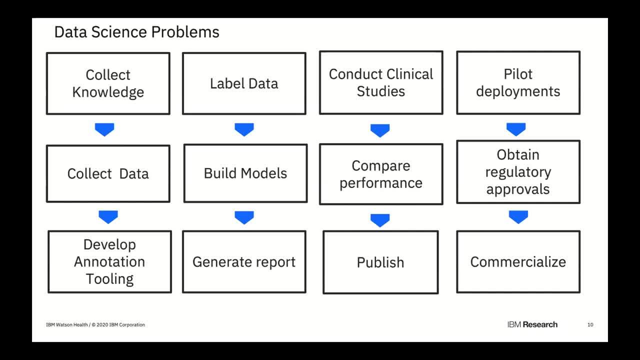 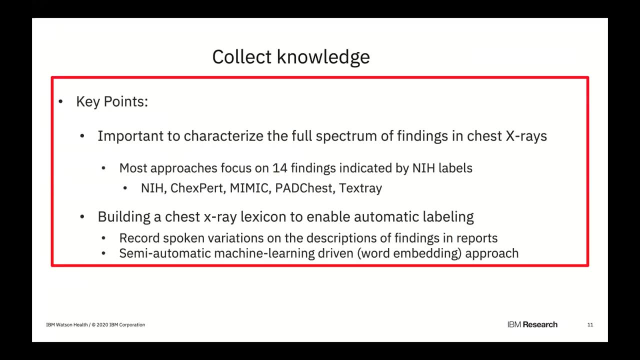 conference about AI and it's using biomedical imaging. many of the problems in data science also apply to us, and you have mentioned over here some of these problems that we'll take you through. In fact, the coverage will cover most of these issues, So let's look at the first one. 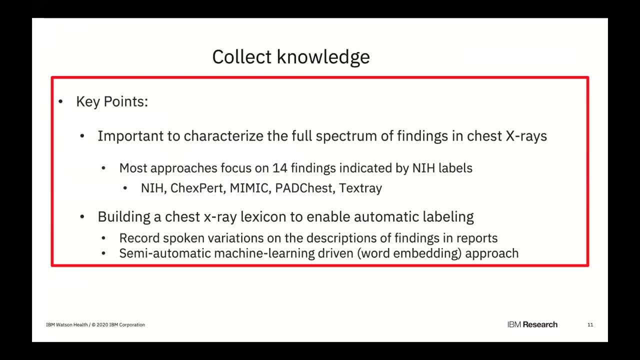 which is to catalog the full spectrum of findings. Now, as you know, the majority of the work in chest X-rays has been on describing mostly the 14 findings that were used to catalog the initially done in the NIH data set and a lot of the new data sets that have come out publicly. 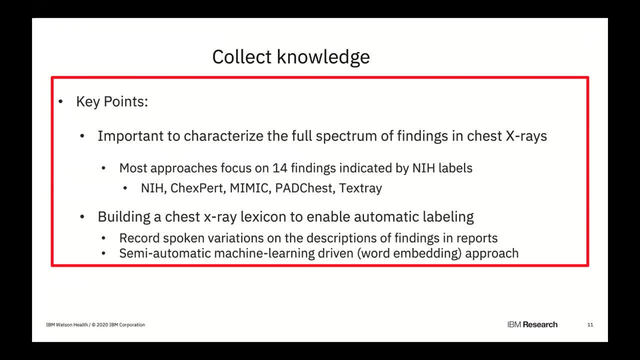 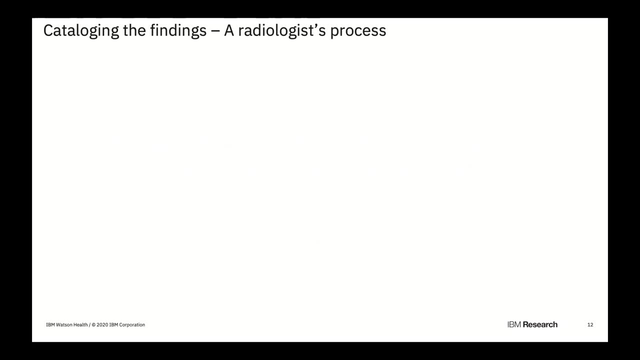 available have basically gone after essentially the same set of findings. There has not been a very good systematic effort to catalog how many findings are there. So this is the effort we took on and essentially the approach we took was to see how to catalog the findings by closely. 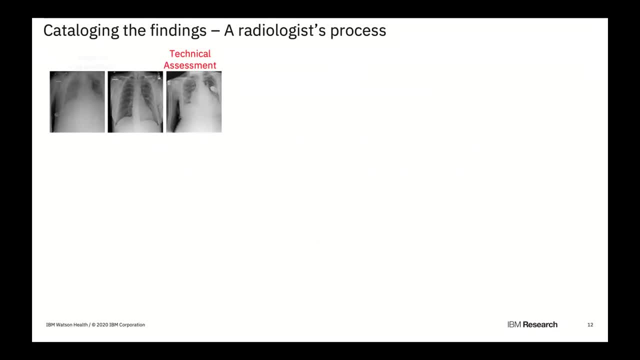 following the radiologist's process. So you can see that a radiologist would first to see whether the image is ready for interpretation from a technical assessment standpoint, whether it is underexposed, overexposed, whether the viewpoint has included the majority of the regions that were supposed to be evaluated, and so on. 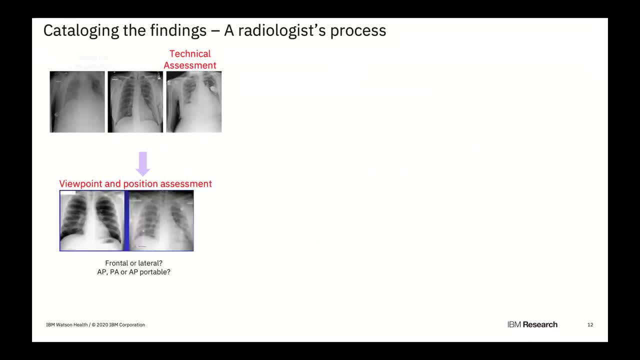 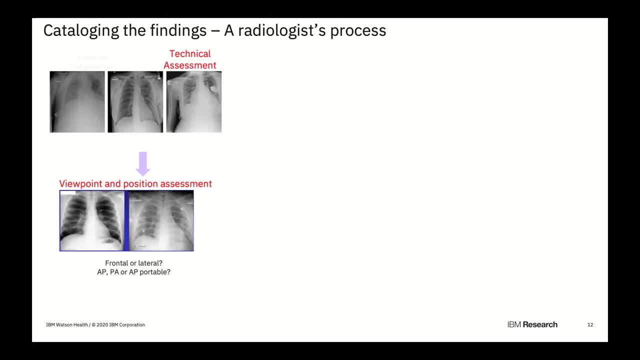 or whether it is a portable setting, as this could then establish some biases. If the patient is, if it's an AP chest X-ray, then this is probably an in-hospital setting and that already sets up a bias for interpretation. If it's an in-hospital image, then one of the tasks is also to see if 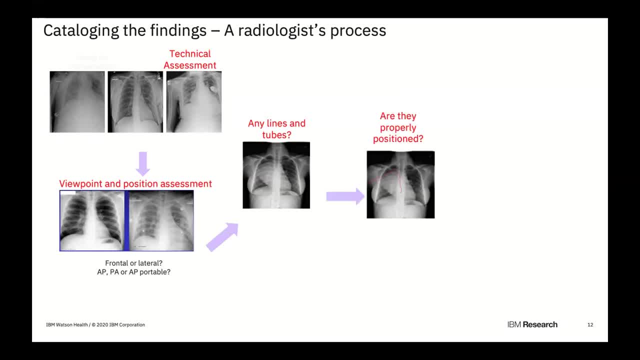 there were any tubes and lines inserted and whether they were properly positioned, and if there were any artifacts- device artifacts such as sternotomy wire and so on. So this is one of the things that we need to look at. So this is the typical process that radiologists follow. 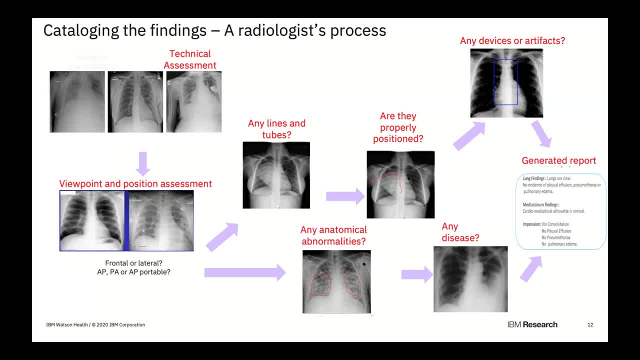 I'm not sure if there are radiologists in the audience, but perhaps they can comment on that as well, But this is what our radiologists used as a guideline to help develop the idea of a PX chest X-ray. So this is a typical process that radiologists follow. 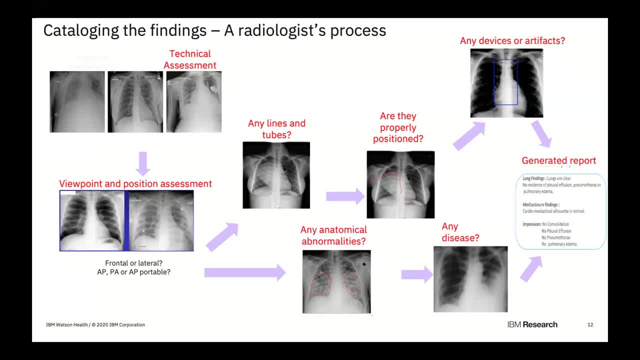 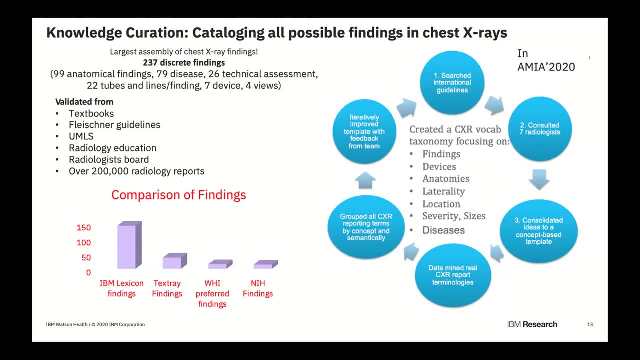 As well, to address each of these problems in the cataloging of findings. So overall we went through an effort with many clinicians using both a top-down and a bottom-up process, to generate a lexicon that describes about 237 discrete findings And you can see over here the catalog. 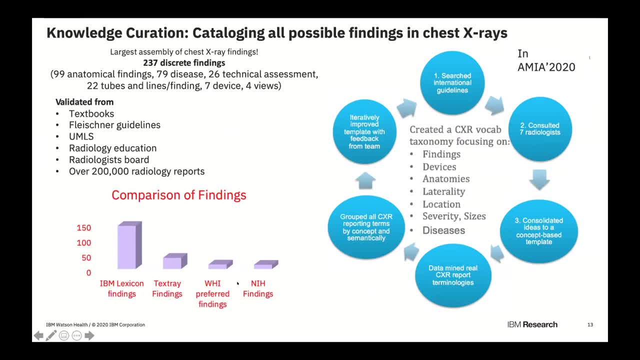 of this. This essentially is one of the largest set of core findings assembled, and they cover the various types of findings, Ranging from anatomical findings to tubes and lines, to bed placements and so on. Some of these datasets we've actually also released in open source, So you can see over here that the generation 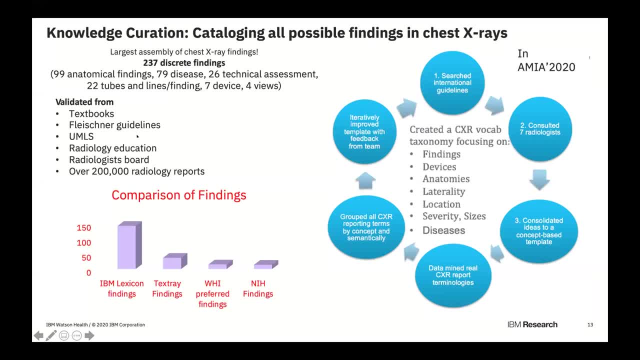 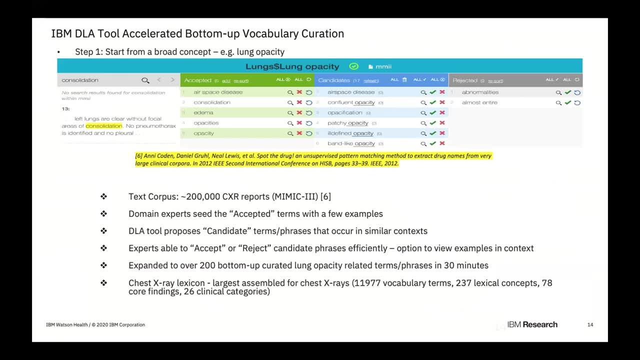 of the findings took both top-down knowledge from the clinicians and guidelines, but also bottom-up extraction by mining about 200,000 records, where we used a tool that has an actual learning capability, where you use ENCOA as self-supervised data, And then we used a tool that has an actual 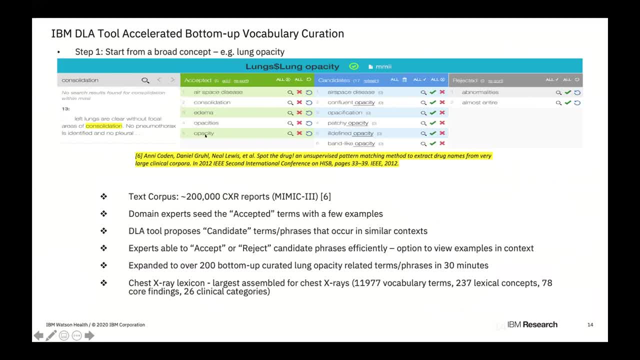 learning capability, where you use ENCOA as self-supervised data. And then we used a tool that has an actual learning capability, where you use ENCOA as self-supervised learning methods for encoding of text and use that for similar expansions of similar terms. So this is a tool called a domain. 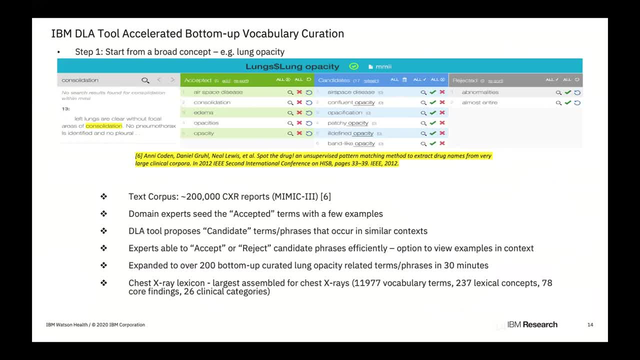 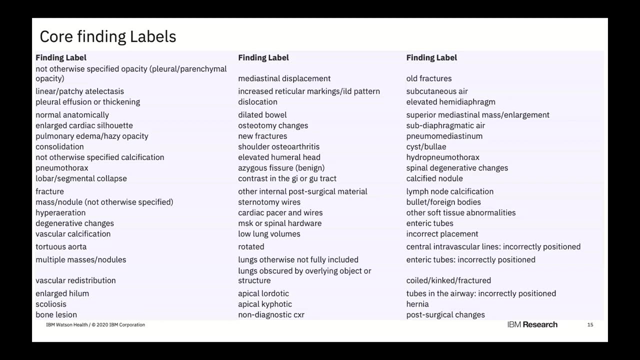 learning assistant, which is used in bioclinicians to rapidly expand the vocabulary. Much of this work we've described in the AMIA publication last year. So based on that we gave rise to a whole bunch of finding labels. So you hear, some of them are documented here and here. the radiologists in the lab. So, based on that, we gave rise to a whole bunch of finding labels. So you hear, some of them are documented here and here the radiologists in the lab. So, based on that, we gave rise to a whole bunch of. 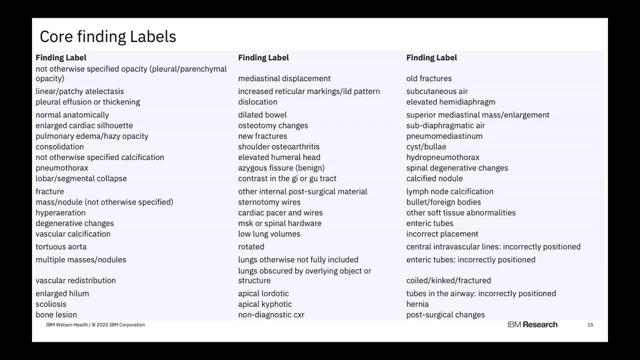 finding labels. So you hear, some of them are documented here and here. the radiologists in the lab. So we gave rise to a whole bunch of finding labels, So you hear, some of them are documented here and here. the audience can relate to many of these findings as such. So the next step was to go and acquire data. 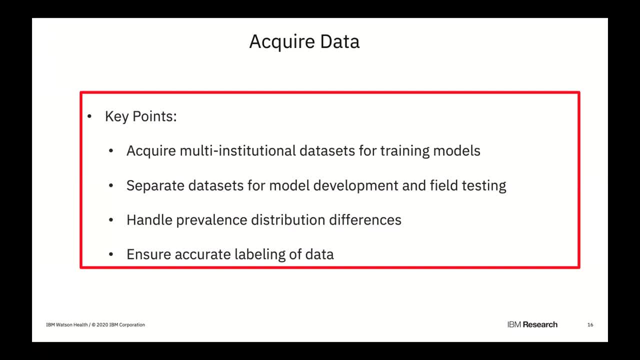 and label such data sets for these findings And, obviously, when you want, the key considerations we'd have to do is to see that we're not just trained on one hospital data, but can accurately do it across demographics, and to be able to understand the prevalence distributions of it. 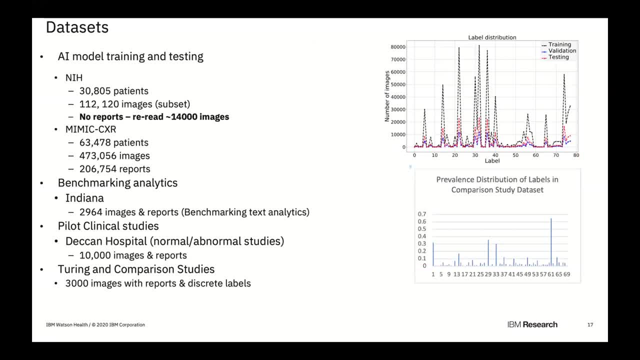 and use them for evaluation purpose. So I think it's a really important thing to do, And I think it's a really important thing to do. And I think it's a really important thing to do. And I think our data sets came from at least three different sources and we set apart some data completely. 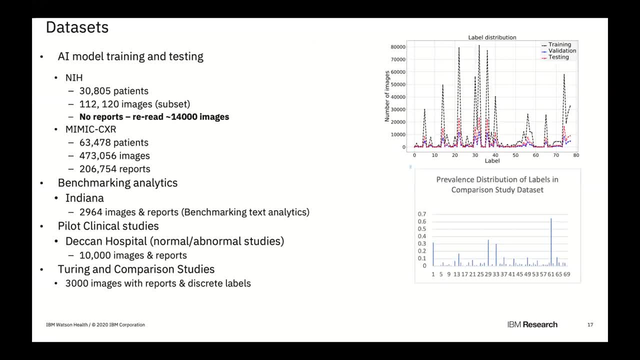 for testing that came from an international data set as well, And this is the data set from India, And you can see that the prevalence distributions and the way the partitioning of the data sets was done for training, testing and validation maintain the prevalence distributions as such. 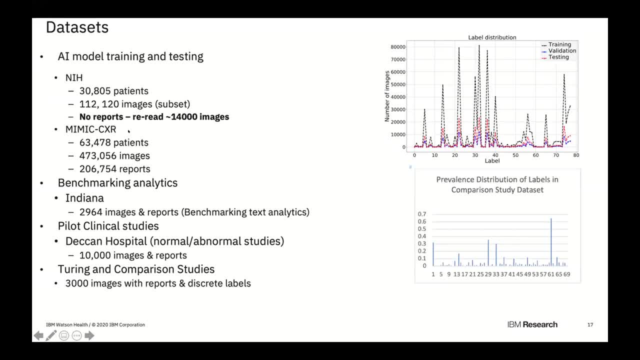 Many of you there. this MAMIC data CXR database is now available also in open source, But at the time when we started, this was exposed to us through a consortium agreement. It has about 60,000 patients and about 450,000 plus images as such, Whereas the NIH 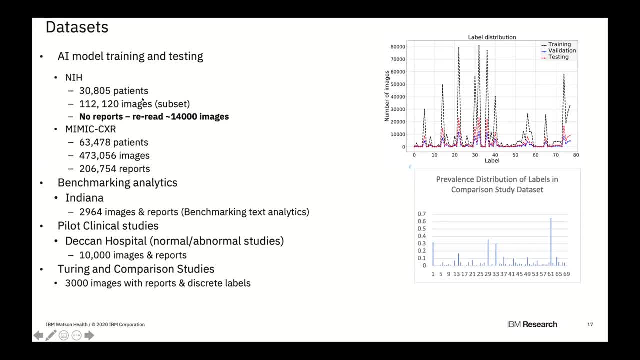 data set came with about 100,000 images from 30,000 patients, but only a small subset of them we could use because the labels that are provided only covered 14 of them. So we ended up having a lot of data set And I think it's a really important thing to do And I think it's a really 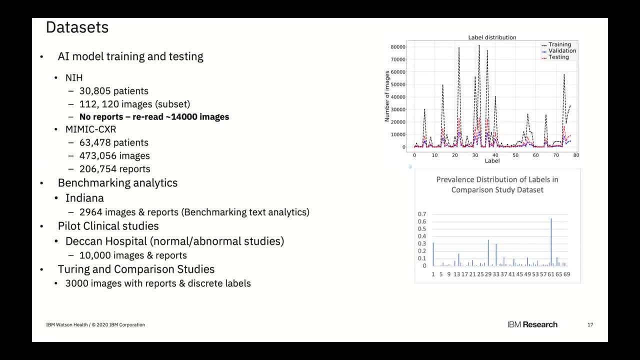 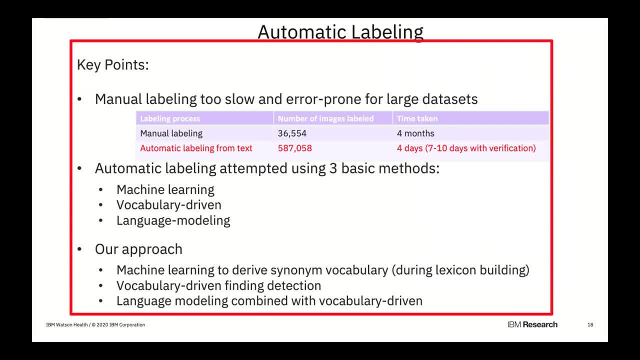 So the next step was to label these data sets- So many of them. now there are labeling platforms. back when we started, there weren't any good web based labeling crowdsourcing platforms that could be used for this purpose, So we built our own such platform. However, using our platform, 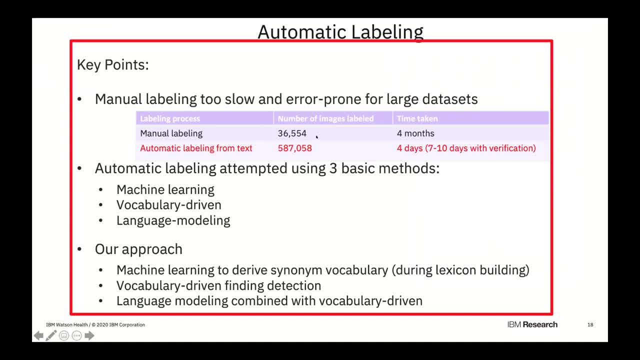 and about 40 radiologists. we could only annotate about 30,000.. And images in four months- and this was if you wanted to go up to a million images. this seemed like a tall order. so if you see many benchmark data sets collected, the number of images are also. 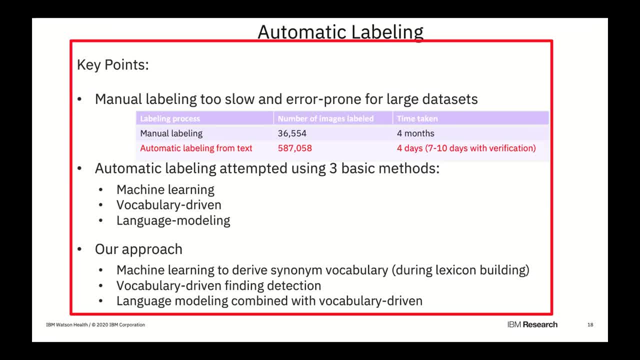 limited because of this manual labeling consideration. so we actually went ahead to develop an automated labeling method that allowed us to to label this in an accurate fashion. it actually used a combination of machine learning with vocabulary and language modeling approaches to to to come up with an accurate description of the labels as such and, with that, the labeling. 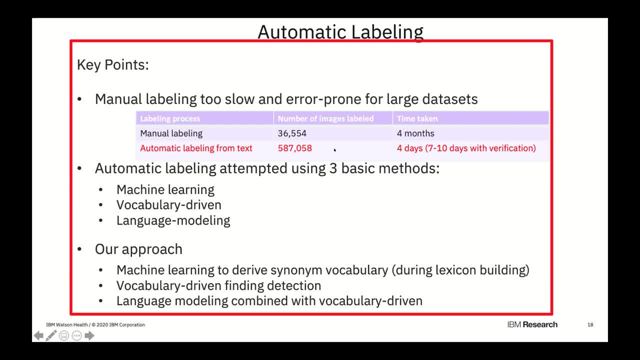 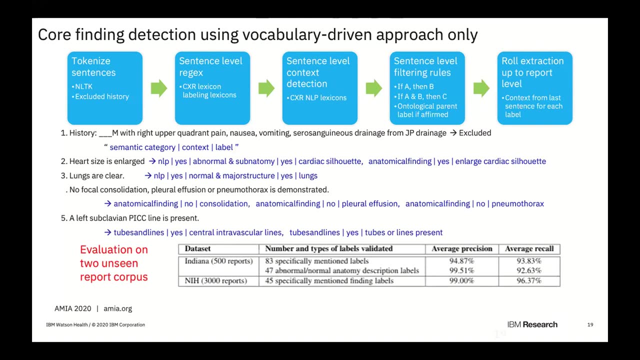 task. once the algorithm was developed, the half a million images could be labeled with verification within a week and the whole labeling process itself took only a few hours. so we evaluated this for purposes for core finding detection and, and you can see that, a typical pipeline used for text analysis. 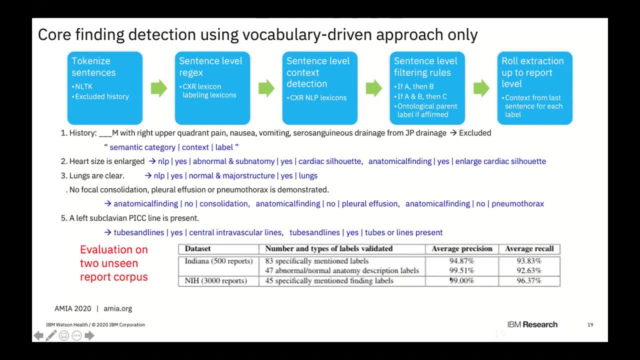 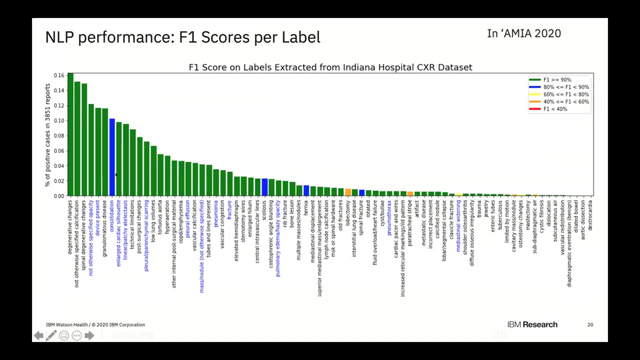 and the current accuracies for such things on evaluated on test purposes. this is also a work that we published in AMIA last year. the key features in here is the way the negations- negative findings- were captured in the descriptions, using pre and post negation rules and such, and the coverage for such findings. you can see in comparison. 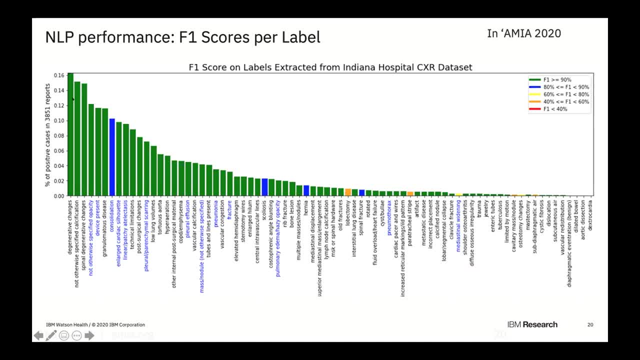 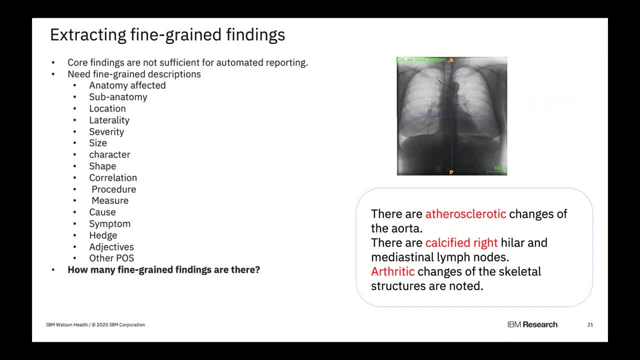 which we were able to use using the chest x-ray lexicon we had developed. it was to look at the variants of the spoken phrases and to recognize those synonyms and so on. But if you want to now group these findings with their descriptions that describe the locality, laterality and so on, then we need to go through a deeper language analysis, as 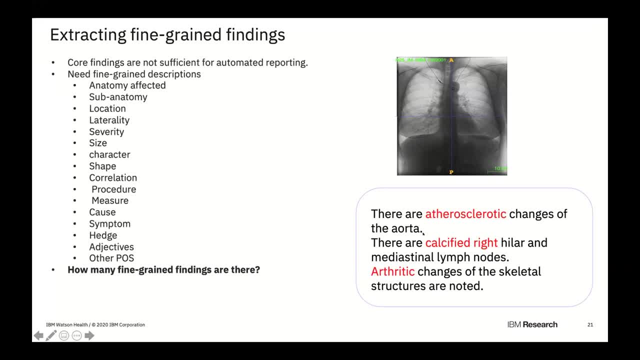 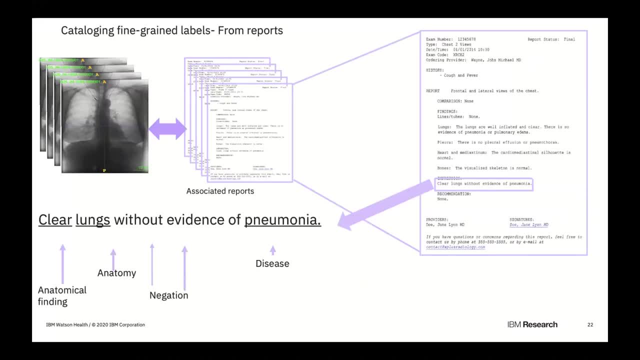 we go through those approaches. So, in this particular case, the highlighted phrases are some things that we would want to be able to extract and associate with the finding. The predominant way to do this has been to use machine learning, language generation approaches such as the transformer-based methods. 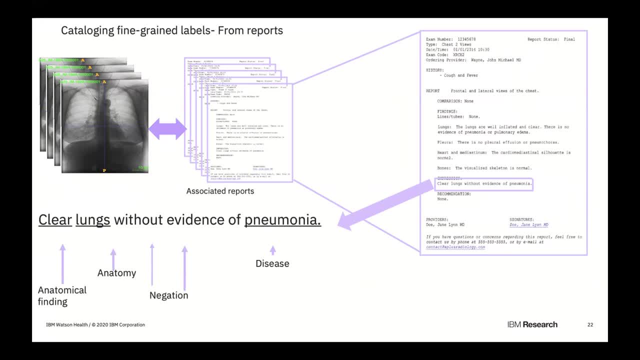 But those approaches, as has been our experience, don't guarantee clinical correctness, even if they can get natural language ways of generating. It was important to make sure that the findings that are generated from reports had to be clinically correct, So the labeling methods had to ensure that finding descriptions that we are capturing. 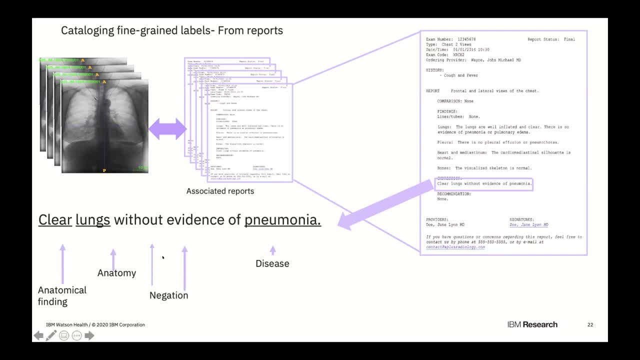 are clinically correct as well. So So the approach we use for that is to analyze the sentence and use the core findings to actually label the various elements. So, for example, we know pneumonia is a disease. Clear lungs is a description of a finding. 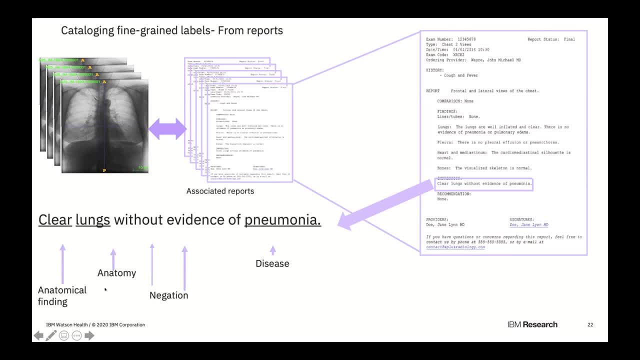 And lungs refers to an anatomy. So this information we can get from a lexicon. if you look at a typical sentence from a report- And these are the companion reports to your current chest X-rays- Then we use a text to describe the findings. 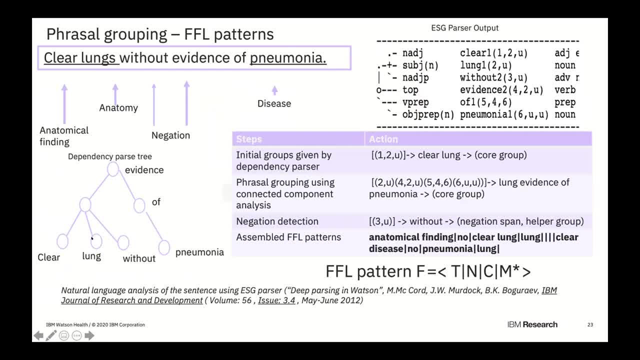 We call phrasal grouping, which does a dependency parse tree analysis of the natural language sentence and successively groups these into forming larger and larger connected components that link the core findings with the associated modifiers as well, And the modifiers themselves are also in our chest X-ray lexicon. 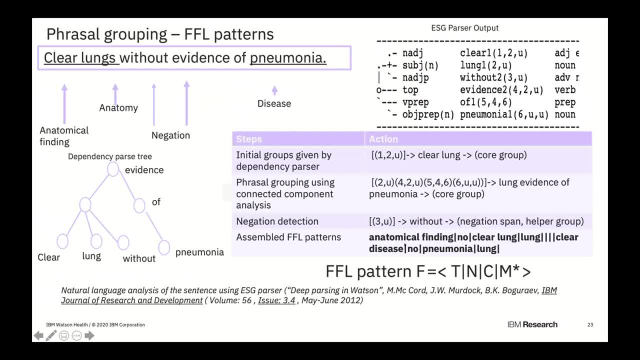 So for a sentence such as this, we can actually generate a finding that is an anatomical finding and it is a negative. It's associated with a core, the description of the finding itself and the one or more modifiers that refer to what section, what portion of the chest X-ray are we talking? 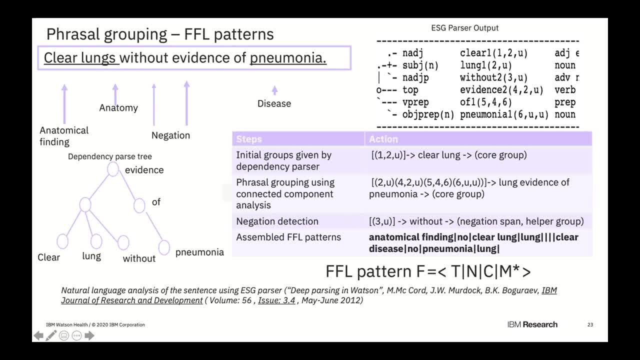 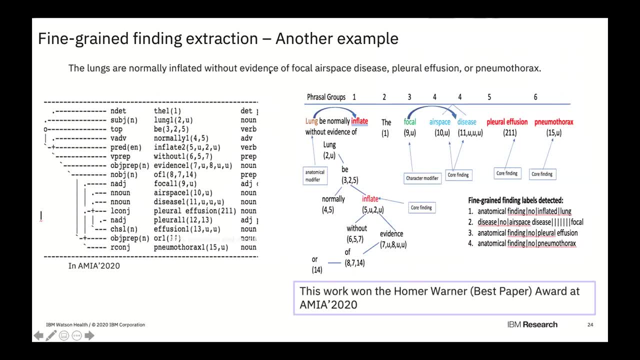 about, And it can also help describe the character and appearance of the finding as such. So here's another example. Given a sentence such as this, the lungs are normally inflated without evidence of focal airspace disease, pleural effusion or pneumothorax. 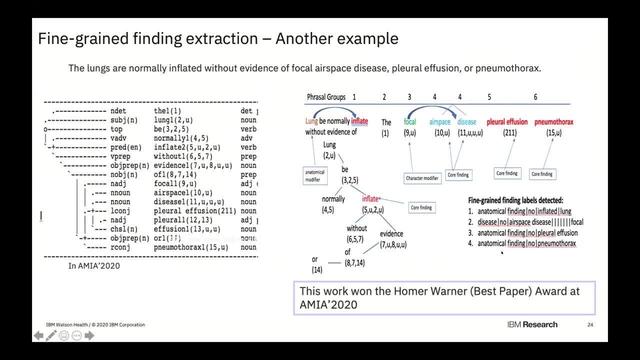 You can break it down into Four sets of findings. three of them are anatomical findings. One of them is a disease which is an airspace disease over here. Most of these in this case are happen to be negative findings, But this type of detailed description of findings enables us to do a fine grain label report. 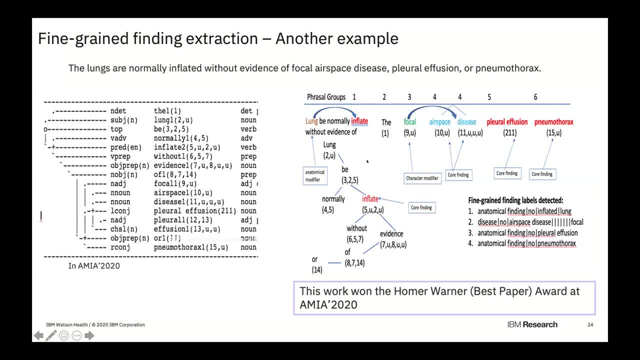 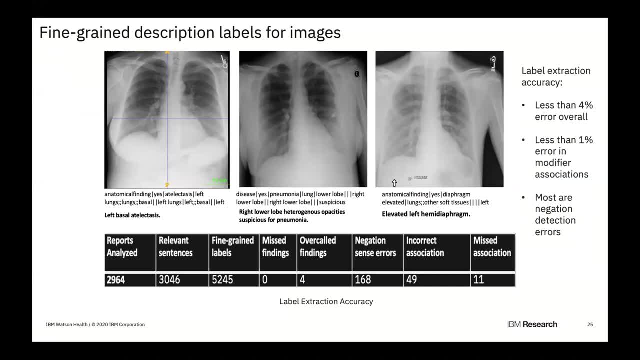 generation that I'll talk soon. This work, by the way, at AMIA won the best paper award last year, So from the fine grain descriptions you can see that it's easy to generate the label. So, given a finding such as this, it's an anatomical finding of atelectasis. 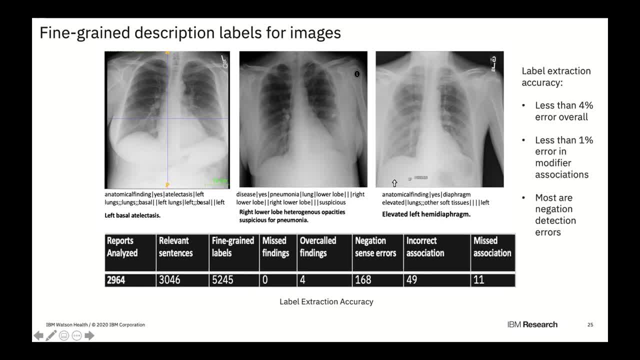 It's in the lung and it's in the left lung and in the basal region. you can issue a statement like left basal atelectasis. We actually analyze the detection capability for such label extraction accuracy for a number of reports in the Indiana collection. 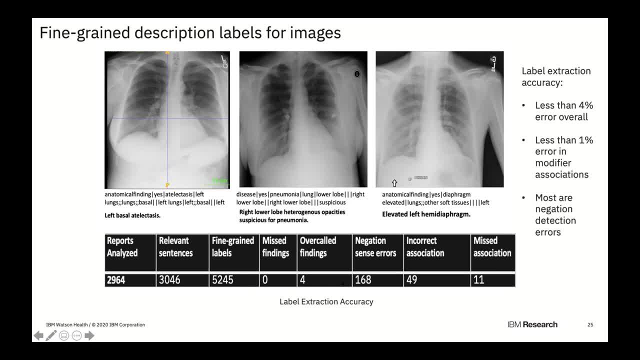 Again and we find that the label extraction accuracy is less than 4% error, but in fact only less than 11% error in associating the relevant modifiers. But the majority of errors are still due to negation sense detection, which remains a. 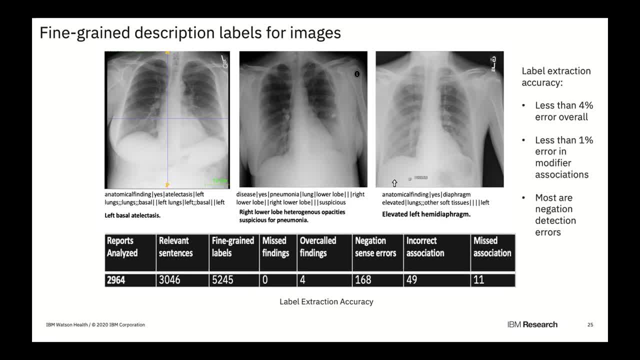 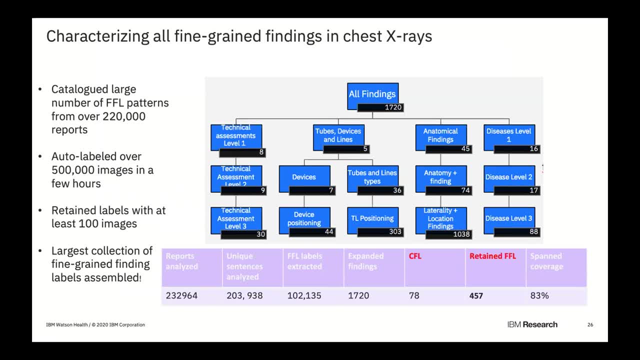 challenge in text analytics. So with that we now had to go to the next step of answering the original question we came, which is: how many fine grain findings Are there? Well, the lexicon gave us the core findings of the 200 or so are. if we were to now catalog, 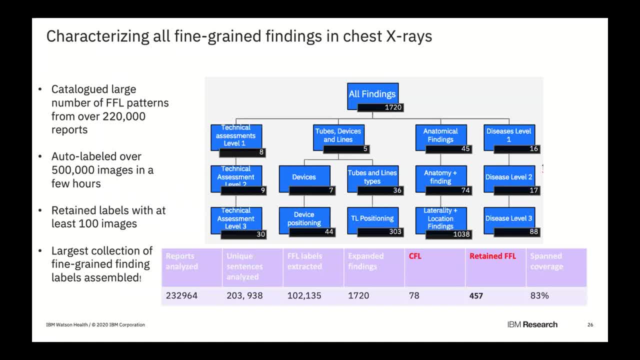 the full spectrum of fine grain findings for a machine to develop. you can see that there are many. In fact, once you use this pattern extraction methodology for about 200,000 reports, we found about 100,000 of these labels, But if you could essentially assemble and group them a little bit further, with respect, 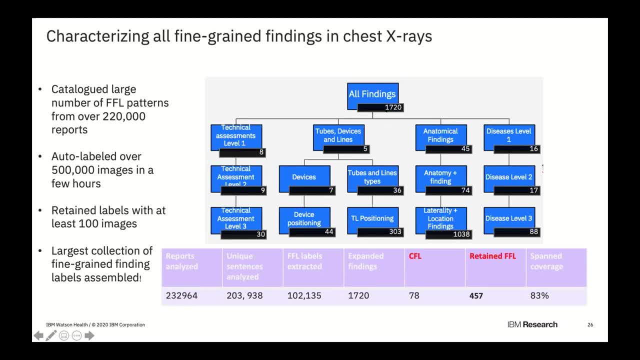 to the resolution at which you want to describe, You will still get about 1700 or so findings Once we analyze the descriptions and try to do a mapping of which of these findings if we were to retain, we could cover about 80 to 85% of the set of chest X rays. 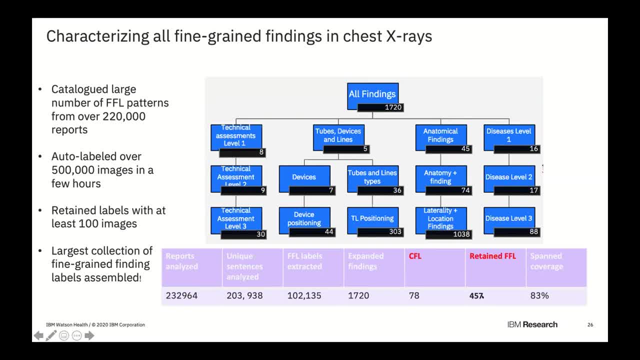 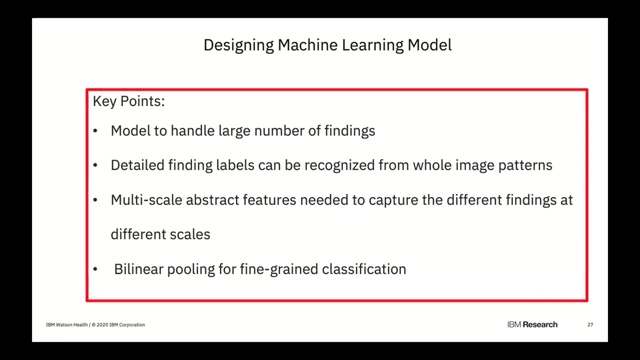 We were after evaluation and curation, we got down to about 457 findings. So this is the current set of findings that that we feel is sufficient to describe the findings in chest X rays and still generate a report that is of reasonable quality. So now we come to, we see that there is a much larger set of findings that had to be. 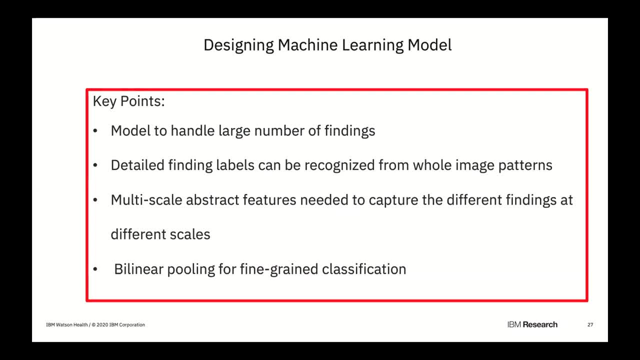 recognized by machines. But by using this methodology of fine grain descriptions in that derivation of the machine learning labels itself, the report generation process could be made easier. So let's go ahead and now build the models as we go from such label provided label images. 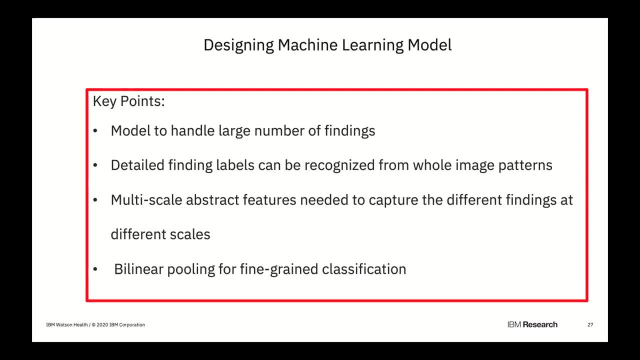 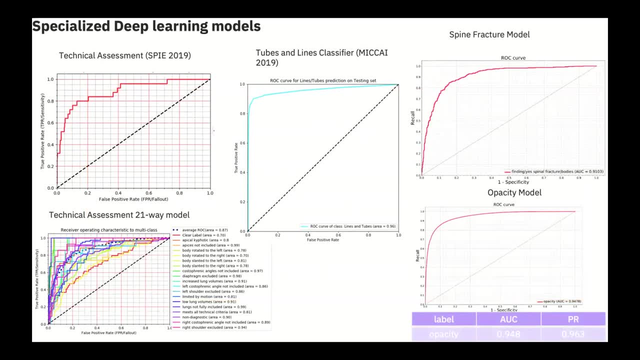 So the current methodology is auto labeling for images from their companion reports and we can go directly to building the machine learning models. So the methodology we used for this: initially we tried to develop a specialized deep learning models, thinking that it's better to divide up the problem and focus on each of these. 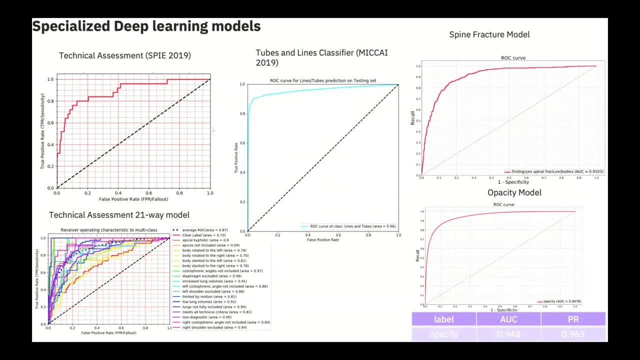 and do So some of the machine learning models we built. These are models for normal, abnormal discrimination, tubes and lines, classification, technical assessments. each of them can have their own applications as we go. But the interesting learning we had was that even if we break this down, the best performance 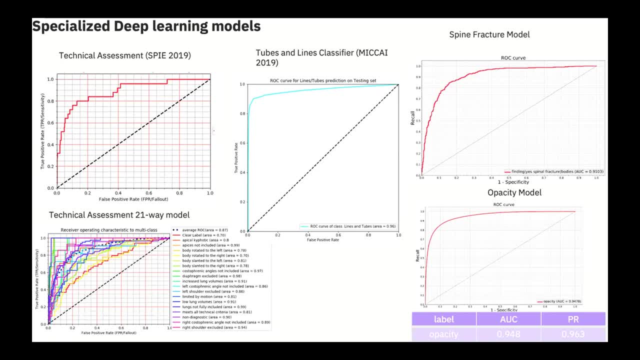 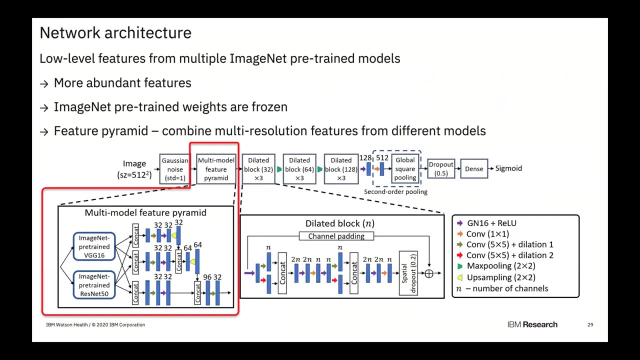 can actually be obtained by putting them all together into one machine learning classifier, And that way and so in the end we ended up keeping one classifier itself. So the next slide, please. So the architecture we adopted combines the good features of most modern machine learning. 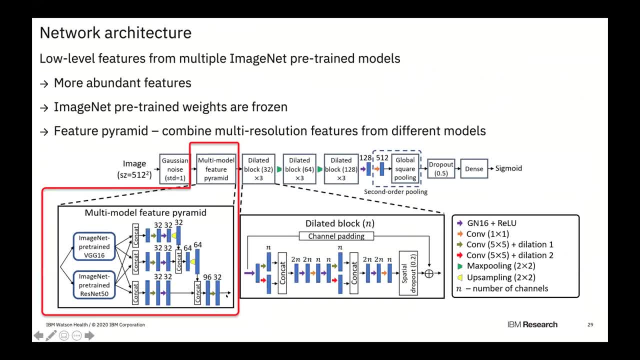 networks for computer vision, So those that are pre trained from VGG or ResNet-50 features. they're built into a multi scale pyramidal networks which give you multi level feature extraction, so to say, and capturing the various. So the architecture we adopted combines the good features of most modern machine learning. 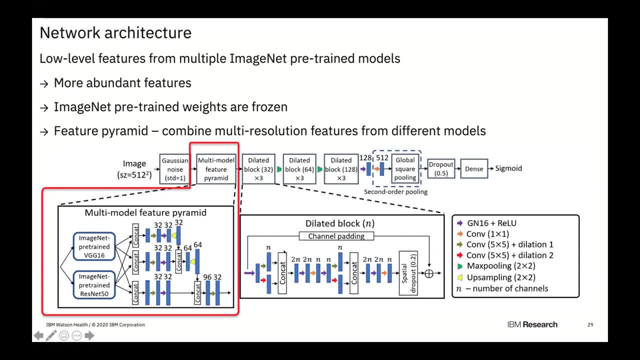 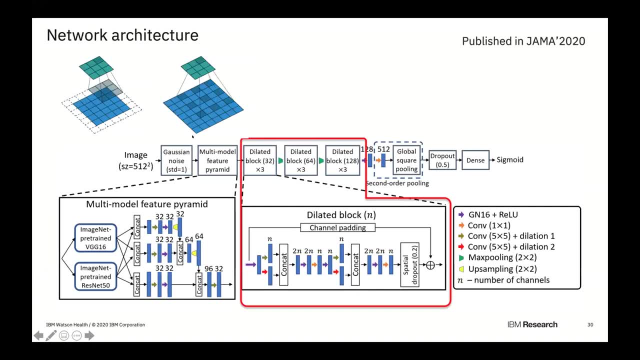 networks for computer vision. So the architecture we adopted combines the best features of most modern machine learning networks for computer vision. So these abstractions and describing the local and global abnormalities through dilated blocks. So this also gave us to the second feature in there that allows you to describe it at: 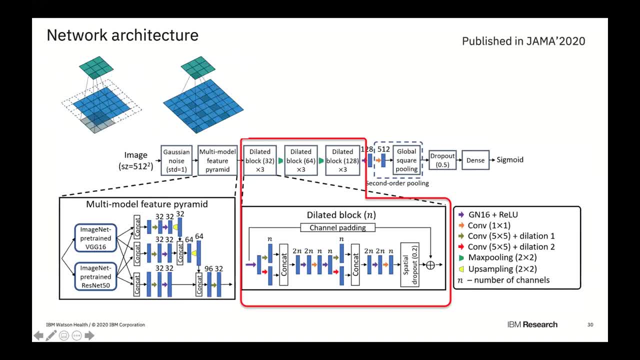 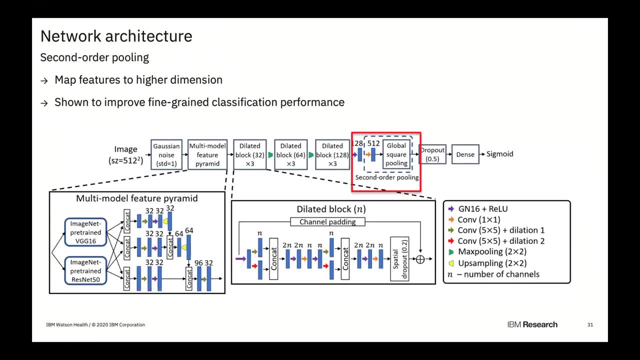 various levels of resolution, the anomaly itself And then, finally, a nonlinear pooling technique. we use that, instead of doing a flattening- that typically happens before you go through a classifier- you do a feature expansion through a global square pooling before you do the flattening. This allows us to capture nonlinear relations between features. 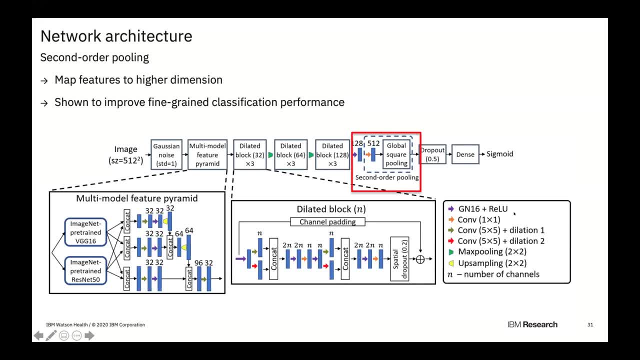 produced by the feature maps as such. So the details of the architecture, for those who can follow this along, is shown over here. The methodology we used minimized the number of parameters. you had to train as well, but even so, the images we were working with were. 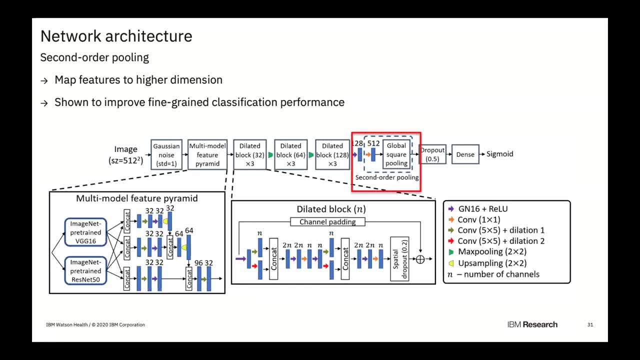 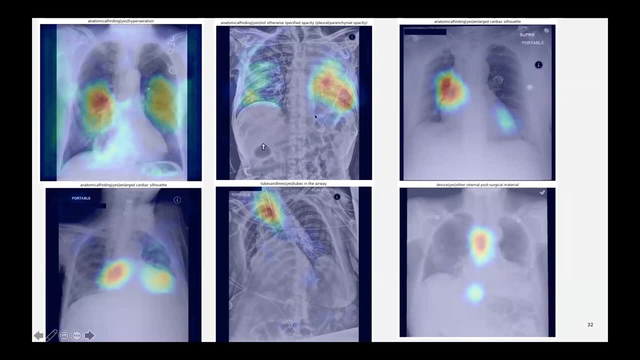 1024 by 2084 to begin with, so the training process took about 10 days to generate this machine, over a million images or so, And the results of these you can see is also doing a good job of localizing, although that was not in the plan but because the labels were fine-grained. 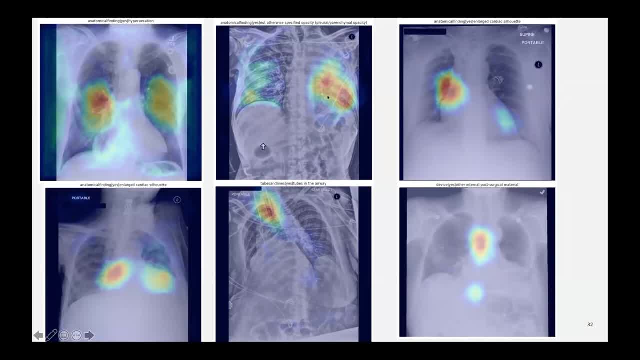 the machine doing the correspondence at a whole image level was still able to locate in relevant regions. So here you can see for a variety of findings, such as hyper-aeration, where it is focusing on the lungs, to tubes in the airways, where it is now pointing to an endotracheal tube over here. 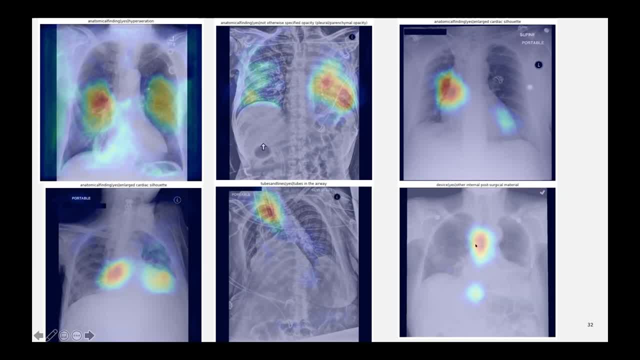 to looking at sternotomy wires that are found in a sports surgical material over here, and then derivations of a large cardiac cell head, which most people are able to get as well, being in the middle of this. But you can see this coverage from the variety of findings as well. 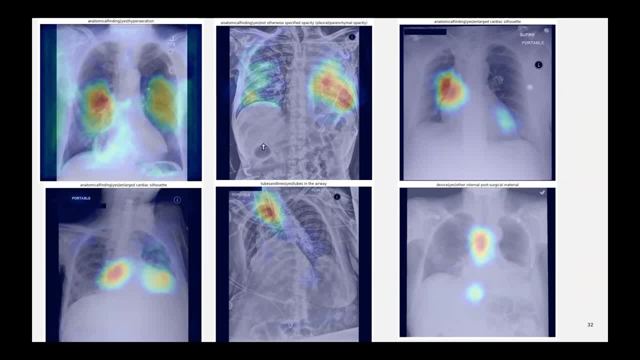 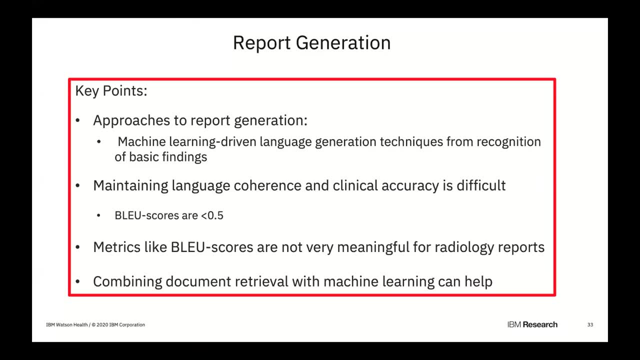 Now, in the latest work, we have tried to improve this, to actually guarantee that you're looking in the right place, and that will be some upcoming work from our team. So now we turn to the last task, which is to do the report generation as such. 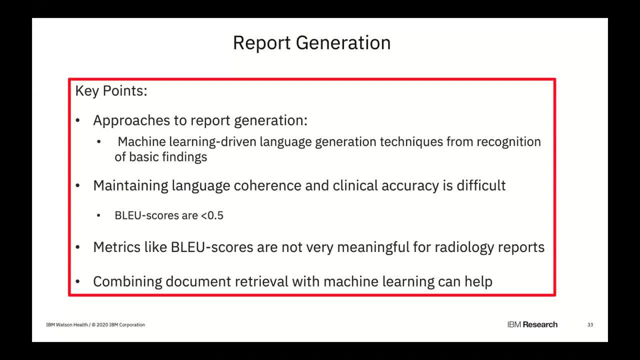 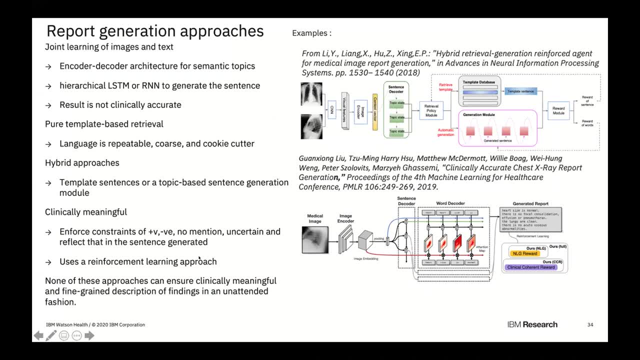 So the approaches to report generation, as I said, has been mostly machine language driven approaches and, as I said, this does not guarantee clinical meaningfulness of the report, even though there have been some improvements made in trying to incorporate some knowledge into this generation process. But the latest work that we have done represents the state of the art in 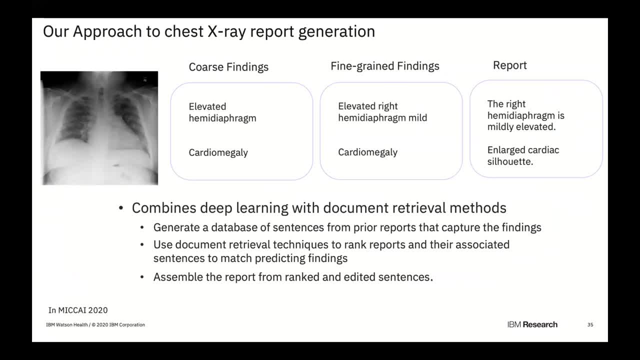 terms of the quality of the report that they generated by, even if you use the same blue score or rouge scores for judgment as you go. So the basic methodology: you start from the course description of a finding like elevated hemidiaphragm, then go to the next step. 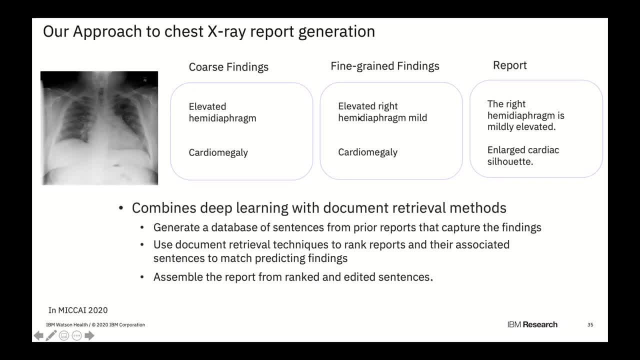 level of classification that describes a final grade. So it says elevated right hemidive from: mild and from there issue the statement. the right hemidive from is mildly dilated, So it's using a combination of deep learning of both coarse and fine-grained deep learning using 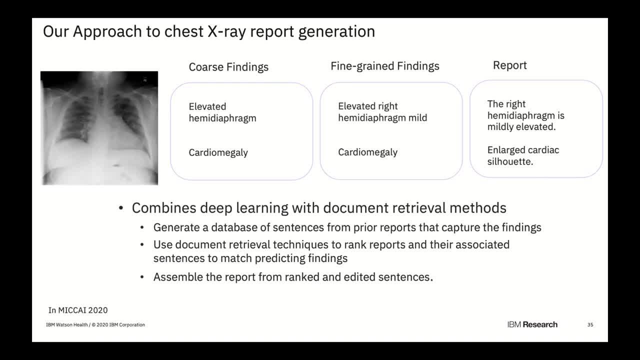 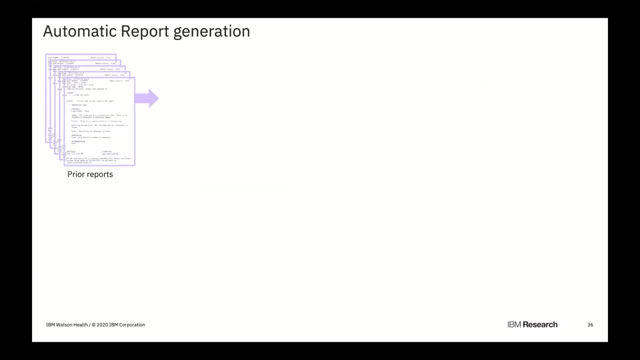 fine-grained labels to begin with, but then combining it with a documentary technique to actually generate the report. The overall workflow is like this: You start from a prior set of reports to actually extract fine-grained labels from them and form these fine-grained label. 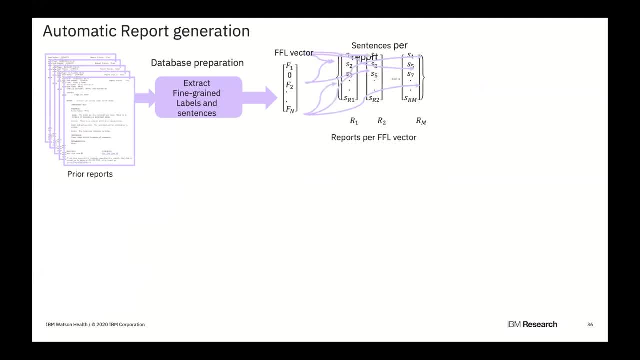 pattern vectors, called FFL vectors. From there you back-index to the sentences and the report so you know which finding label came from which sentence and which report. And this set of pre-processing goes into a database so that you have a set of pre-ranked 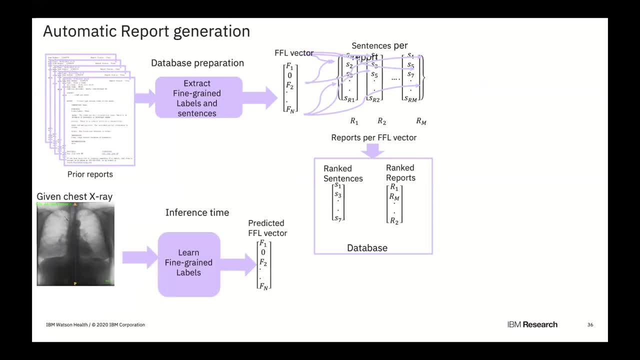 sentences and reports. Now given a new chest X-ray, you would go through the additional pre-processing and then you would go through the pre-processing, and then you would go through the additional pre-processing and then you would go through the additional. 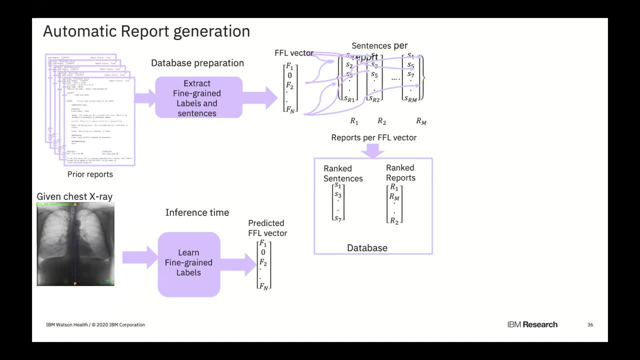 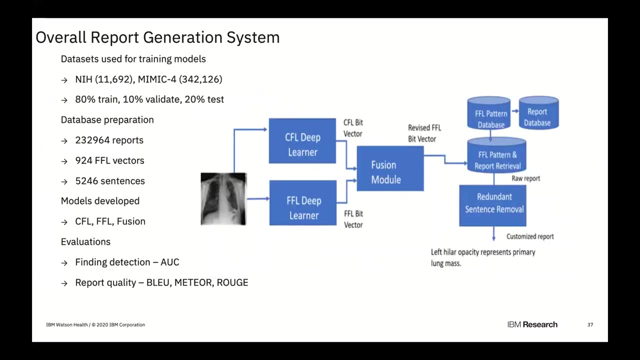 inference time, learn and classify the fine-grained labels to form these vectors and use that to index into this database to retrieve relevant sentences, And then you take the fragments of findings that correspond to the relevant deductions within the chest X-ray to reconstruct a report and that's the overall process that we use. So the overall report. 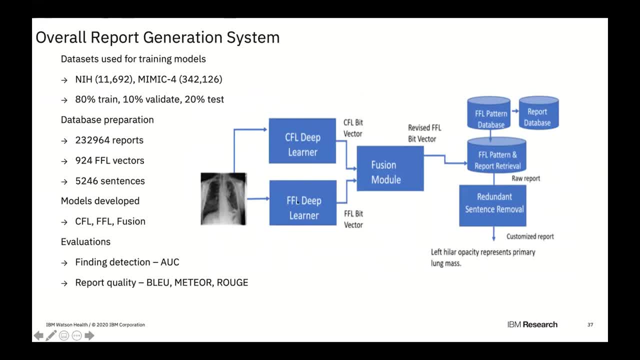 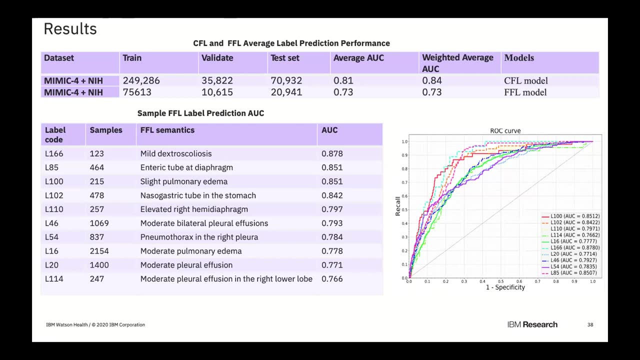 generation system has dual learners, a core finding and a deep finding, and a multi-model fusion model that actually tries to combine the findings followed by a core generation stage And the details are described over here. And if you take the overall evaluation by putting them to all of these together, that both the fine-grained and the average AUC for 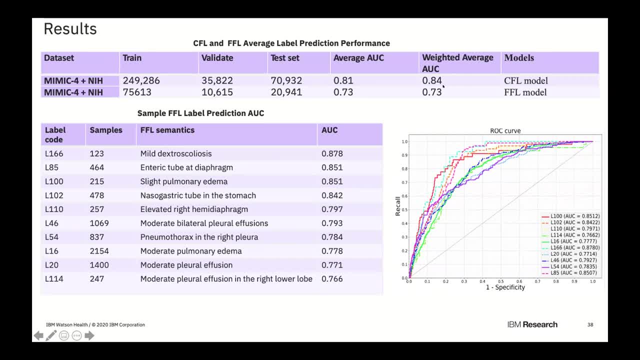 both core-finding models and fine-grained finding models. you can see as here. From here you can also see that the fine-grained finding detector's accuracy is lower than the core finding reduction, as expected, but for the majority of the findings. 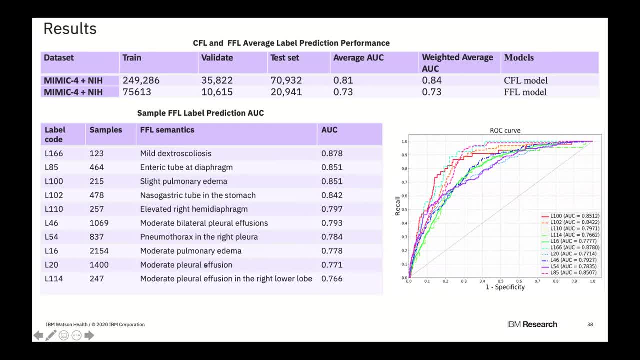 even the findings maintain decent accuracies, But from the nature of the process you can see that you can directly emit a label that says things like moderate pleural effusion in the right lower lobe, whereas most classifiers would simply say pleural effusion at best. 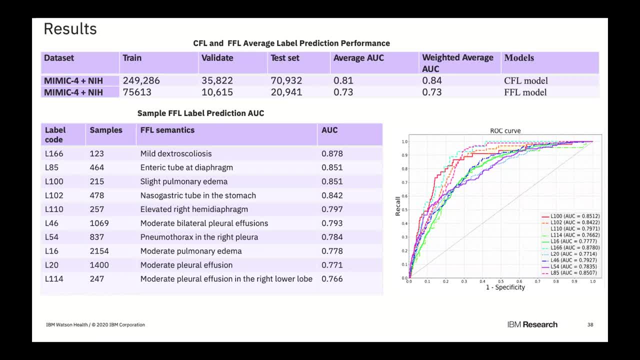 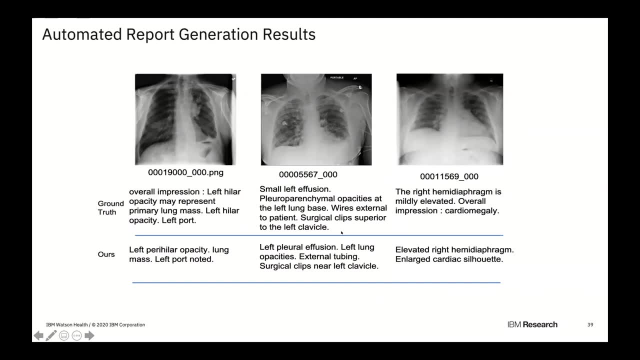 so severity is assessed as well as laterality and location. So here are some examples of automatically generated report, and you can see that the report that is generated is guaranteed to be natural language ready, because we are picking up on prior sentences and reports. However, the methodology of assembling the sentence is 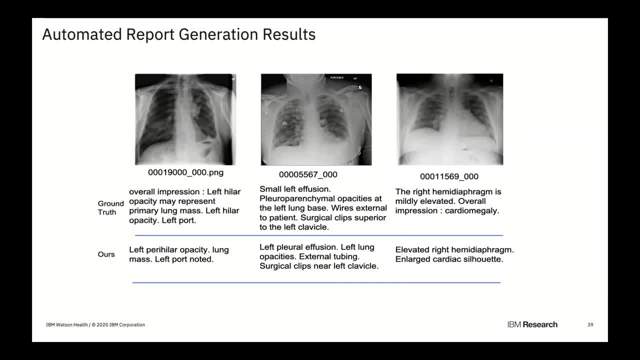 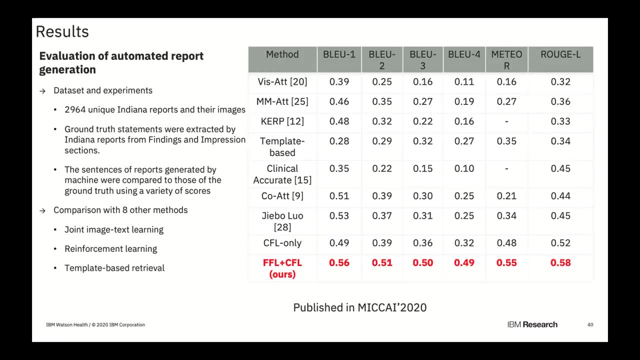 focusing on the relevant findings and making sure that these findings are actually likely to come from a report with the joint application. So the occurrence of these findings is also likely, and these are the two features that distinguish the quality of the report that we generate. We did an evaluation against a variety 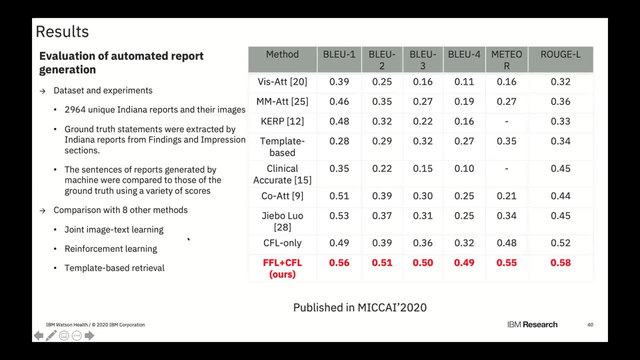 of methods and this was published in MechEye last year, so you can see the comparison with different methods in terms of joint text learning or reinforcement learning or template-based retrieval methods that have been used And to date. I think this type of quality is, every year, the 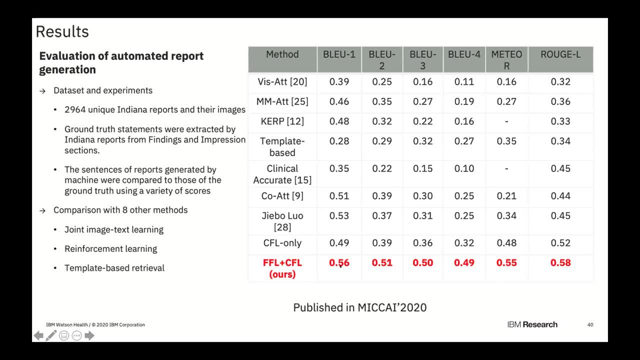 quality will improve but as of last year, this was the best quality report that could be generated. We have to say that the quality judgment through these lexical or even partially semantic matching scores are not really a good indication of how good the report is from a clinical standpoint. 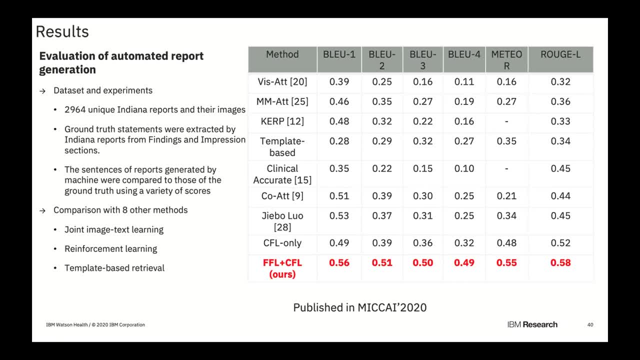 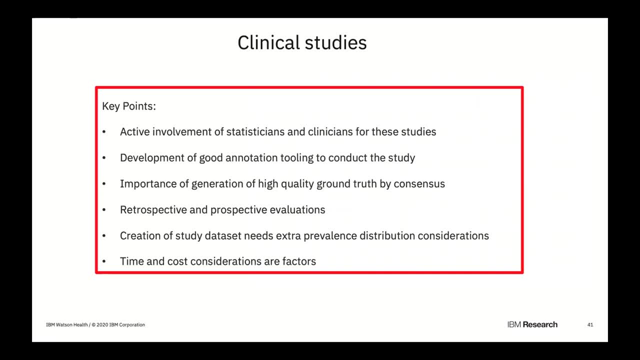 and actually new metrics need to be developed to do the assessment of these as such. Okay, the last section. in the few minutes I have left, I will talk about the clinical studies we did to actually assess the performance of automatic report generation, both in the cataloging of the 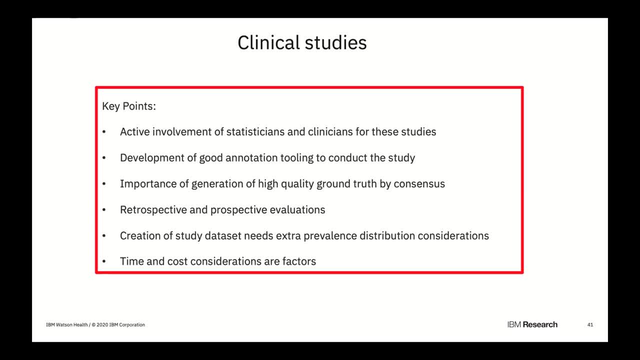 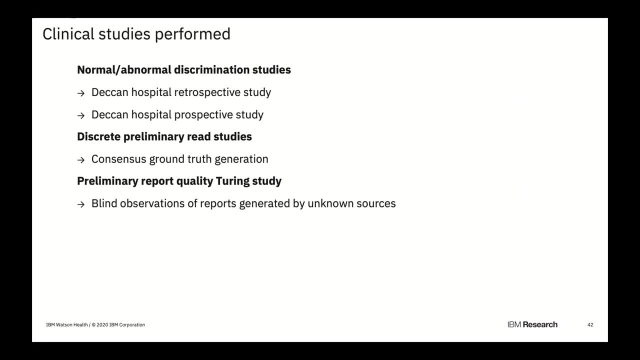 findings and as well as in the evaluation in comparison with clinicians. So the clinical studies we performed are for normal-abnormal discrimination as well as for discrete preliminary studies and the report quality reading, which is a Turing test we gave to the machine versus the radiologist. The normal-abnormal discrimination study was something that we conducted in an 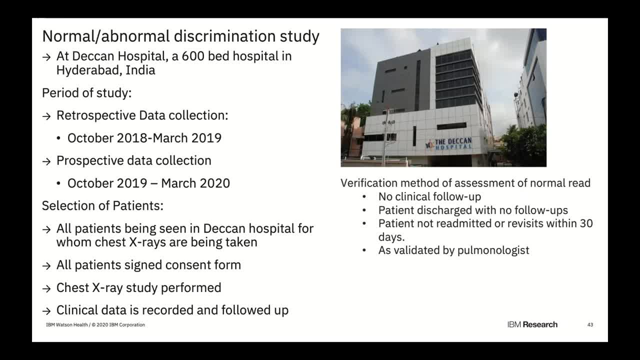 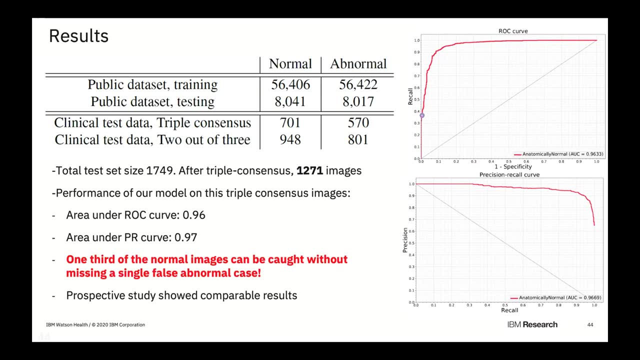 using international datasets, which is a trained model on US datasets, and then performed, tested it on, in international settings. So this was done under an inappropriate IRB. Again, given the interest of time, I'm going to skip through some of the details, but you can see the main result. 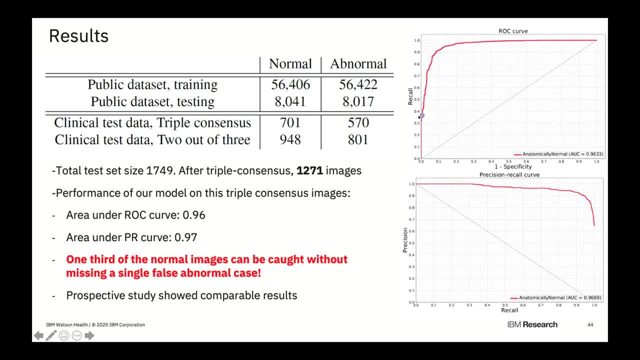 said that we could filter out as many as 30% of the normals without missing a single abnormal case with the classifier that we built when tested on a brand new field dataset as such. So this points to a potential utility of such tools for normal-abnormal discrimination and reducing the 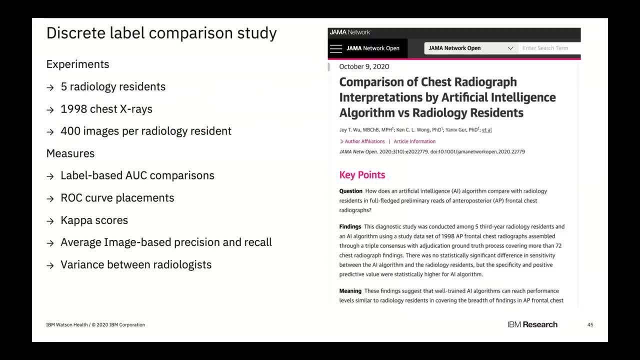 expediting clinical workflows in some sense. The next study was a discrete label comparison study that we reported in JAMA last year. Thank you, Dr Saeed Mohammed. So we only have one minute, Dr Saeed Mohammed, So we can discuss more about these studies, The overall result of it. I will probably say that 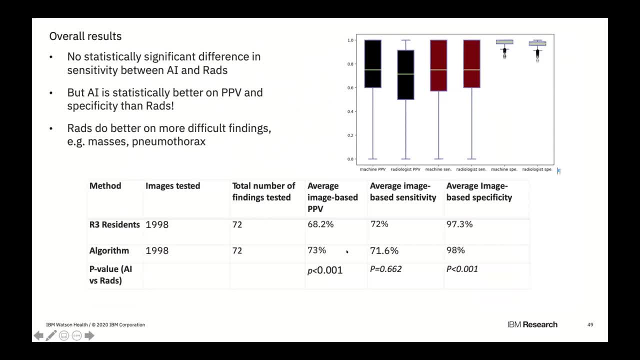 the average sensitivity and specificity of the machine was comparable to the radiologist from this particular analysis as such. So maybe we'll stop there and leave that as the overall result that by building carefully these models and using a well-known, documented process, we were able to. 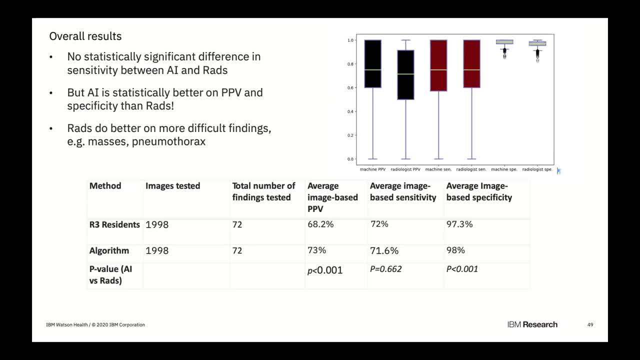 reach a comparable performance to radiologists. for the particular task that we took- And this is in comparison to radiology residents- that showed that the sensitivity and specificity and the positive predictive values are within the ranges of what the radiologists are able to achieve in the automated report generation task that we took on. 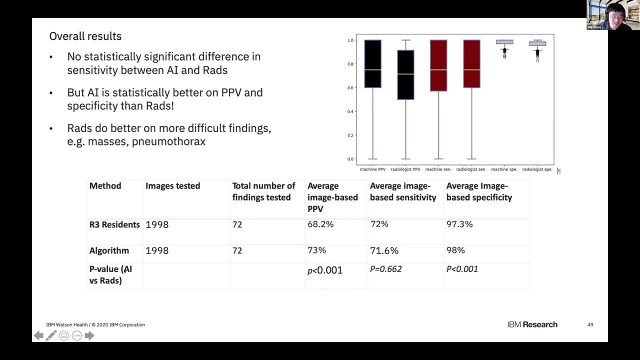 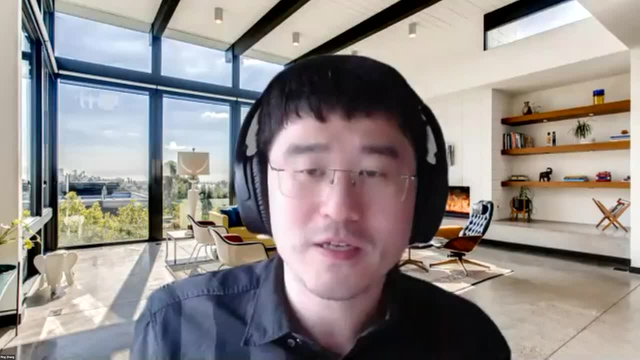 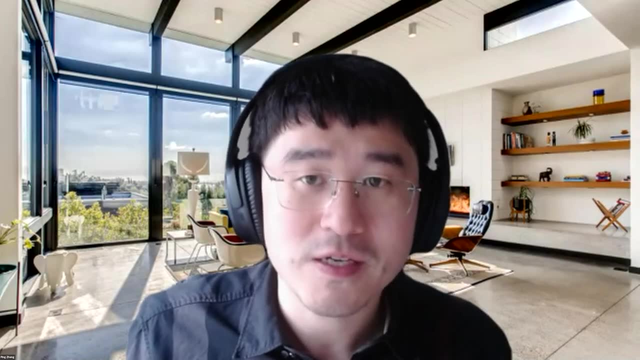 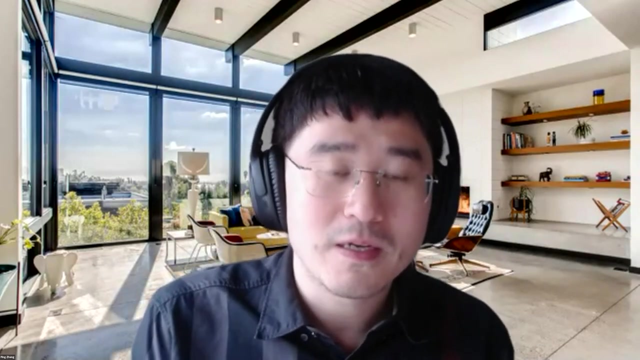 Dr Saeed Mohammed. Thank you so much for the excellent talk, Dr Saeed Mohammed. So we also received two- at least two- questions in the question and answer, So let's discuss in the panel discussion. Thank you so much. Our second? yeah, thank you. Thank you so much. Our second speaker will be: 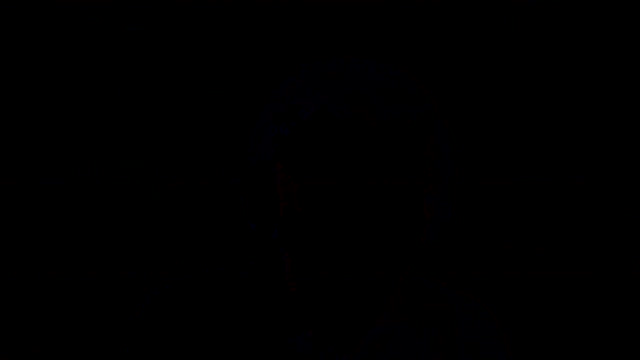 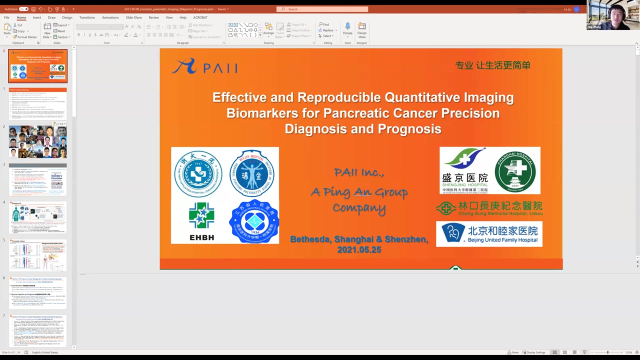 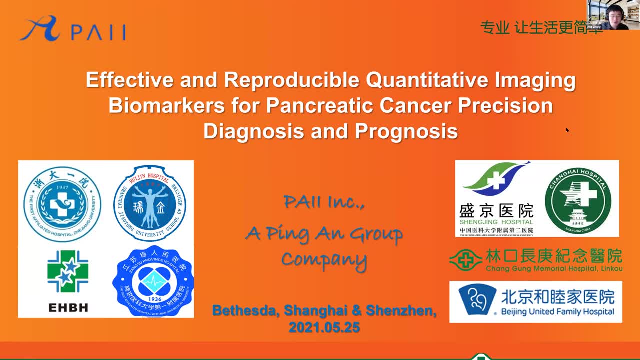 Dr Saeed Mohammed. Dr Saeed Mohammed, Actually, he is a researcher at NIH and also the director at NVIDIA AI Infrastructure Divisions. He is an IEEE fellow on medical image, AI and oncology image. He also is a social editor for PAMI and many other. 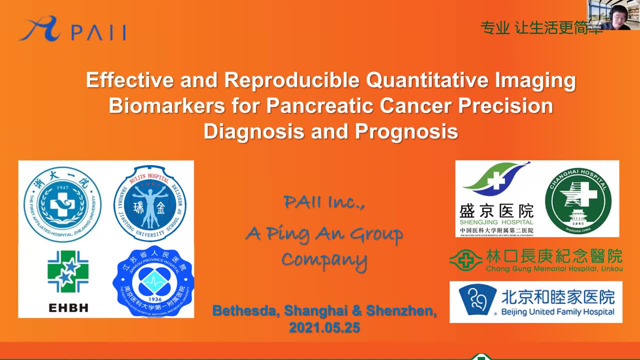 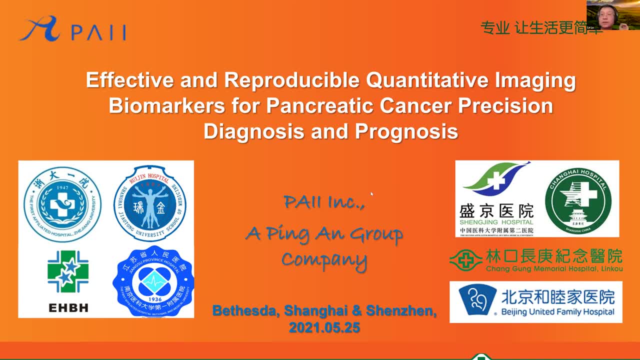 Dr Saeed Mohammed, Dr Saeed Mohammed. Okay, So you can see my screen right. Dr Saeed Mohammed, Dr Saeed Mohammed. Yeah, Excellent, Dr Saeed Mohammed. Yeah, today I'm actually going to discuss something new. It's not really new, but 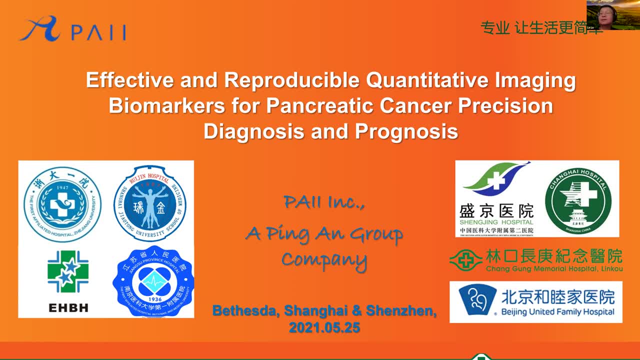 they haven't talked about this. We're only starting to talk about this topic, like starting this year, but this work has been done than in a couple of years. So the purpose of this work is: we talk about the pancreatic cancer. 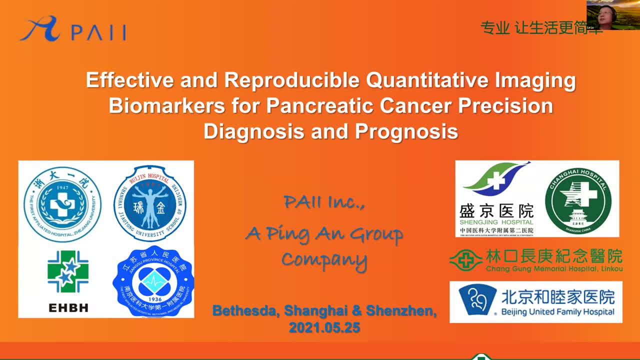 which is one of the hardest cancer for prognosis. So the basic concept here is trying to show the whole pipeline, you know, from diagnosis to precision prognosis, prognosis, deep prognosis and even like a treatment response. So as far as I know, I have been working on 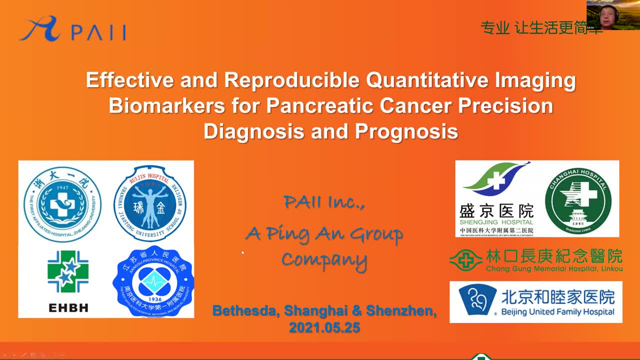 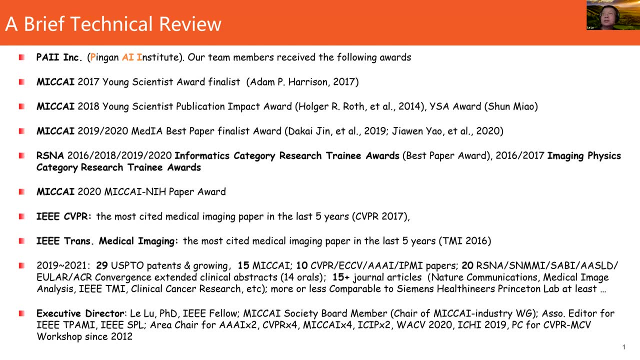 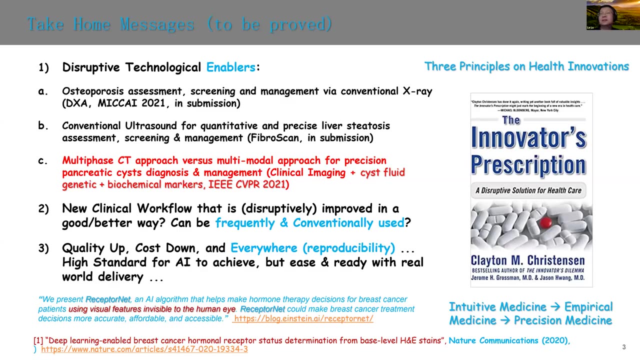 I have been working on. can I see my okay? So this is a couple of words. we won in the last couple of years. This is our current team with interns. So the topic here is really about- I'll give a showcase about- one of the most difficult cancer case. 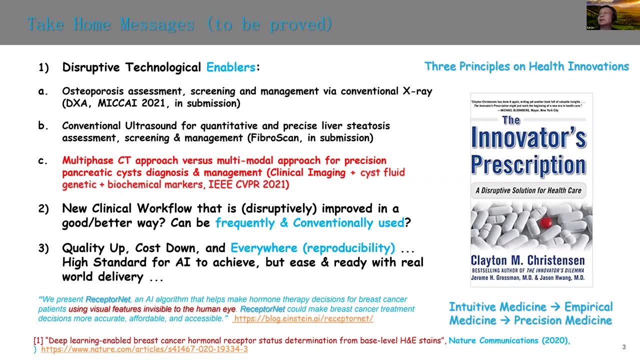 and our recent work. Most of the paper was copied last year or this year. has not been very present in the conference yet, but you got preview, So you know this is actually my slides. I give talk. you know several places. 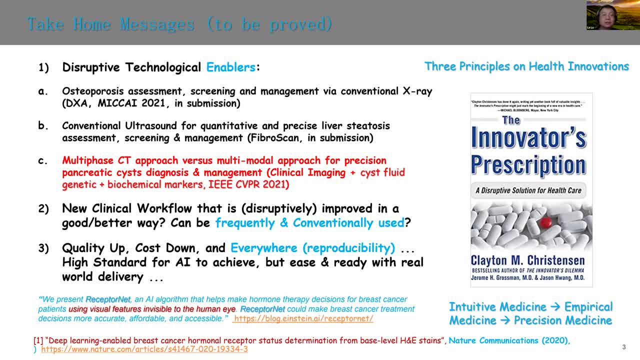 So you know we are at the industry right or industry or hospitals. What we do is really for, you know, traditional medicine. You know we don't just public paper for five, It's really for patient care, you know. 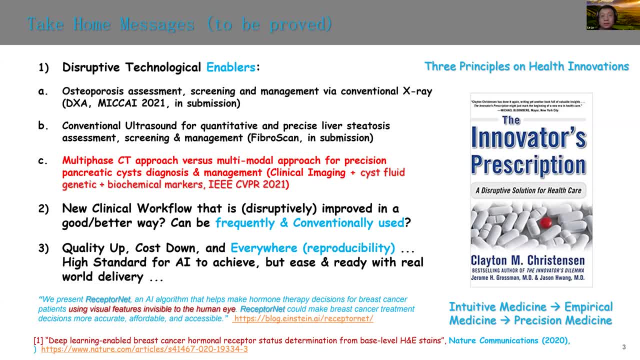 Siemens. you know, in my first six years of my professional career with Siemens, then the last, then the next five years was at Edge. So you know I'm pretty much like a very, very influenced by Siemens and Edge. So I'm very clinical relative. 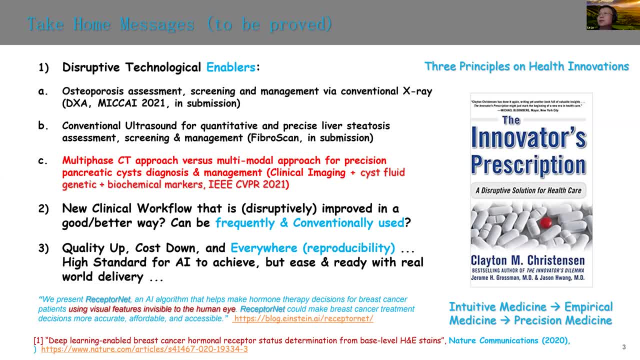 relative. compared to other industry researchers, I'm more clinical, yeah. So basically we all think about it. is you know translational medicine and how would we make things that will work in a practice that will help patients right? So the three things basically. this book has been popular. 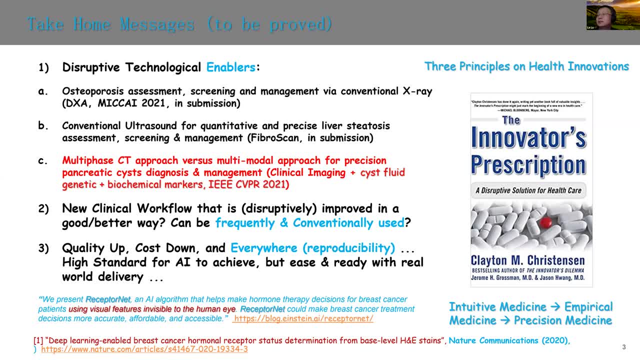 for more than a decade. It's a very it's excellent book about you know how to make things work, how to make you know healthcare cheaper and better. So basically, right now, many of the things we do is really intuitive medicine. 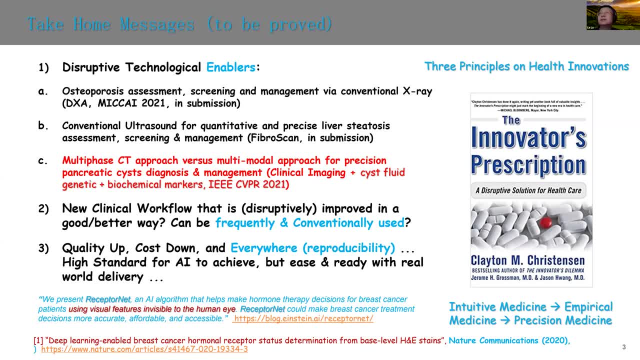 means like when you know I would take examples later on. I would give the overall message at the beginning that I used my material to prove that right. So right now, still many things. I mean especially for cancer care. you know I'm mostly oncology. So for the cancer care is in even US it's a lot of like the inequality you know, 85% of the patients. they cannot be treated as the top 50 NCI certified cancer centers, right, And even in those kinds of centers it varies a lot. 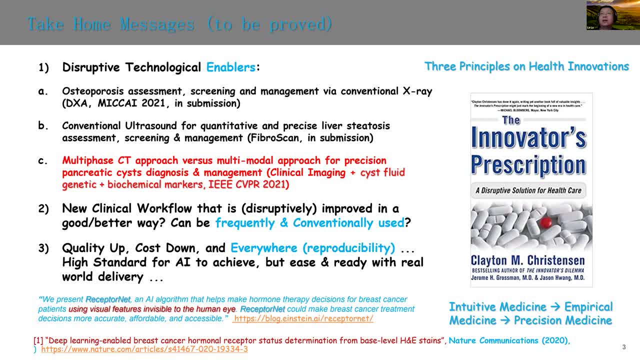 And this: there are certain things it only can be done, maybe by one or two, the top list, like hospitals on the planet that can do certain things for a certain lucky patient or non-lucky patient, right? So really like, what we do is trying to make intuitive. 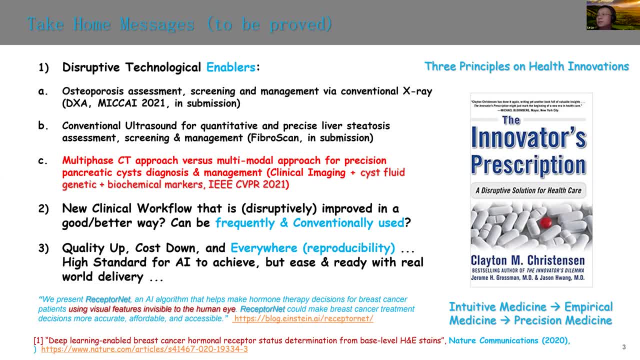 medicine that can only be solved by the top expert into the face of empirical medicine. Empirical medicine means, like there will be, you may understand, there will be a lot of computing, a lot of reproducible communication process that can be easily translatable, right. 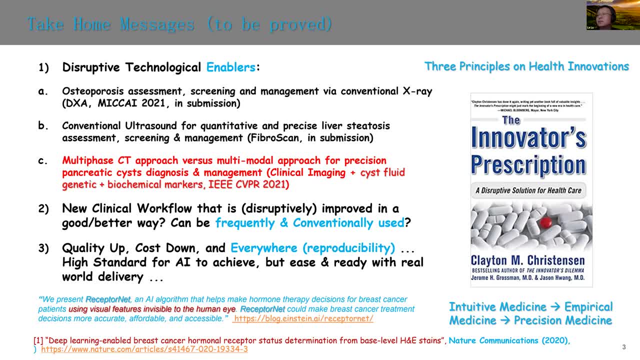 Even we want to go to the face of precision medicine. We're not there yet, We're still in the model of the empirical medicine, but it's fine. There's a lot of things you can do in there. So you know people talk about the. 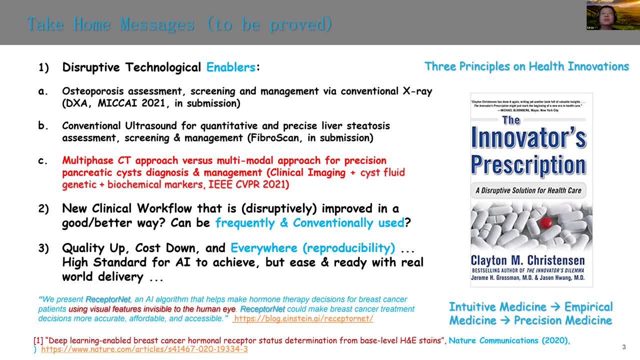 the three principles about this book is about how to make things work, especially in healthcare. So people talk about a lot of disruptive medicine, disruptive technology, especially in the city of Kalamati. Really, I think the thing that was something you know. 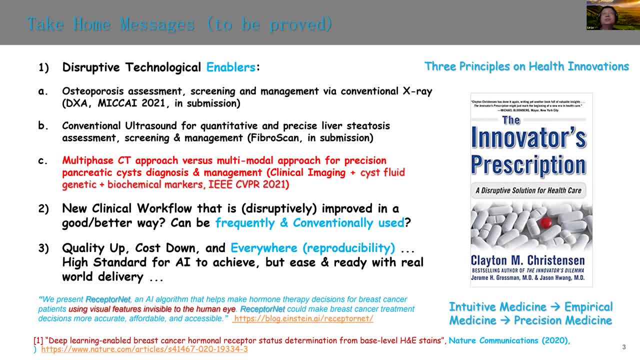 that was something that was really important to me, you know, when I was meeting with the enablers. you know what we do can make some nice thing happen, some nice thing possible, feasible, reproducible and useful right. So I give a few examples, and actually three example. 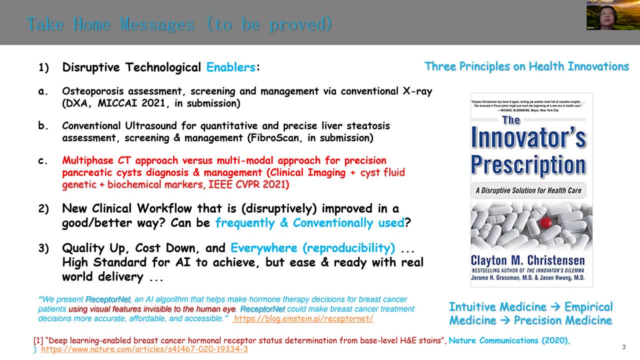 from our own work and the one example from USC, the paper is. it's popular this year. So the AI, what AI can do, or what deep learning can do, is really I think deep learning is really a nice thing. I'm not sure you know a lot of people. they still. 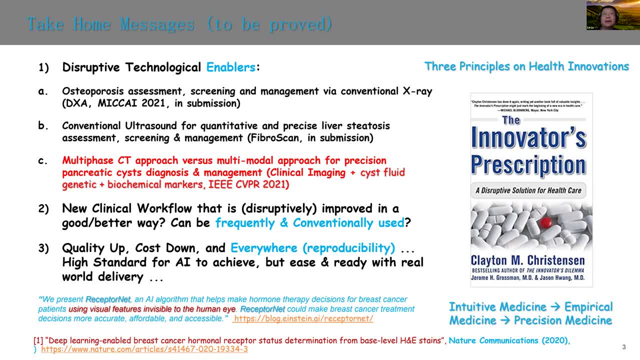 if you are still hesitant or you have a question mark, you should not based on my opinion, So I moved to. I moved to, like in the year of 2012.. Then, in 2012,, I decided to move to IH. 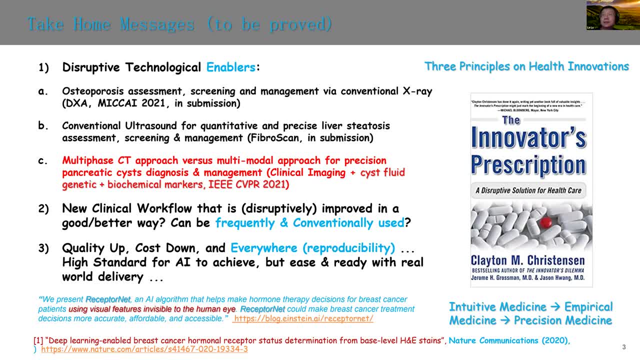 I make it happen in the January of 2013.. I remember it was a very cold January. I drove by myself from Pennsylvania back to Maryland. Yeah, The real reason is I feel we can make deep learning work in medicine, in medical, in being per se. 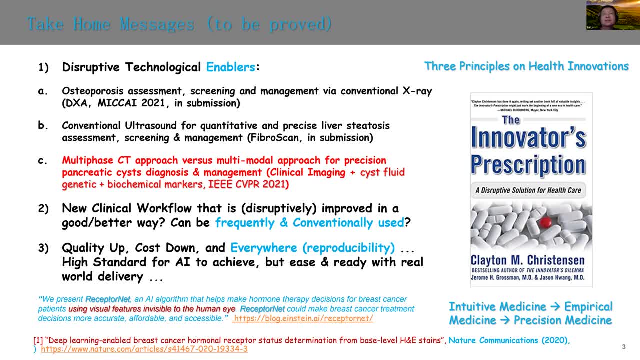 I will make it happen And the you know, with this with you, some working at IH was highly influential, but I think our recent work is more make me more excited because it's very translational. I'll give you three examples. 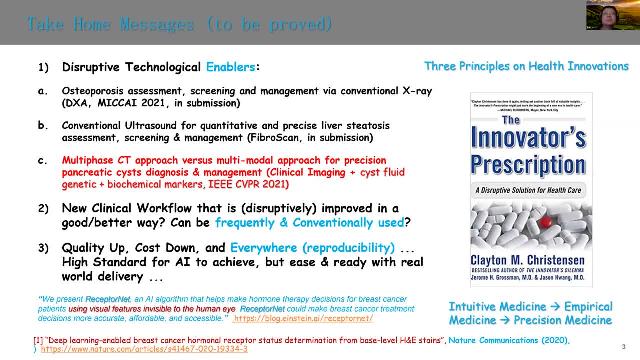 So the first work was published in McKay this year and it had not to be published by early except and we have a clinical paper that's under review. So basically we can do osteoporosis using conventional x-ray, So it was not possible. 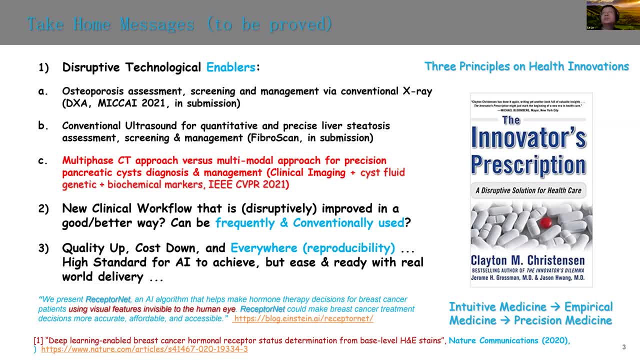 And you know the current is by DSA And what we do by conventional x-ray is really for optimistic screening, because a lot of patients actually have such kind of disease but they were never sufficiently screened. So this disease is under-diagnosed, under-treated, right. 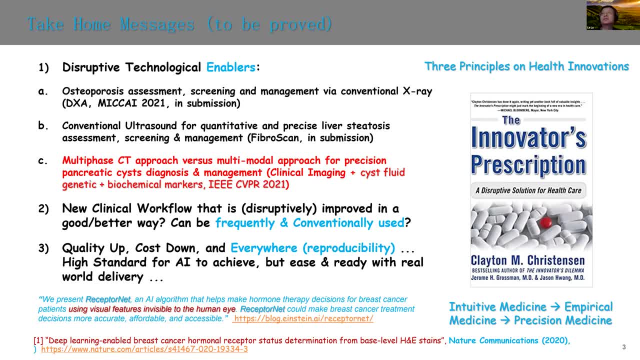 So if you know, you imagine all the hospital, you have a lot of x-ray, you know matter. there's a chest x-ray, it's a lateral vertebral x-ray or a hip x-ray, right And physician, the top physician. 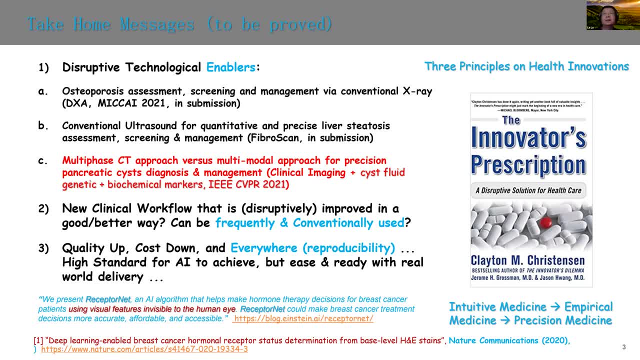 actually not from the radiology department, from the rheumatology department, they actually they can guess if this patient has osteoporosis or not, right? So this domain expert, they can guess. But this is the thing, it's not translatable. 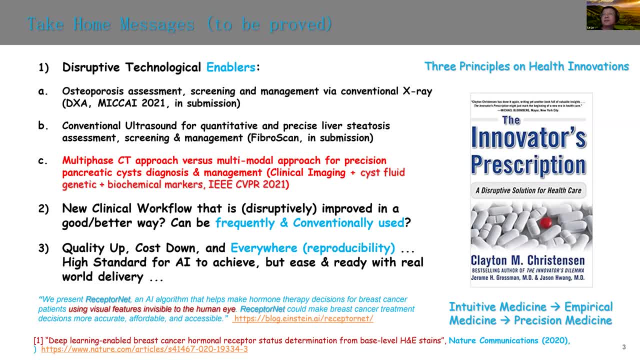 It's an intuitive method. You have to have top expert. They can guess for a few, you know. But we make a computational tool and we can achieve the quality as good as the Hologic DSG machine or a GE DSG machine. 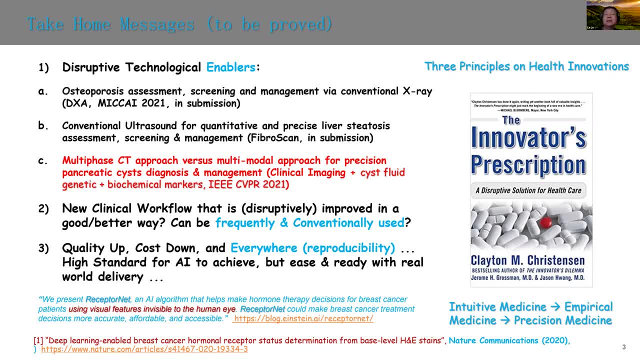 So that's the work. the first part of work with the to be and the clinical work is right now under revision. It's not in some, it's already under revision. The second example is actually, you know, to precisely access the quality. 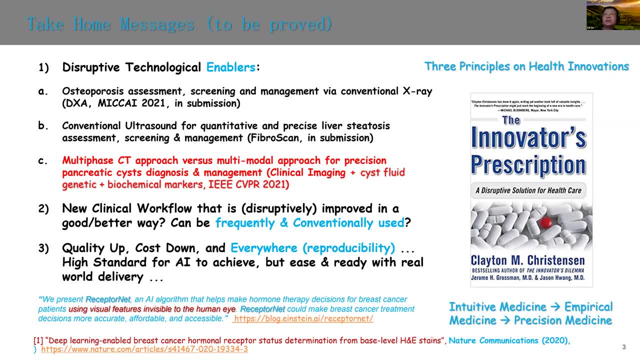 or the quantitative score of the liver steatosis, right. So right now, the machine. the thing was, the clinical practice was done by FibroScan. FibroScan is a special machine, special ultrasound machine, like an electrograph, And it has some problem. 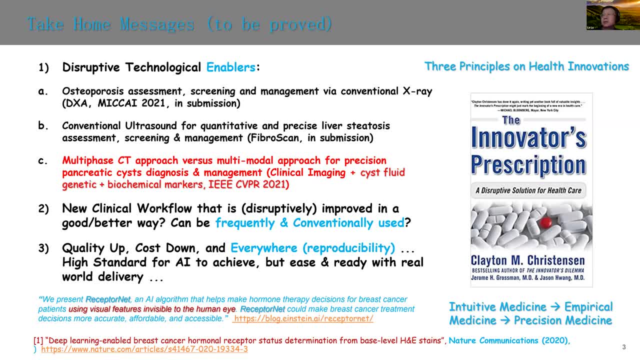 And basically our deep learning algorithms. of course it's not easy, It's a lot of work And we can achieve the quality better than FibroScan by right by, let's say, FibroScan's published AUC score is about 0.85. 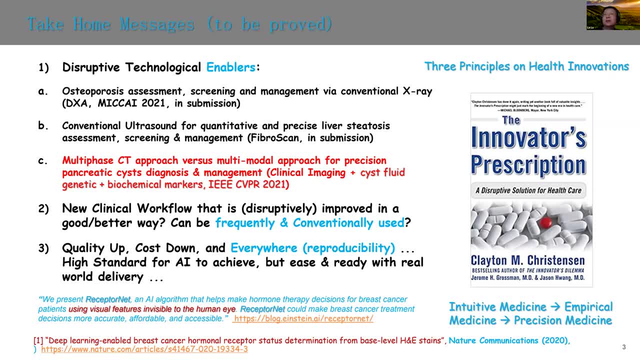 And we are at AUC 0.95.. So we're noticeably better than a expectancy machine And also we generalize better, we cover better, because the electrograph is actually sensitive to the liver inflammation. And but our argument, our imaging modality, 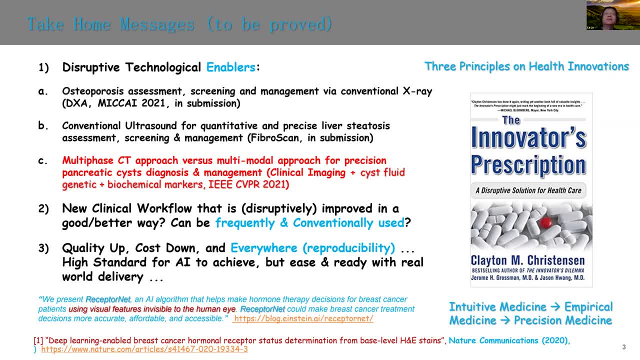 and algorithm are more stable. Okay, So that's that right. But this, this is a two topic. I would not be, because the time issue I we already partially published about you know, because time we're not going to talk about here. 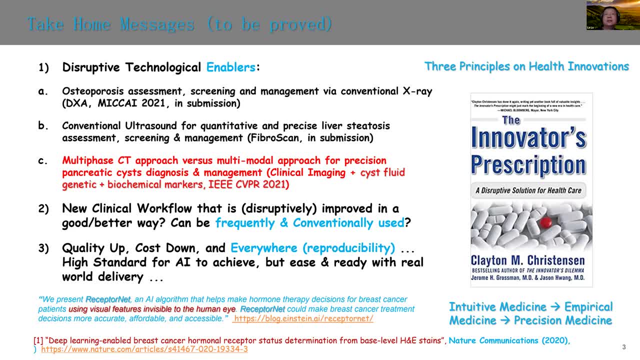 but I will focus on the third And then I will talk about the third. you know that's using multi-phase CT imaging We can do a precision diagnosis for pancreatic cysts. Pancreatic cysts means like all the tumor, like 10 types of tumors and the patient management right. 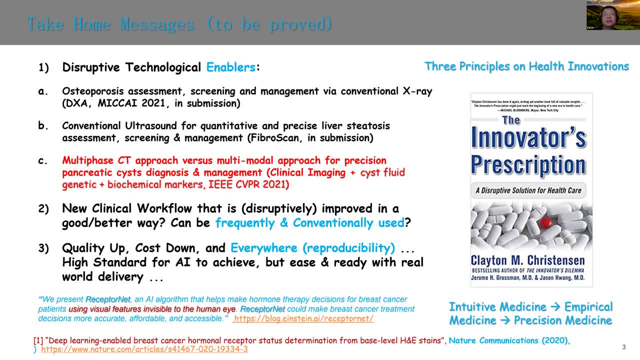 When we do this, And also I asked you to see the reference, you know, at the bottom of the slide that we call the raptor night. That's actually, you know, means you know what my message trying to convey is deep learning. 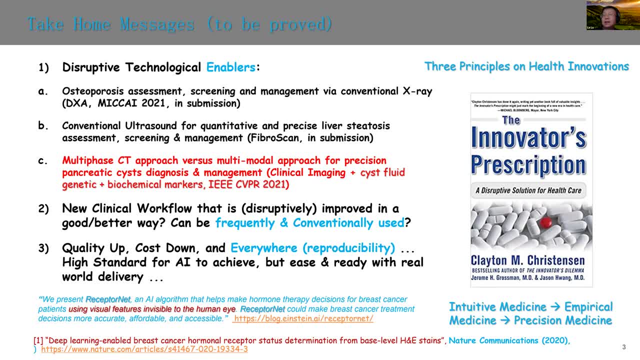 plus a conventional imaging modality, They can actually do more than the more expensive more subjective imaging modality or other means of diagnosis or treatment. You know treatment planning tools right, So. so so this work, the, the work from USC, is the actually stand as a. 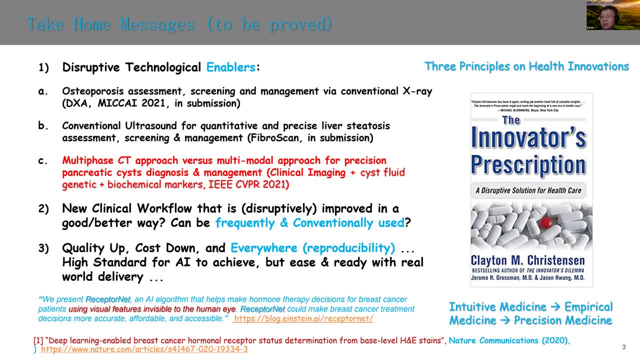 as the most popular stem for the pathology images and they are very easy to reproduce, right? So for the for certain of the breast cancer patients, they need to find the receptor or not. If they have a receptor or not, the treatment path would be different, right? 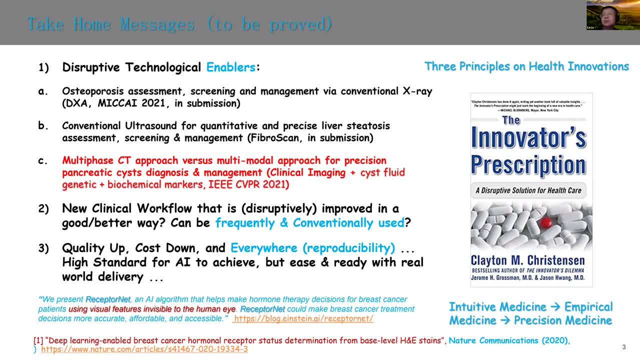 And the, the tab, the K, past those, theы, the, the, the. today, today there's actually 20, now they have to use the emo therapy, kind of like a stain, like a for a very expensive, not very reproducible thing to look at the receptor by human readers, right, but the machine or the deep. 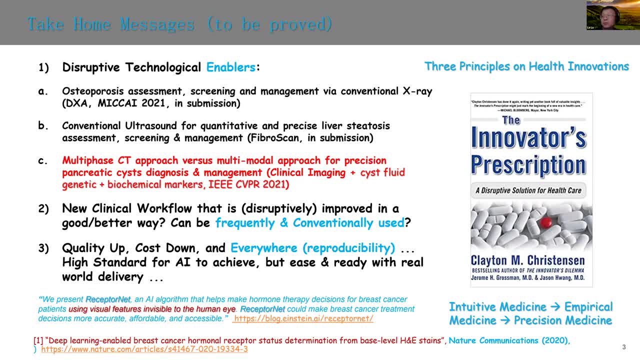 learning algorithm they can actually just look at the actually stands the the cheaper, the more convenient way they can achieve the same or even better than human readers in this assessment. they say they want to, you know, basically make a decision if the patient- underlying patient- has the receptor gene or not. right, so they actually make it a lot cheaper. right, they can just use the. 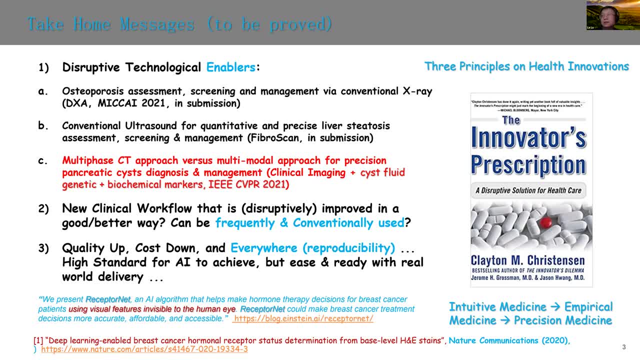 regular uh stand. they should achieve the same result. and for the- you know big hospitals, the, the cost will be lower, right, the cost will be lower and the quality, at least not not worse than before- probably is even better. and for other developing countries, you don't even have the, the method. you. 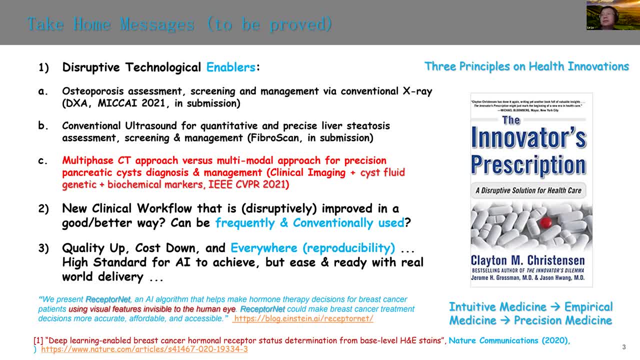 don't you have the know, feasibility doing this like, uh, emo, like pathology states right, so so, and you don't need to do it right, so this really means like quality up, like costa, and also is this has very good reproduced reproducibility, right, because we want to make it much. we want to make medicine cheaper. 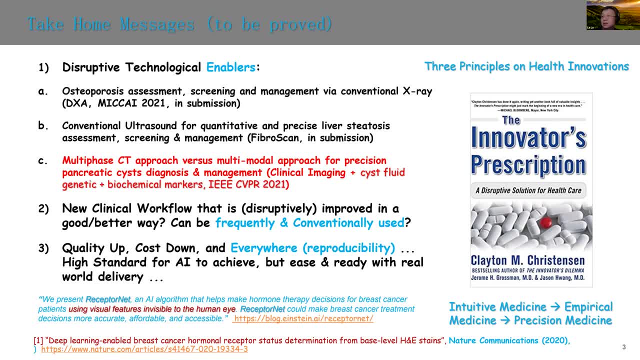 and everywhere and solve the inequality and solve the cost issue right. so the few examples here i, i hope, give you a heads up. you know what's going on. i think it's we, we. it's not hard work, but i think we have a we should have. 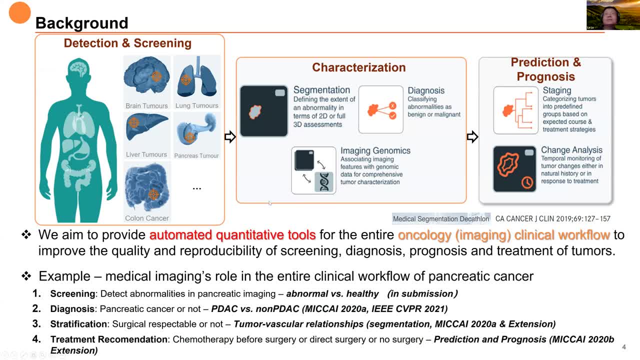 a bright future. yeah, this is. this is the main topic about. you know, i have been doing uh oncology for uh 15 years and i work with a lot of a lot of doctors, a lot of hospitals, and i i don't just work with raj, i work with oncologists and and surgeons in different departments as well. so i kind of 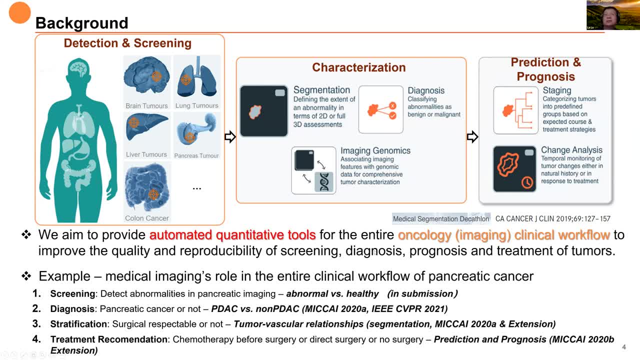 reasonably good, uh, overall understanding about the cancer care. um so, uh, you know, this is basically the the most popular top five, uh, tumors or cancers, right, uh, i i never work on brain tumors but i work on the rest of the four for a long time and so mostly we do is characterization, right, sanitation. 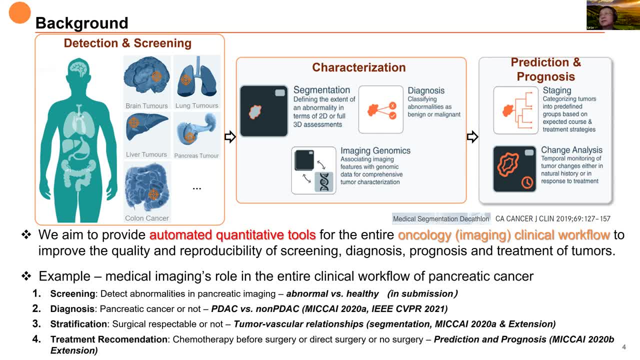 and the direct from sanitation can do diagnosis of guessing something was going on, or detection, you know, over uh imaging genomics means like from pathology images you can guess what's the genome characteristic of the of the patient. this is just like the example from usc or you know some. 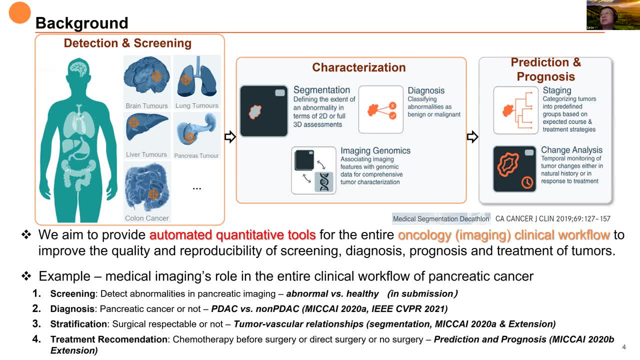 people they feel from uniform radiology or pet imaging. they can. they can, um, you know, have some strong correlation with the genomics feature of the patient, characterizing of the patient and more. I actually will discuss more about the prognosis. Prognosis was not really fully solved before. 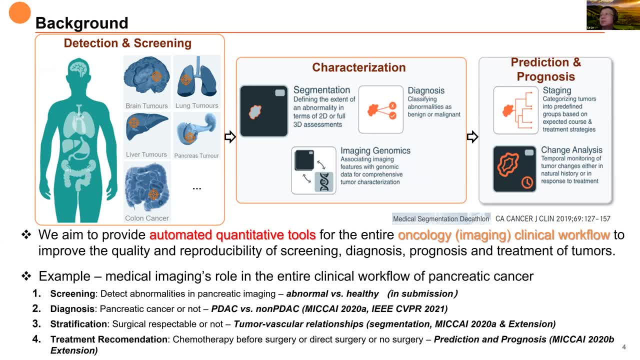 And I think we'll have some recent work that really push forward this field. And prognosis is basically trying to see, hey, this patient can survive for the next six months, or not right- Or a year. even in a year, will this patient be still surviving? 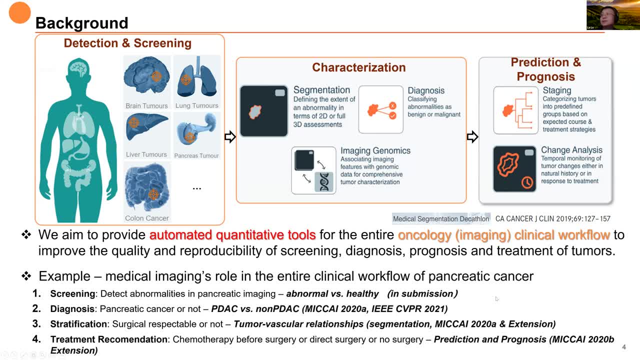 You know this kind of thing And you know this is based right now as the most accurate doctor you can guess, but they certainly they cannot be done better than machine. You know certain medical tasks. machines are much better than humans. 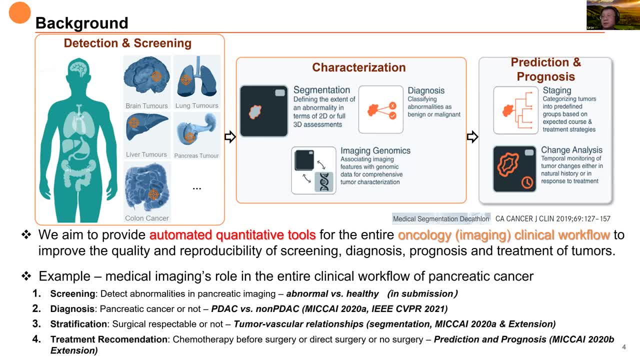 and they're complementary to humans. They're not going to replace humans. They make human doctors more powerful, in a sense right, We're not just solving the problem. that's easier for human to do, but really something on their wishlist but it's hard to do. 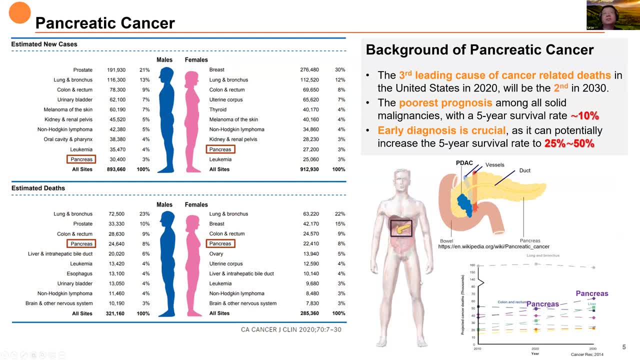 And we make it a lot easier to do. So you know I cannot talk about all the cancers. We work on a few right, But here, just to give you an example, is using pancreas. So pancreas in US, you know. 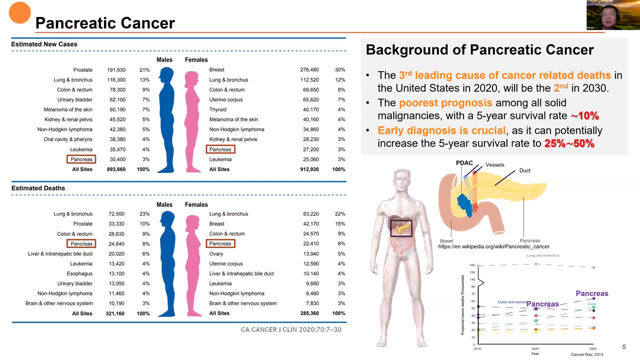 the death rate is also the third right. The number one is lung, the number two is colon, So the number three is pancreas. You know they have like 25, 25,000 people die in male and the 22 people die for cancer. 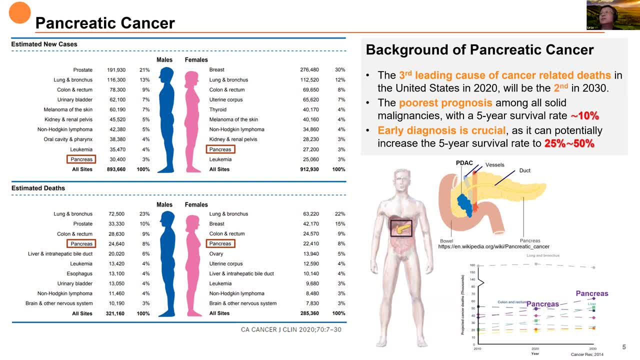 And this is because the pancreatic cancer has really poor prognosis, right. So the pancreatic cancer will be more and more important in the sense because- it's just you know- we actually achieve a lot on managing the breast cancer and the lung cancer, even the prostate cancer. 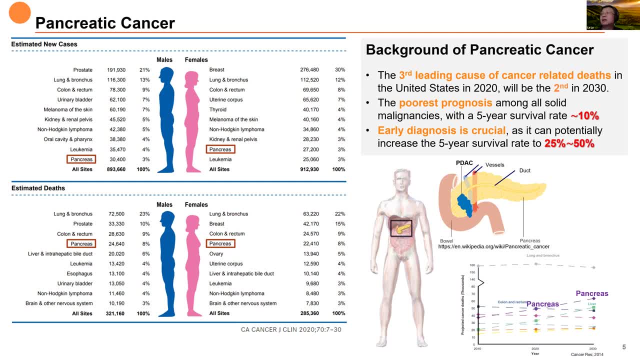 But really like. the pancreatic cancer is one really hard one. We haven't really made much progress in the last five to 10 years, And right now for the best hospital, the five years survival rate increased from 9% to about 10%. 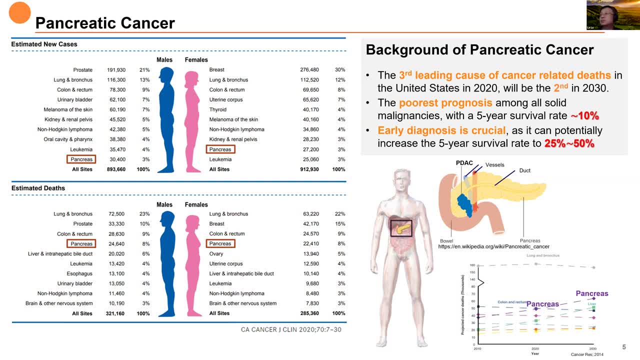 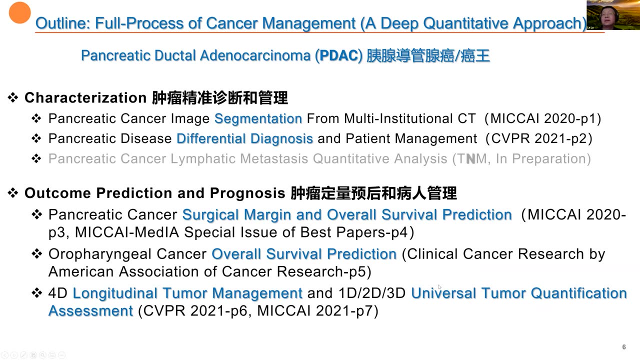 So, in essence, the early diagnosis is very crucial And if the pain can be early diagnosis, the survival rate will be drastically improved to 25% to 50%. The major thing is because the pancreatic cancer, there's basically no thing that we can do to treat the symptoms at T1 or T2.. 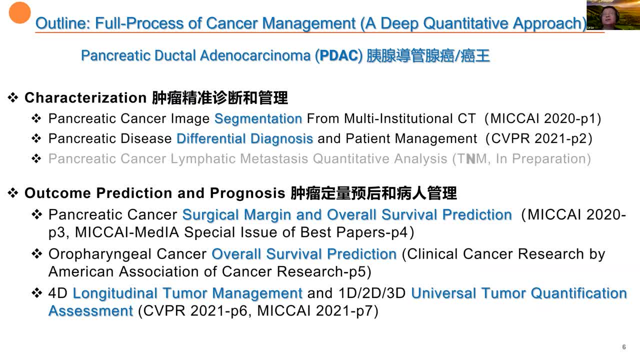 Really like there's no direct symptom. you know, it's not very easy for diagnosis or screening, right, I will not talk about screening. The screening work is under submission. So here is basically- this is basically today the manual. Like, I will basically focus now on the diagnosis, you know. 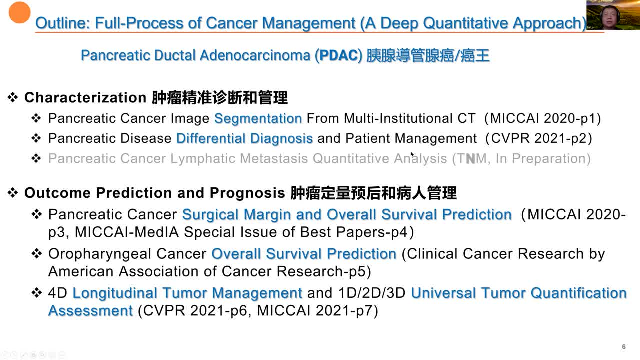 forgive me, I have some like Chinese characters in there because I can talk to the Chinese audience as well. Sometimes, you know, I can talk to the Chinese audience as well. Sometimes, you know, I can talk to the Chinese audience as well. 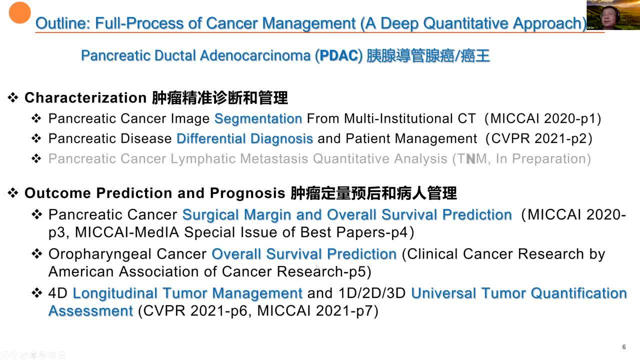 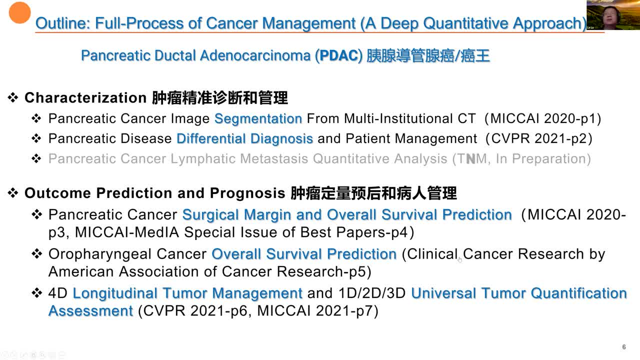 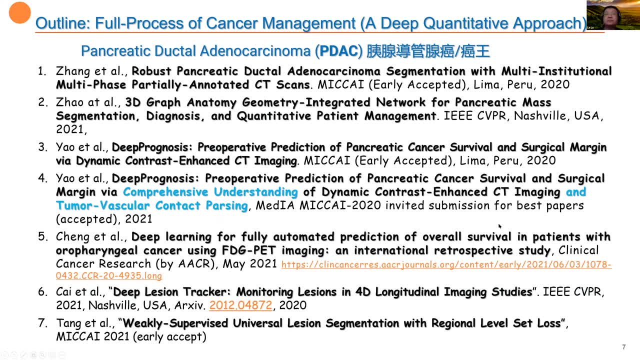 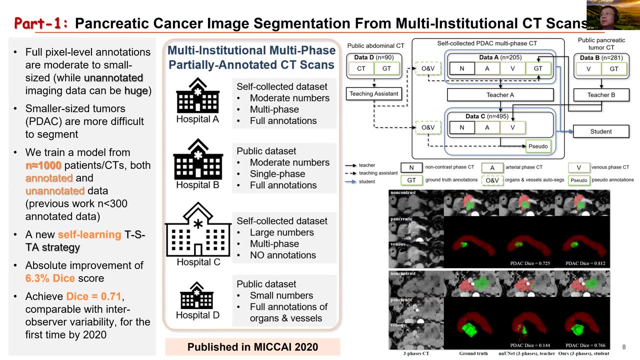 Yeah, so I basically talked about this: few papers, seven papers. This is seven paper I'm going to cover. yeah, So the first work is: I'll go quick because of time issue. I think I don't have much time. I basically showed a lot of pictures. 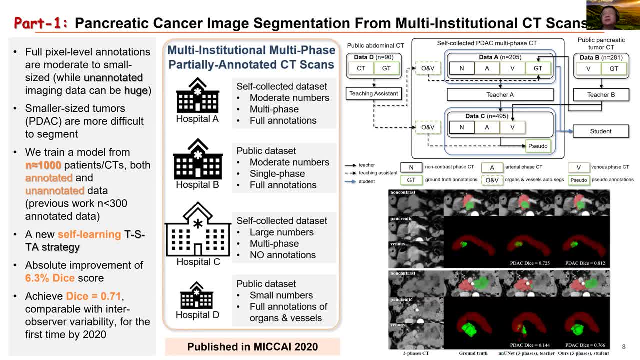 So this is actually the first work in that was done. like We submitted last March, it was published last year in MeKai. I think this is the first work multi-institutional, first work about solving the sanitation of the PDAC. 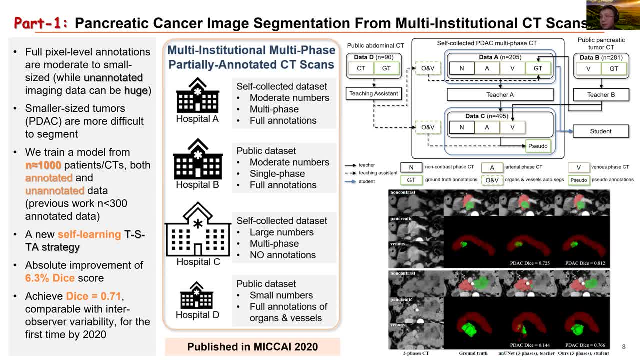 PDAC is the 85% to 90% of the pancreatic cancer, most of the deadly one. You know, we all know, we probably all know, like you know, Su Zhao would die because pancreatic cancer wasn't. he actually had one with a fairly much better prognosis. 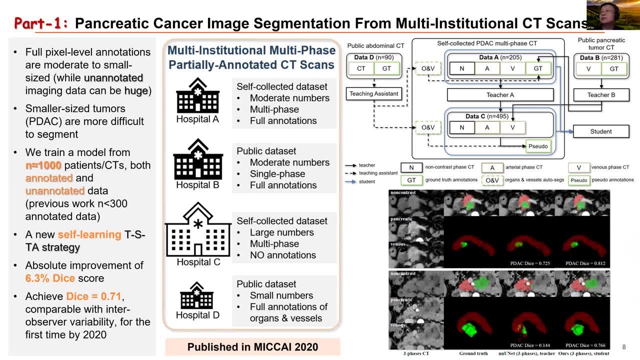 Like she paid actually for diagnosis on PDAC. So that's a much slower growing cancer compared to PDAC. PDAC is really like the most aggressive cancer at all. So you know, the thing is to detect or to just smaller tumors. the really key is sanitation. 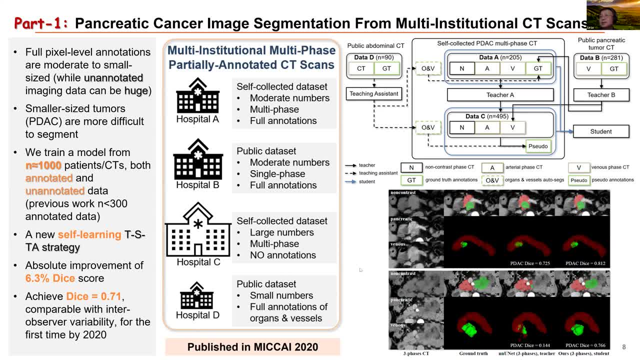 You have to segment them or you're detecting by sanitation. basically, You have to segment, you have to figure out where it is and you can segment a few voxels or maybe more voxels, So you can, you know, you can- find the. 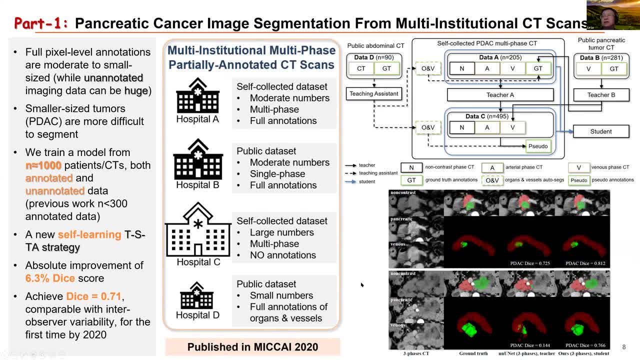 you can find the tumor and you can. you know, you know, give the human reader say, hey, this is potentially a pancreatic tumor And you need to look at it or you need to follow up. You know, even you cannot confirm fully from. 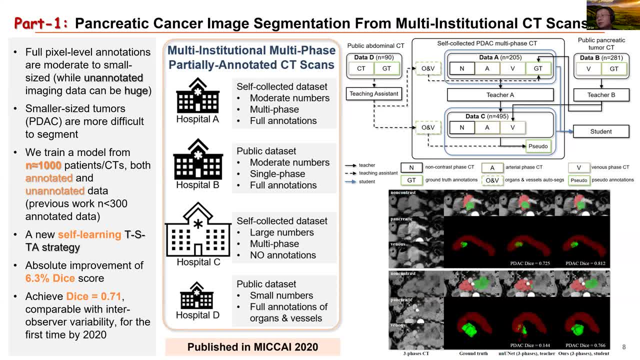 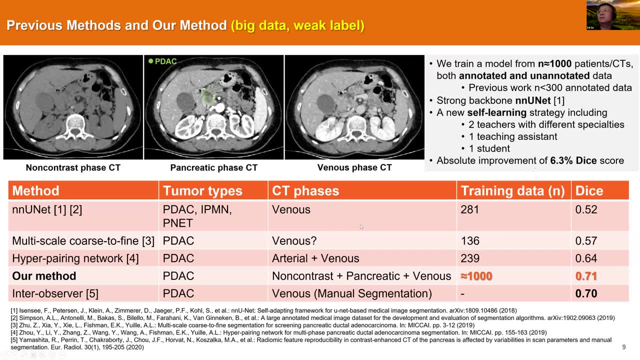 let's say, from like a non-contrast CT, you need to do a multi-phase CT or you need to do some like an MRI or something like that to get a confirmation. So this is. you know, we basically we got data from four institutes. 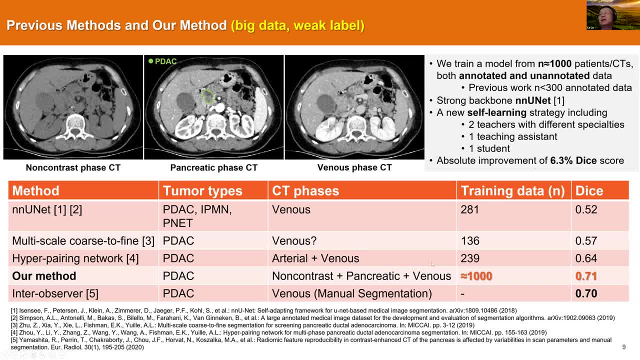 And this is a comparison to previous work. You know, really, we got big data. We got one solid patient at that time. Right now, we have six solid patients. Yeah, we are making progress And by then it's a year and a half. 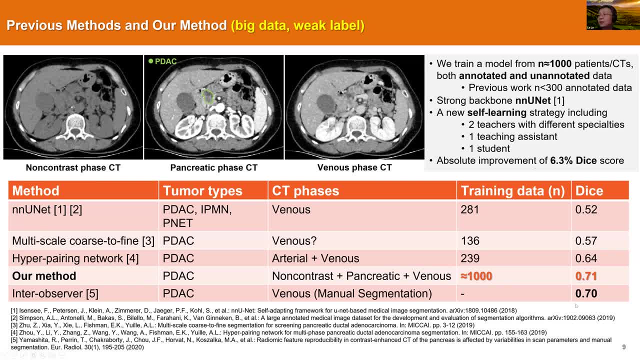 year and three months ago our death number was 0.71, right now we're at 0.76.. That's probably an upper bound that you cannot, because even for human readers the inter-observer variation is about 0.770, yeah. 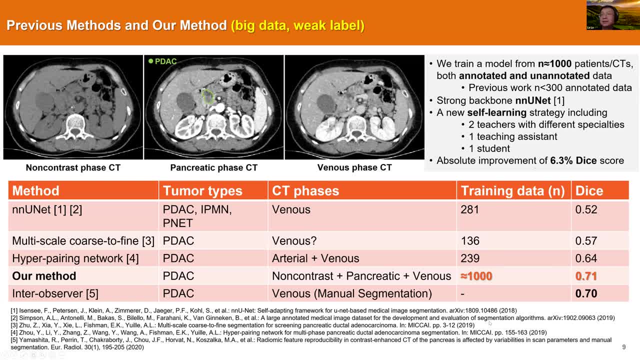 So we- I don't know it's a little bit better than the human readers. You know we work with very, very good physicians, just per se. yeah, So this is basically the technology flow chart. I don't have time to give detail. 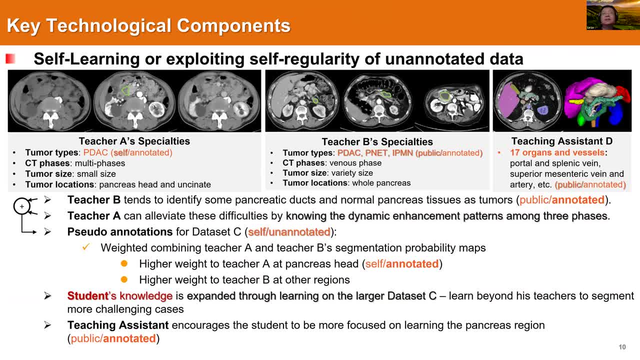 You can read the paper I have reference. yeah, So basically it's, you know, we have two student share model where you will have a teaching assistant. Basically, we're trying to gather, you know, the data, all the information from elsewhere, everywhere. 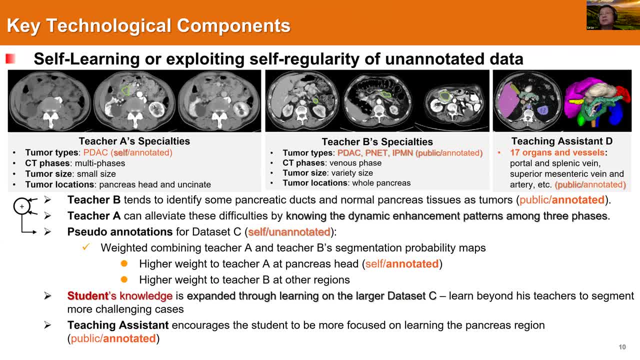 and even they are annotated in a different level. So basically we use the technology innovation to bridge the gap, So we can basically learn from whatever. As long as we have data, we can learn, we can improve. So this is very much from the information theory. 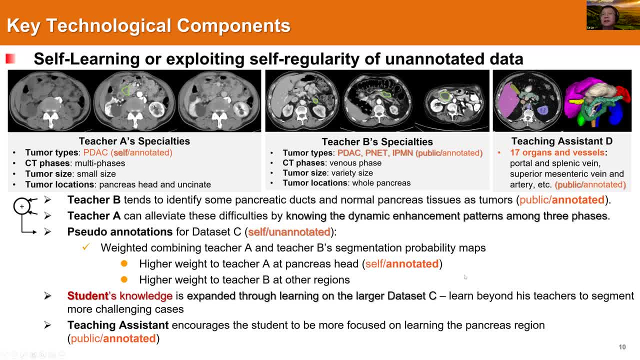 You know you have multi-channel. some channels are noisier than others, but if you are good enough on the field, you can always get better, not monotonically, but improve the result right, Not to decrease the result. 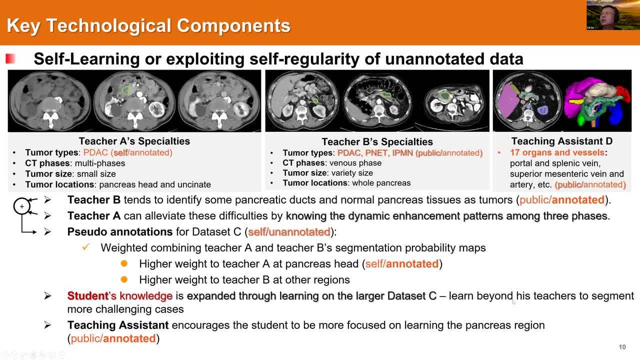 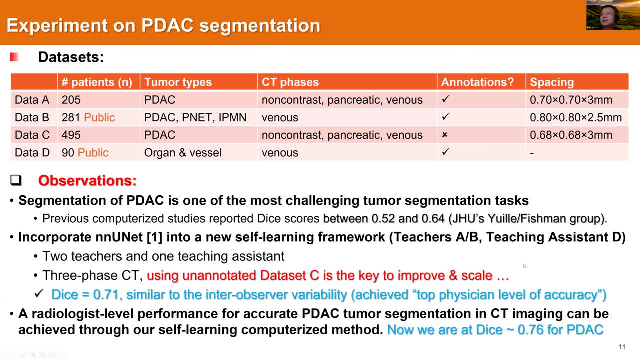 You have to be smart on the algorithm design and really be innovative on the software part. But more data is better, yeah, in a sense. So this is basically you know the dataset. I think our strengths is we got the dataset C. 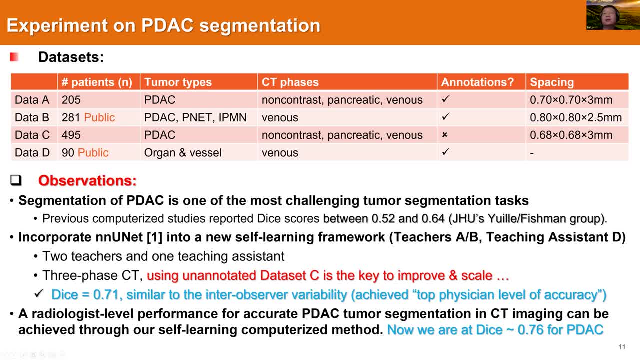 That's for a hospital like a, really like we have at the time. we have 500 patients. You know each patient use three scans, So we got, you know, three scans, About 3,000 scans, 3,000 CT scans. 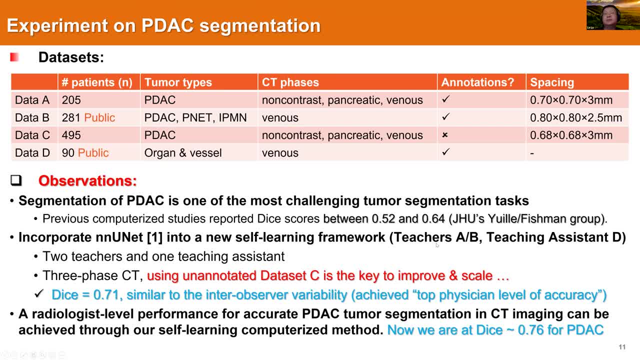 And there's no annotation. but we know the, we know the, we know the report. So we basically know the, what patient they have they have, how they have this disease or not. We have the final report, Not just the renal report. we have the clinical report. 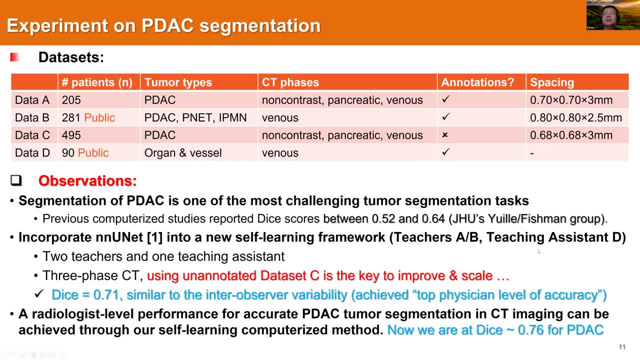 So we know what's going on with this patient, right? So this is basically you know how we get at that. This is the first step and you know I'm sorry for like I only can be able to cover. 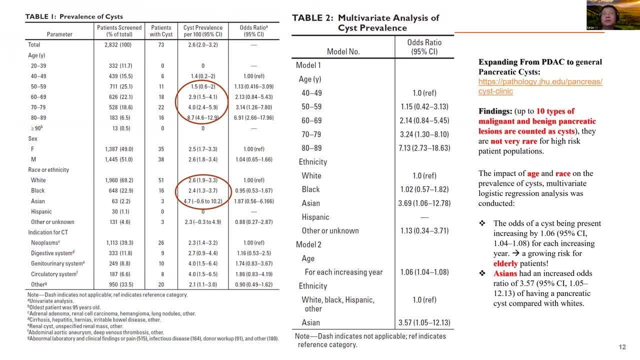 be able to cover it very briefly, but you can read the paper. The paper has all the details in there. So the next step is a work that we're very excited about. This is going to be presented later this month. We'll be in CUCAR 2021.. 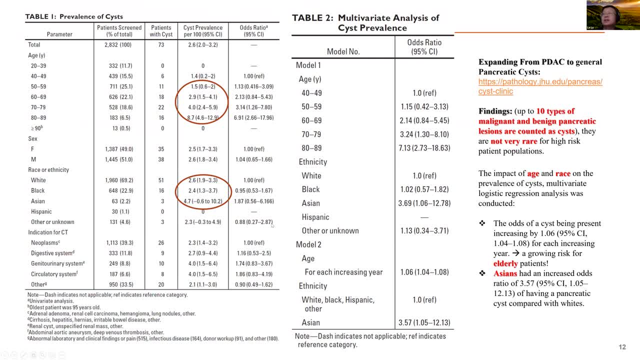 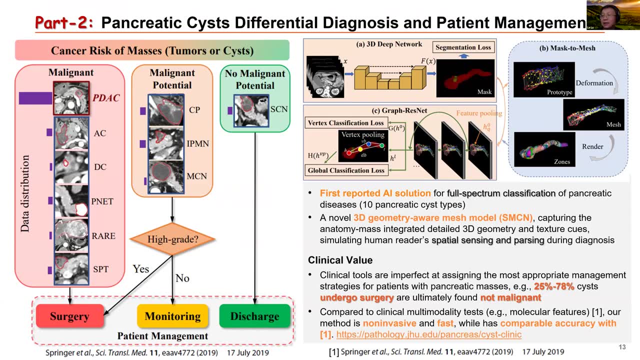 So we're solving. a problem is for pancreatic cyst. Pancas cyst here means all the tumors. Pancreatic tumors has 10 types, 10 subtypes, right, 10 subtypes. The P-type is the dominant one. Most of them are pancreatic. 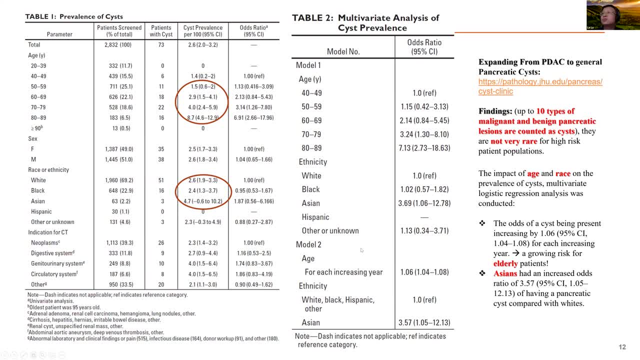 There's also the deadly one, but there's some other non-types of it, right. So the first work in any hospital: when people find a cyst inside the pancreas, first thing they will ask is: is this a P-type or not? 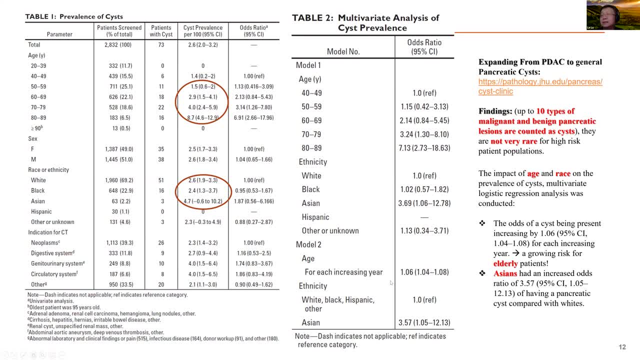 So this is basically the first step, all the first detectives trying to get right for any physician And all you can see is that the pancreatic cyst is actually. the prevalence is actually higher than what the audience think, especially is correlated with age. 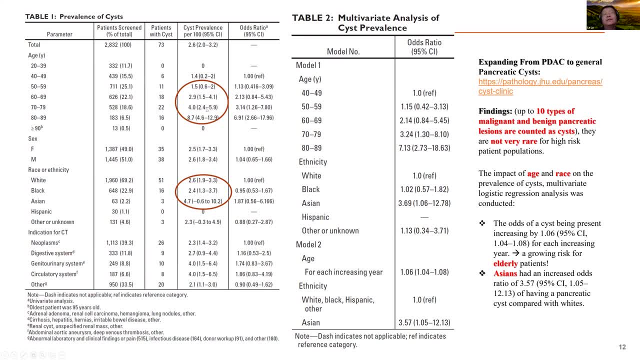 So if you are so, I'm going to be 50 years old in the next few years. So if you are 50 years old, it's already like a 1.5%, 1.5%, right? So all the people from six and above. 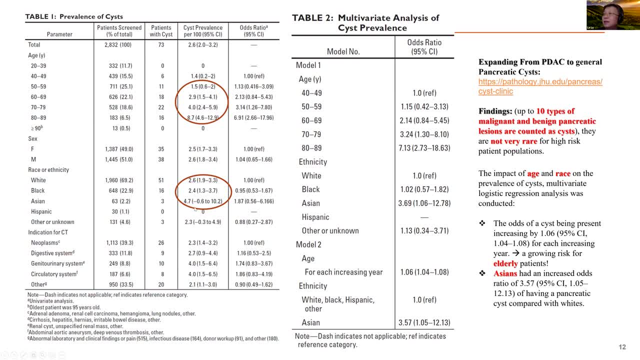 for Asian is 3.7,, 4.7%, I mean nearly five people out of 100, if your age is about 60 and you're Asian, and the risk is not small, 5%, yeah. So the best particle is actually from John Hawkins. 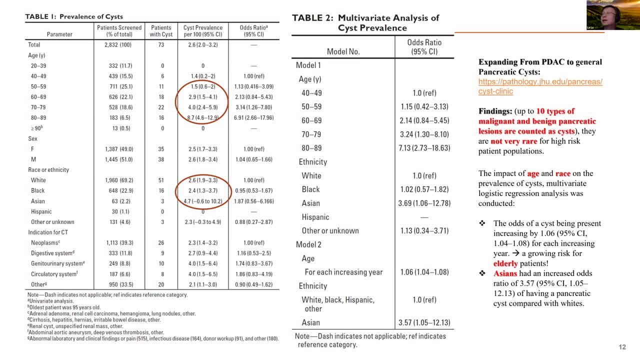 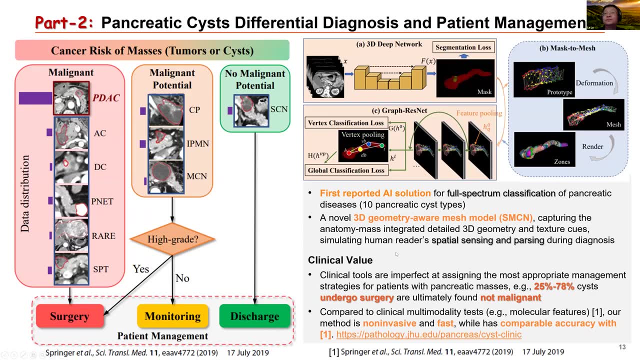 You know, just you know. I read from John Hawkins, but this is my honest assessment, not because I read from John Hawkins that they are the best. You might understand. they are the best, Yeah, So our work is very much inspired by their work. 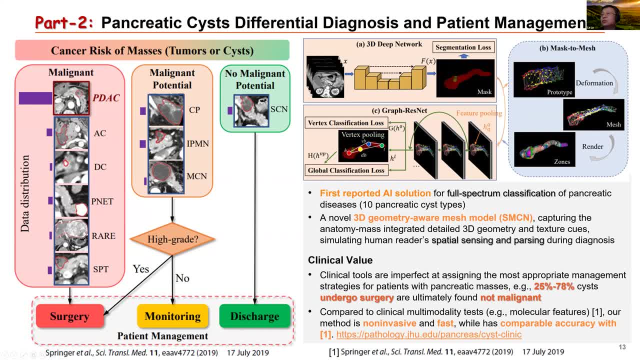 by Hawkins' work the property in San Francisco University of Medicine in 2019.. So it's a very dedicated procedure. You know- maybe I have to hear- It's a very delicate procedure, including a lot of things, a lot of magic things. 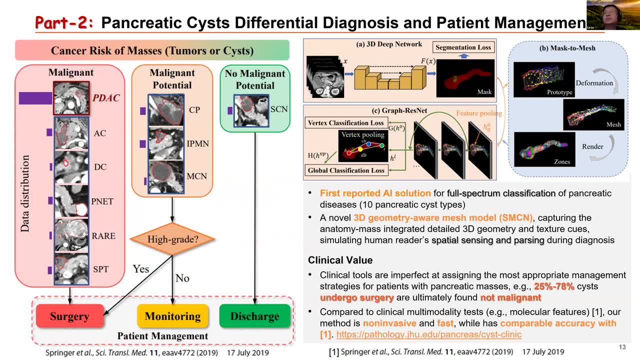 but they are not really fully translatable or reproducible. Our method is fully translatable because we only need the imaging. So basically we have a sophisticated imaging particle and on the top right is our algorithm. So basically we actually simulate what the human reader will do. 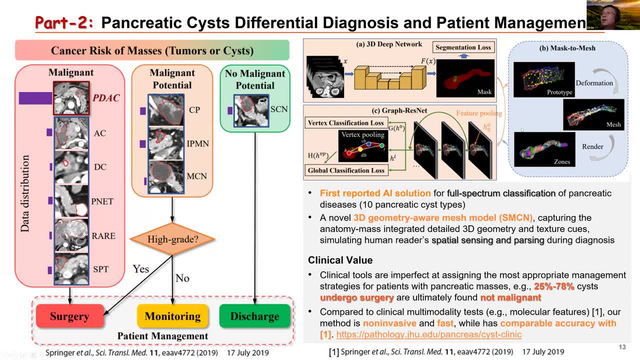 We basically we segment the pancreas, we segment the tumor and we parse the different zones of the pancreas. So we know relatively where is this tumor located, right. We also even know some vessels passing by, some anatomical structures passing by. 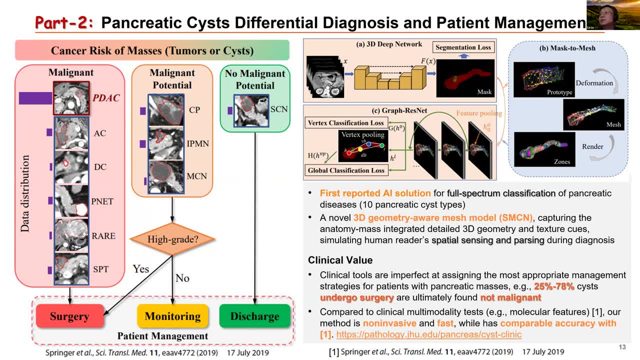 So when people making decision about what this tumor it is, it's not just how it looks like, also the geometry, also the geometry inside the human body and the geometry against the pancreas and its surrounding anatomical structures. So basically, we can do the same as just as human readers. 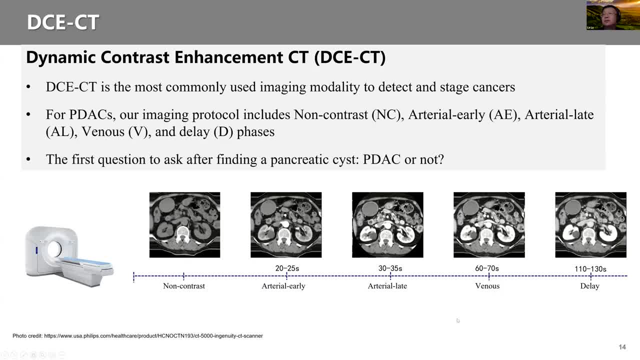 just as human reader will do. yeah, So we have a sophisticated for this problem. we have a sophisticated task. So, basically, giving a product we have five phases. So five phases is rare, relatively rare, I have to tell you. 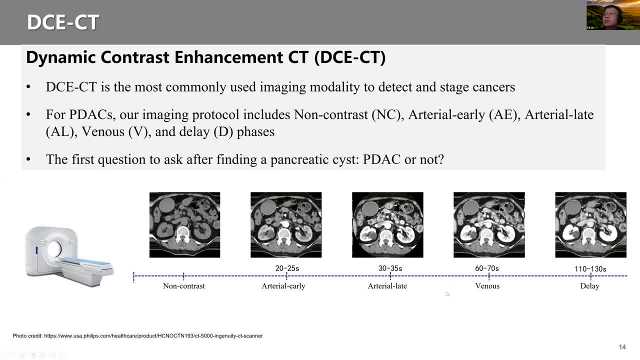 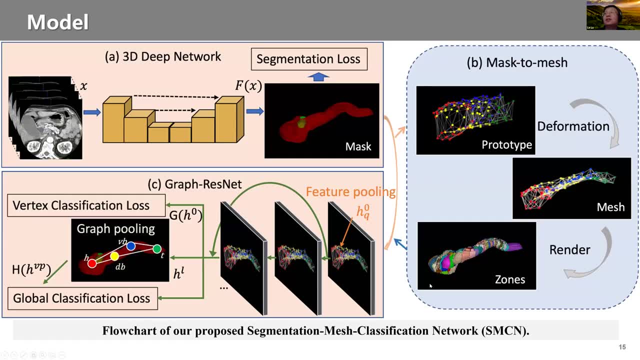 But it can be done. I mean, when you have a modern CT machine you can do this. It's just the patient will have more dose, redeeming dose. but the current protocol is actually human, So the patient need to do a biopsy. 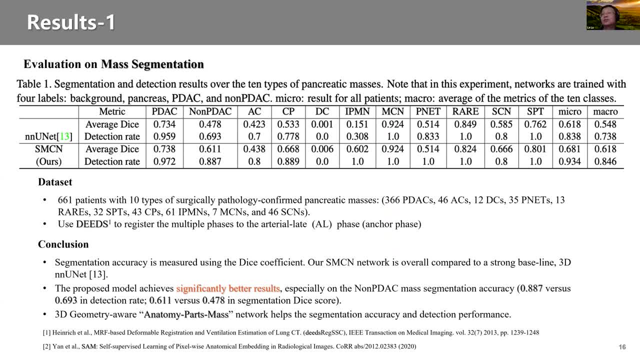 and doing like a gene sequencing and the protein screening and the wet labs and also some like a manual reading by the top radiologists on the planet, right. So I think that it's still relatively. our approach is less helpful for the patient. yeah, 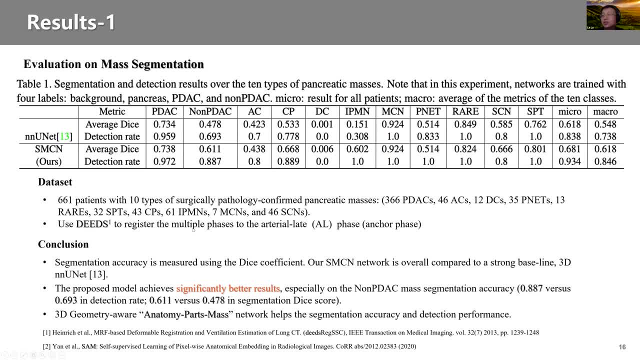 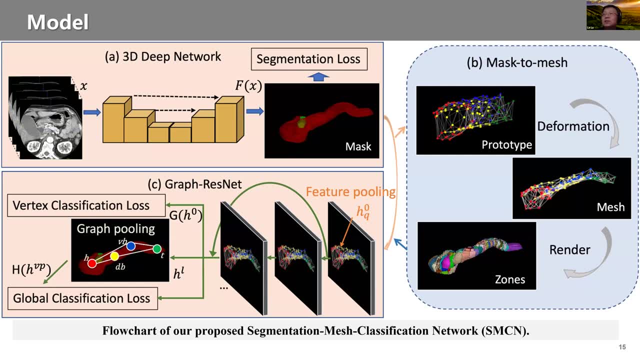 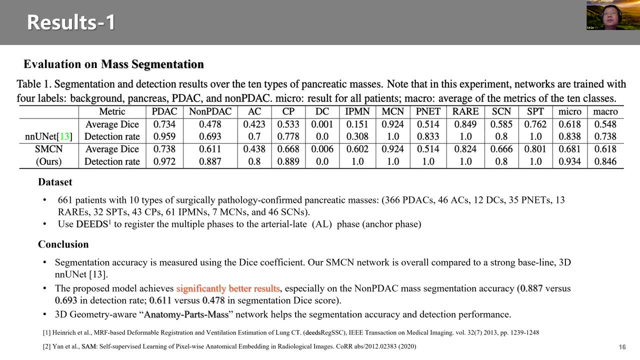 So I don't have just that. there's a geometry. This is our main contribution from the technology perspective. It's called SMCN network. This is a new method will be will be presented in two weeks. So, basically, what do we do is we can significantly increase. 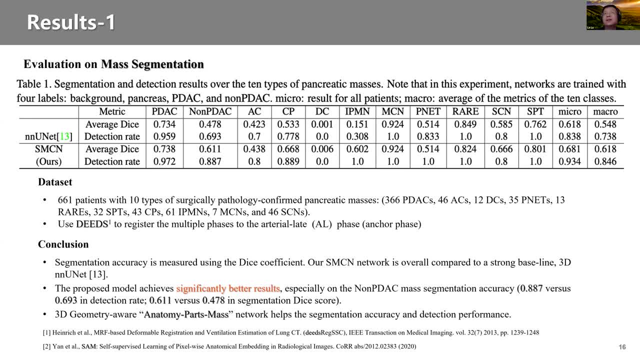 the detection rate of the non-PDAC We talk about. PDAC is difficult, non-PDAC is even harder. So we basically increase the detection rate from, you know, 0.69 to 0.887, yeah, So it's much better. 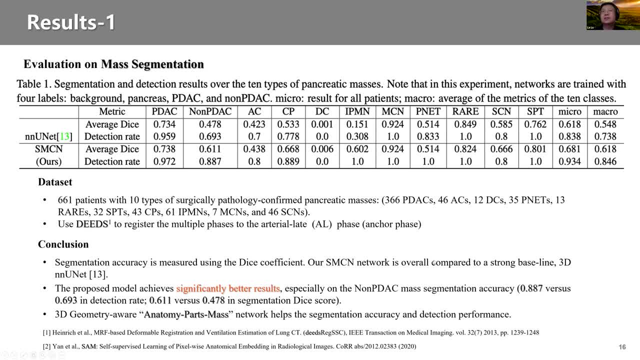 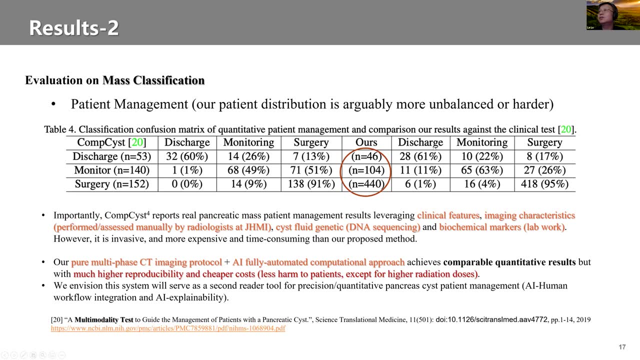 So we can detect all this like non-PDAC tumors and we can basically do a differential diagnosis about if this is a PDAC or non-PDAC or the three categories. So three categories. what matters most is this tumor is. 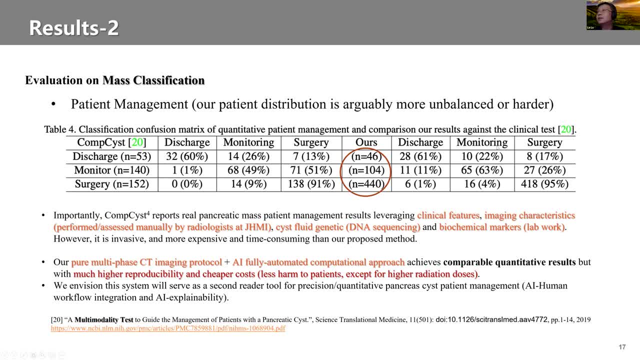 you can discharge the patient or you have to monitoring them, giving them a say: hey, you have to be back in three months, six months, for re-exam, So to see if the tumor grow or not, because they don't know. 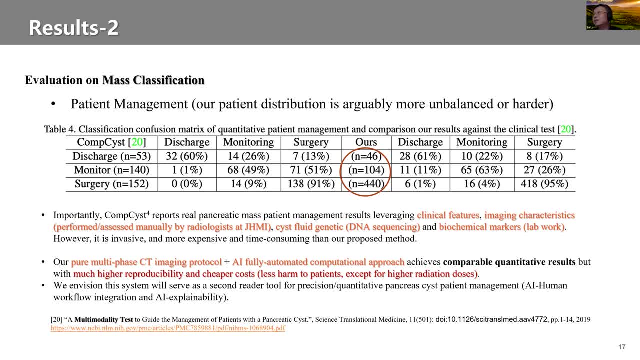 for this type of tumor they don't know if they will grow into benign, into malignant or not At the time. for the time being it's benign, but we don't know if that will grow into malignant or not. So for the discharge it was just. 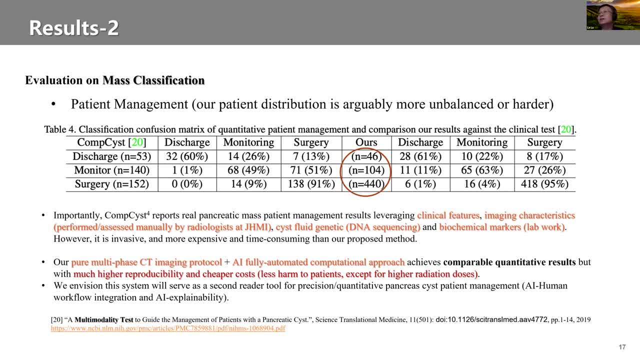 it has the same probability as no tumor, the chance that they will go into malignant. For the other six, you know really thing we do. you have to evaluate if a patient can undergo a surgery because that's other six tumor, including PDAC. 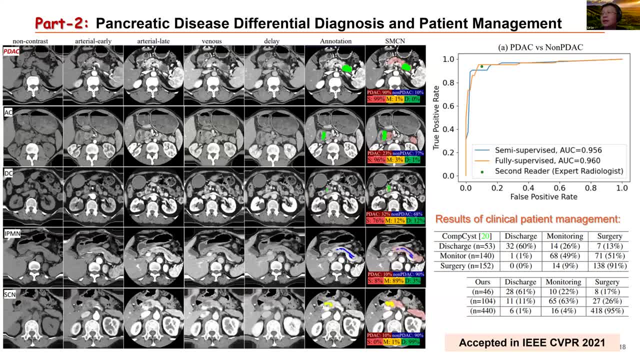 you know you should consider to resect them when you can. So this is basically our system on the flight, on the ride. is this actually? the AI will show up, will segment the tumor, It will give you like a decisions: PDAC or not, PDAC. 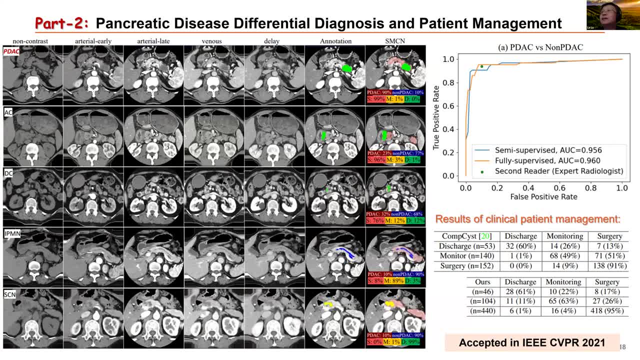 and 90%, not PDAC 10%. so now PDAC and it recommend surgery, 99% recommend it. It should go to surgery. You know machine machine results. it doesn't say absolutely is based on a probabilistic cost effect, right? 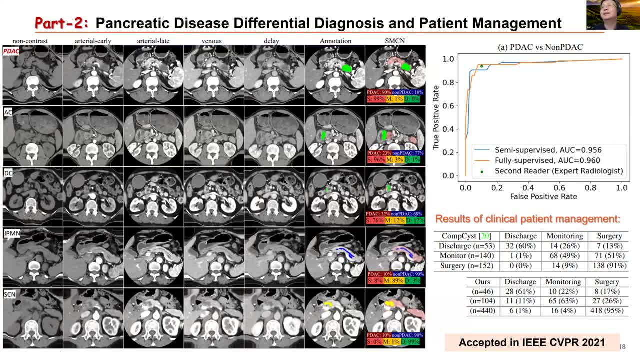 So it gave a probability. It's not like human would say, is this for sure or something, But you know, I think it is typical It's. you know, we handle everything. that is this right. So this is also. we have a small human. 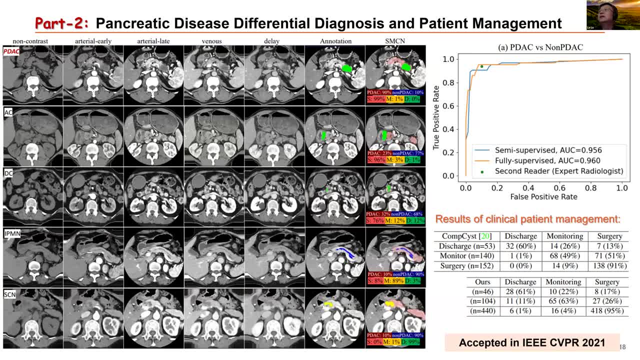 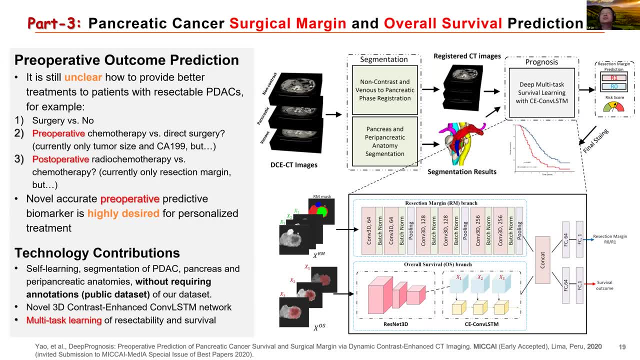 small-scale human radar study. It's comparable to the best of the expert. we're not just focusing on the speciality cell and practicalities with more than 10 years architects. So the next step of work- I will go even quicker- is just say hey when you find that this tumor. 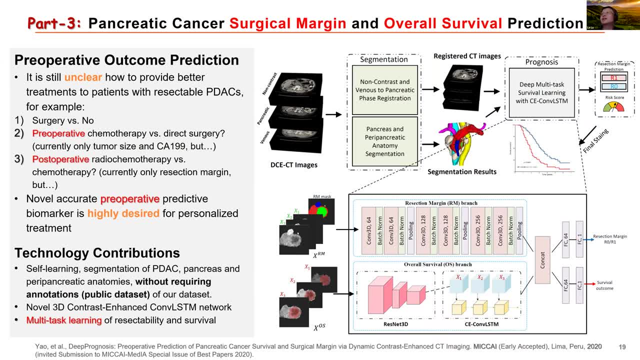 is recommended for surgery. are they resected or not? right? This is a hard decision actually. I mean, really you want to resect them, but you don't know if they're resected or not. This is the including the treatment recommendation, right. 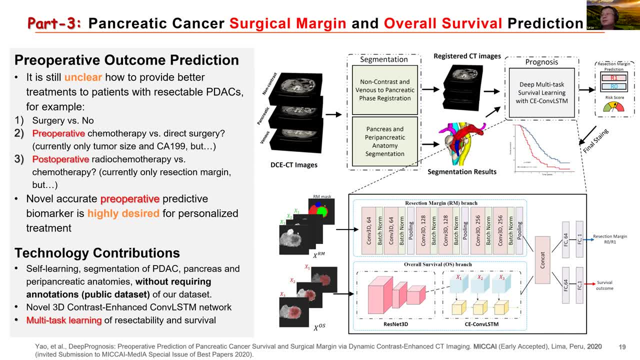 So you have to decide a lot of things pre-operatively in order to get the optimal outcome of the overall survival. So this is the work published last year: Mikai. it was one of the best paper candidate and our general version has been accepted. 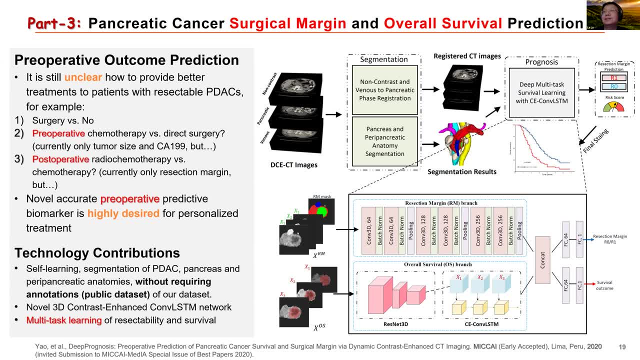 We don't know if we will get the best result now. that will be decided in September, October. So that's where our paper is one of the candidate for Mikai 2020: Medical Human Analysis Best Paper Candidate. so in that sense, right. 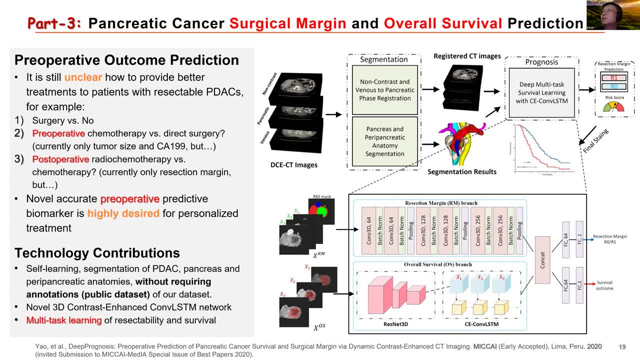 So basically it's a multitask, it's a multitask work. So we basically predict not just overall survival but also the, the clinical margin. The margin has two margins. it has two value: R1 and R0.. R1 and R0 means that, like within the margin, 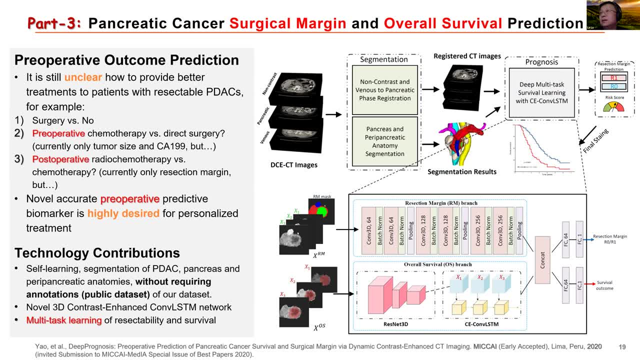 there's no like cancer cells from the pathological images. right And R1 means like you cannot resect the tumor very well. The tumor already has metastasized. at least within the margin you can see that there are already some cancer cells. 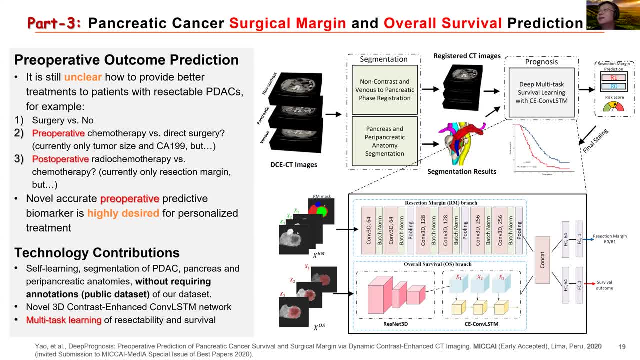 So at least some may not be like a remote metastasized, so it has local metastasized In a sense. So of course, with local metastasized the patient's level will be worse than without right. So so this is a. 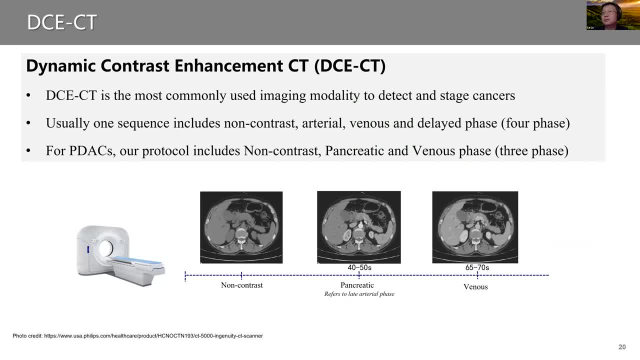 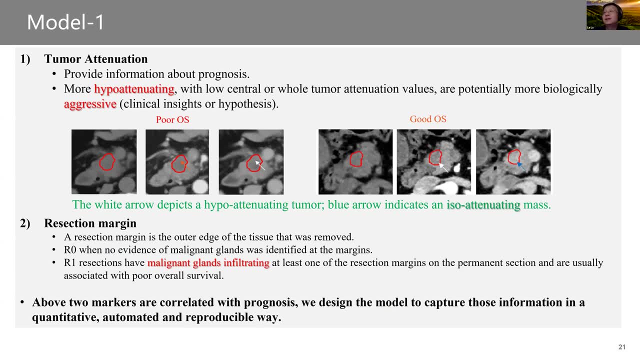 this is an immune protocol we use. It's a three-phase. This is a very typical. this is a very typical three-phase- And you know this before- is human gas. You know this is how human gas it's very, it's really like it's art. 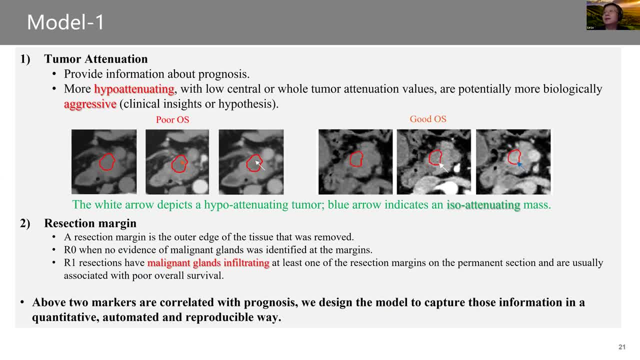 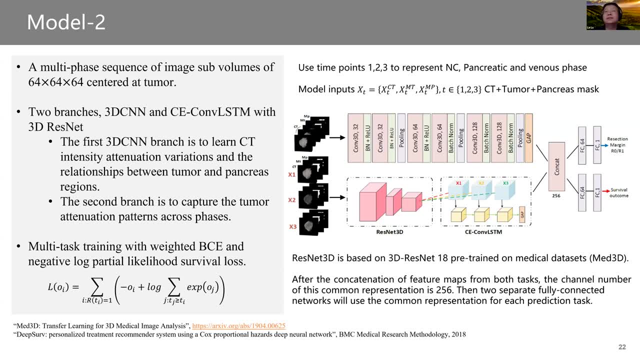 You have to find the intuitive medicine, the top expert. they can guess better than the other physicians, right? Those are physicians not always feasible to find, you see. So this is basically the network we do. We use this network to kind of do this task. 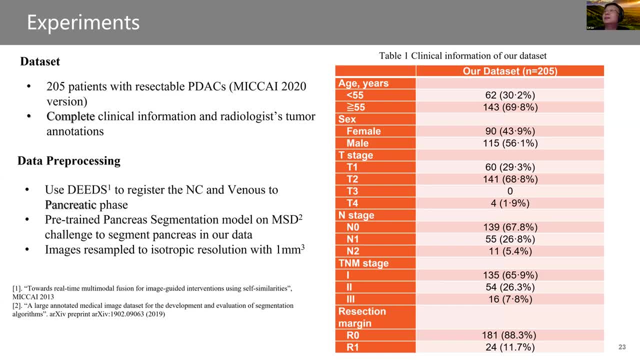 on behalf of human. In a sense, there's a sound like about by that time. we only have 200 patients. right now we have much more than that, And this is a conference version of the statistics. So basically, basically you know. 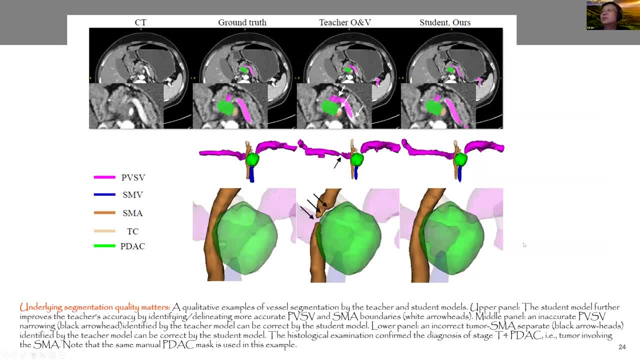 also the algorithm looking to the tumors. what's the vessels? what's the? what's the anatomic structure of the pancreas? You know the receptor or not. it's very much relevant with the vessel, Because you know tumors need a vessel to feed in. 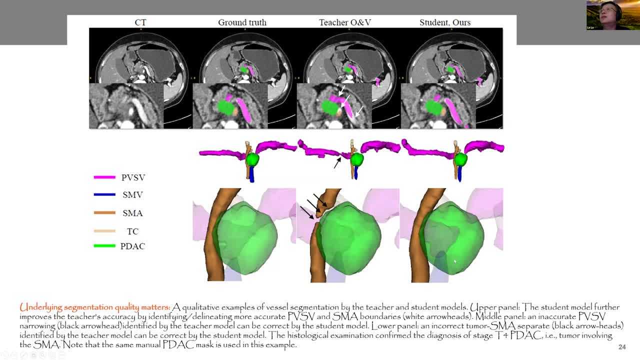 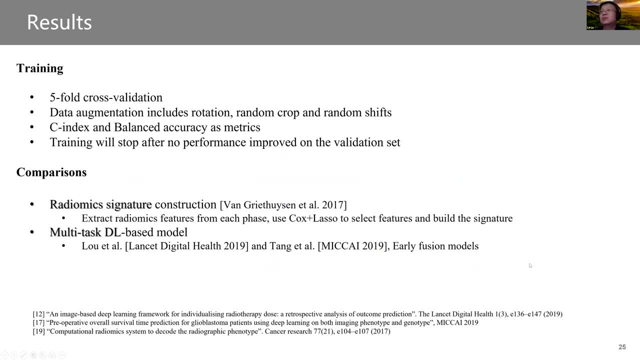 the nutrition they need. And also you have a relationship between with the vessel depending on the cancer receptor or not. basically Because if they're fully wrapped around the vessel, I mean it can cause massive bleeding. You actually cannot cut the cancer anymore. yeah. 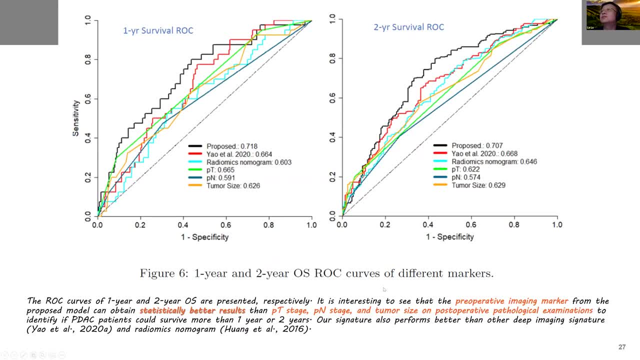 So this is, you know, I would just you know this, this business, as promised, the prognosis model And this RSC score, we can predict if the patients are still living and still alive, still, you know, in the first year or second year. 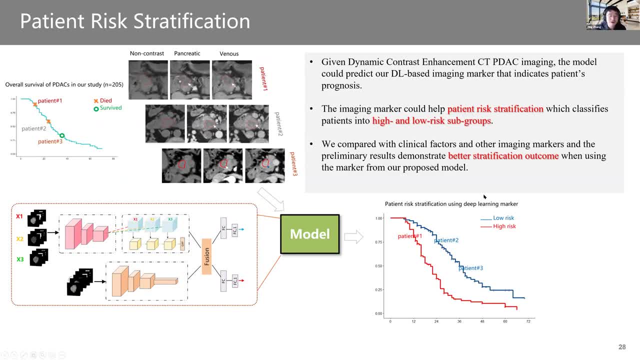 you know this is Sorry about the one more minute. Okay, Okay, Yeah. So so this is basically: yeah, this is basically. we can the patients who higher risk or lower risk patient, And the, even the given. 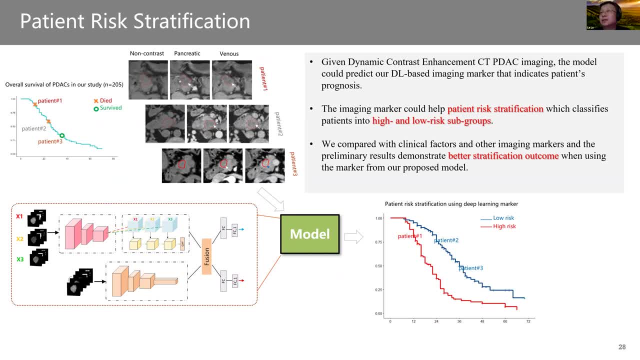 the given default. a protocol is TNM, the typical TNM protocol about, you know, making staging about patient. but our algorithm will really make it more personalized. So even within the, even the TNM staging are the same. the patient actually have different risk. The deep learning or the 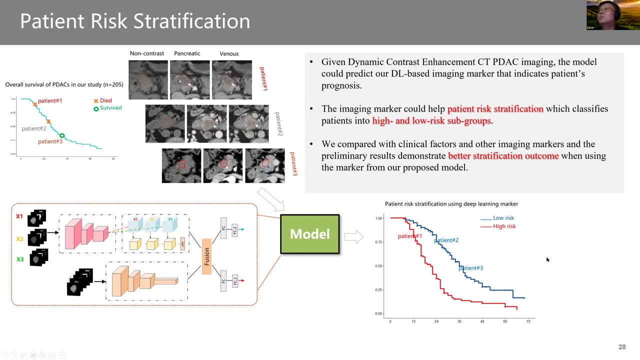 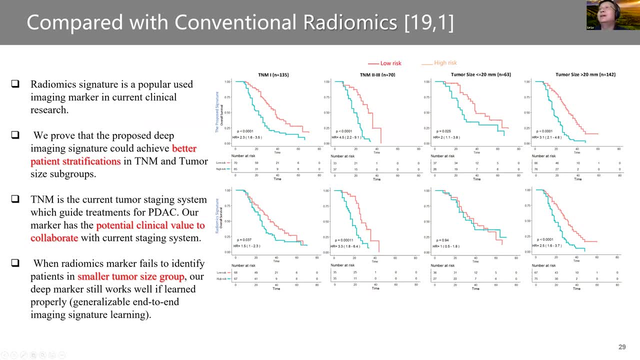 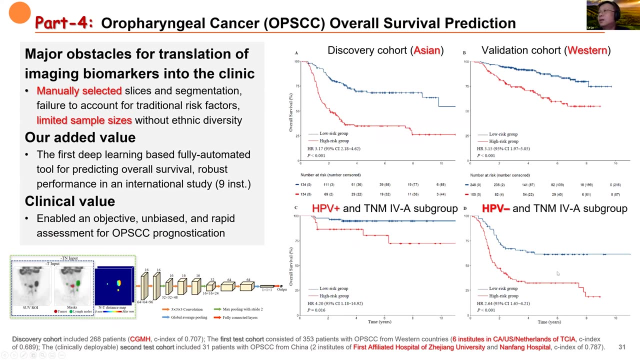 quantitative computing really make a patient can be more personalized, And this cannot be done by him, And this can only be done by computing. I'm not saying just deep learning, but really it should be done by computing per se. Yeah, So this is another example. We not just for. 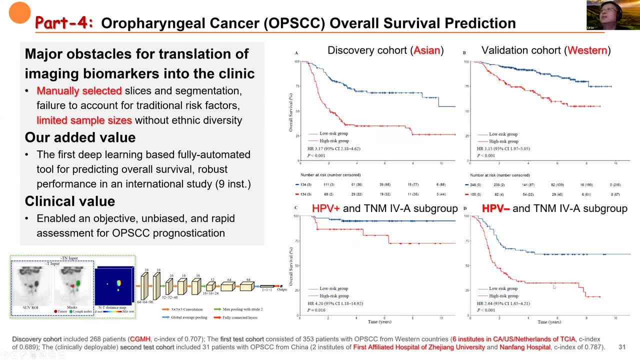 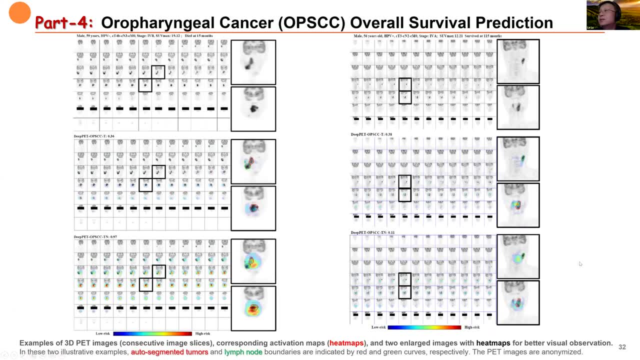 pancreatic cancer. we can also using just 3D PET imaging and we can use for OPSCC. So this work has been copied in the CTR this month And so this is basically showing the methodology of translatable. It can deal with two cancers, Or maybe. 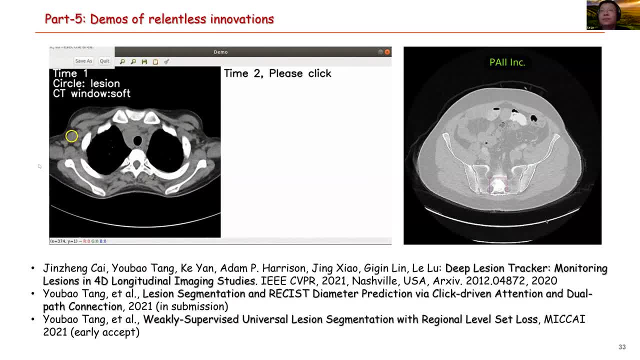 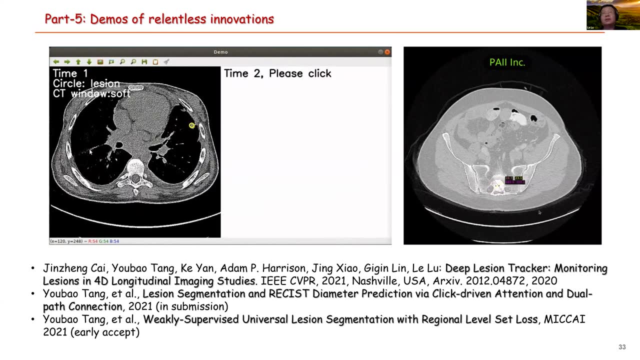 more than that and deal with a complete different imaging modality. So this is my last size. I just play the video You can have a look about the tumor managing. The tumor managing is the sizing and the if they are grossing or not. you know you have to find the multi-time point about a 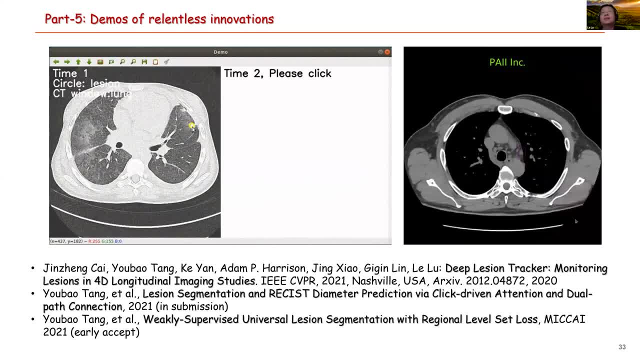 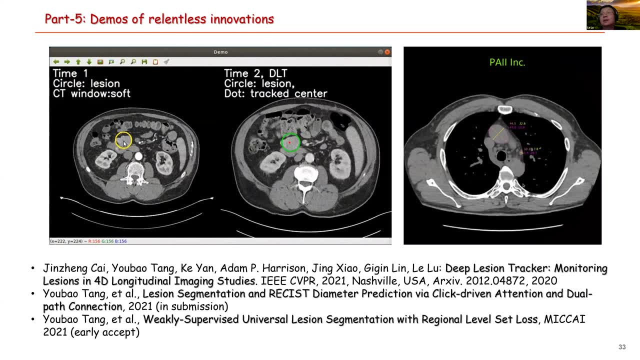 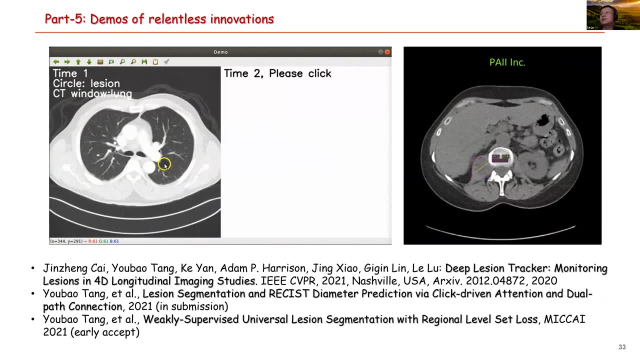 certain tumor and then you can compare visually or you can compare them quantitatively. So so the thing I talked about here is already like in the process of commercialization. So we, we work with past companies, We, we, we kind of mix this into our smart packs or intelligent packs. 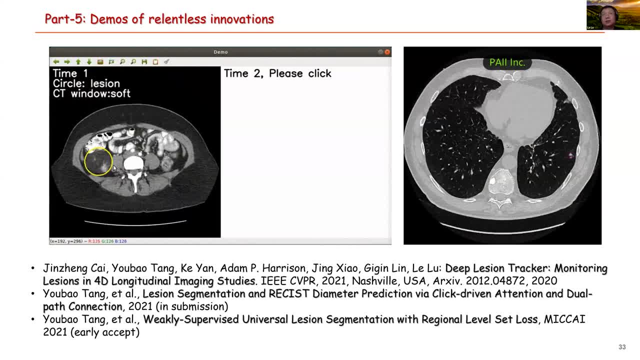 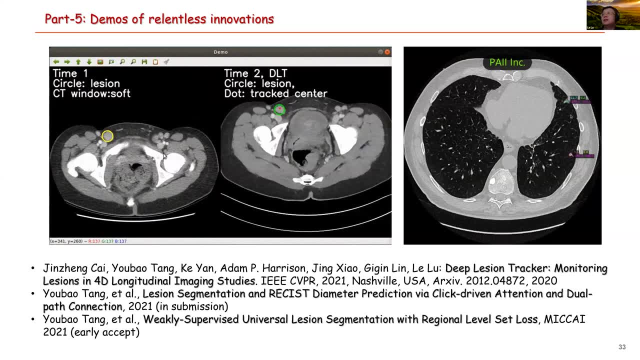 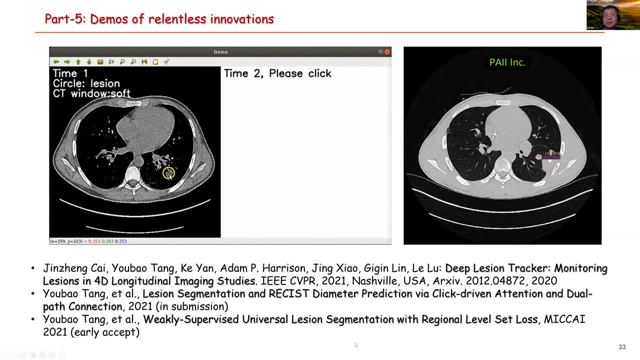 for the offering in essence, or even some like a, you know, research platform. So more, more, more, more physicians they can play around with that They can use for a patient within the hospitals. So that's actually pretty much that's it. Yeah, That's, that's my last slide. 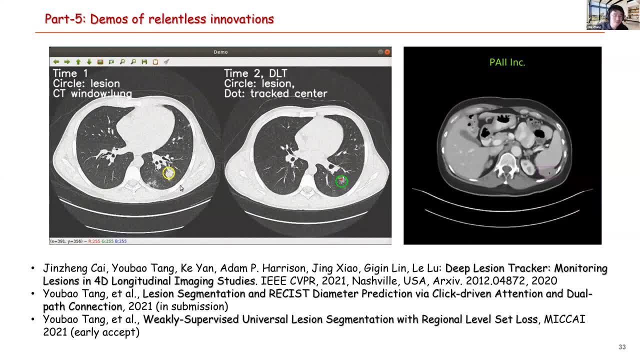 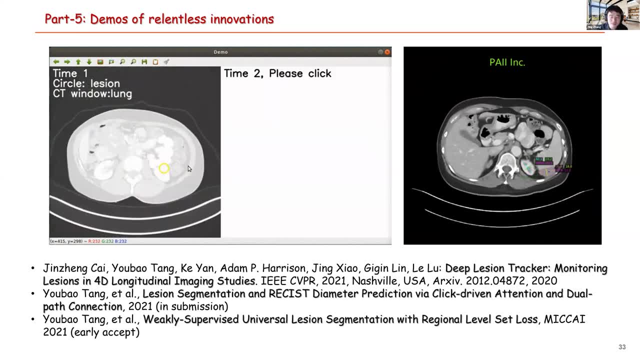 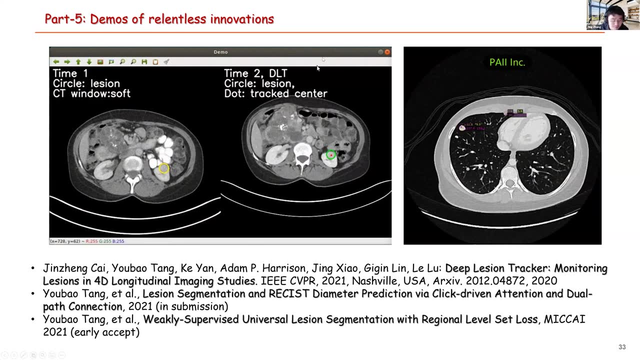 Yeah, Thank you, Thank you. Thank you so much for looking really for the excellent talk. So, for the people, if you have any questions, just a key in the chat box and we will have a panel discussion section after one o'clock. the sort of speaker will be a. 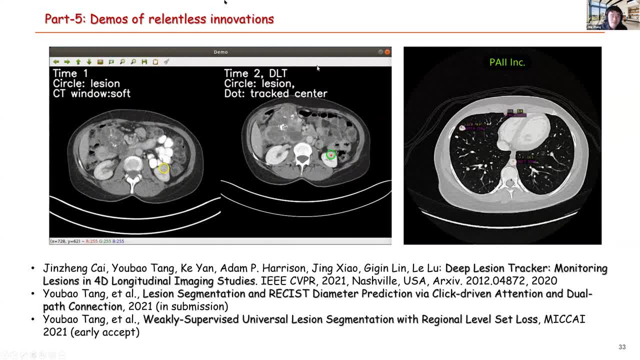 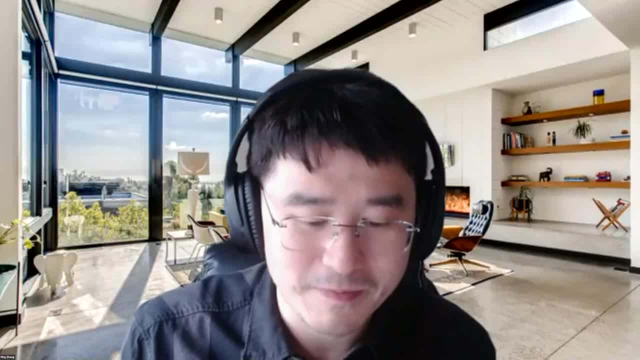 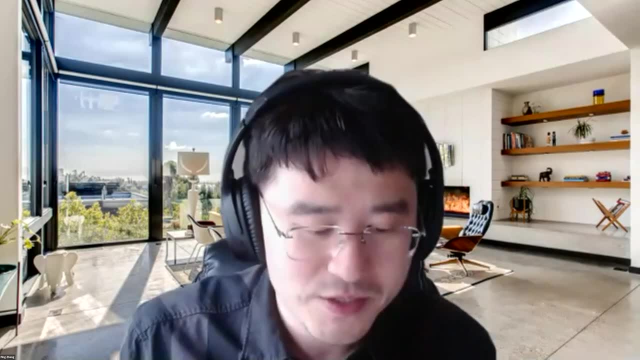 professor Lacing from Stanford university. He's the director of the medical physics division at Stanford university, So he is very famous in the medical image. artificial intelligence in medicine treatment and planning, image guided intervention, neural manage medicine and application to a molecular image in radiology. 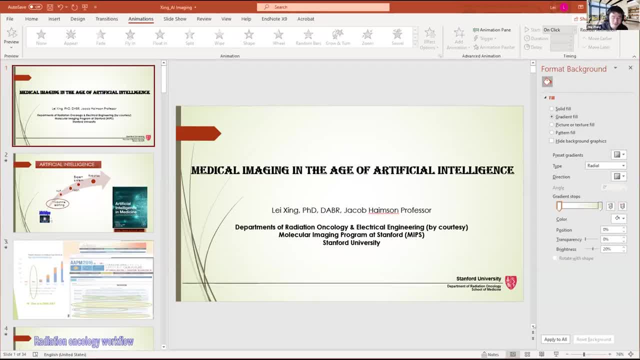 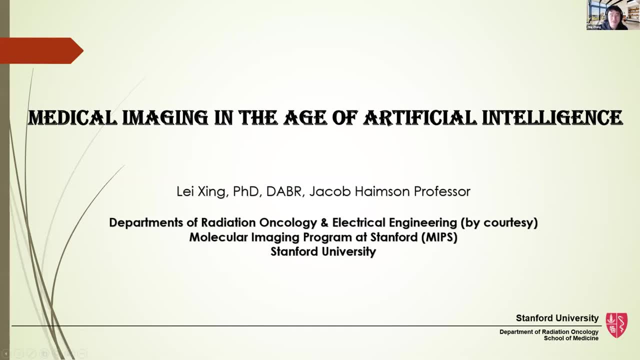 So he is a PI for many, many grants like NIH, DOD, NSNA and other awards. He's a fellow of AAPM and AIMBE And he is also the associate editor or editor in many journals in medical image. Thank you so much. Well, good morning everybody. 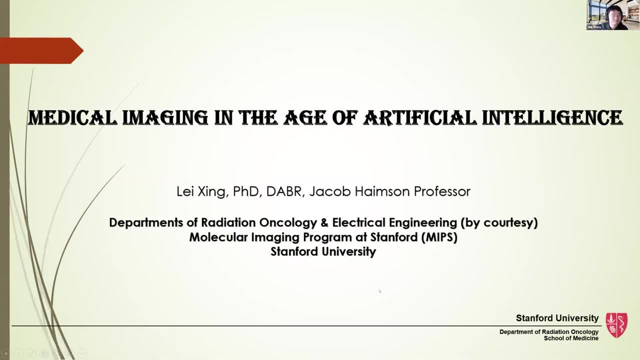 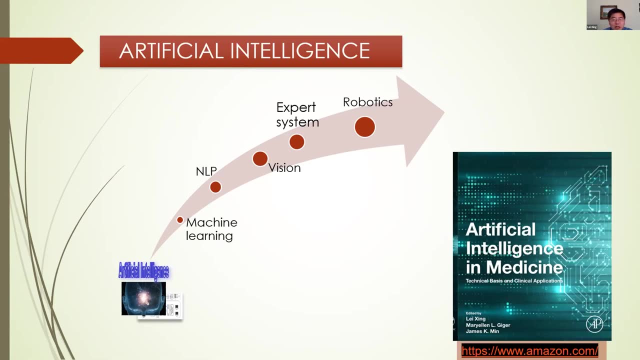 Can you hear me? Okay, Yes, Excellent, Okay, great, All right, Thank you, Like to you know. thank also the all the organizers for putting together this wonderful conference. So I don't need to give too much introductions. Just want to remind everybody, you know, when we 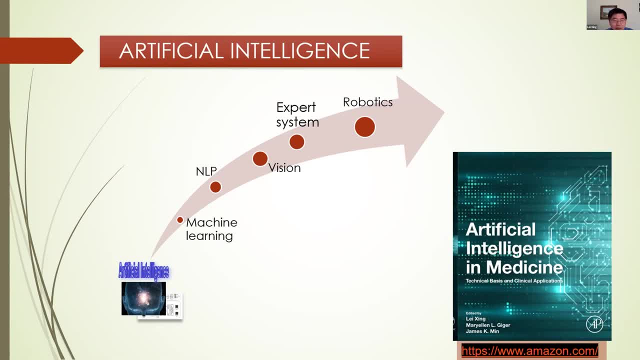 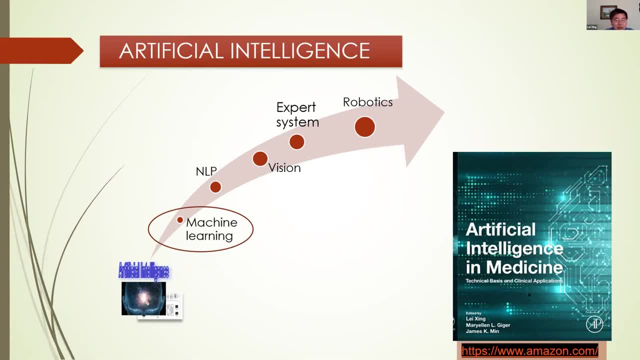 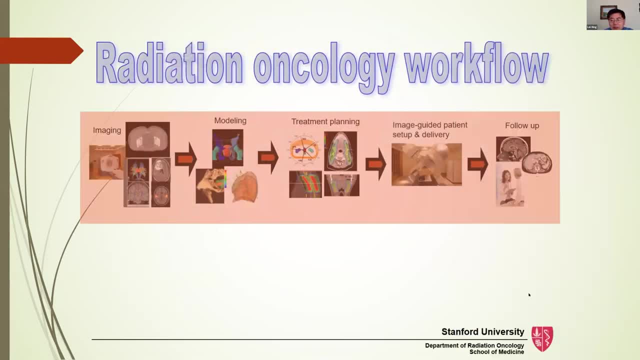 machine learning too. So let's start with clinical workflow. I think it's very important, especially for students, to understand. you know what AI can do and AI cannot do. you know for our clinical decision-making right. I mean, this is our clinical workflow in radiation oncology. 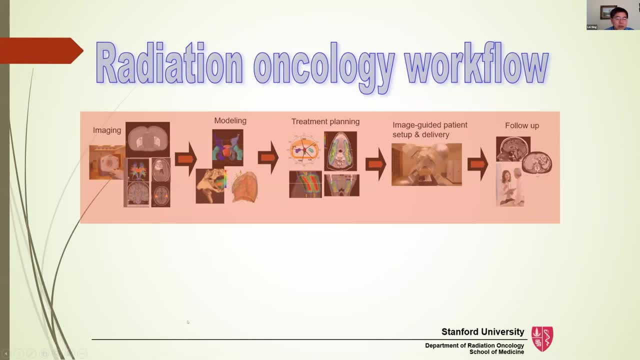 You know when a cancer patient- or actually we go beyond cancer- we treat a lot of functional disease. So I can briefly mention that you know, patient typically goes through a imaging. we call it a simulation. The goal here is really to set up a patient model, right? 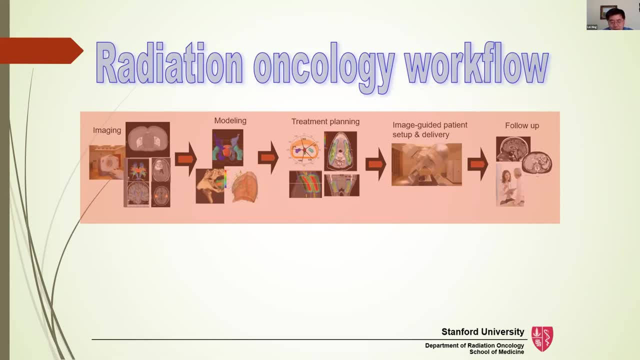 So it's a geometric model that we we set up by doing imaging. So this is not a diagnostic scan. You know, typically we use CT and occasionally we use MRI, and PET is obviously part of that, because you have to identify the target And then go to the modeling. So this 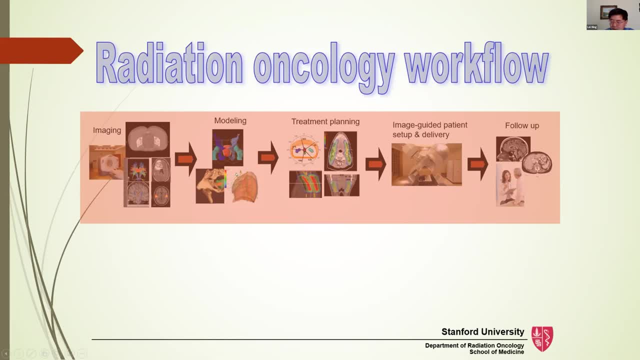 is a part that you build a patient model and then do a treatment planning. So where you simulate your radiation treatment, you know, in the case of a surgery, obviously they should say you simulate the surgical procedure. So what is the optimal path for the needle coming in? 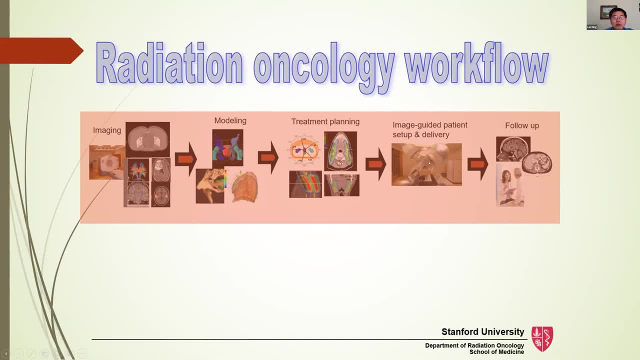 et cetera. And then patient go to the treatment room, treat the patient according to the simulation right And then follow up. you know six months and one year, two years, So there is a follow-up. So in this whole workflow, 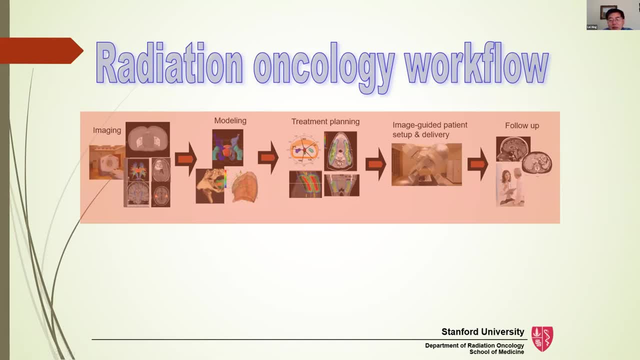 there are a lot of labor, all right- A lot of inefficiency in current practice And also there are a lot of decisions. So on the imaging side, you know we have to do imagery construction right. So this is the task that AI can help with. you know imagery construction. 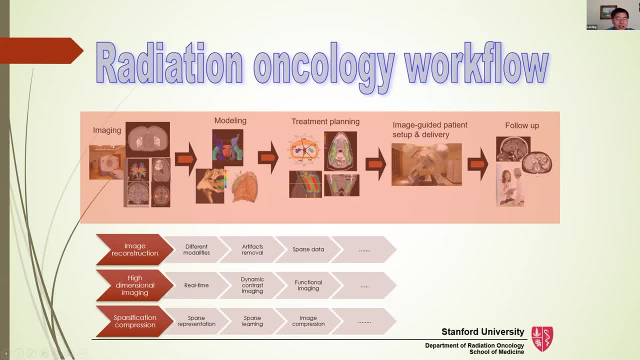 So I will come back to this point, because the current imagery construction is not efficient. It's certainly not ideal, because if you want to take an MRI- I'm sure some people took MRI before You talk about you staying in a dark, cold tunnel. 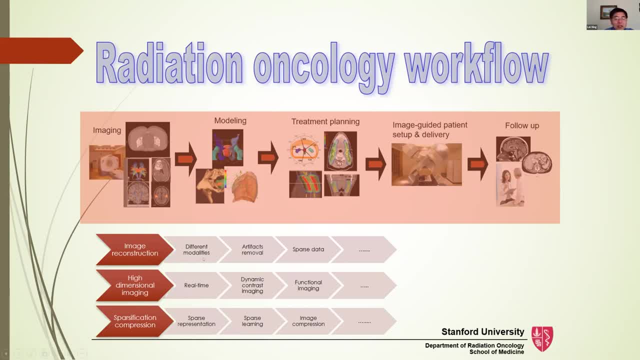 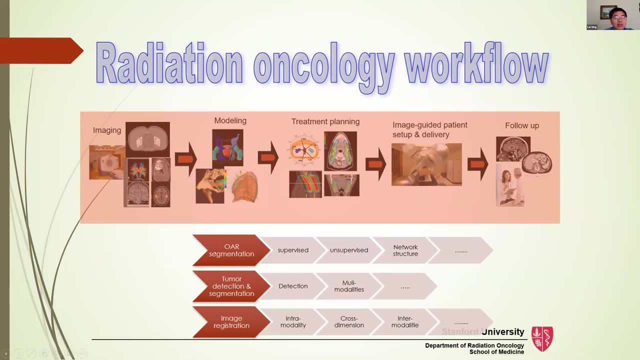 for 20, 40 minutes. So you need to speed up the data acquisition. So modeling, segmentation, tumor target definition and also registration of different image modality, And this actually Dr Lui gave a very nice talk on this topic. 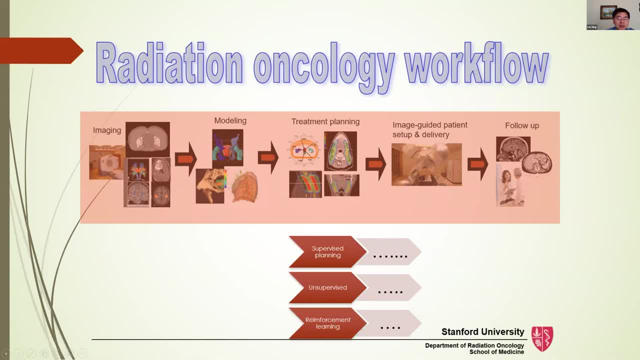 Treatment planning. So this is really specific to radiation oncology. So this is a procedure. like I said, you simulate a patient treatment And on a computer, and so there is a simulation. basically come from two parts. One is the geometry, where you have 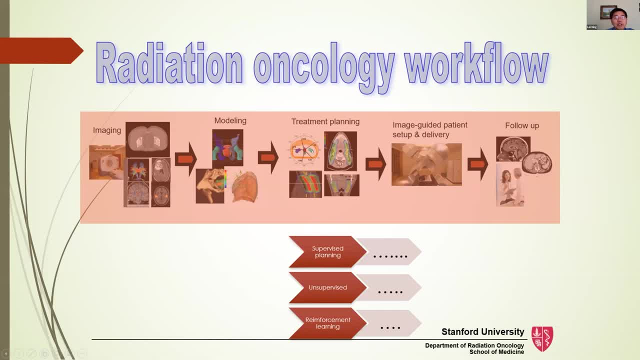 to select what is the best beam for radiation beam to come in. And the other thing is really the interaction between high-energy photon and the tissue. So that is, we have a very accurate model to model that interaction so that we can deliver. 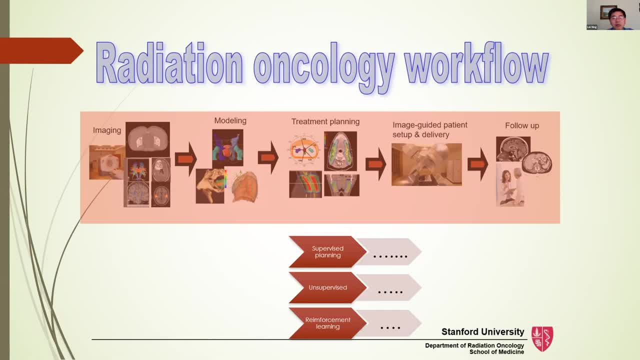 Essentially within 2%- 3% of the dose that's prescribed by the physician. So this procedure needs a lot of image guidance and also the patient follow-up. You have to tell patient after radiation therapy what is the predicted toxicity, what is the survival. 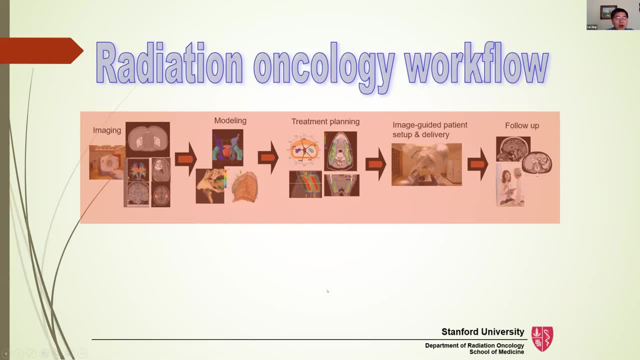 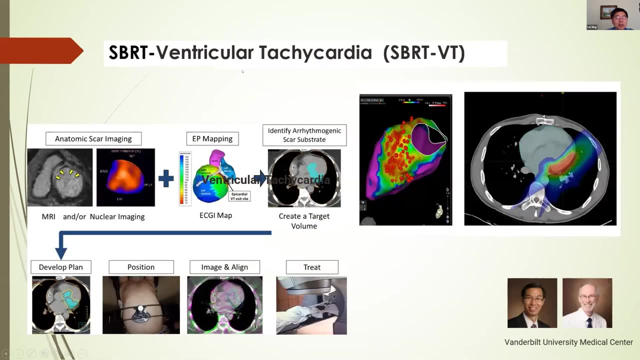 So all this decision can be helped, that can be made much easier by AI. I mentioned that we treat not only cancer patient, we also treat a lot of functional disease and also even the cardiac like weighty. So this is just say an image basically on the heart. 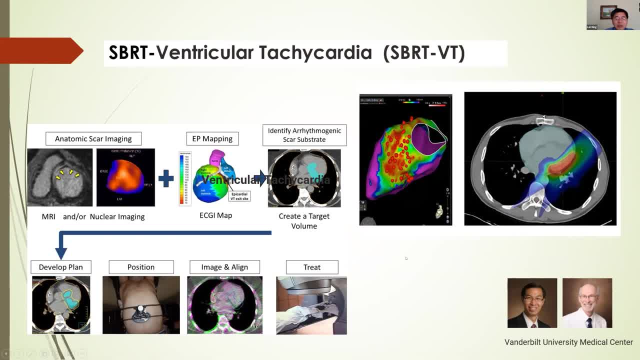 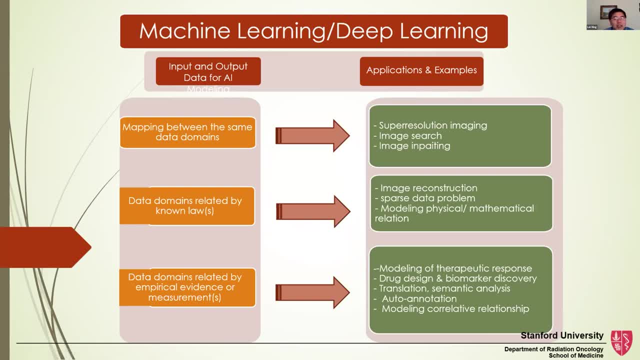 and then you actually define a target And then use radiation to treat the disease. So, mathematically, I like really to simplify the deep learning into a problem of mapping. You're mapping from one data domain to another data domain. Really there are three categories. 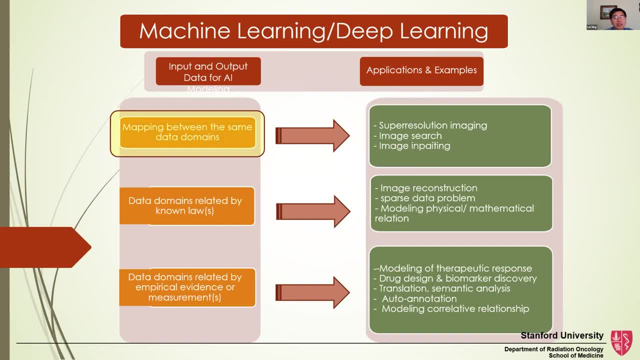 The first one is really you're mapping between the same data domain. This is the same. This is probably the easiest task. super-resolution imaging I mean. I'm sure you're familiar with that concept. That's an example. You just want to really map a low-resolution image. 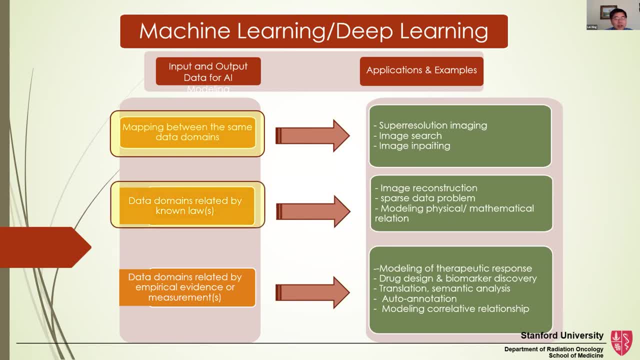 to a high-resolution image. So the second category, the data between input and output, belong to a different domain, like imagery construction. So that would be a good example: You measure the data and then you map that to an image domain. So there the problem is slightly more complex. 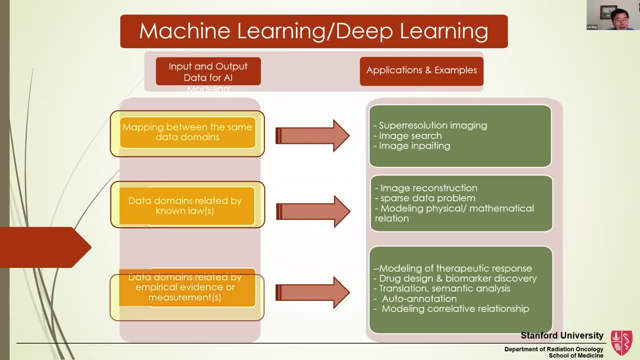 because you have to change the domain. And the third type is really- it's also different domain but different from second category- It's a two type of data. I have no idea. It's either a physical or geomagical relationship. 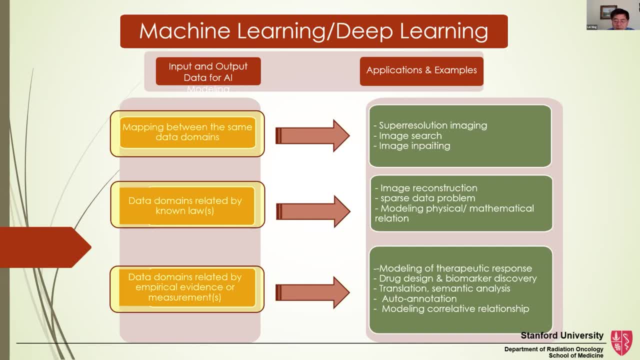 But you know they correlate each other, but you don't know what is the relation. Like a clinical trial, right, You gave a certain drop like cisplatine or immunotherapy to the patient and what's going to happen. So you have an outcome data. 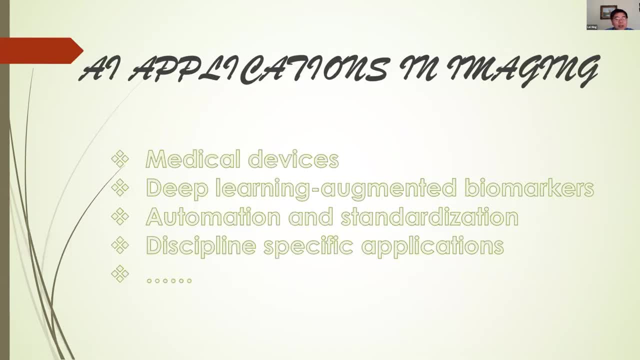 So you try to build a correlated model, Imaging. basically, image is data. It's actually a very special type of data, has a spatial correlation. So actually deep learning has really changed the way that people do image analysis, people do image reconstruction. 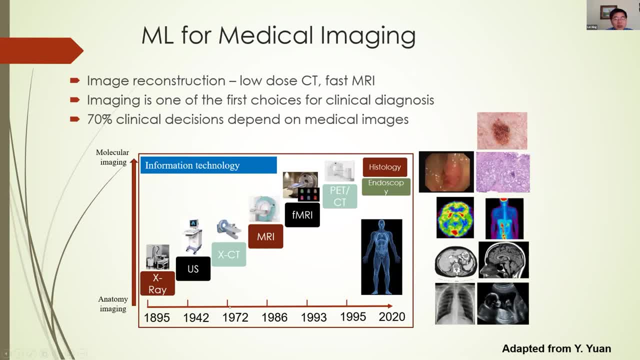 So this are the commonly used image modality in the clinic. you know 2D colonoscopy and then dermascope, you know cystoscope et cetera, And then on the 3D side, PET, fMRI, MRI, CT, et cetera. 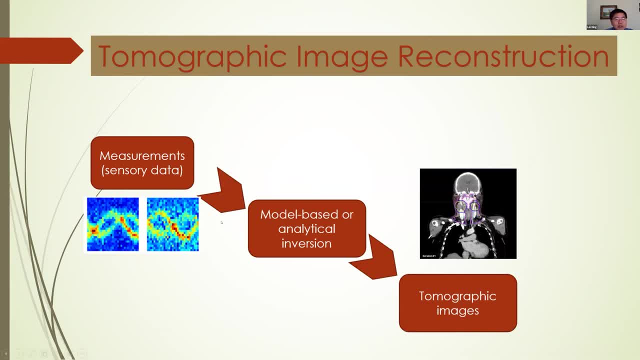 So image reconstruction, you know this is where actually I can see that deep learning can change the way people do image reconstruction. So currently in all the commercial CT MRI scanner or ultrasound, you know the reconstruction is based on the physical model, right? 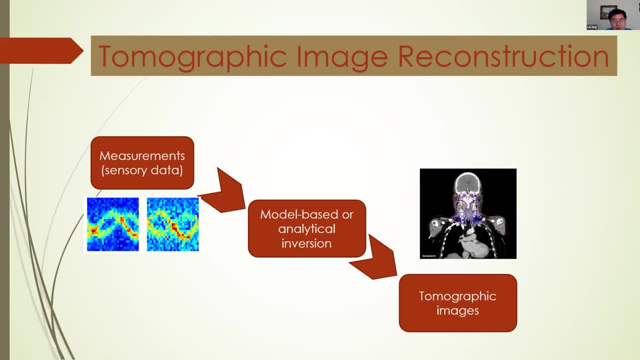 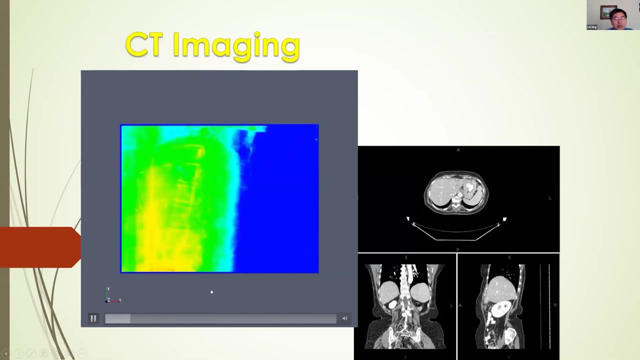 Either a model-based or analytical model. So you do a so-called in the CT, you do a radon transform to universe, the measurement data to the image domain. So what I'm showing here is a data acquisition process for a cone beam CT. 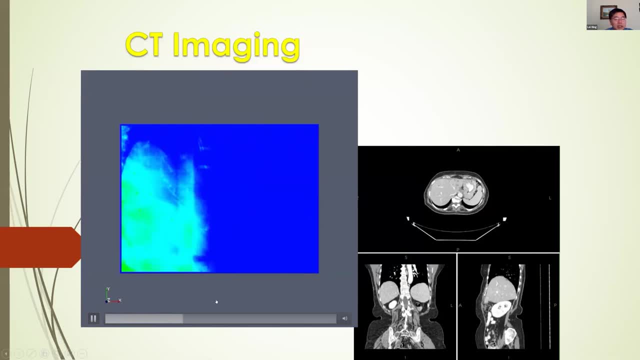 So this is one of our- actually our- lung patient And typically you need to collect a lot of data: 1000 projection from zero to 360 degree surrounding the patient. So the condition: if you are electrical engineer, you know that you have to satisfy the so-called 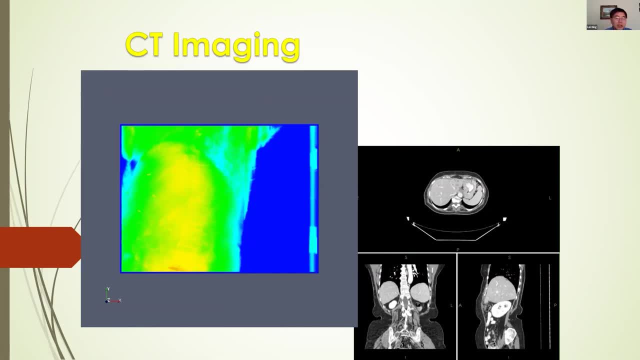 Shannon Nyquist theorem right, Because you have to have enough sampling in order to get a, you know, really a decent image. But this is not true anymore when you have a deep learning. Because, Shannon Nyquist theorem- you know people call it a no free lunch theorem right. 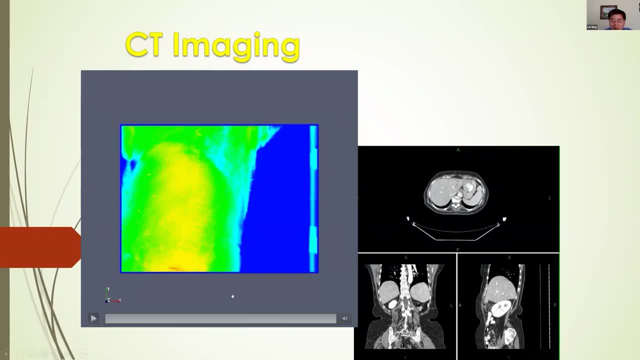 Because if you want to get a high resolution image, you have to pay. So you know, if you want to get a high resolution image, the reason you have to pay it: because you don't include any prior knowledge. And so if, once, you have a prior knowledge, 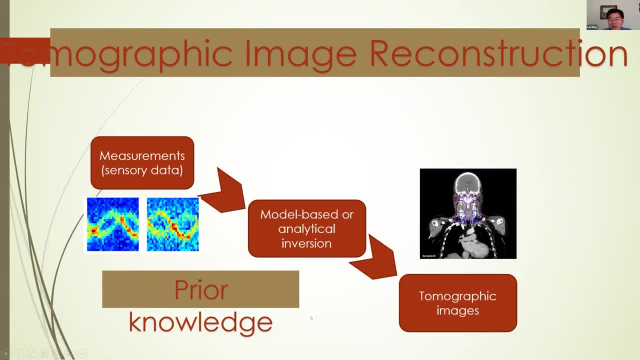 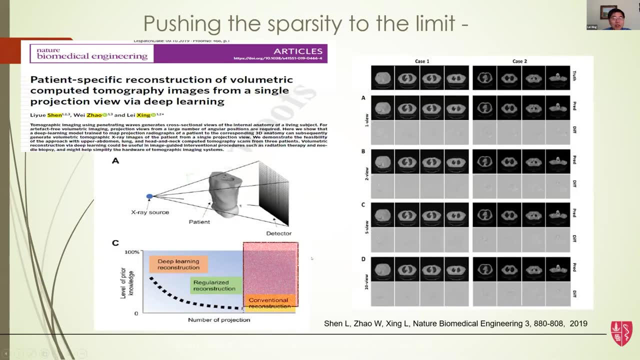 and then you don't have to pay. So so you can get a free lunch, but you know, maybe it's you can call it a leftover lunch, right, Because it's a free, free. it basically is: it's a prior knowledge. 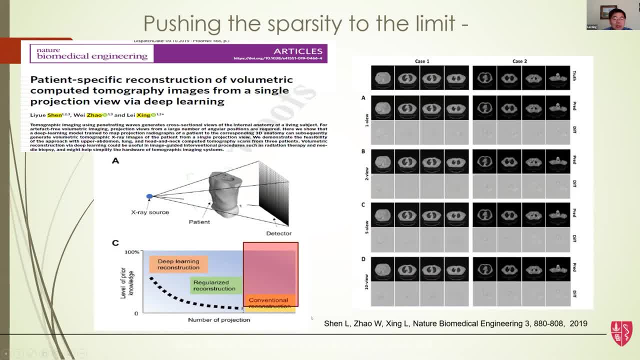 It's. it's a leftover lunch. You can order it from the previous patient. So this is conventional imagery construction scheme. You have a number of projection. that's basically sampling, And this is the level of prior knowledge. So if you don't have prior knowledge, you're here. 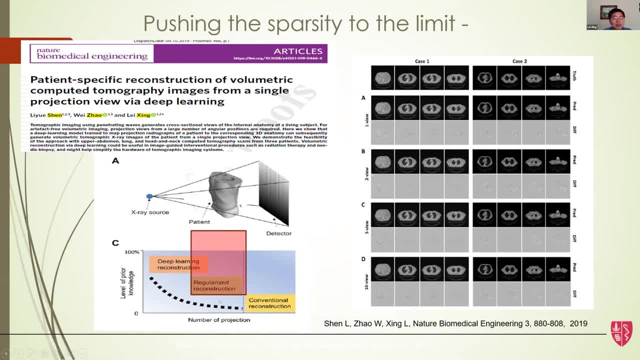 If you have some prior knowledge- and this is so-called the regularized imagery construction And before the deep learning. you know a lot of people work on, you know you have to pay, You know using compressed sensing, et cetera. 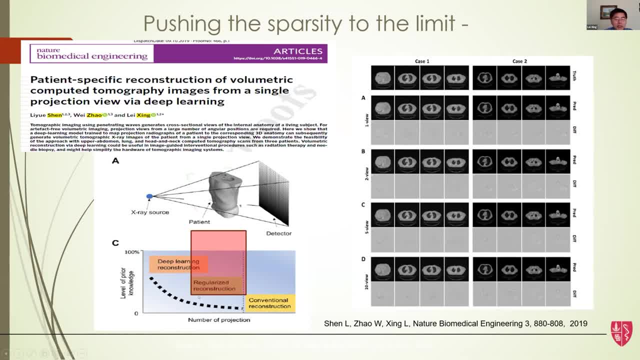 to include some prior knowledge, So you can reduce the number of projection, but not too much. With deep learning you can really push the push the sparsity into the limit. So so in this work we actually push the sparsity to one single projection. 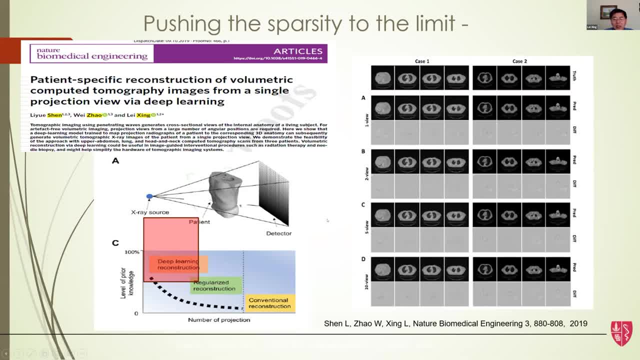 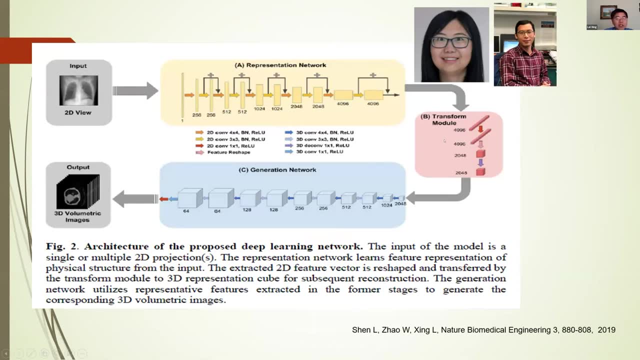 So what that mean? That means that when you're taking a test x-ray, you actually can use that information plus prior knowledge to reconstruct a volumetric image. So yeah, this is the reconstruction process. So, like I said before, you know, 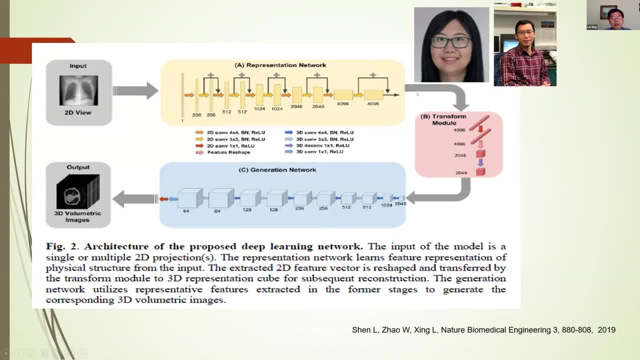 you have a 2D measurement data and go through, you know encoder and then dimensionality transformation in the image domain, in the field feature domain, and then you know you do a decoding so you get an image. So that's how. 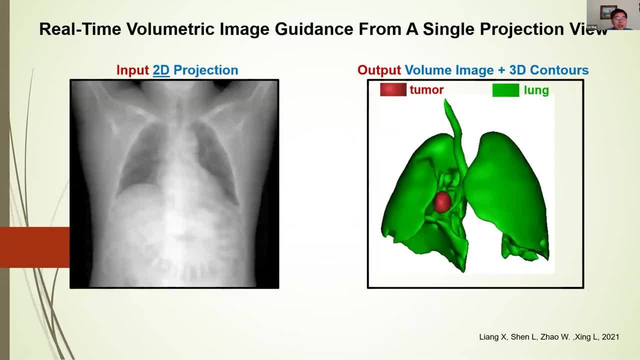 it's a very complex network but it works. So- and this is actually one of my postdocs, Xiao Kun, so he did this work- you know, you can actually use a fluoroscopic image and then convert that into a so called a 4D. So this is a 4D image. So 4D, you know, 3D, spatial and the 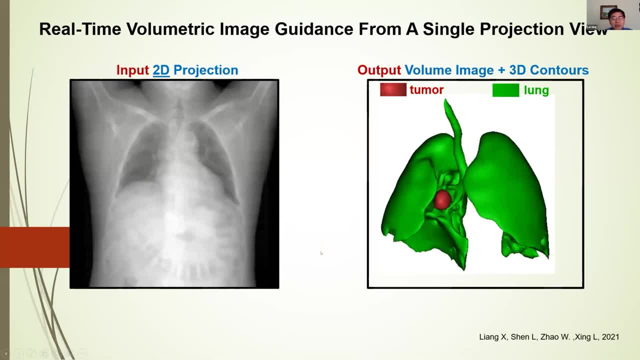 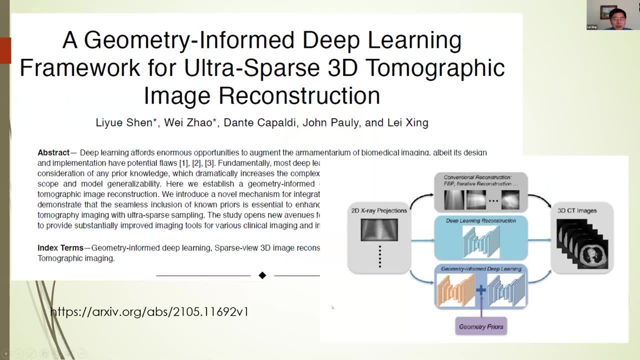 plus 1D time. So this is. you really can push that into limit. So recently, actually, we pushed this reconstruction scheme further. So this is basically try to include, you know, some known genomes. So this is a 3D image. So this is a 4D image. So this is a 3D image. So this is. 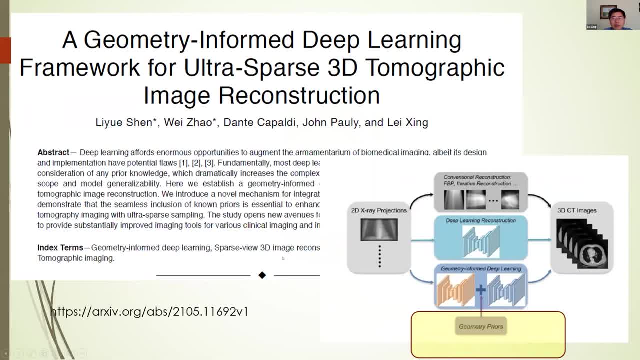 own knowledge into the deep learning process so that we don't have to have a very complex network. right, because if you can inform the deep learning algorithm with some geometry information of your imaging system, you can actually do much, much better. so this is already in the archive. you. 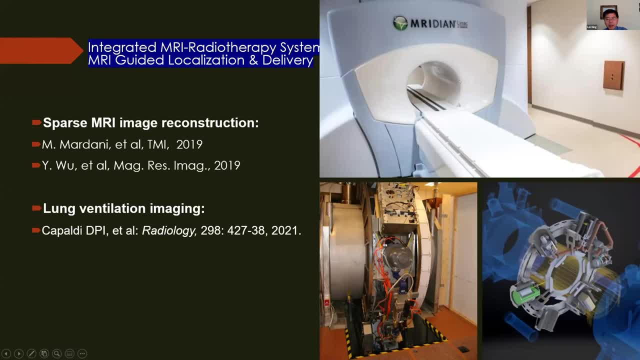 can find it. uh, this is our mr linux machine. so it's the same thing. you know, sparse reconstruction, you can use that to speed up. speed up the mr reconstruction too. so you know, in a nutshell, this is a, a hybrid between a linear accelerator and uh and mr, ms, mr system. so, uh, the 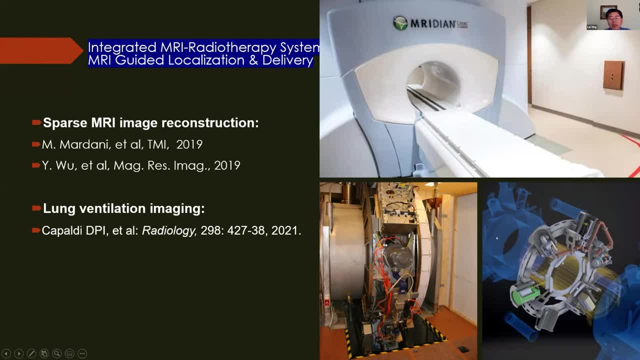 mr provides real-time image to guide the delivery of radiation uh to the patient, but today. so this guidance is actually 2d. so you know, because you have to take a lot of data, so the reconstruction very, very slow. you can only get real-time 2d image. you know, either sagittal, axial or 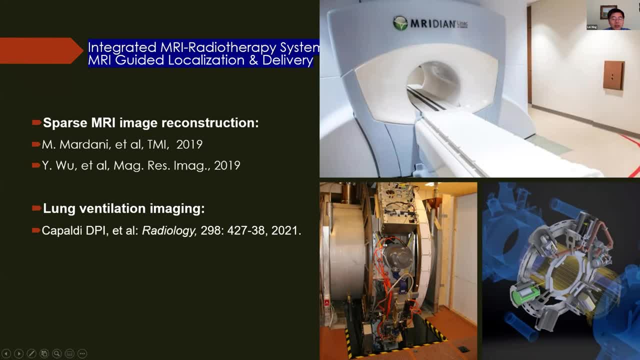 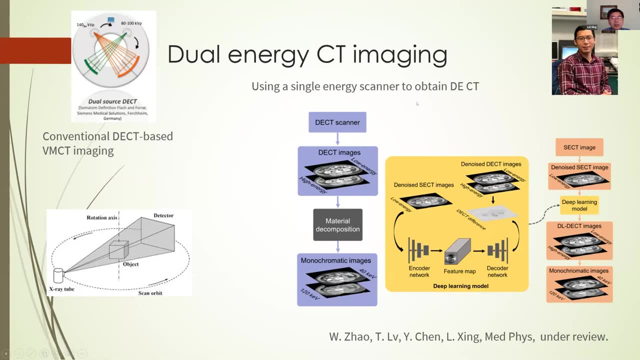 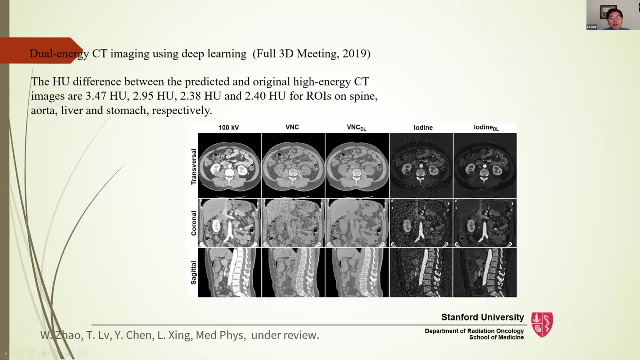 any plane if it is 2d, so which you can use that to do the deep learning. you can push that into 3d in real time, right, uh? this is another related reconstruction, so you can actually use a single energy ct, so, which is much cheaper and widely available, to derive a, you know uh, derive a dual energy city, which is very 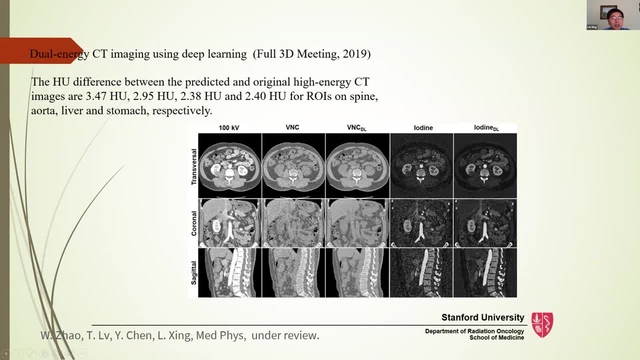 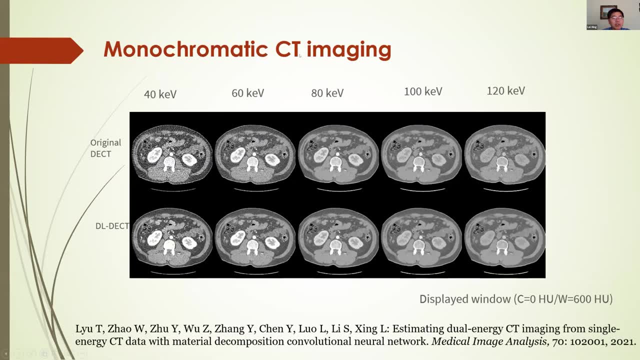 expensive and, uh, also, you know, has a lot of technical issues. So so that this is, you know, really a deep learning, bring a lot of free lunch to us and then you can even convert that into a monochromatic energy. so like a 40k you can use basically a regular CT scanner. get the, you know. 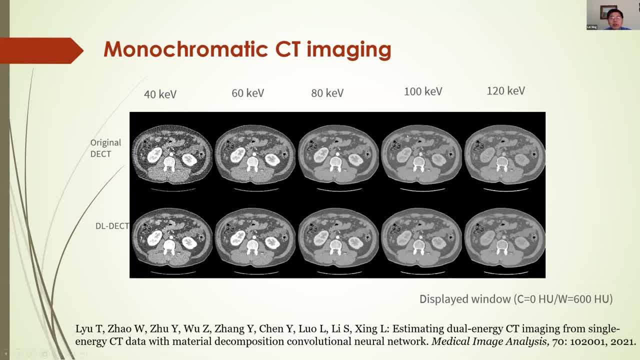 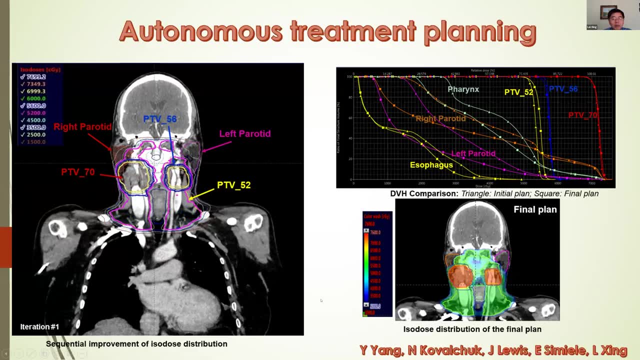 monochromatic energy CT. so this is really important for quantitation of imaging modality. But I'm not going to the detail of the application of, you know, monochromatic CT. so treatment planning: We were able to again use the treatment plan from you know prior patients. 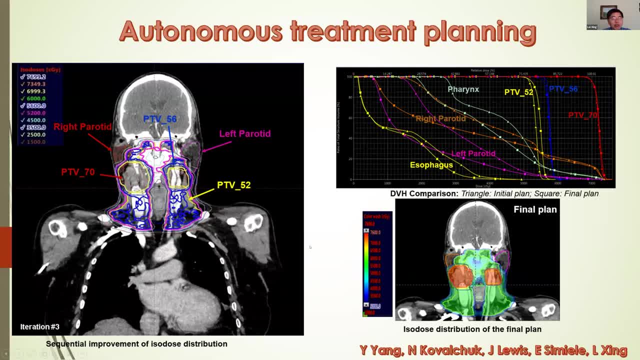 And then to speak, Speed up, to automate the treatment planning process. you know, for a patient like this, this is a head and neck patient. We talked about one day, or even two days, labor of a technician. you know the only thing he does, you know, it's really just sitting in front of computer and tweaking to get a, you know, desirable, those distribution. 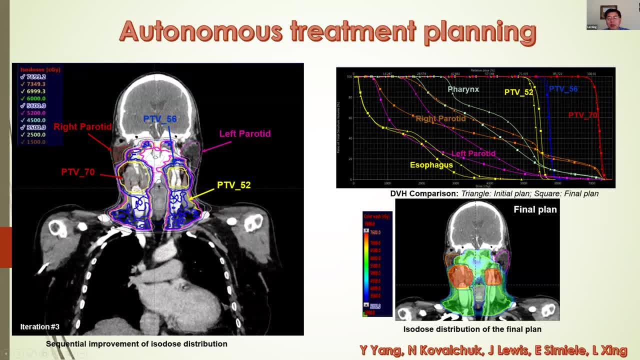 This takes one day or two For the complex case and you know, with a computer you just with a button push, You can actually get it down. So this has obviously has a lot of clinical impact, Because you know reducing. so talk about, you know, AI replacing human. I think this technical repeated work will be replaced by AI. 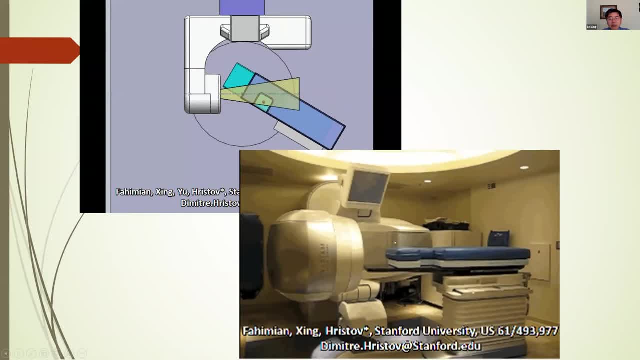 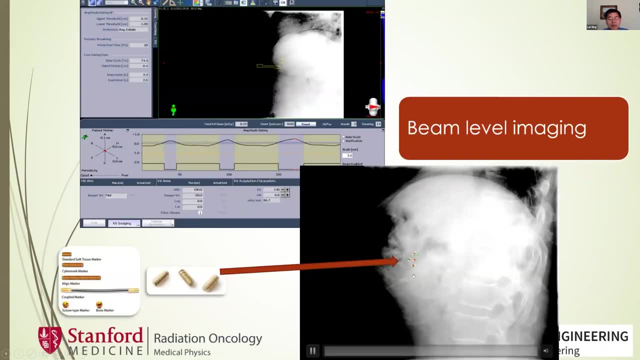 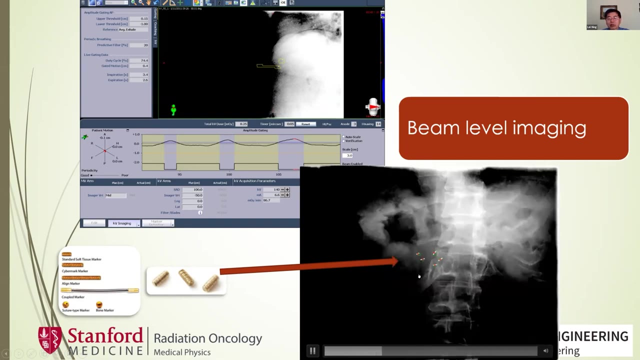 So we talked about the radiation therapy delivery. so this is the machine. So this is the machine. The machine has a lot of bells and whistles, but I guess the key issue is how do you visualize, how do you identify the tumor? you know, doing the treatment? 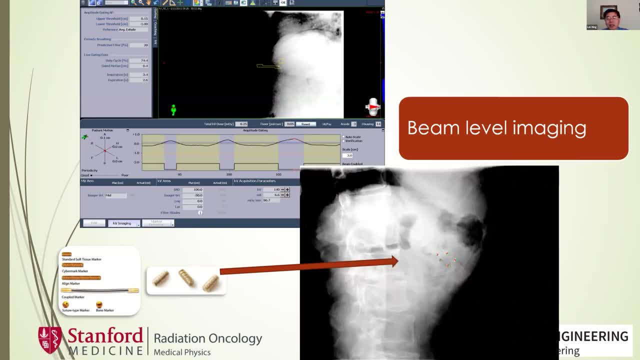 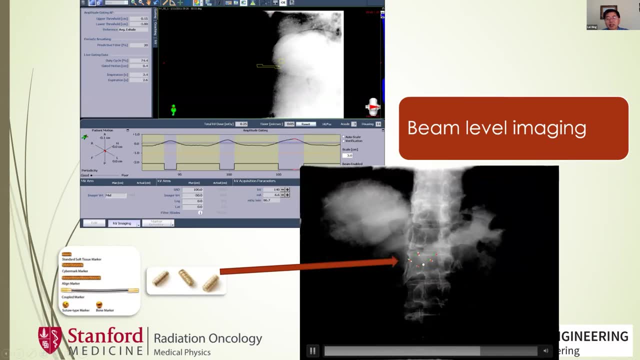 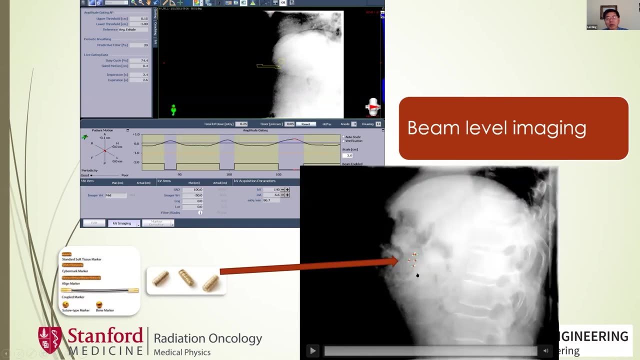 So I show you the MRI CT machine. but this is actually a integration of x ray image with a linear. So what you're seeing here is a patient. This is actually seen on the on the x ray image. So in order to see them, we have to surgically implant some metallic- like in this case is a book gold- into the tumor in order to see them on the x ray. you know, obviously this is costly, invasive. 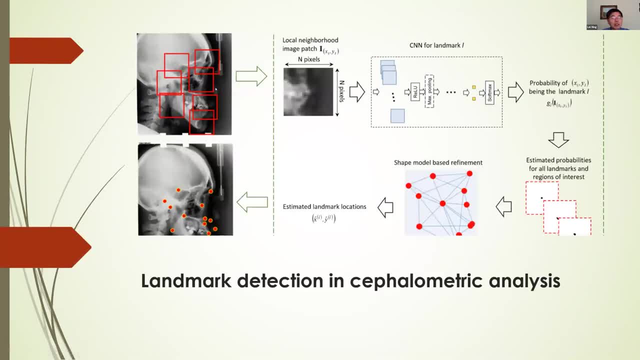 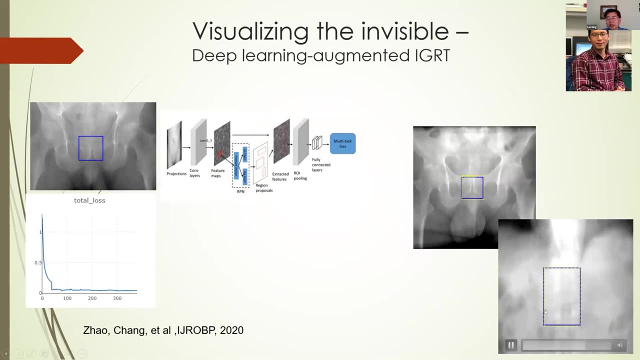 So. so with deep learning, You know the question theory is: can you actually use deep learning to identify some inherent tissue marker right, So that you don't have to implant those, those gold marker? And this year it's actually It's been done. you can see that this is a pancreatic tumor, that without fiducial, we can actually track the motion during the treatment. this is the prostate patient. 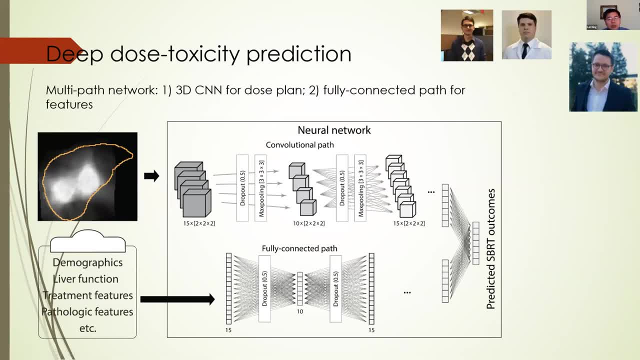 So, in terms of predicting outcome, Predicting the toxicity, this is also very important. So, current practice: you- you basically based on your training, your physician or the resident, Make a prediction based on some historical data. right, you tell patient you likely to survive three years or five years, etc. 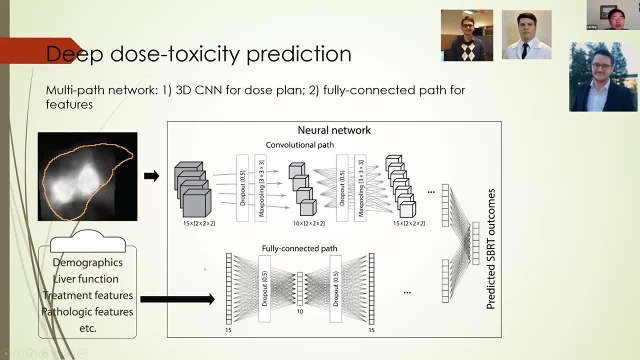 It's a very accurate. so this normal ground based approach very accurate. It's actually a A lot of clinical implications. So here with a deep learning We can train model including. so really just individualize the prediction, right you. 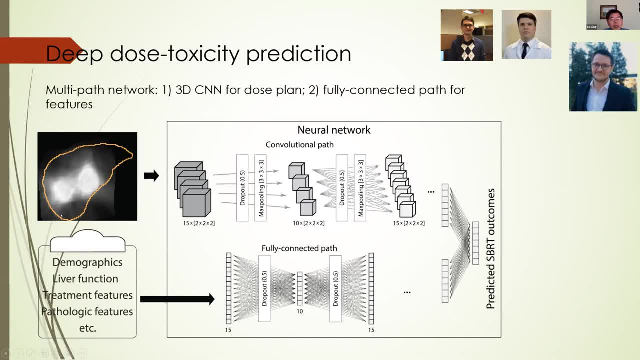 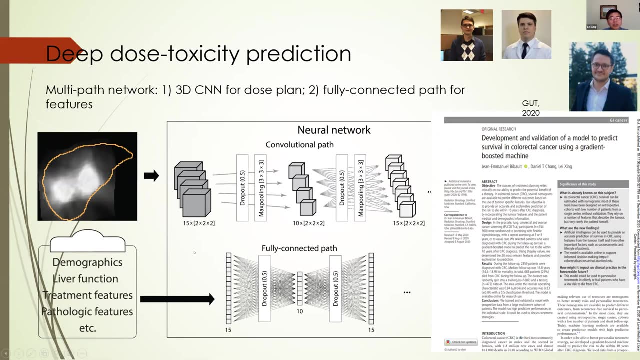 We have not only image, but also the SO, those distribution, the treatment plan and also demographic information. so feed them into a deep learning model And then you can. you can actually Predict. You know what he is, The chance for patient to survive and what it's. 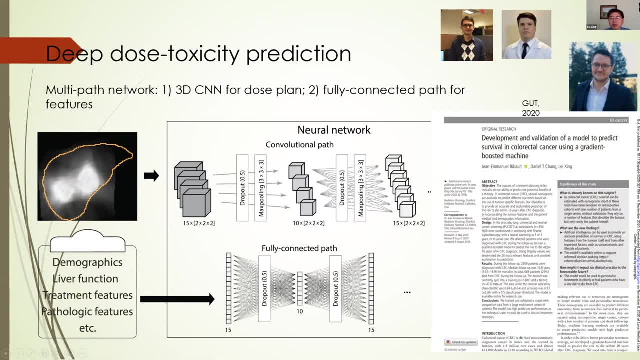 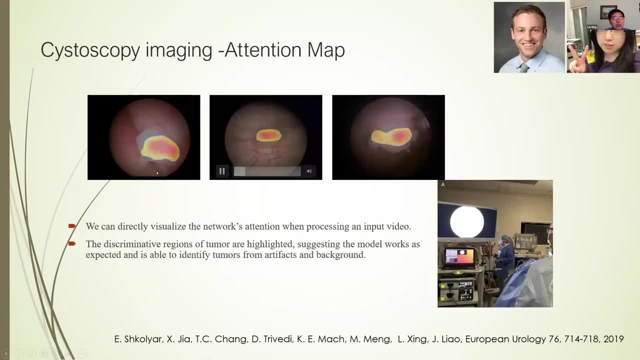 What are the possible complications? so, so, this is our senior work on colorectal cancer. You can, You know, talk about image guidance. so this is a work in collaboration with the urologist Joe males group. So we are actually, you know, analyzing system scope image. 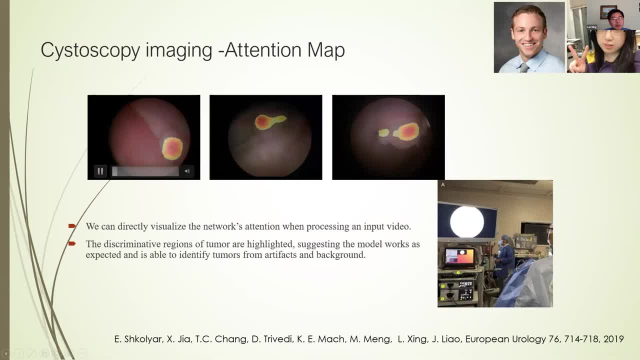 Basically, Basically, use the system scope to build a existing model, to build a beauty deep learning model, to identify the high risk region During the actually the surgical procedure or system scope procedure. you know, you know, for those who are not familiar with the bladder to bladder tumor is actually the most expensive tumor to manage. 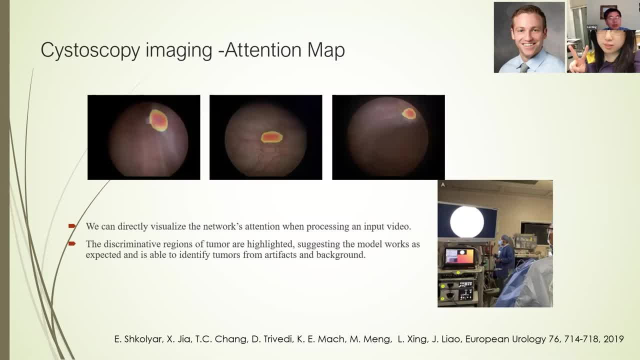 Because you know the false name Is, you know the false negative rate- false positive, false negative- is quite high. And also you know the patient has to be. you know, once, Once diagnosed the, you know the patient has to really monitor. you know, almost like every three, six months. 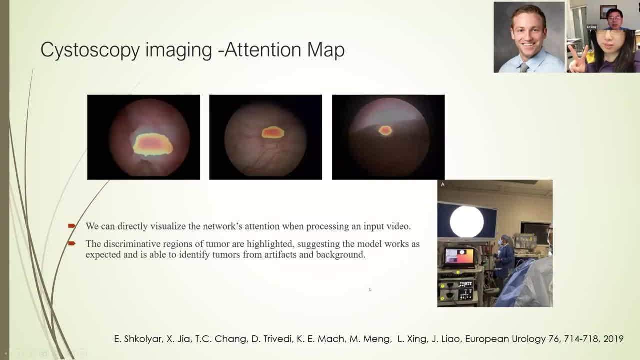 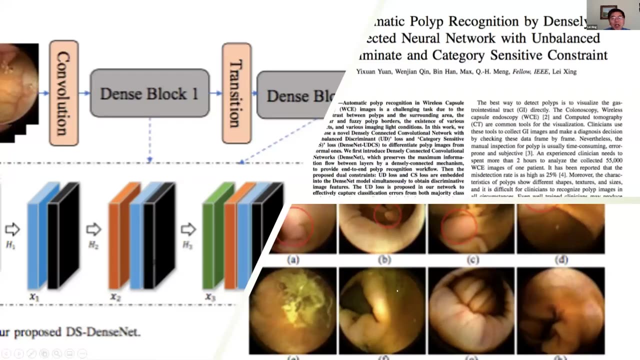 So so that's why it's become very expensive. so using a you can actually really reduced The Mistake And then, you know, provide some guidance. you know our room, So the same technique actually can be applied to. you know, colonoscopy, right colonoscopy. 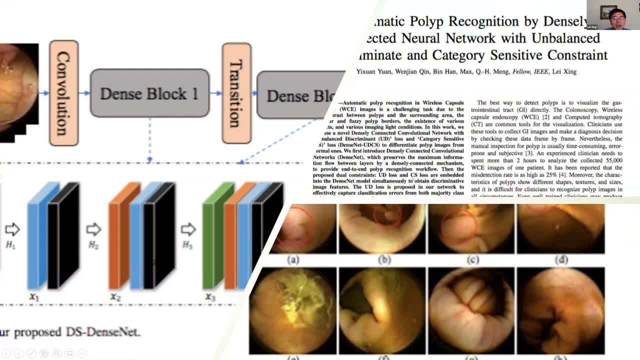 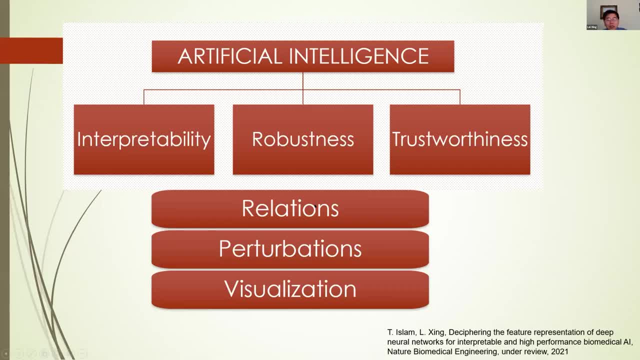 It's a different problem. You know it's actually a. it's a very long procedure. sometime up, you know, physician get tired doing the procedure, So so it's very important actually to To how I, To how I. 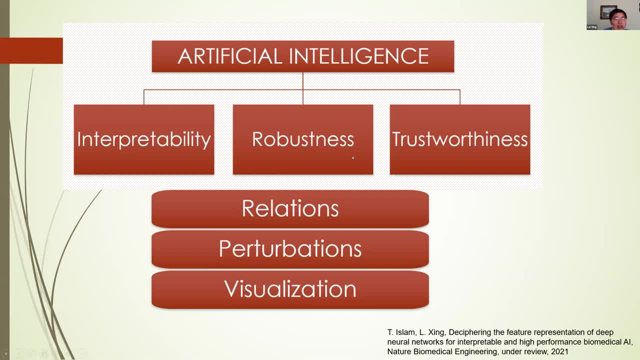 Just to identify it's a high risk region. Well, you know, I think one of the very important question is: you know, how do you trust the AI model right? that's interpretability, robustness, trustworthiness. it's a It's very important. so we work- We have done some work recently- along this line and you know, basically there are three. 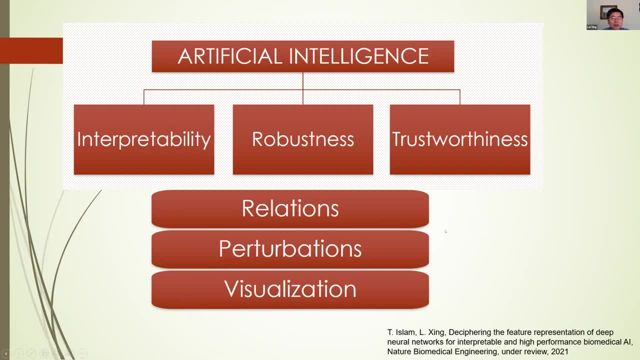 We have done some work recently along this line and you know basically there are three. We have done some work recently along this line and you know basically there are three. One is a Type of approach to enhance the robustness right. 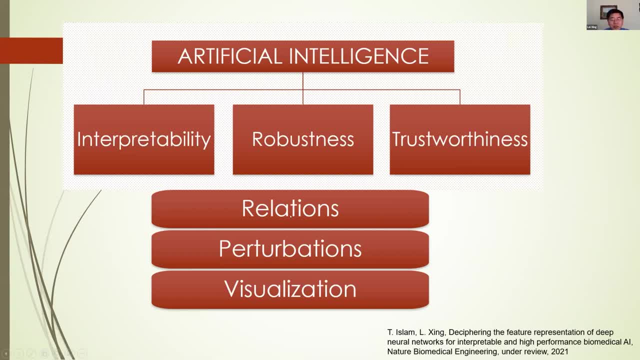 So, or to understand, To understand Deep learning model. So one category is really you, you'll find a relationship right, you, you know like attention, or you know Just a heat map type into your network, into the input data and to see what are the response. So. so the third type is really- I think it's more fundamental. it's really you know how can I understand the feature space data right, because 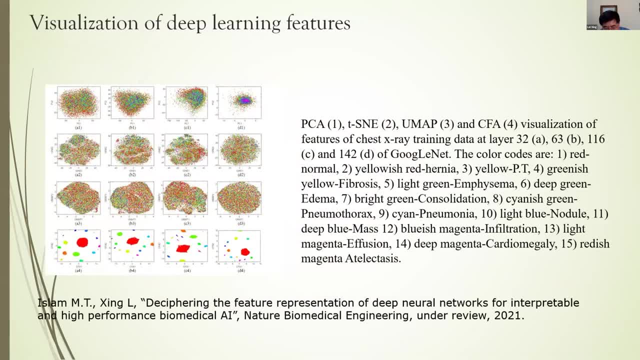 I know it's a black box And you know, once you go to the deep learning model, you don't know. you know you may or may not get something meaningful out of the model. And, even worse, you know you get a result, you don't know whether it's right or wrong. so so, visualization of the feature. I think it's very important. 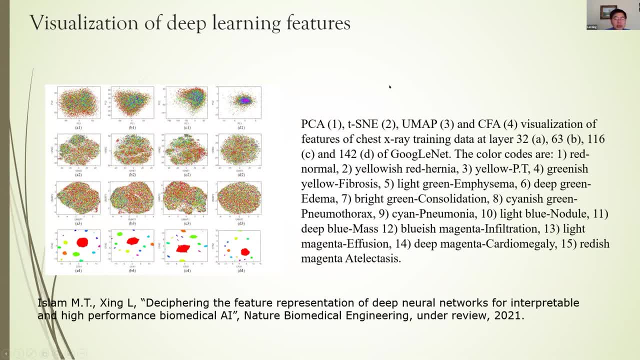 But currently there are many techniques right: PCA, t-SNE, UMAP, etc. So so this is actually a very interesting example. So this is a Google net. We use NIH. you know that x-ray test, x-ray data that Dr Liu involved. 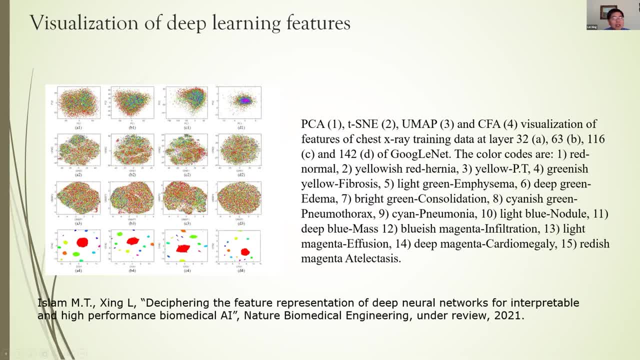 You, you can see that with t-SNE, and this is actually a visualization of different layers, So the layer up here, 32, 69.. So with this t-SNE or, you know, any existing technique, you actually don't see the cluster. 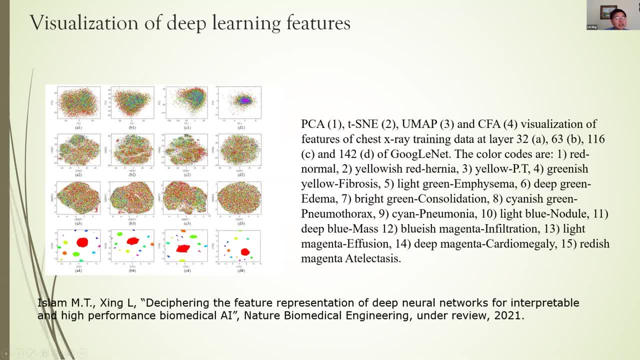 Okay, So this is actually using a learning based clustering technique. you can see that even at a very early- like a 32, we can see the 14 classes So that actually go along. you know when you go change from one layer to another. 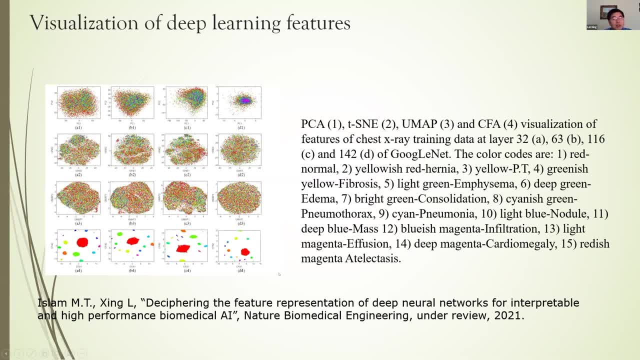 So it's really, you know, monitor this whole process. So I think this type of model is very important, You know, for for the future of deep learning modeling, because not only we can see them, we can also tell you which layer is not doing useful job. 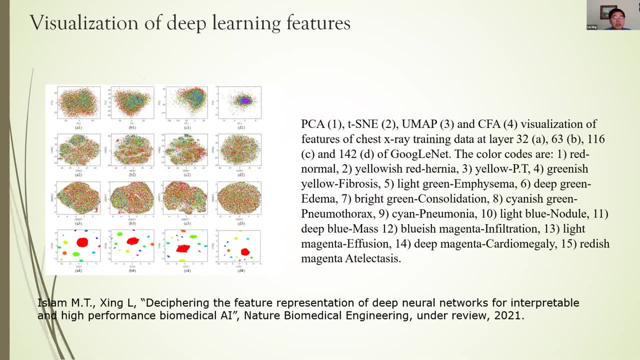 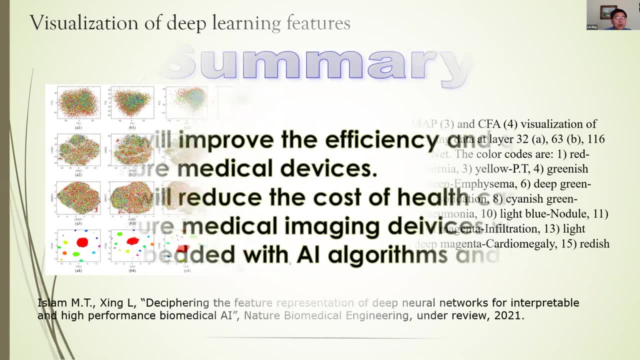 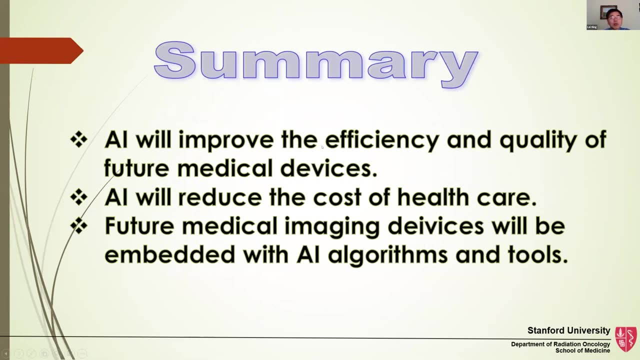 It's actually making the work, make the model worse, So we can actually prune the network to get a better performance. So with that I'd like to summarize: Yeah, So, so I think AI will improve efficiency and quality and also will be reduced the cost of healthcare. 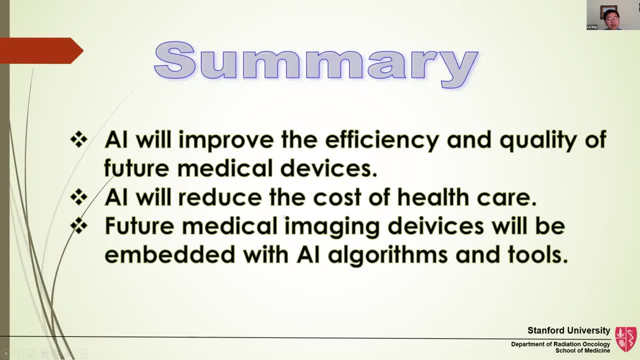 Just think about you know a human how expensive. like you know, like a treatment planning We hired in our department. we have like 11. Even 11 technician just do treatment planning. So each one of them, if they do 30 treatment plan a month and that's a super dosimetrics already. 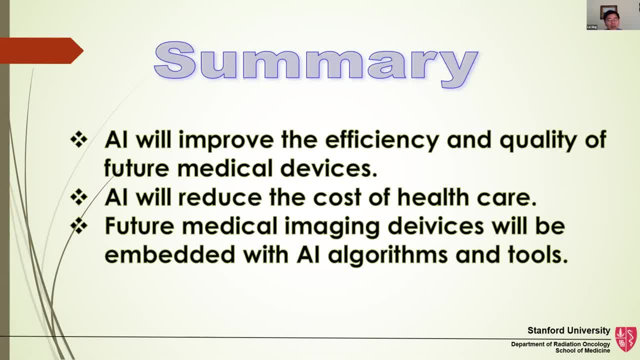 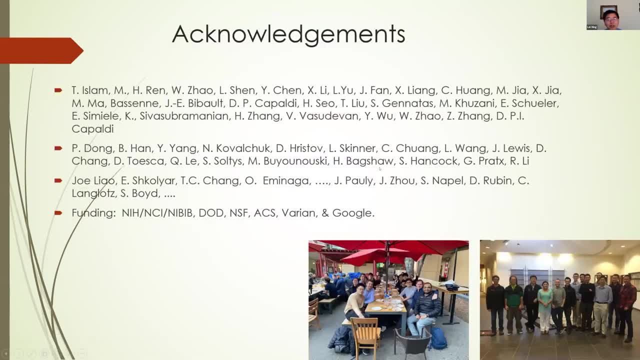 So you know it's computer. essentially there's no up limit. So I think, and of course the robustness and the interpretability are very important. Also like to say the student collaborator and also funding agency. And thank you. 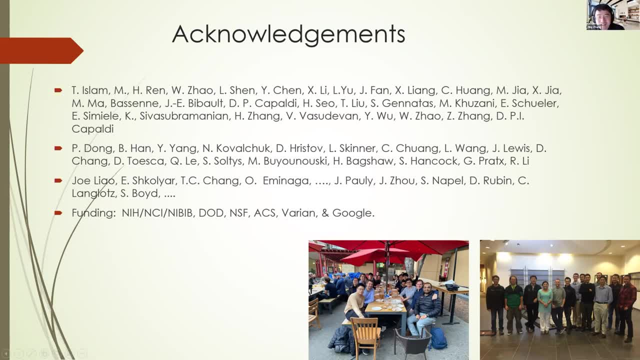 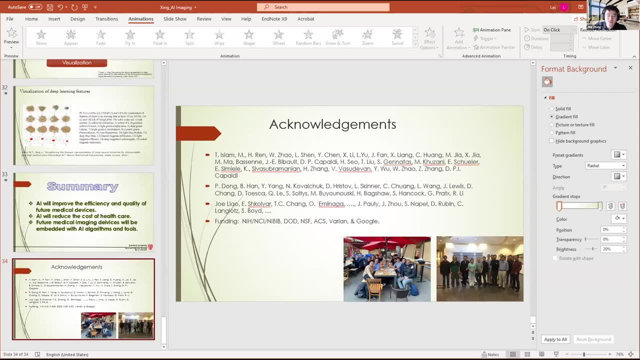 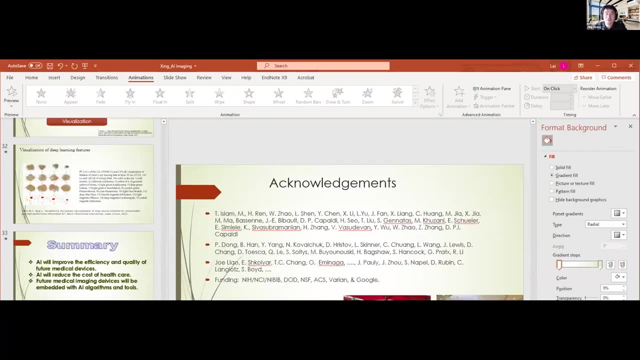 Yeah, that's it, Thank you. Thank you so much. Yeah, So for the attendee who have any question to talk, So please key in the chat box, So Dr Huang will organize the panel discussion after the talk. Thank you so much again. 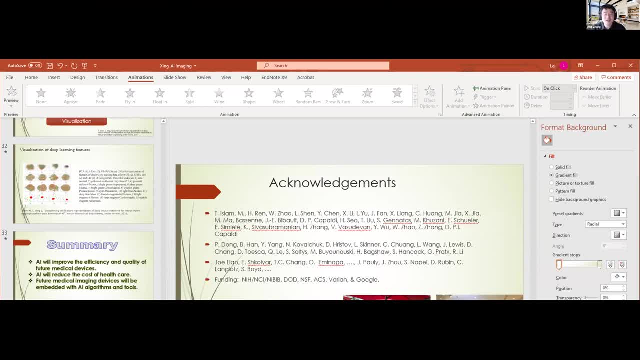 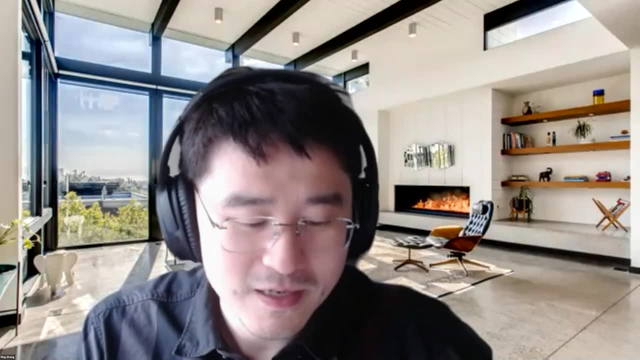 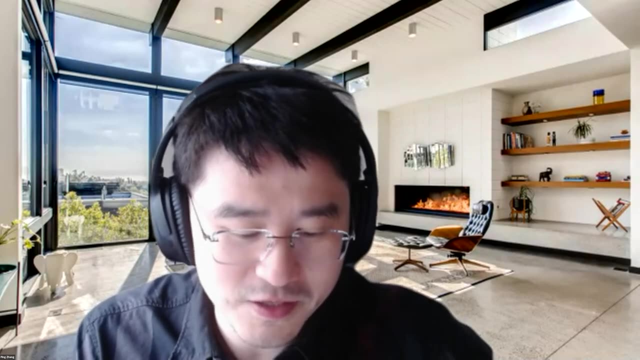 Dr Cooper. So are you here? Okay, Yeah, sure, Thank you. Yeah, Our last speaker will be Dr Lee Cooper, who is who is right now in the during the Department of Pathology of Northwestern in 2019 as associate professor and director of the computational. 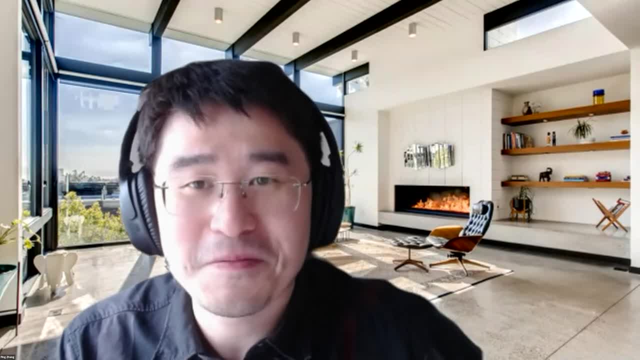 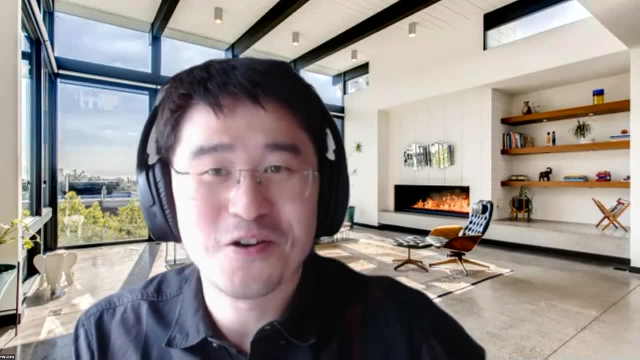 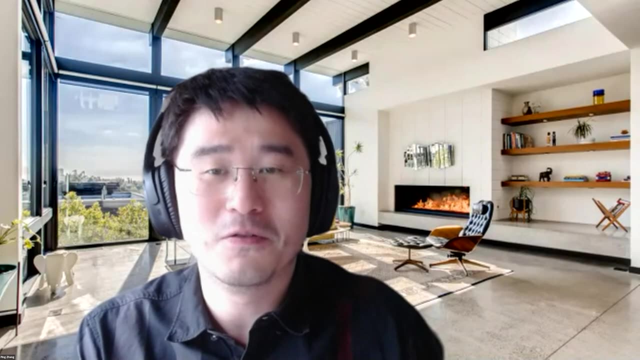 pathology. Actually, is my really my owner to introduce him because he has graduated from Ohio State University in 2009.. So, yeah, Thank you, Thanks. Actually, he has a very successful career Right. So he's really the role model for in the in the both the UC Department of Electrical Engineering. 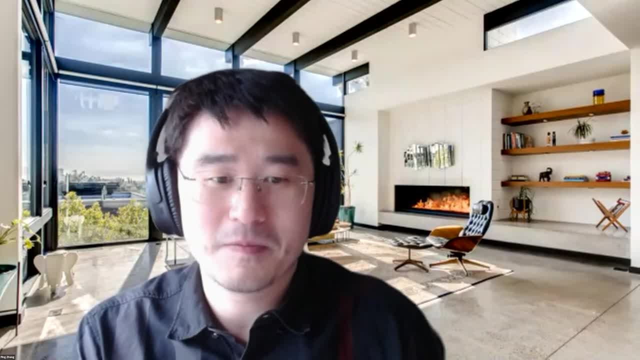 and Department of Biomedical Informatics- Really my owner. So he he joined the BMI as a faculty in Emory in 2012.. So and have a joint appointment in GATTAC and then joined as the associate professor in 2012.. 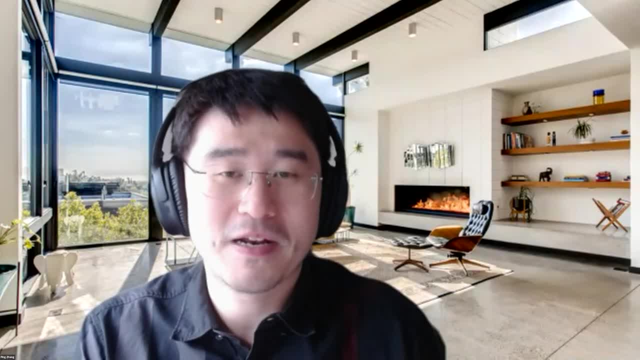 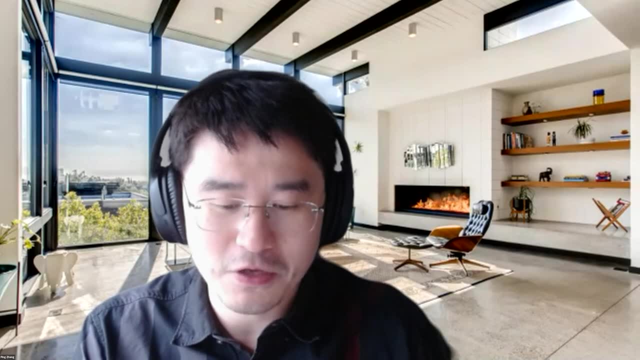 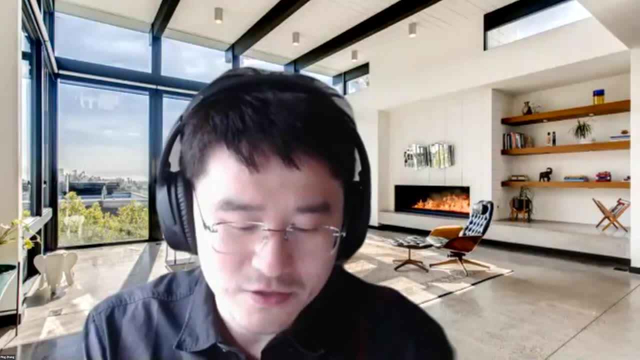 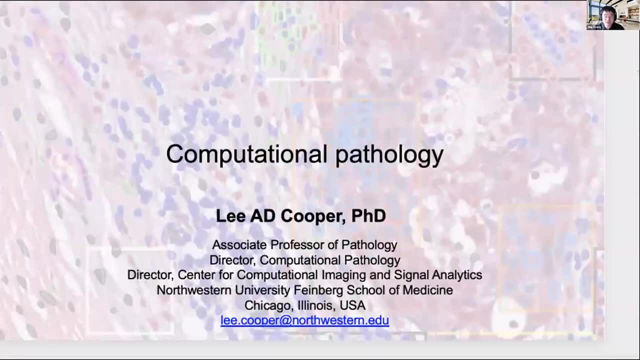 Thank you. So he's joined as an associate professor in the Northwestern So he his research actually funded by the NLM, NCI, N101B and NIMDS and a lot of industry resources. So he published a lot of people in computational pathology. 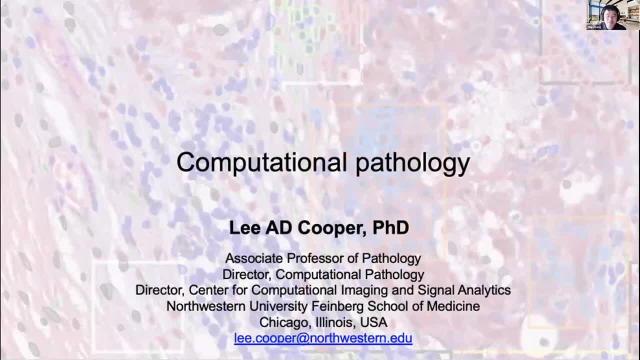 So let's welcome again for the Dr Lee Cooper. Welcome home, Welcome to OSU, Thank you. Uh, thank you, Ping. I appreciate that nice introduction. It's good to be always with fellow Buckeyes. so, um, yeah, i'm at northwestern, i'm in a pathology department, although i'm an engineer, and a lot of. 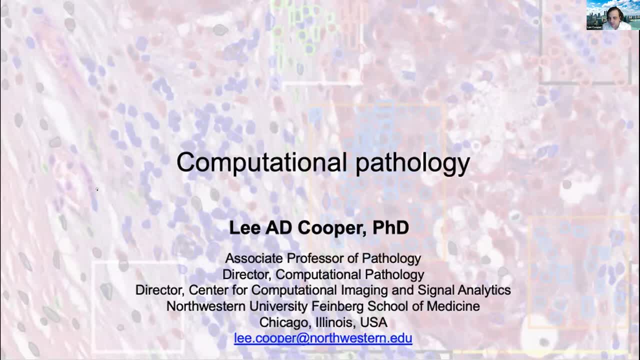 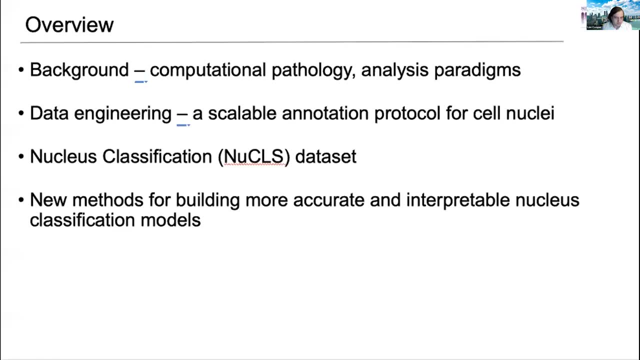 our work just focuses on building. you know informatics tools, you know computational models for prediction and also you know data infrastructure and resources. so, um, today i'm going to just give a background on computational pathology- i think it's a more popular topic, but a lot of people may still not really know much about this- and talk about some. 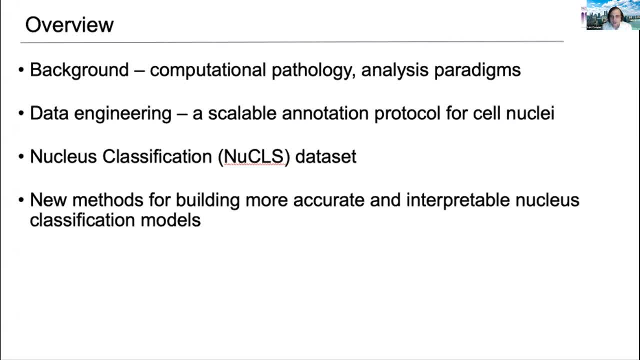 of the different analysis paradigms that are used. i'm also going to talk, you know, the main topic today will be, uh, focusing on one project. it's really a data engineering project, which is like: how do we collect large amounts of ground truth data? and i'll give, i think, a good motivation. 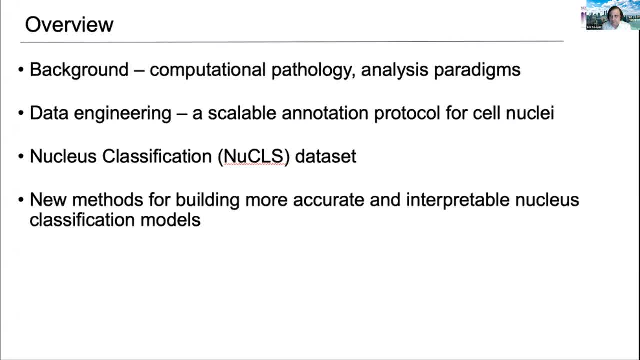 for why. that's the way to think about a lot of these projects where we have really good deep learning algorithms and it's really more about getting the right kind of data for them. and then i'll talk a little bit about some of the work we've done in terms of improving the interpretability. 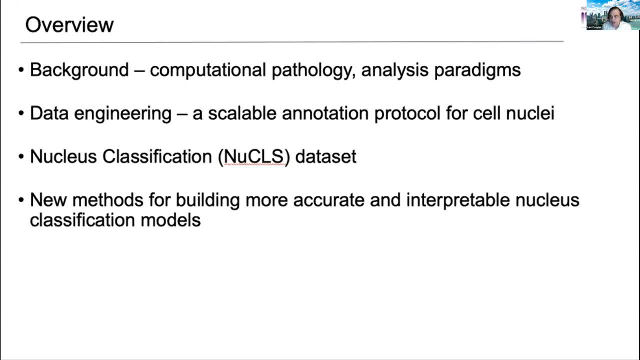 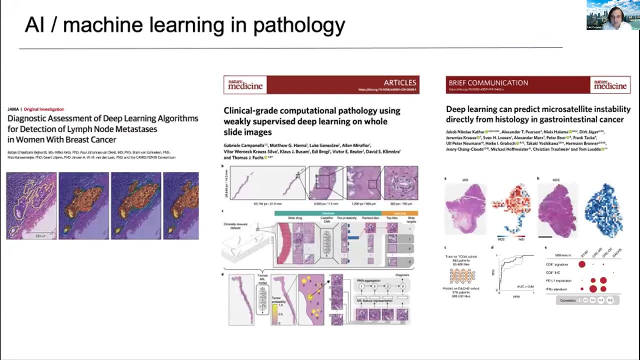 and the capabilities of some of these commodity: deep learning models that are used for things like object detection or classification. how do we really make those more specific and function better for pathology? so, um, you know there's been a lot of success. i think you know when i first started. 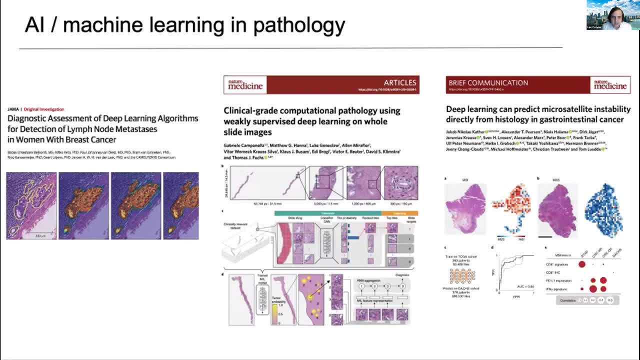 messing around with this stuff. it was just kind of a toy or a novelty, but, you know, starting around, you know, 2013, 2014, there's starting to be some really interesting results. uh, and applying, you know, deep learning algorithms to medical images and pathology in particular. so, uh, you know, there was a study that showed that. you know, using this data. 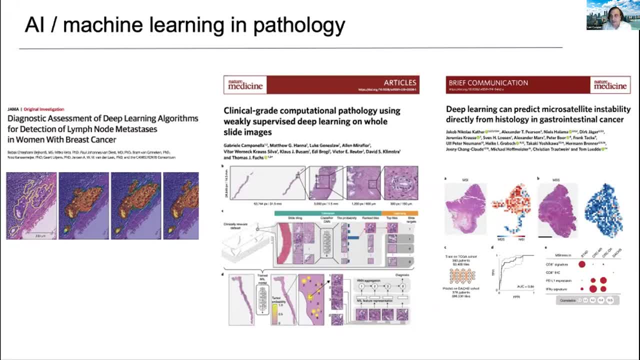 set called chameleon, that you know, deep learning algorithms can surpass humans, uh, in detecting metastases and breast cancers. uh, in lymph node sections, uh, when you, when you put time constraints on the humans. so you know, in practice and clinical practice, time constraints are in reality and so you know that was, i think, a big moment in our field to realize that we could. 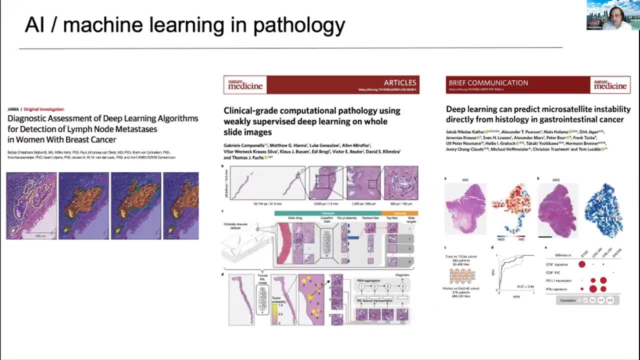 you know, achieve similar performance to humans and and perhaps even, uh, you know, exceed their performance. um, you know, there's been. there are a couple companies- path ai and page ai- that each have, you know, over 100 million in seriously funding. uh, you know, it's really. 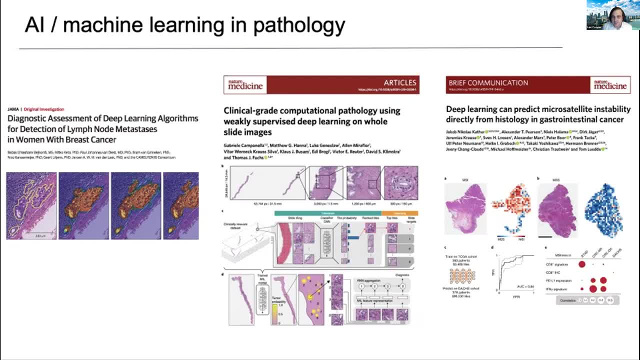 tremendous accomplishment. uh, you know paige had published a really nice paper in nature medicine that showed that if you get um these large data sets, where you have these massive images and you have like patient level labels about whether someone has a cancer diagnosis, you can really train without using any kind of annotation and develop really powerful diagnostic systems. 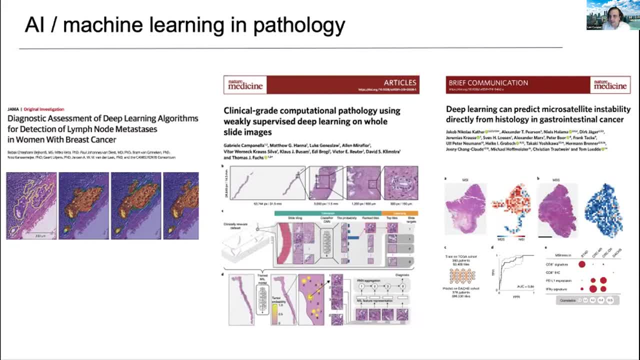 and there's also work that looks at predicting things like mutation status from histology. it's not extremely accurate. it's not definitely not going to replace sequencing, which is getting cheaper and cheaper, um, but it's an interesting result and it could be used for sort of screening. 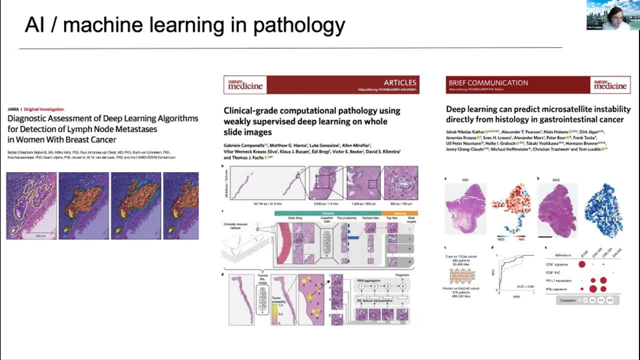 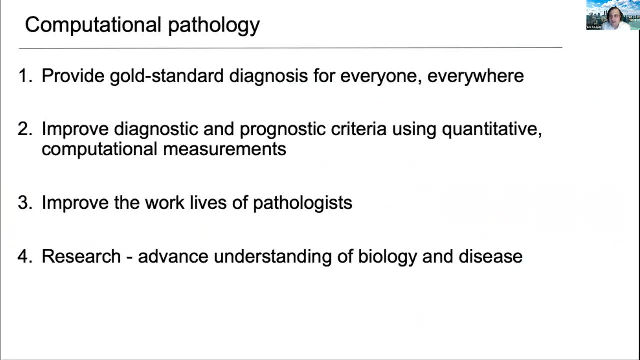 for eligibility for, you know, applying some of these assays, um, so, you know, computational pathology, what's really the potential? i think you know the most exciting thing is that we could take sort of the expertise of the best pathologists in the world and, uh, you know, in few. 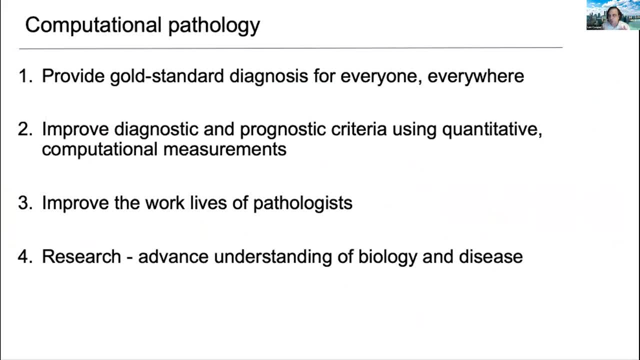 areas of the world and, you know, use that expertise into these algorithms and then make that quality of diagnosis available to everybody, whether they're in, you know, rural ohio or illinois, or in our major cities where they go to the james or where they go to our cancer center. 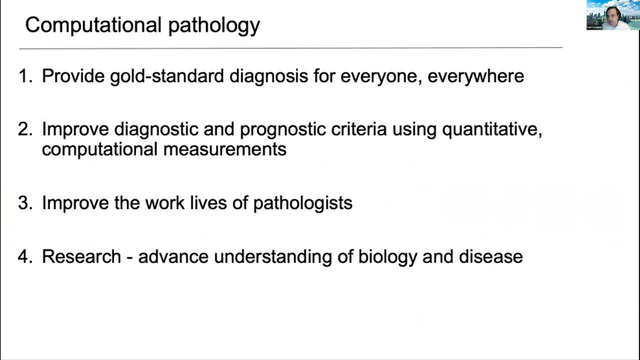 or you know out in lower and middle income countries. you know we can package this expertise up in algorithms and then disseminate it out to the world, and i think that would really be a tremendous accomplishment. you know specialization and experience matters when it comes to diagnosis. that is a limited resource and not available everywhere, so let's try to, you know, make that. 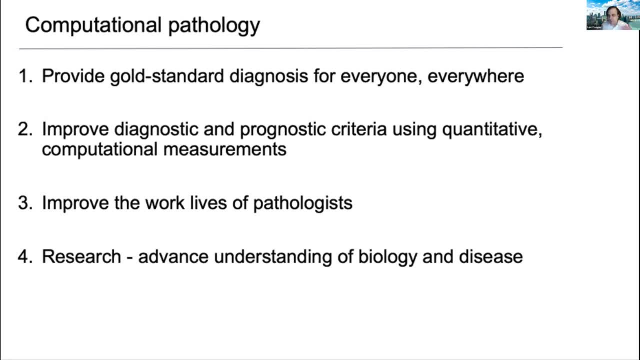 available. um, you know all of the rules that pathologists use uh to diagnose diseases. they're sort of uh done through, you know, studies, but they're, you know, subjective and kind of empirical, and so what we could do is to use algorithms to generate, you know, quantitative measurements from 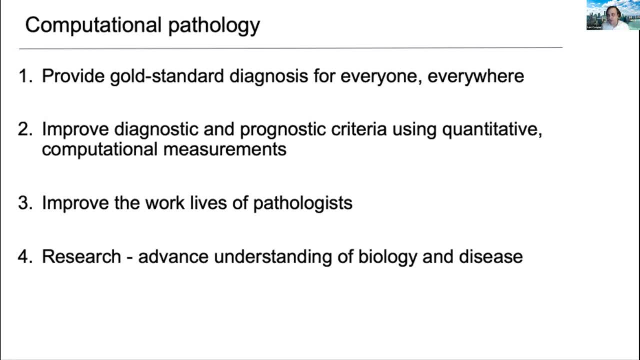 histology and then use those measurements to inform these diagnostic criteria. so i think that's another big opportunity, uh, improving the work lives of pathologists. they're really, you know, mostly overwhelmed. um, you know, i think there's a big decline in the number of pathologists that are training in the united. 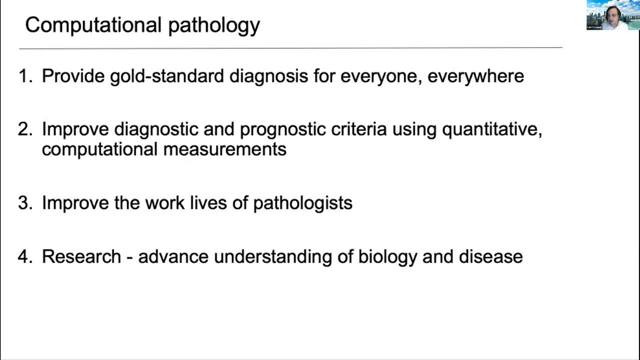 states, but there's increasing demand, uh, due to, you know, cancer incidents and aging population, etc. and so it'd be really great to be able to provide them with some tools that allow them to- uh, you know, handle a larger volume of cases and sort of, you know, ignore the easy things and focus. 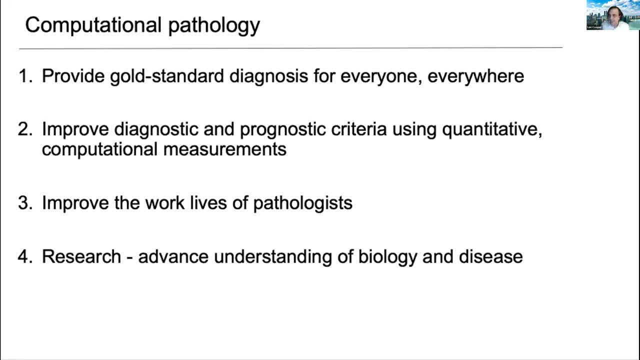 on the more interesting or more challenging cases. and then, finally, i think you know, a big opportunity is not in diagnosis, but in how we could use these tools to like characterize tissues, sort of like omics, but with images, and make that really a research resource, where it's a commodity that people can use and that could really advance. 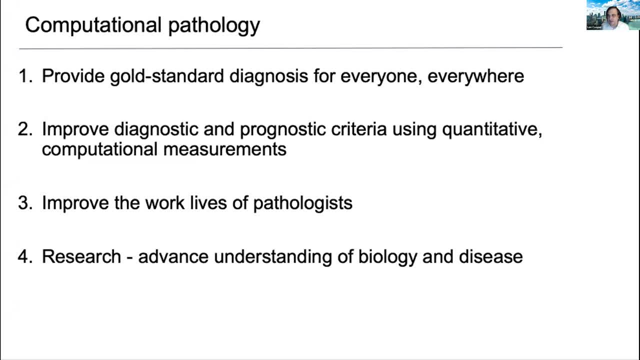 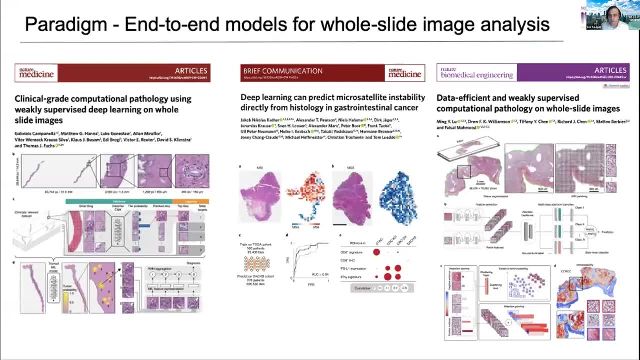 our understanding of biology and disease, and so that's a big motivation for the type of approach i'm going to discuss today. so, uh, one of the paradigms is, uh, what we would call, you know, end-to-end models for whole slide image analysis. so this is like a slide that i'm going to show you. 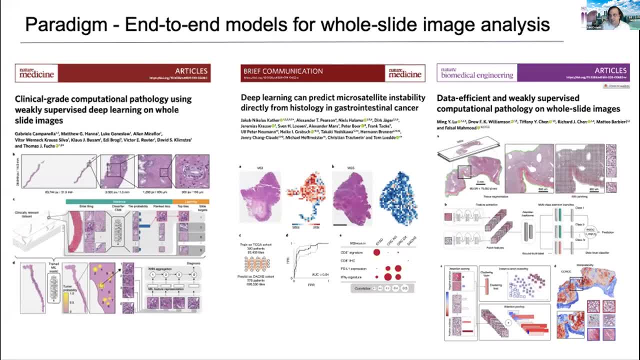 here. uh, this is like the two papers i mentioned before, where you have kind of slide level labels like cancer diagnosis yes or no, or mutation status, and then you know, you consume these massive images and learn and make some predictions. uh, you know, by consuming, you know billions of 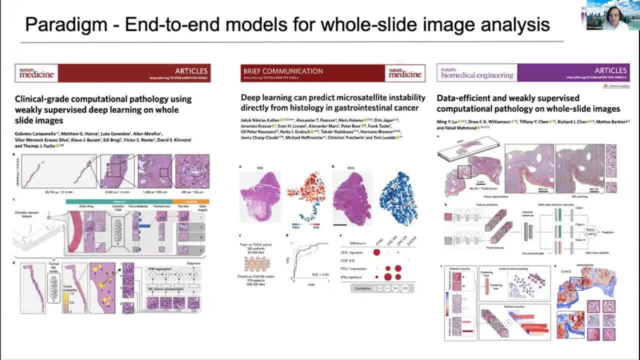 pixels for each sample. these are really powerful models. it's really exciting. it's it's kind of like really follows the deep learning paradigm of like raw data in and predictions out. it's just like pure machine learning and i think you know it's a really powerful approach. 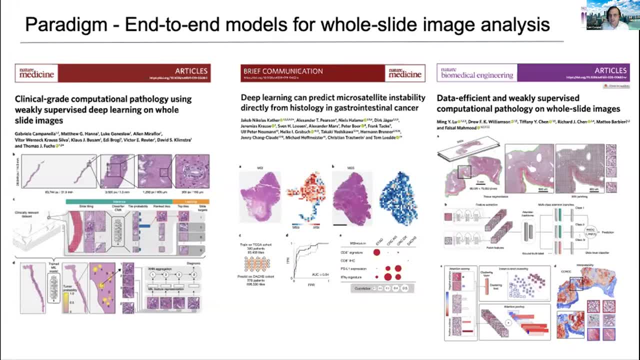 But there are really some, I think, challenges to using these types of techniques in some diagnostic applications and definitely in research. So, you know, if you're doing cancer diagnosis, it may be okay to have these types of models that are black boxes, right. 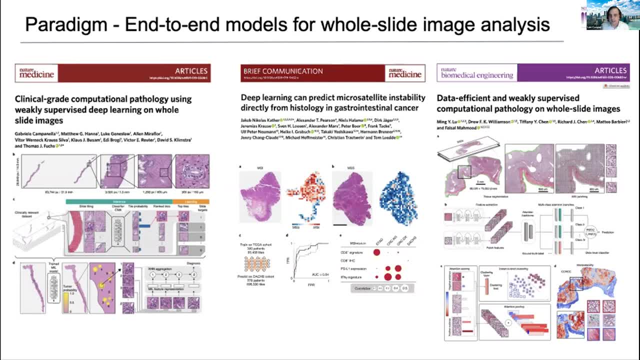 You know a model that looks at a prostate biopsy and just highlights the regions of cancer and tells the doctor to look at those areas. that's fine. You don't really need to interpret those models. But there are some cases where interpretability, you know, might be necessary or you might. 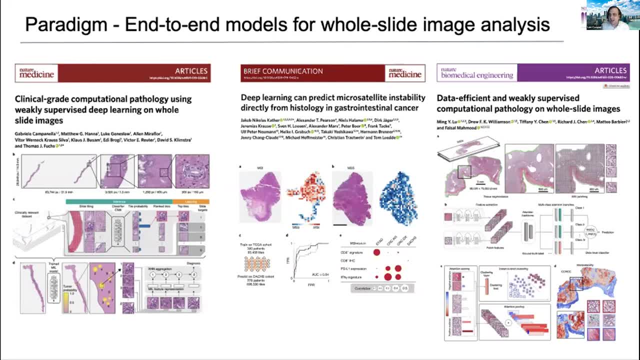 need a different approach, And so a lot of people have applied sort of interpretability methods in these whole slide imaging approaches. They're really post hoc And so there are challenges with doing that kind of post hoc interpretability. The first thing is falsifiability. 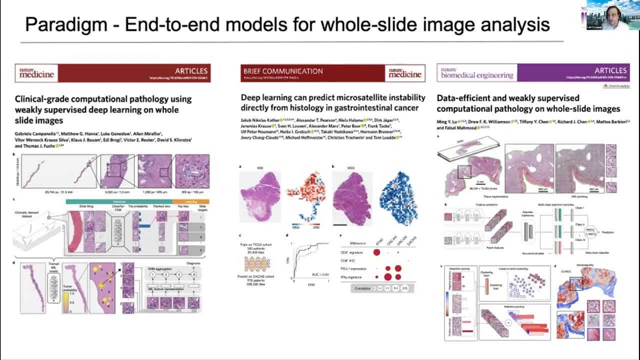 So if you have like a heat map of an algorithm and where it's looking, you can't really prove that wrong in any sense, And you know you can always. It's kind of like horoscopes: Whatever interpretability research you do, you can always come up with some interesting. 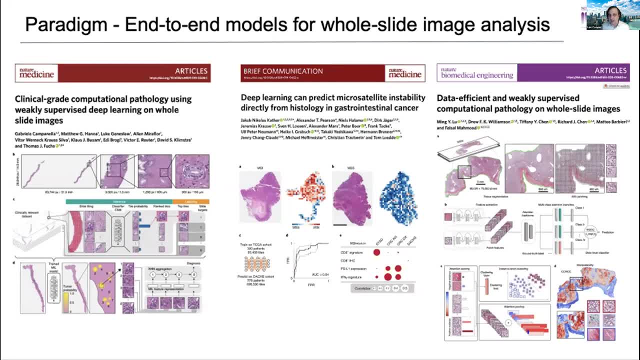 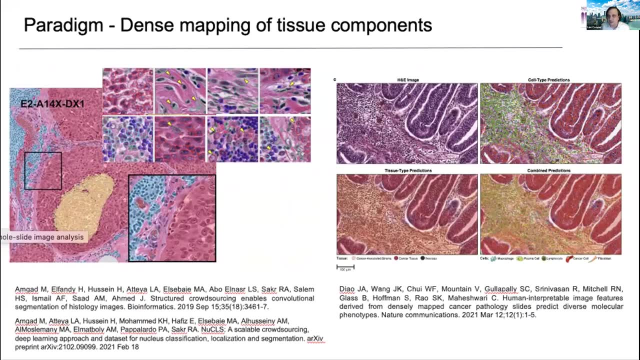 pattern that it's found, But you know, it's still essentially a black box, So an alternative approach is something called dense mapping, And so this term is from a paper that came out in March from the Path AI group, where it's in Nature Communications, where they generated all these annotations. 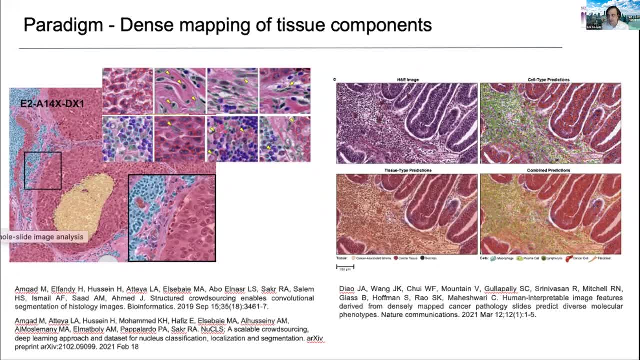 And what they do is essentially map all of the tissue structures and cells you know, classified, And so they're able to define them and segmenting them. you know with, you know terms and class labels that pathologists understand and appreciate. 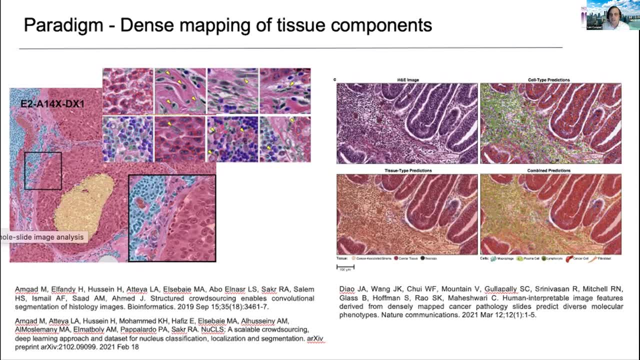 And so this is really kind of driven by like annotation of images, And you know, we have similar work that we've published. you know, back in 2019, we released a data set of breast cancer segmentation where we show, you know, if you have. 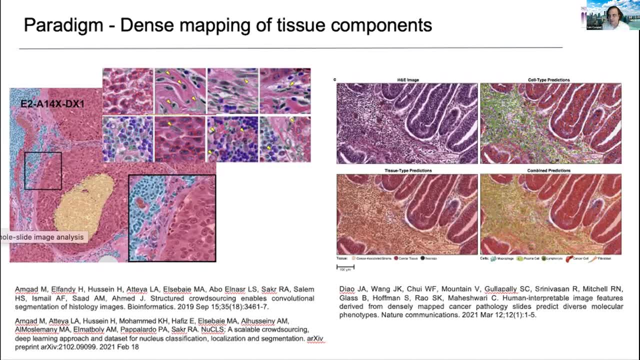 Get people together and trace, you know, breast cancer tissue regions. you can use kind of commodity models for semantic segmentation and get really high accuracy. And a paper we released more recently on archive just this year, looking at the same problem but with nuclei. 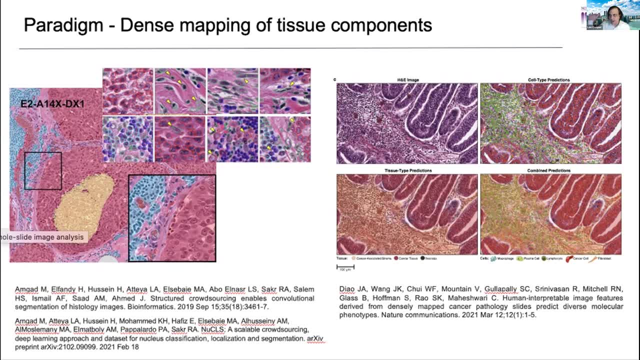 And so this dense mapping is a different paradigm. It's really kind of more like bottom up. So we use the deep learning algorithms to really accurately detect, classify and segment. But we're starting from a point where you know we're working with concepts and things that have semantic meaning that you know the pathologists already work with and are familiar with. 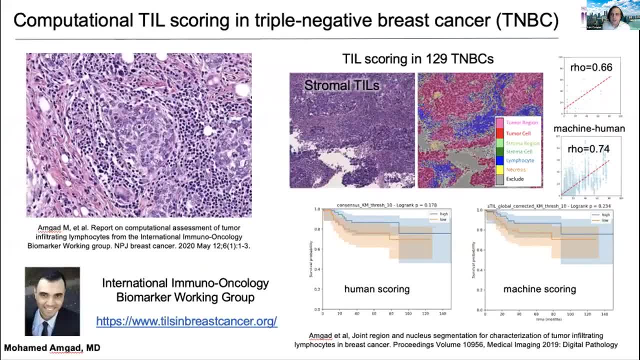 And so it's less of a black box. So you know an example of that And you know a couple of the types of things you can do with this. We work with this International Immuno-Oncology Biomarker Working Group. 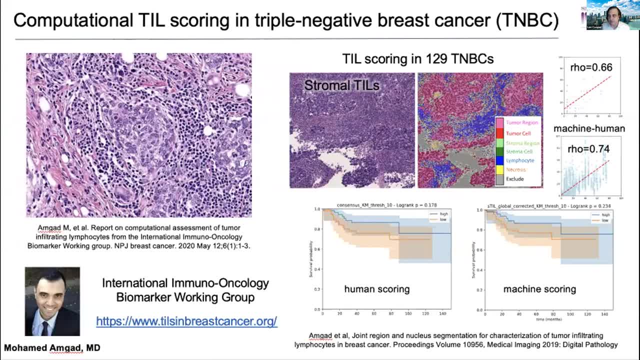 And what they do is they come up with rules for scoring immune infiltrates in breast cancer. So if you look at solid tumors and you look at the immune cells- and there are for many solid tumors- you know the type and the quantity and abundance of immune cells. 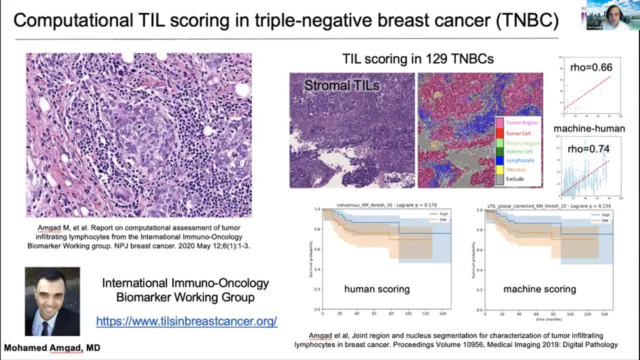 Is predictive of outcome, independent of other things. And so you know, you can take these sort of rules that humans have developed and you can encode them into quantitative systems using this kind of dense mapping approach. And so our student, Muhammad Amgad, who's done a lot, 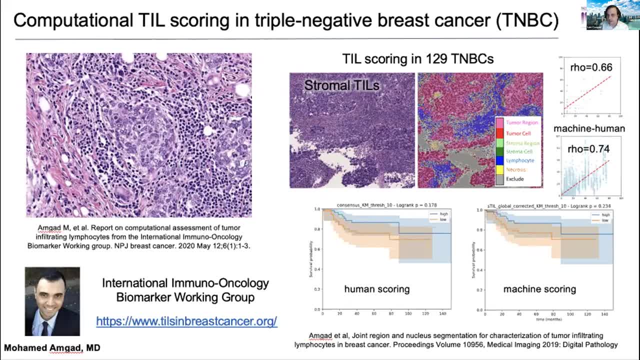 of the work that I'll show you today- has done some work with this immuno-oncology working group, but also looking at you know how do we build these algorithms and score things like, you know, immune infiltrates in breast cancer? and just showing that you can really make this. 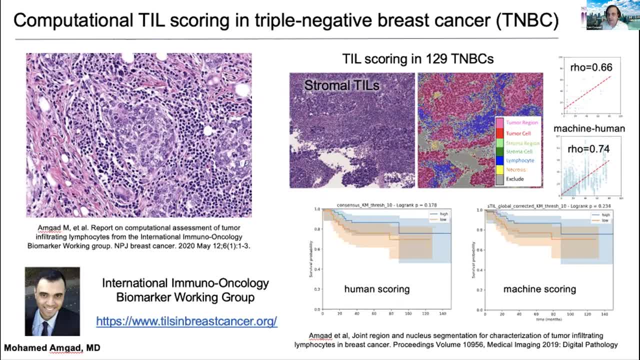 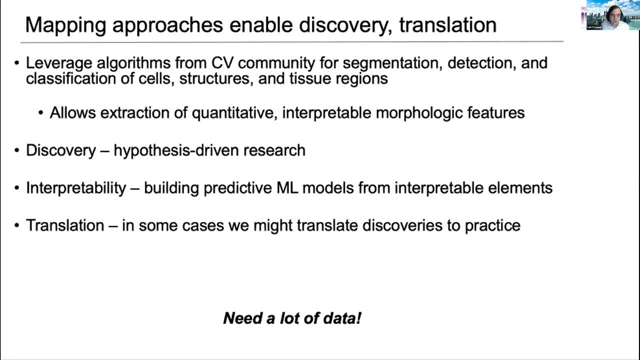 highly reproducible And you can do this in a way that you know is consistent with you know breast cancer experts scoring these same tissues. So you know these mapping approaches. I think the thing that's exciting about them is they enable 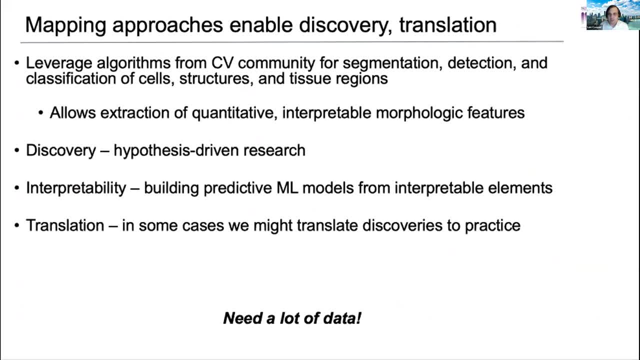 discovery and translation. And so what we do is we generate all these annotations and then we just leverage algorithms from the computer vision community for segmentation, detection and classification. So you know, the algorithms that are out there work quite well. I'm really less. 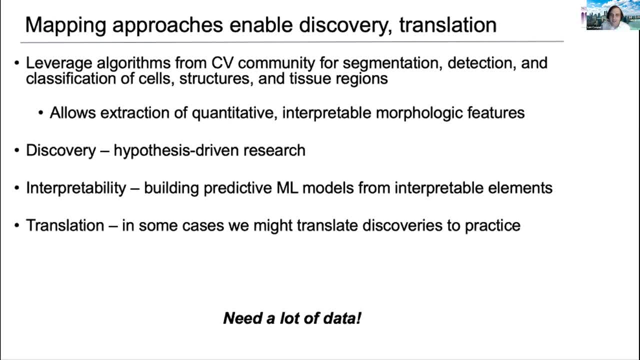 kind of interested in the algorithms. I'm more interested in how we produce the data, And if we're able to do that then we can do a lot of other things. So you know, we can generate these mappings of tissue structures and cells. then you can sort of come up with you. 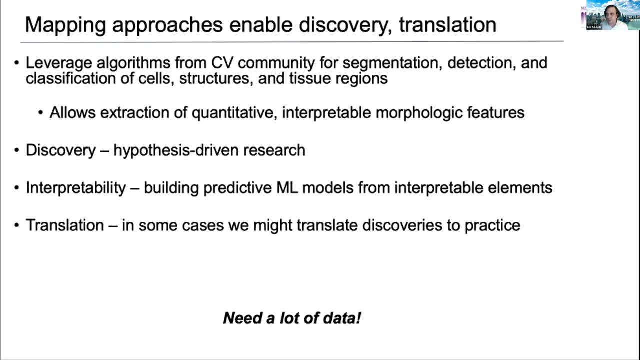 know quantitative but really interpretable measurements of tissue morphology, things that you know make sense to pathologists, and what that allows you to do is to sort of test specific hypotheses, and you can't really do that with the end-to-end deep learning models. so, for example, 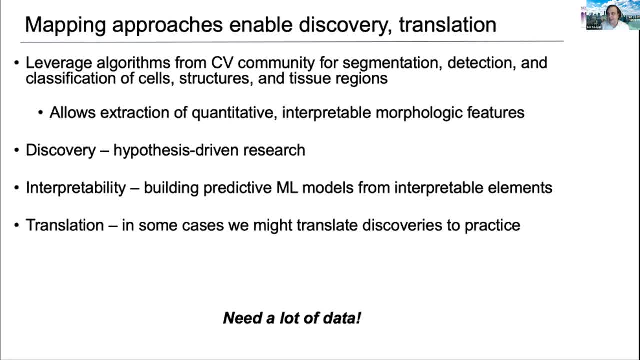 you could look at, like stromal cells and breast cancer, and look at their morphology and some of the patterns and look at relationships between, you know, genomic data or clinical outcomes and response to treatment. that's essentially, you know, impossible to do with these sort of end-to-end. 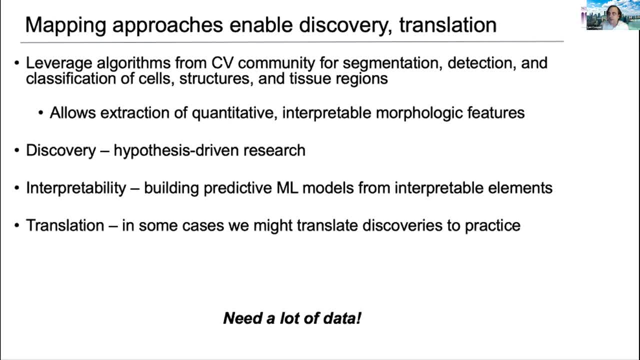 models. you know they don't. they don't really have any. you know notion of different cell types that are encoded in them, right? Of course, interpretability is important when we talk about, you know, clinical translation. I think some of the more immediate opportunities are to use these. 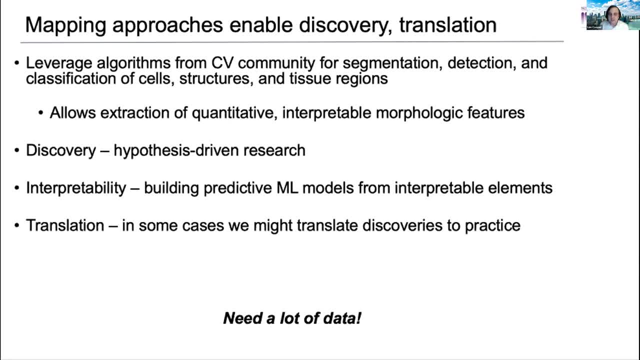 quantitative models and approaches for dense mapping to measure characteristics that pathologists can see and appreciate and to identify which new patterns you know still add predictive value to the current grading practices. and then we can take these and, you know, try to translate them back into clinical practice by teaching the people how to. 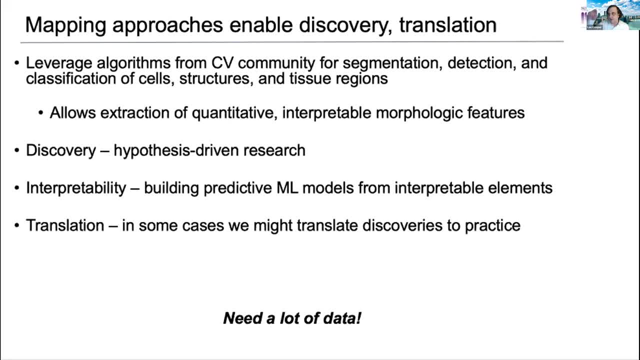 score these things. So you have, in that case, you know the the loop of the humans generating annotations to produce the algorithms and the algorithms being used to identify biomarkers and then translating those biomarkers back to the clinicians and teaching them how to do that. 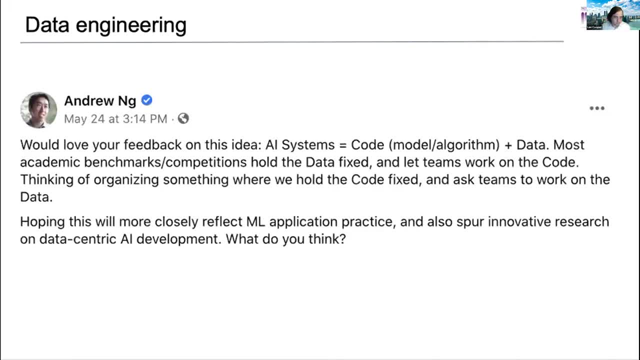 So I think it's really important to think about how to score those things. So this is a post from Andrew Eng recently that I was really glad to see. I think it kind of illustrates our idea about you know how this research should go. He's talking about how can we develop new. 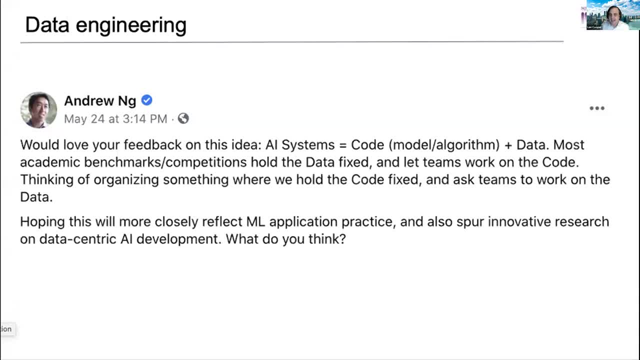 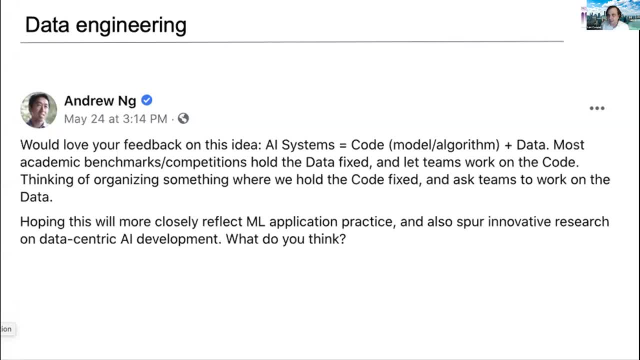 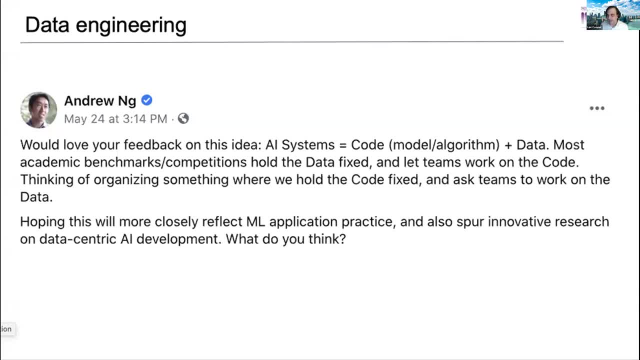 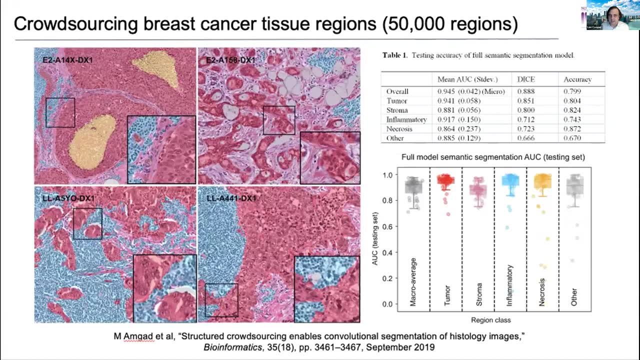 really aligns kind of with our academic mission, because we have the hospital and we have the experts here. Okay, So this is an example of what you can do if you can collect massive amounts of data. So this is a study we published in bioinformatics. It looks at crowdsourcing. 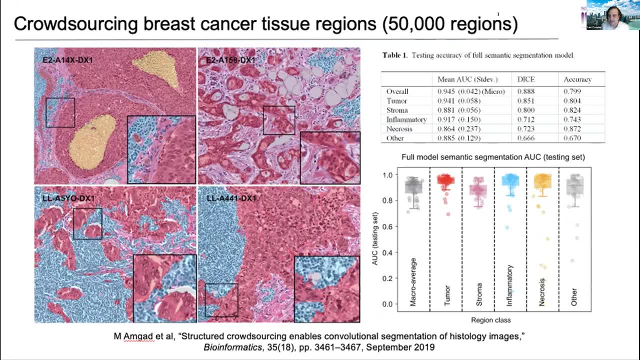 breast cancer tissue regions, And so we had people annotate 50,000 tissue regions. you know tracing essentially boundaries- I'll describe how we did that later. But what you can do, if you can generate this data, is to make extremely accurate computational models using things just like mask RCNN, just like regular semantic segmentation. 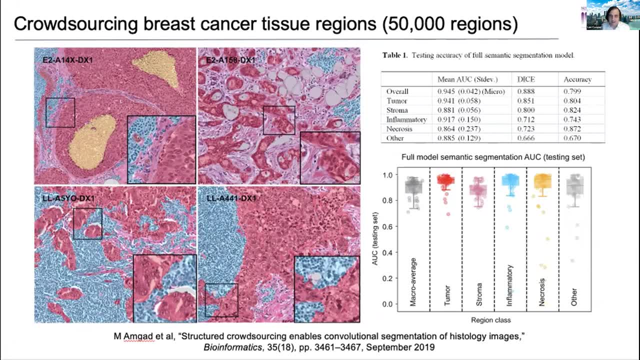 models. So what I'm showing you on the left here, these are actually segmentations generated from a computer. These are on cases from medical labs that were held out of the training set. So these are from labs that have not been seen by an algorithm before, And it's really pretty accurate. 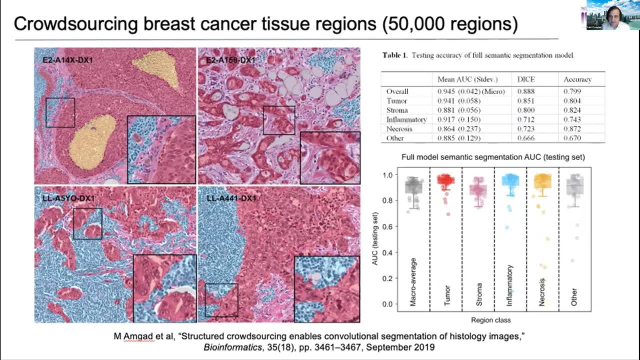 You know, if you look at this, it's sort of hard to tell whether this is done by a computer or a human being. The computer tends to be a little more detail-oriented and less kind of lazy than the people, And so that's maybe a little bit of a tell. 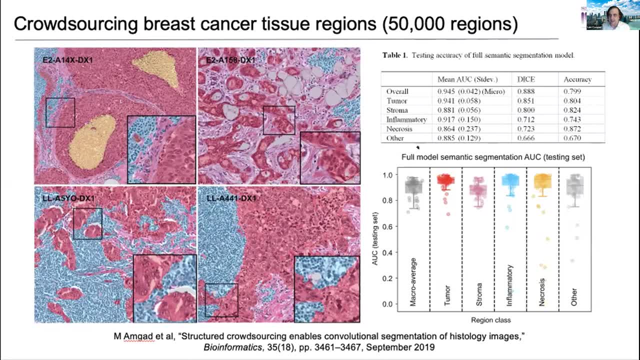 But we're getting you know extremely high accuracy from these algorithms, And the secret ingredient really is the data. It's not this specific approach or the network that we used, So I'm going to talk now about a protocol we developed for annotating cell nuclei. 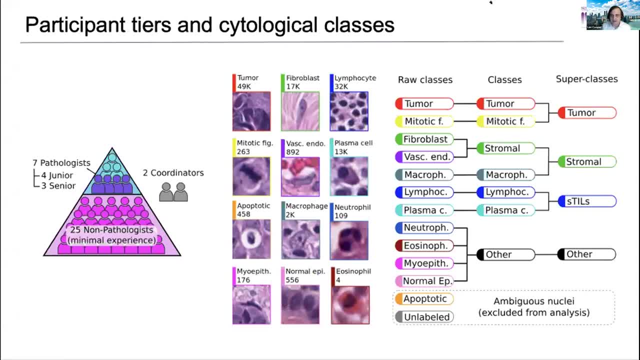 You know I won't bore you with like breast cancer biology, but I'm going to talk about a lot of different types of cell types you could be interested in. We looked at, you know, at least 12 cell types and did our annotations, And so these annotations were performed by a group of 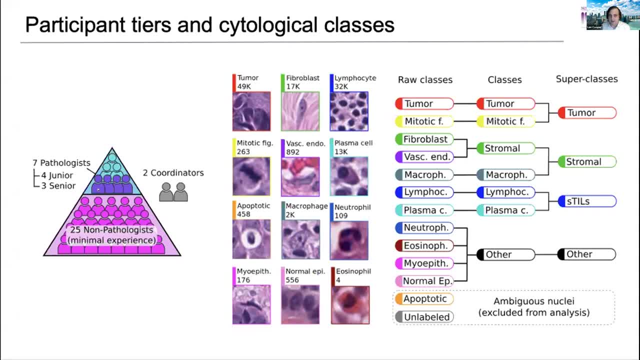 non-pathologists, so like medical students, And then we had pathology residents, pathology fellows and pathologists, And so they sort of worked together in this group, with the medical students doing the bulk of the work. Okay, So you know, we collected over 220,000 annotated cell nuclei. 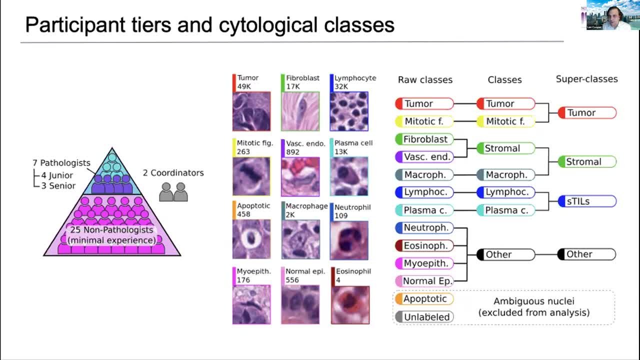 And then we defined these groups, So we have the raw classes that were annotated. This includes, like all, different kinds of cell types, some that are very uncommon, like these ASN fills, for example, And then when we're doing our analysis, we're essentially grouping these into 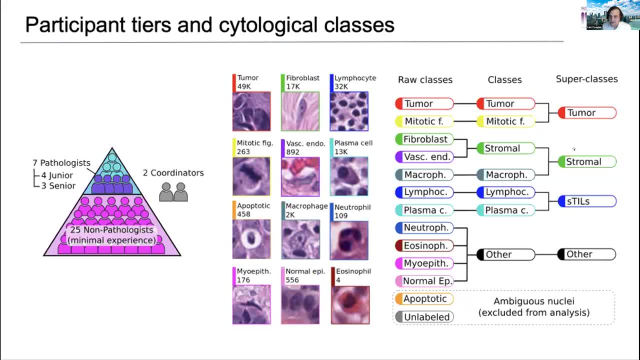 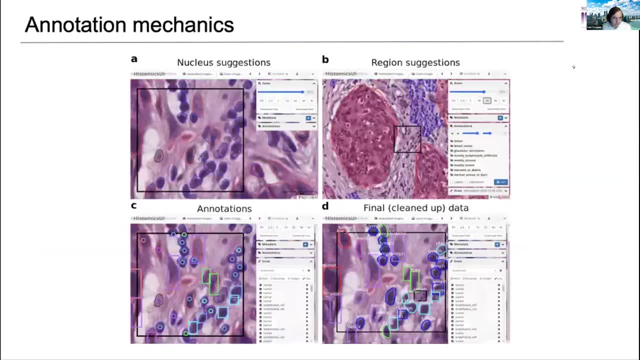 different classes. you know tumor cells, cells you find in the stroma, immune cells and other types of cells. So we call those things superclasses. So the mechanics of the annotation are that we have a weak algorithm that goes in and makes suggestions for the humans. So it's a very weak segmentation algorithm. 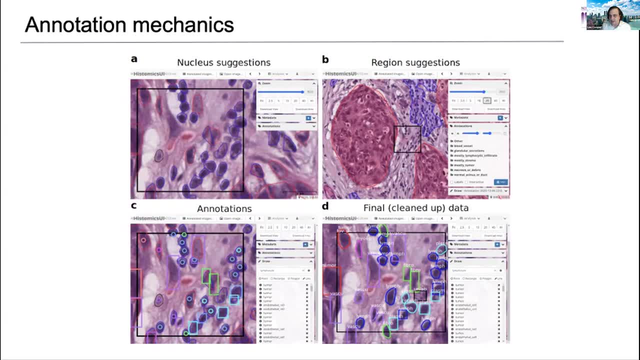 that just does a kind of a decent job, but not good enough at segmenting nuclei. It just uses basic image analysis like primitive operations, And then we use rules based on morphology to classify things into different cell types, And so that's just an example of what the human 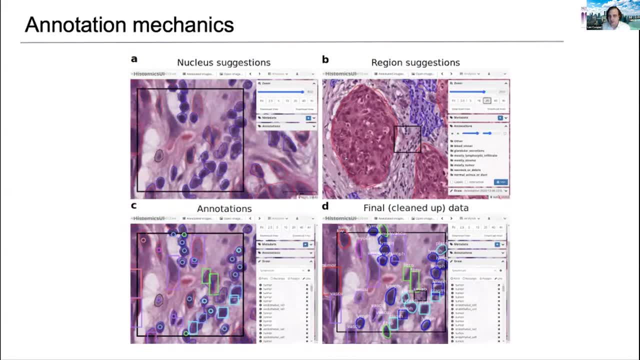 beings will see when they're doing their annotation work. We also provide suggestions from region annotations from our data set we developed previously. And then what the volunteers do is they're going to do a lot of work on the annotation, And so we're going to 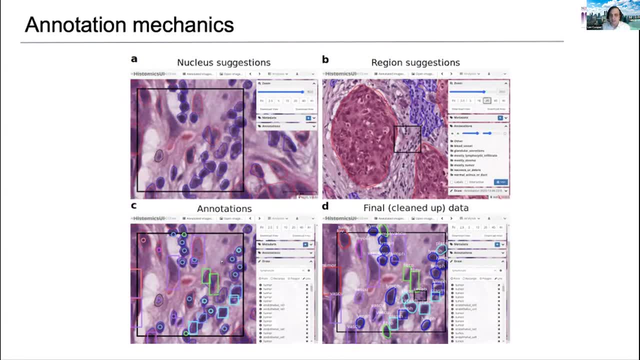 do a lot of work on the annotation, And so what the volunteers do is they go in and they confirm by clicking correctly segmented cells. So that just involves a single click for each of those cells. For cells that are missed or incorrectly segmented, what they'll do is they'll draw a bounding box. 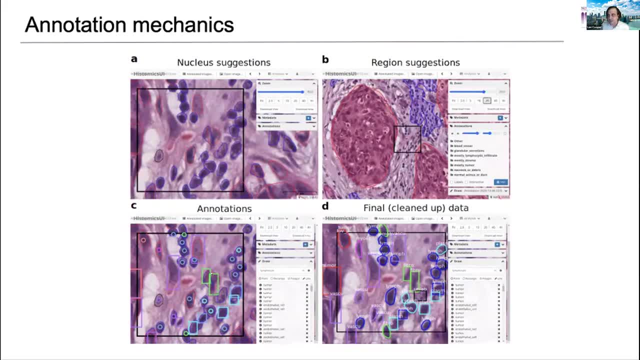 And so what this allows us to do is to collect a combination of segmentation data and bounding box data, which we call a hybrid data set, And it really relieves the annotator from having to actually trace individual cells, So we get that kind of segmentation data for free. 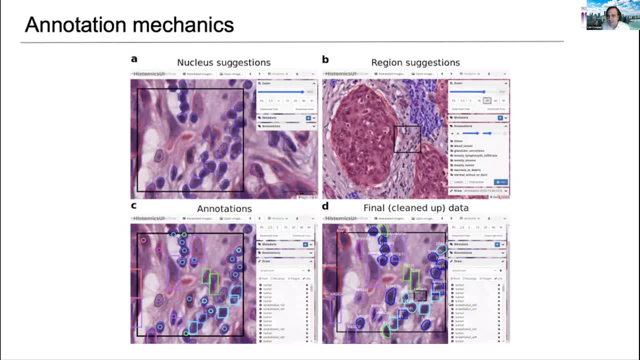 And then, once we clean up this data, we get rid of the bad segmentations and we have a mixture of, like I said, these good segmentations, polygons and bounding boxes. So one of the things that we did that I think was interesting was to use 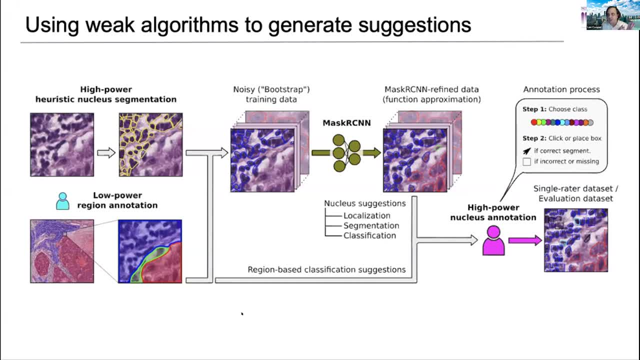 this mask R-CNN algorithm to take our weak segmentations that we use for suggestions and to improve the quality of them quite a bit, And so you can think of this as like fitting a line to noisy data. So we have all these noisy segmentations using just basic image. 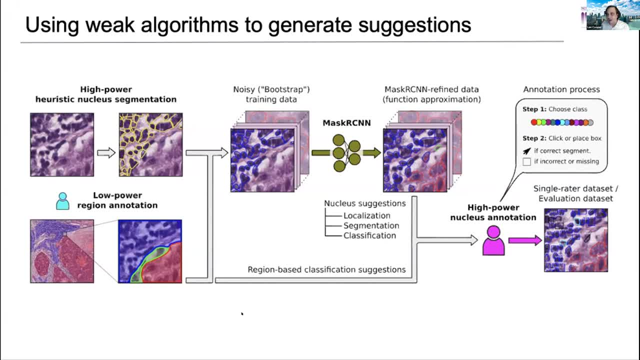 analysis operations And then we feed them into this deep learning model, which is essentially just like a curve fitting algorithm that operates as a function approximator, And just by doing that process it really tends to improve the quality of the suggestions we show people. So you can see. 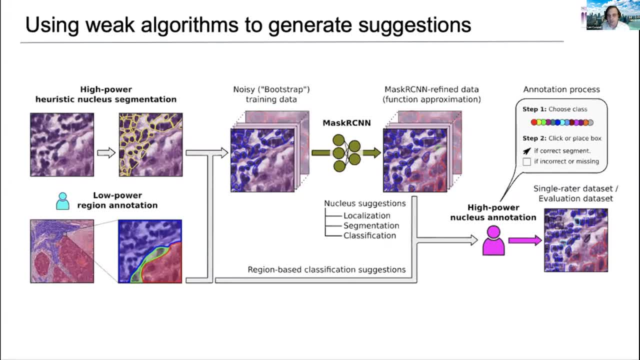 in the center. here we go from a bunch of segmentations that are missing these tumor cells in the lower right corner, And when we're switching over to the other side we're seeing a bunch of segmentations that are sort of missing these tumor cells in the lower right corner. And when we're sort of 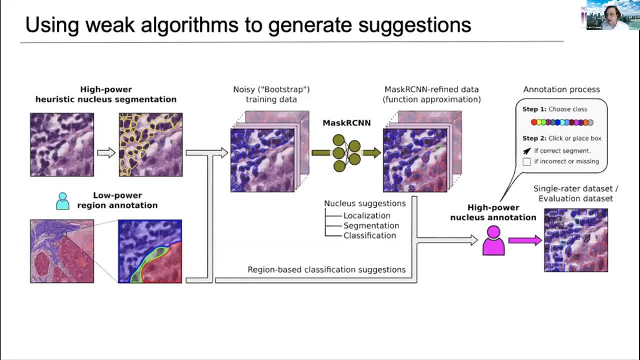 so we pass things through the mask R-CNN and train it and then use inference on the training data again, we get these nice tumor cells that show up and also this fibroblast that was missed. So this is something I haven't seen before. I think it's some novelty that we have, which is to 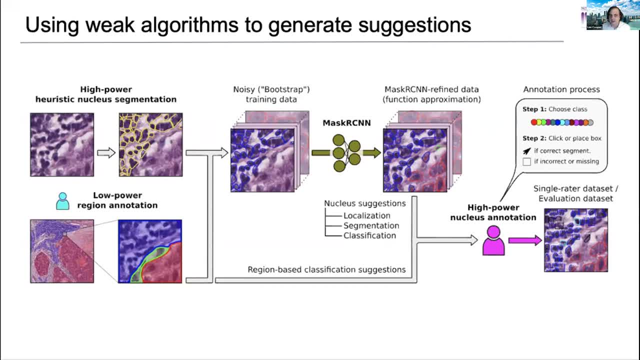 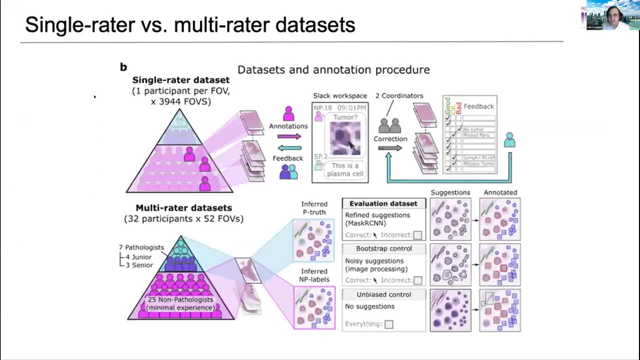 you know, sort of bootstrap our way into getting these kind of higher quality suggestions that we have. So we have two types of datasets. One is a single rater dataset. This is where we take a bunch of ROIs and we, you know, assign them out to. 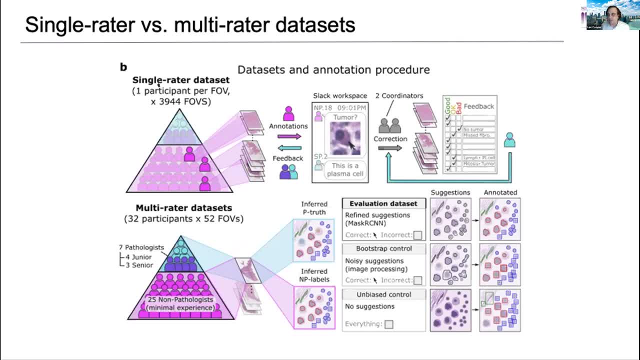 different annotators, And so the purpose of this is to generate breadth, So we have, like, the scale of data that we need. In this example, you know all of the people who are junior who are shown in pink here- they have a Slack workspace where they can ask questions for the residents and the 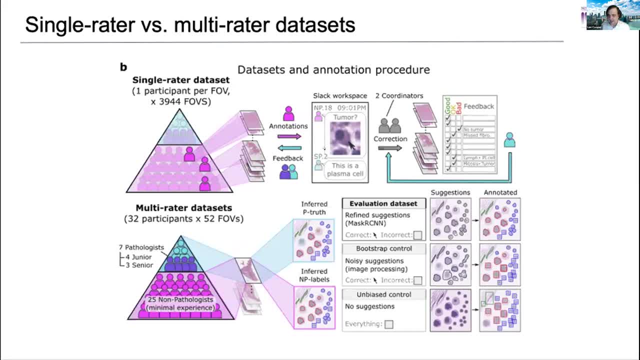 fellows and pathologists, and they get feedback And then at the end all their annotations undergo like a quality review before they get entered into the dataset. Then we have a multi-rater dataset which essentially is used for looking at inter-rater variability. 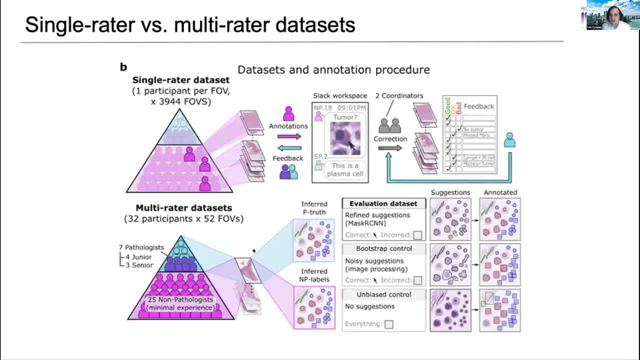 And so what we do in this multi-rater dataset is we show them different combinations of things. So we show them first of all this unbiased dataset where there are no suggestions. So we just get their- you know- bounding boxes on everything. We don't really bias them in any way. And there's a. 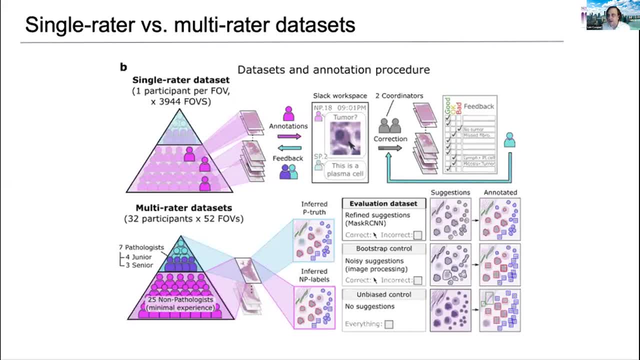 washout period and we show them the noisy segmentations that are the sort of the weak algorithm suggestions, and another washout, And then we show them the refined suggestions that are generated by MaskR-CNN. This sort of study design allows us to look at differences between people. 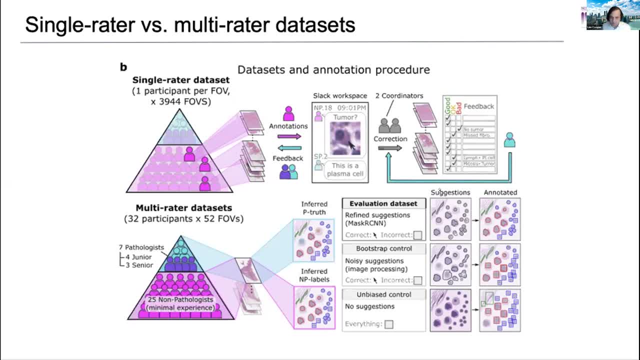 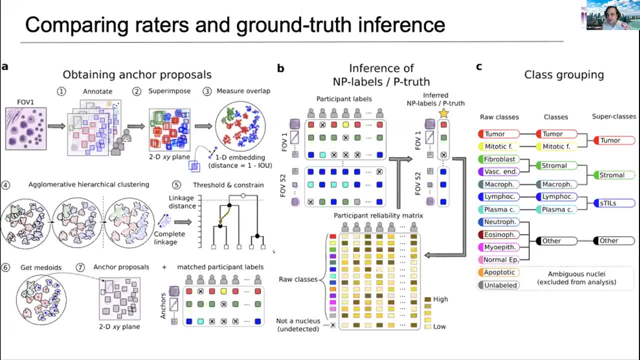 and also the impact of the suggestions on the annotators as well. So one of the challenges is when you're looking at inter-rater concordance. when you're talking about cell detection, you know it's much more challenging because you can't. 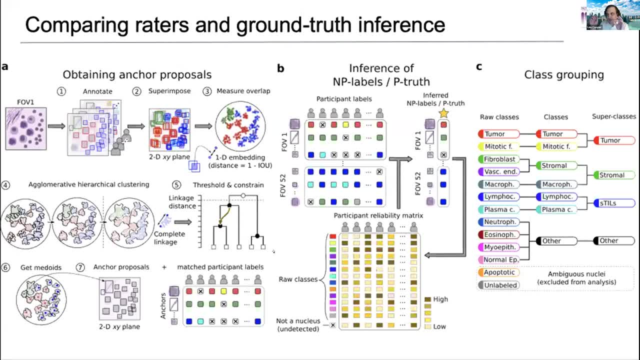 like compare pixel to pixel, like masks, You have to figure out correspondences between you know, different cells that have been annotated by different people in the same area, And so that required us to a new type of constrained clustering algorithm. I don't want to go into this. 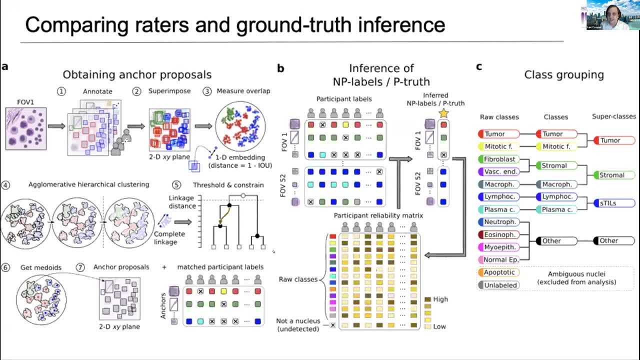 it's like a little too complex, but it just kind of illustrates the point about, you know, challenges in simple things like measuring inter-rater variability in pathology. So what we did was to create this clustering algorithm that allows us to essentially generate a type of ground truth from our pathologists. 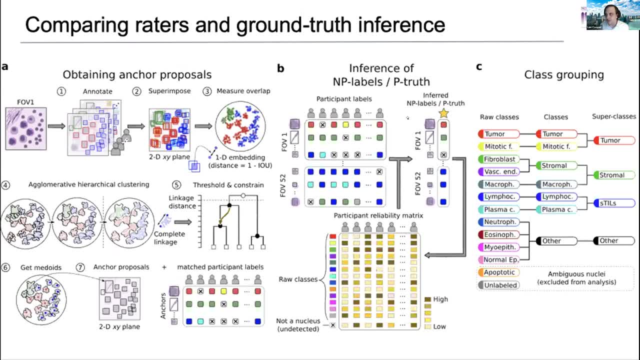 And we also use a EM algorithm to kind of estimate. you know, a single ground truth from pathologists that we can use to evaluate performance, And this essentially just like weights pathologists by class, to figure out who's good at what, who's more sensitive, for example, with tumor cells. 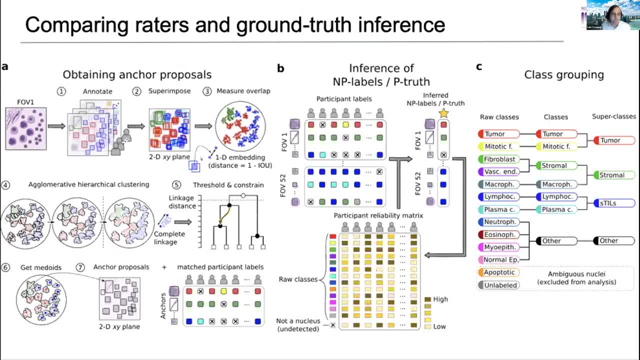 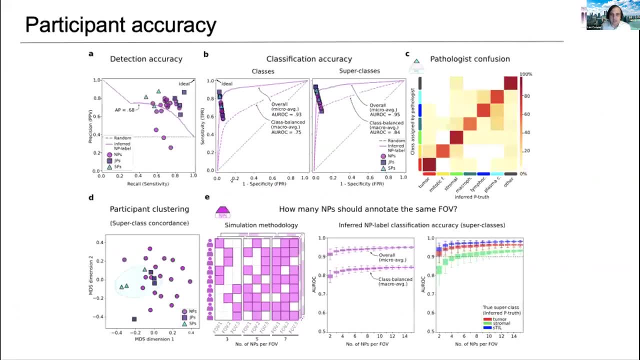 and who's more sensitive with stromal cells, or visa versa. Okay, let's talk about the dataset itself. So when we started looking at some of the statistics, there's some interesting patterns that emerge. The first thing we looked at is detection accuracy. 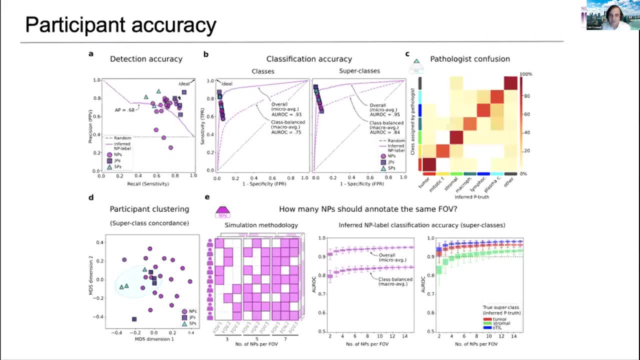 and you see, there's really like a range of precision and recall for detection accuracy. So we have a few people who are kind of outliers, who are just not really good, you know, annotators. but most people sort of fall along this curve of being like either having better recall, 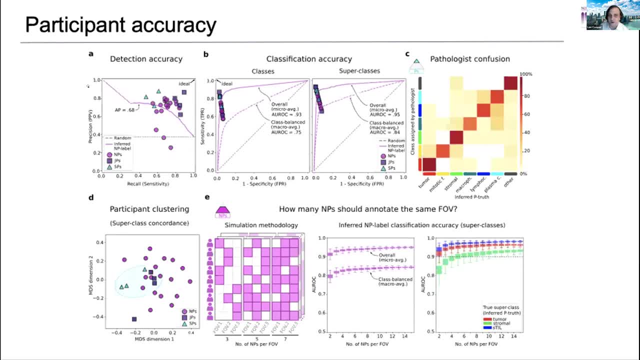 or better precision, which is what we typically see from algorithms or these types of inter-observer studies. One of the things that's interesting is that our junior pathologists tend to have a little bit better recall than the senior pathologists. One of the hypotheses we had in this case 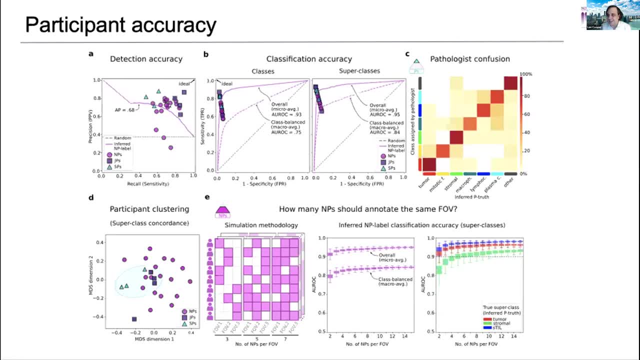 was that maybe they have more time to do this and so they tend to spend more time, you know, annotating and looking for missing cells, where you know maybe the senior pathologists just kind of go a little quicker and don't pick up on those things. 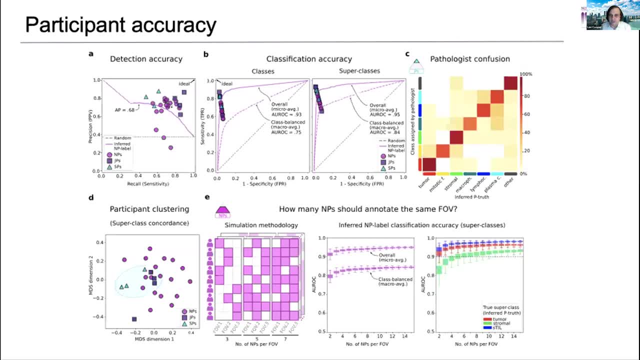 But we have, you know, pretty good, you know, I would say, for compared to our ground truth, we have pretty good accuracy for detection, For classification. it's pretty similar, You know, when we look at sort of the superclasses. 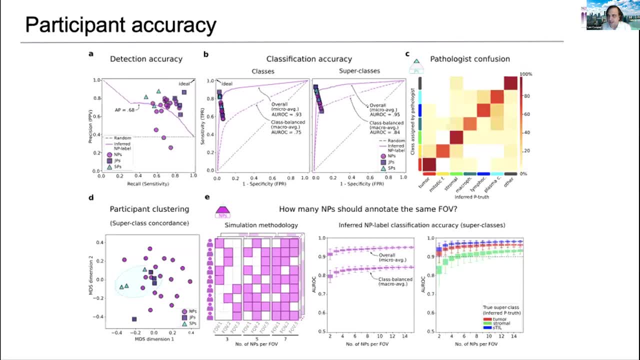 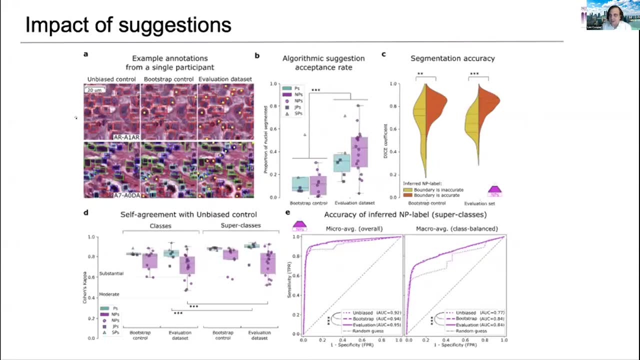 in our macro averages, you know, we get a pretty high AUC. Okay, One of the things we looked at then is the impact of these suggestions on people, And what you really want to do is to look at. you know, the suggestions essentially bias people in a negative way. 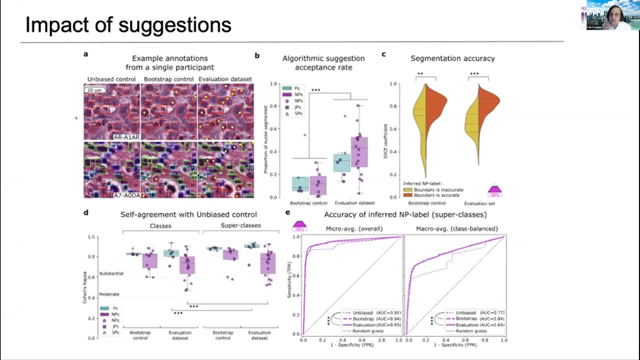 And the second question is: how much time are the suggestions saving? So one of the things we looked at is, you know, for this acceptance rate for the suggestions. how does it vary whether we're looking at our noisy bootstrap data versus our evaluation data set? 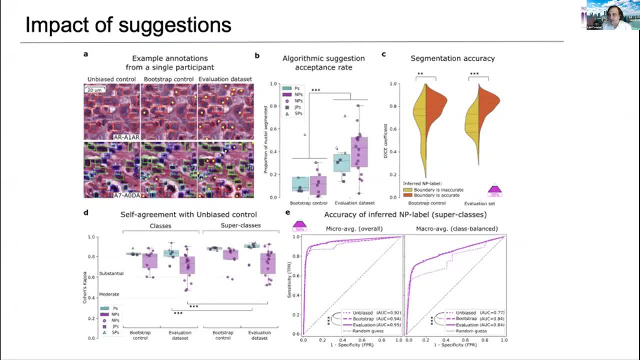 And so quantitatively we can see that as we go through this MASK-R-CNN refinement, people are clicking more of that segmentations because they like them better and they're more higher quality, And you can also see that in the figure on the left. 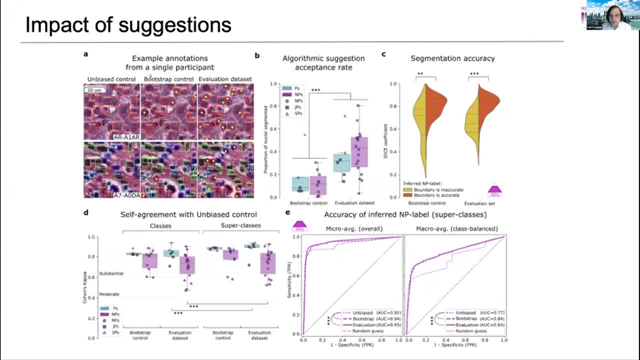 over on figure A. if you compare the middle column of figures versus the right column, you can see that on this refined data set, where we've applied MASK-R-CNN, you get like a lot more clicks, And so that's essentially saves people time. 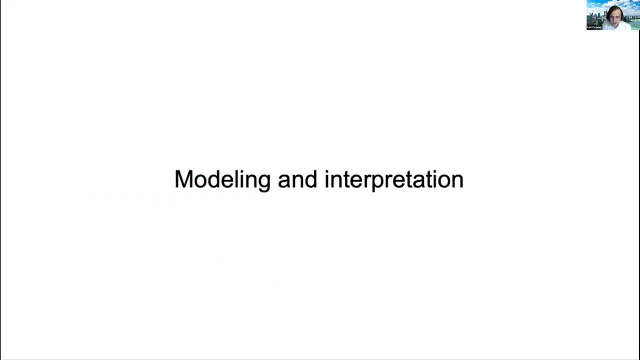 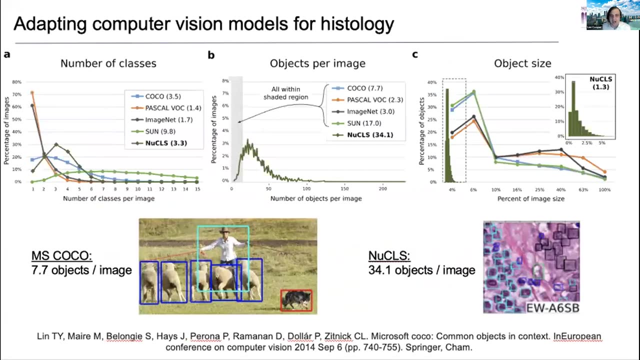 Okay, So let me skip ahead here. So let's talk about the modeling and interpretation component. So we have this data set with 220,000 annotated nuclei. The next step is to figure out: okay, how do we model this and generate algorithms from this? 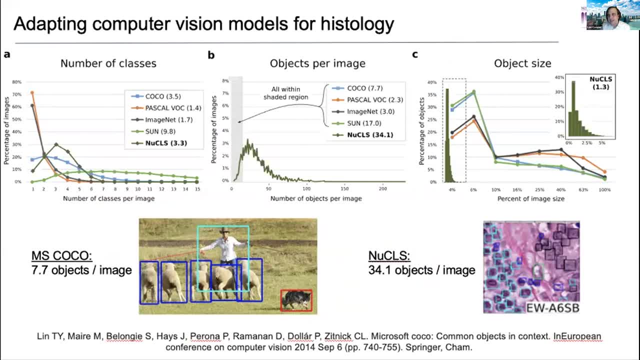 And one of the first things we looked at is like kind of the differences between these nuclei data sets and data sets like COCO that are used to develop like faster R-CNN and all these detection algorithms, And there are really some differences in the statistics. 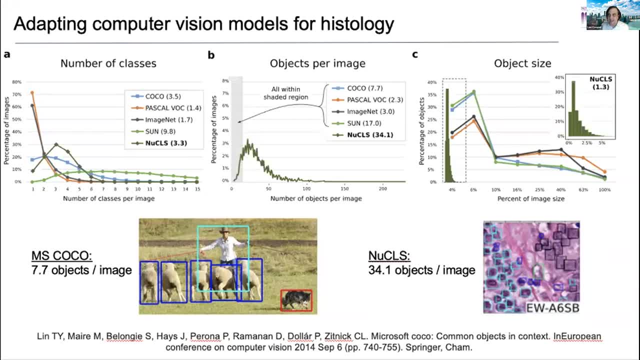 like in terms of the size of the objects which is going to impact, like network design and kernel size, but also the number of objects that you find in a single image. So if you look at MS COCO, it's got you know. 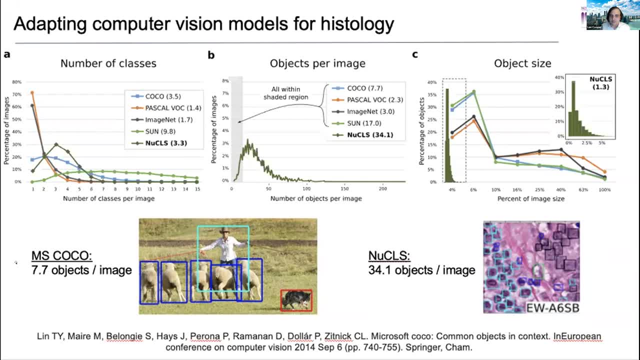 pictures of natural scenery and stuff like that. You see roughly 7.7 objects per image. That's kind of the average in COCO. And then I think the average size of one of these objects is like: it takes up roughly like 10% of the image. 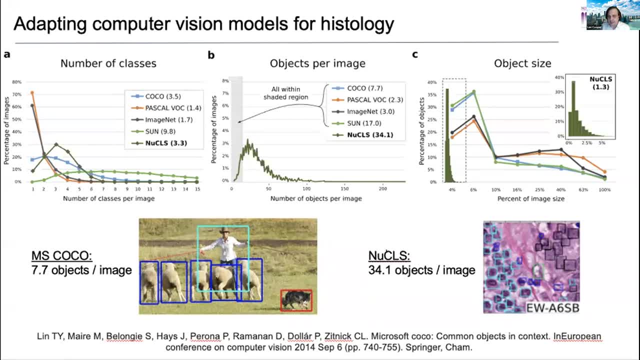 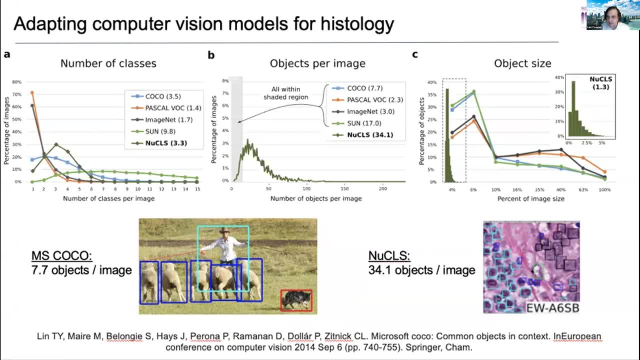 So that's a lot of data, And the average, I think, size of something in the image is like 1% or less, So the objects are smaller, They're more numerous, And that should really, I think, inform the algorithm design. 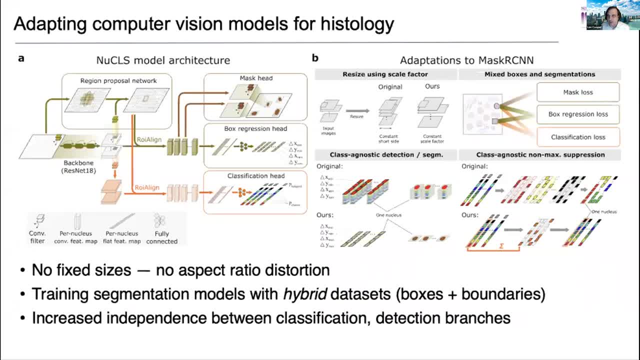 So we did take this mass R-CNN algorithm and then adapted it with these things in mind. One of the things that we looked at is making sure that we can handle variable sizes of images without resizing everything to the same aspect ratio. to the same aspect ratio. 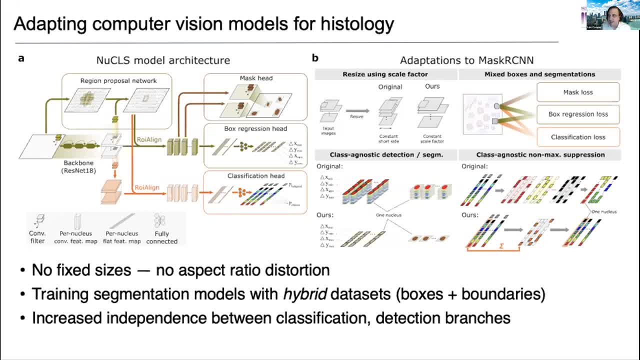 Or, I'm sorry, to the same fixed size. This really helps with avoiding distortions of the image content and your aspect ratios, which is a bad thing. Another thing this model allows us to do is to look at training with hybrid data sets. 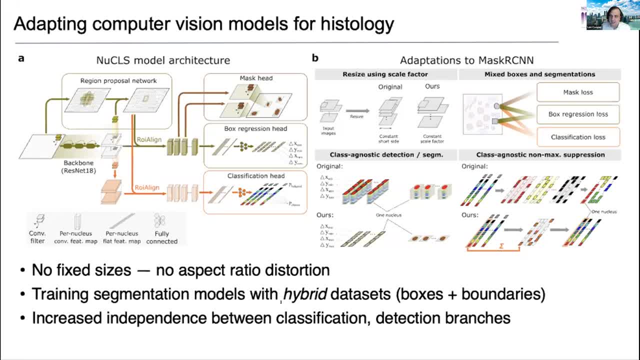 so a combination of bounding boxes and boundaries. That's, I think, a first thing that we've seen. So normally you either have to work with bounding boxes or with boundaries, and you can't really combine both of them. So this network combines both and it kind of does it. 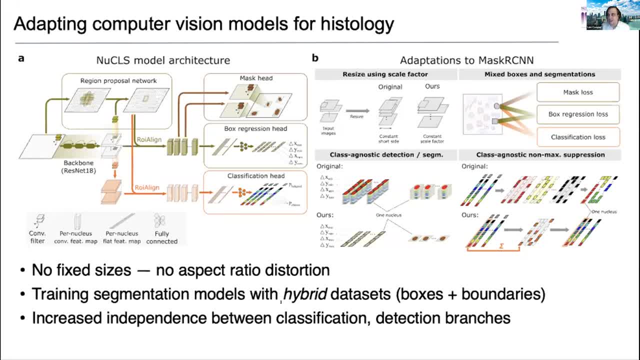 through this masking process. So we don't train the segmentation loss if we have a bounding box, If we have a segmentation instead of a bounding box, then we train that loss. So another thing we did is to increase the independence between the classification and detection. 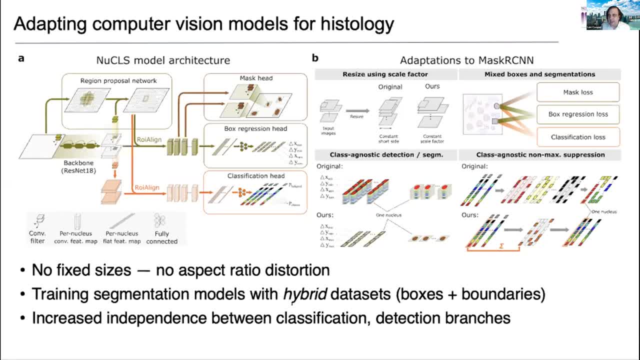 branches. This doesn't really help with performance, but I think it really helps with freedom in designing the algorithm And it gives you more flexibility and allows you to develop an algorithm that works faster And that makes the tuning much, much easier. So here are some results from our algorithm. 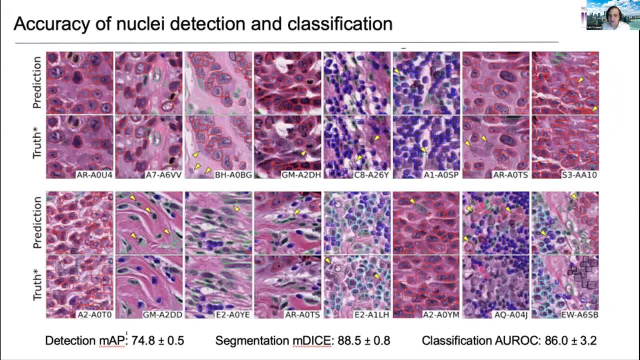 So overall our median average precision was 75.. That's pretty good Segmentation dice for the nuclei it's 88.5.. That's pretty high for dice. I mean it's not like some of the things you see in the tumor segmentation. 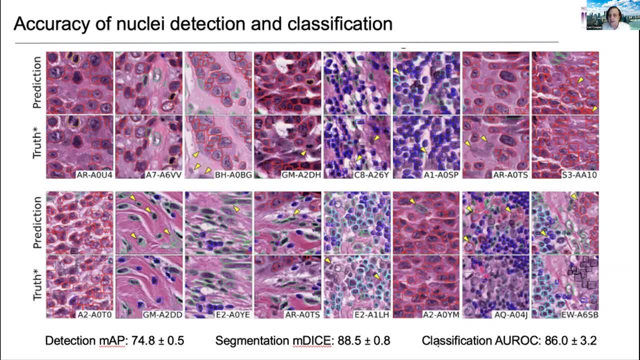 studies for radiology, But I think it's pretty good for pathology. And our classification, our OC was 86.. So one of the things to note is I'm showing sort of two rows of results here. On the top of one of these rows is the prediction. 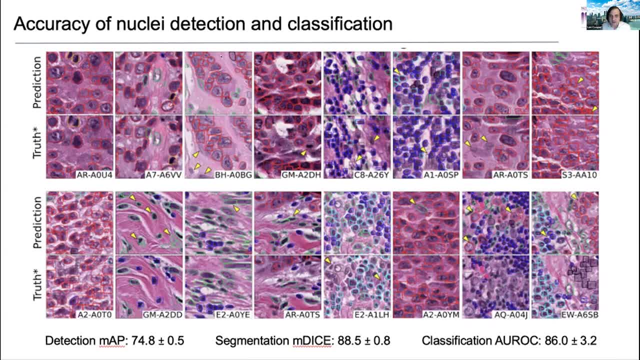 And then on the bottom is the ground truth, And one of the interesting things is that where the algorithm and the human disagree, the algorithm is not always wrong. So there are a lot of cases where we see the algorithm will pick something out And then that doesn't exist in the ground truth. 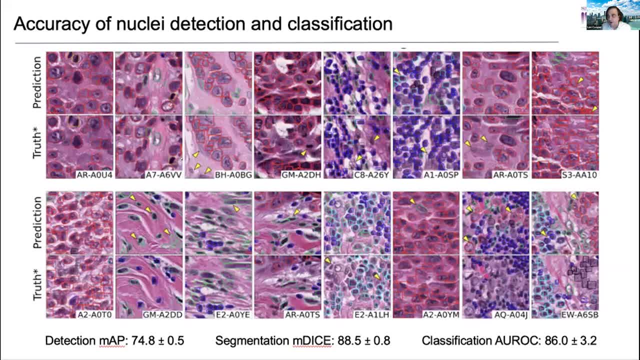 But finally, This one is % française, or I, and so you'll see, it'll be called a false positive, for example. So right here, for example, you have these stromal cells that have been detected by our algorithm. Those were missed. 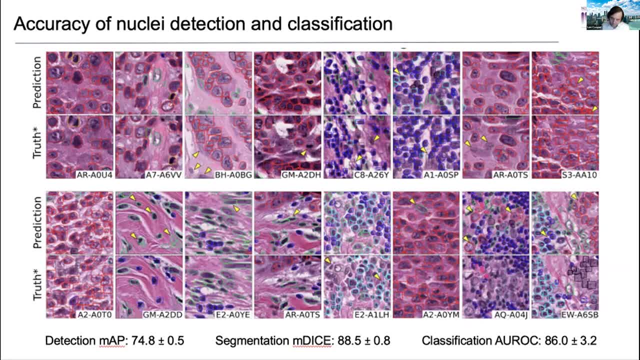 by our human annotators. They just weren't annotated for some reason. So this sort of just points out, I think, the kind of fuzziness, and like evaluating the performance of algorithms in this area: No matter how hard you work to collect ground truth, there's going to be imperfections. 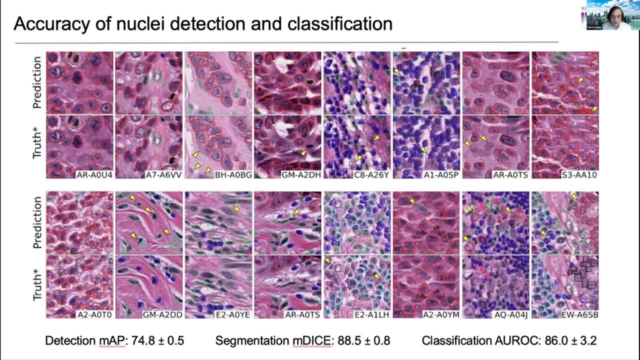 and errors in it, So there's always just some kind of gray area. But overall we were satisfied with the performance of these And I'll note we made just minor changes to this mask RCNN algorithm. This is not like a cutting edge segmentation algorithm, It's just sort of what. 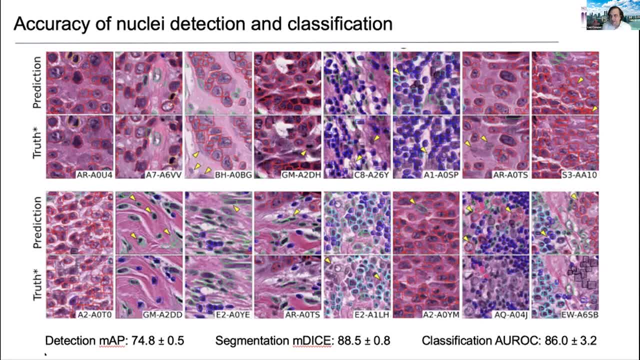 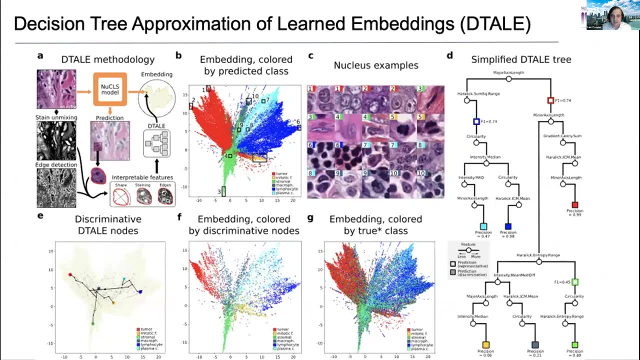 everyone's using. I think the key to getting this kind of performance is really just like having a large, large amount of training data on a bunch of different hospitals, right, Okay? So the next piece that we worked on was like: if we have a like, for example, a nuclear classification algorithm, 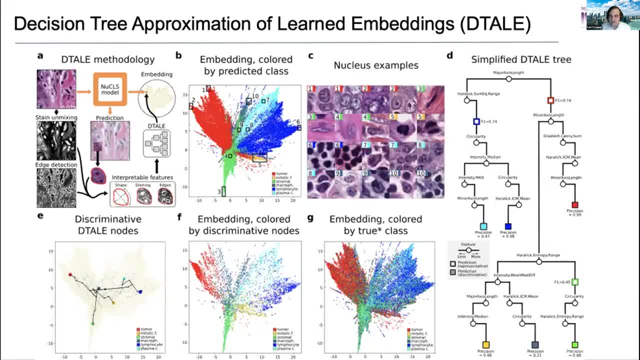 how can we develop a process that will allow us to take this black box algorithm and understand some of the rationale behind its predictions? So what we came up with was this idea of generating a companion algorithm. So we have this classification algorithm and we have a 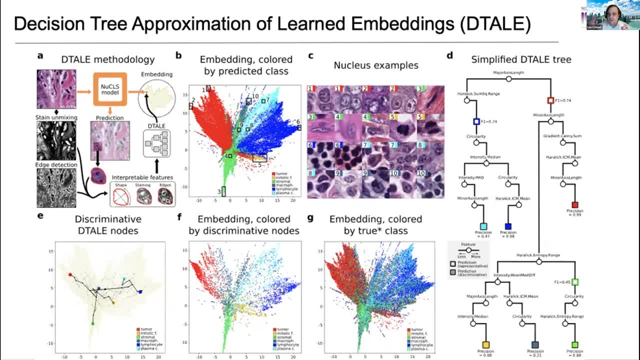 companion algorithm that is not deep learning based, it's tree based And it sort of models the behavior of the deep learning algorithm. So we have this classification algorithm and we have a multi- deuxième mixture. So we might want to build on this decision tree algorithm including all of 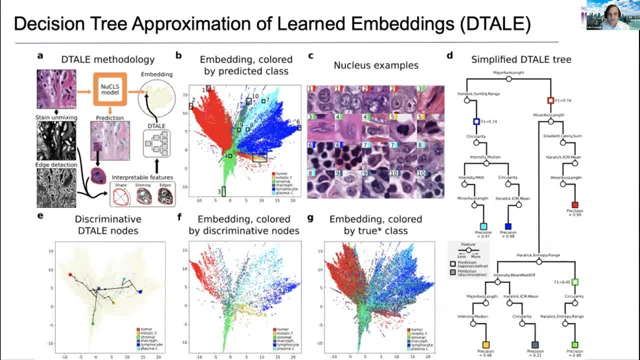 its imperfections, And so the way that we did this was: we have our segmentation data. From our segmentations we can calculate all kinds of morphologic features like texture, shape and size, And then we use those to train this decision tree algorithm to approximate the performance of. 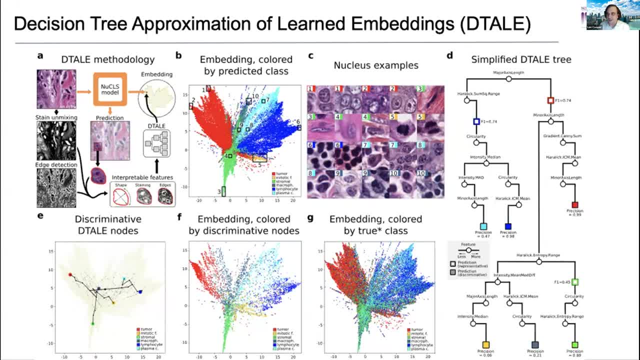 the deep learning classification algorithm, And then what that gives us is this tree that has all kinds of decisions based on morphologic features that we understand, And so that allows us to, short of like, try to understand what types of morphologic cues this deep learning algorithm is using for. 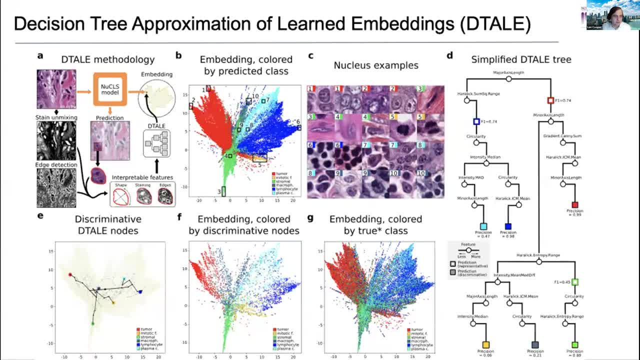 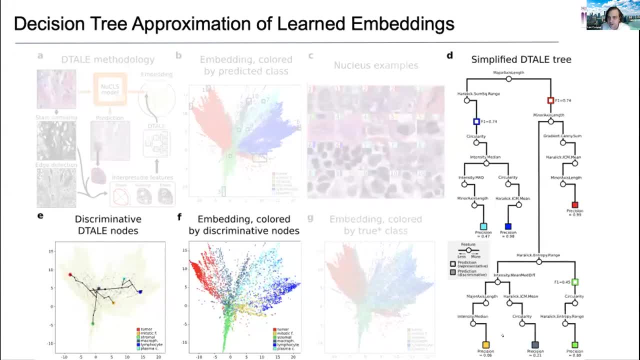 classification. So I'll just skip ahead here and show you this example. So we created this decision tree And then at each point in the split you see a feature that's used in making a decision between different types of nuclei. So at the top level split, we have the difference. 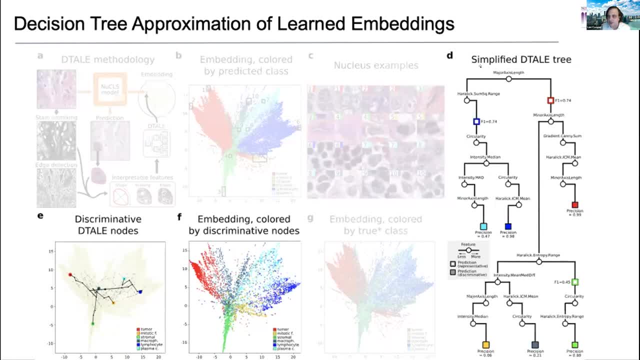 between immune cells and tumor cells And what's being used there by the algorithm. the primary determinant is major axis length. So if you have a long major axis length, you're more likely to be a tumor cell or a stromal cell. If you have a short axis length, you're more like a major axis. 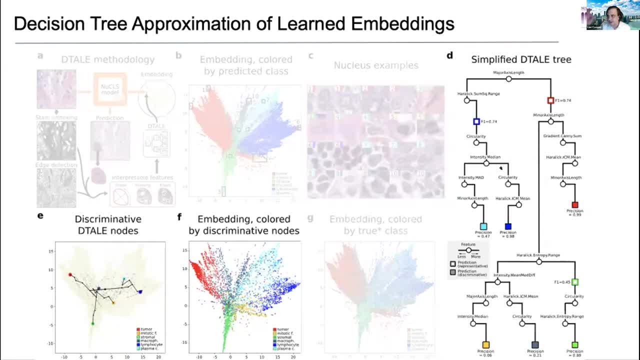 length you're more likely to be an immune cell, And that's true. Immune cells are kind of like small and round. So if you go down the left side of the branch the difference between, say, plasma cells and lymphocytes is really kind of based on the intensity. 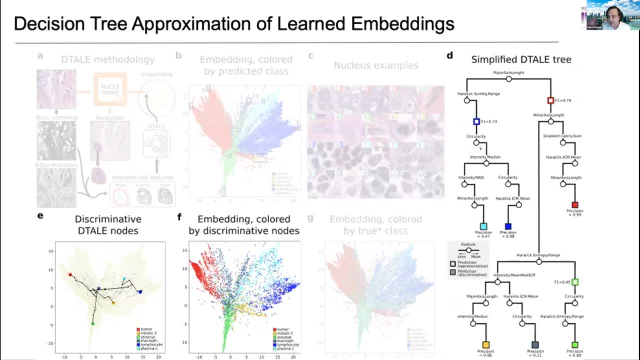 of the staining, And so plasma cells have kind of like a lighter and rougher texture. The lymphocytes are really small and dark, And so we see that. you know, we see that pattern here reflected in this tree. If you go down the right branch of this tree, what you see is that you 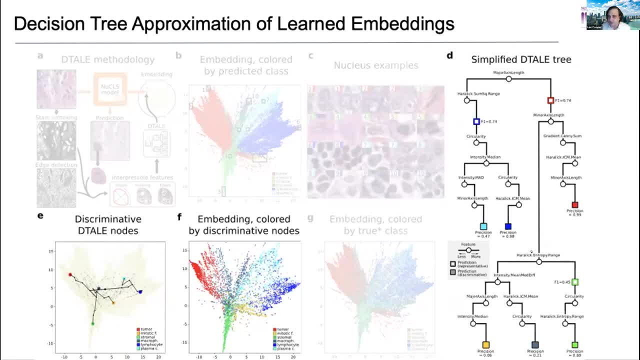 know, some of the other differences in terms of determining tumor versus strom are the minor axis length, So tumor cells tend to be like just kind of large and you know, oblong, where these fibroblasts and stromal cells will tend to be. like you know, like you know, like you know. 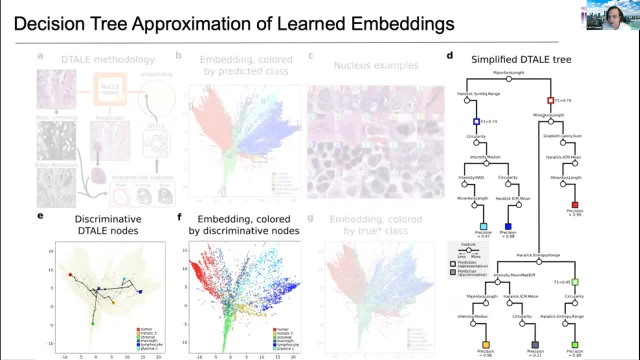 really kind of more spindle-like, And so the minor axis length is really what's being used to distinguish tumor cells versus stromal cells. So this type of approach, I think it can be used with any kind of unsupervised or- I'm sorry, supervised- learning And it just lets you sort of model a. 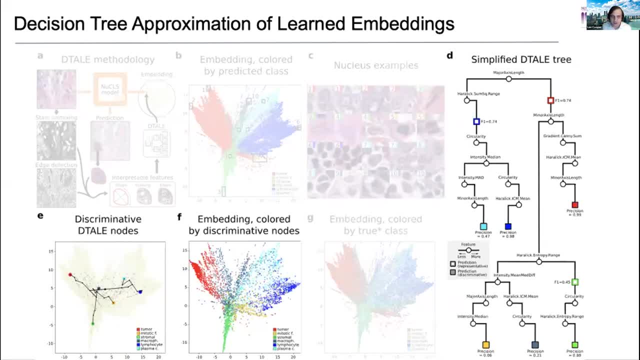 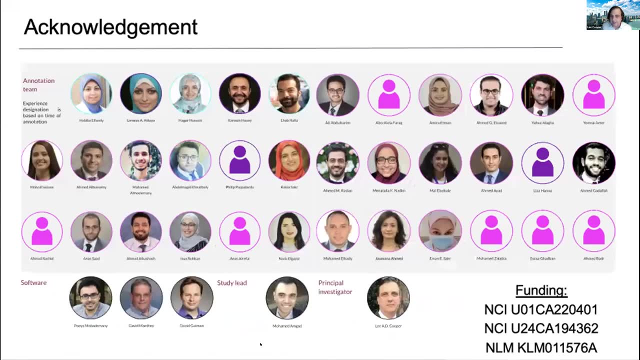 deep learning algorithm of the tree, which I think is kind of a neat approach. So, just to conclude, I wanted to, you know, acknowledge some of the people who participated- Mohamed Amgad, of course, who you know conducted the study, And I think it's really important to acknowledge some of the 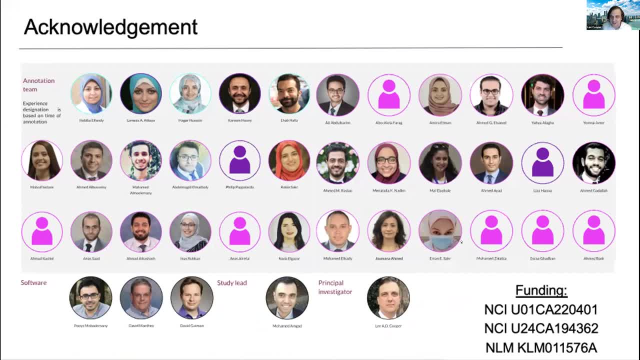 people who conducted all the study and managed the efforts of over 30 volunteers- All of our volunteers, many of which have gone on to pathology residency. we really appreciate their help And our team who also worked on the annotation platform that we use, as well as the funding. 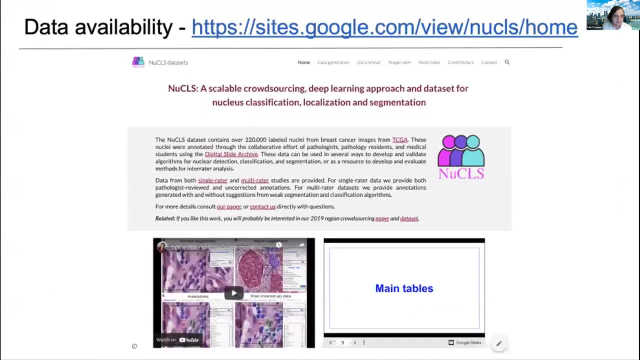 source and the people who pay us to do this. And then, finally, just to point out, this data set is all completely open. Our region data set is also open. We have a web page we set up where we describe the entire process, And we have a web page where we describe the entire process, And 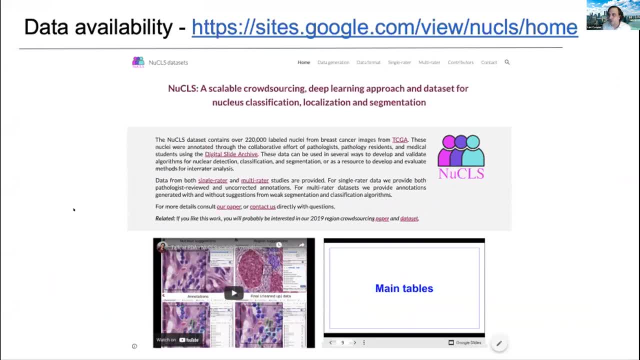 we have a web page where we describe the entire process and generating this data. There are videos that walk you through what the data is and how it's organized, And you know you're free to come and critique this and use it to benchmark your algorithms and to develop new algorithms. 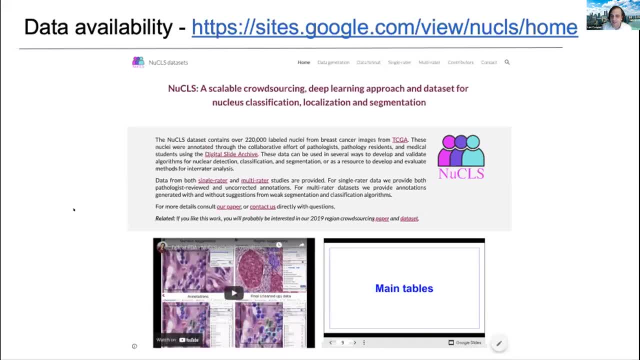 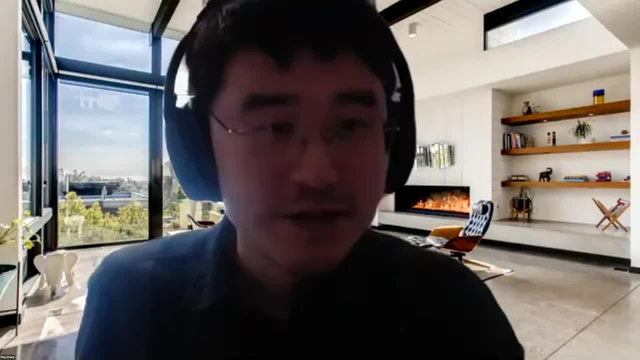 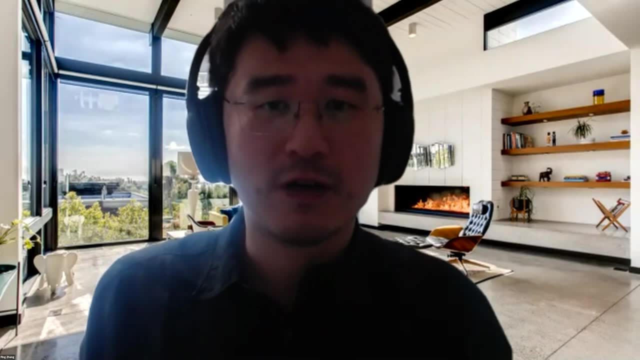 We really like to see that. So that's my time, Thank you. Thank you so much, Dr Kuber. Yeah, it's excellent talking to pathology, Yeah, So, yeah. so we are conclude the this section four And again. so thank you for the four. 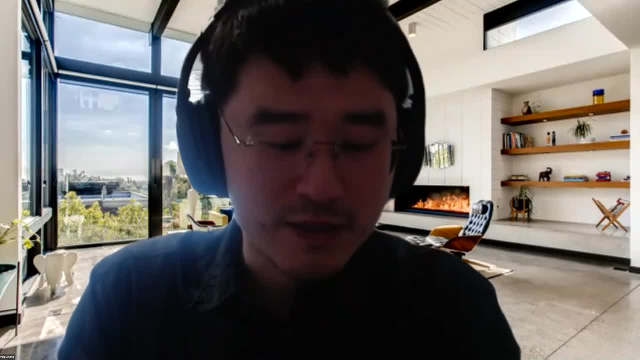 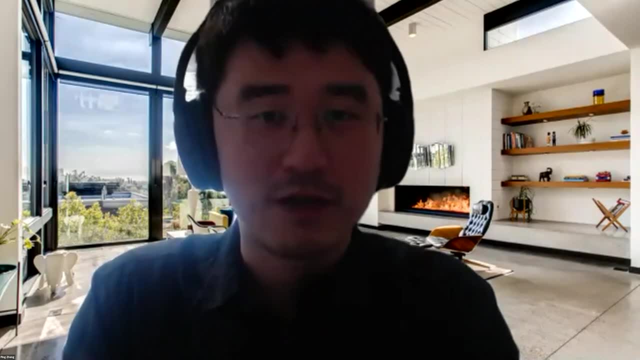 speakers for excellent talk. For the next 15 minutes, I will invite my co organizer, Dr Kun Huang from Indiana University, to host the panel discussion with the four speakers. Actually, I want- I would like to send a word of speakers. they already addressed many questions in the 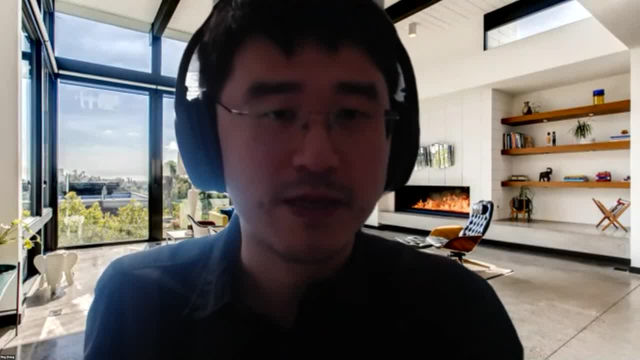 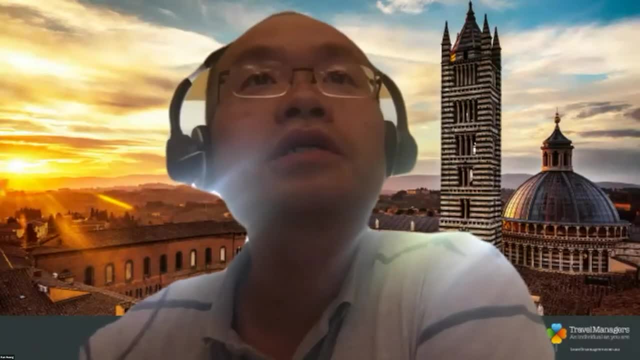 question, question and answer sections. So, Dr Huang, please lead the discussion for the remaining questions. Thank you, Yeah, So I mean there is one one new question coming up And in the Q&A panel- actually that's for Dr Li- that is talking about getting ground truth. 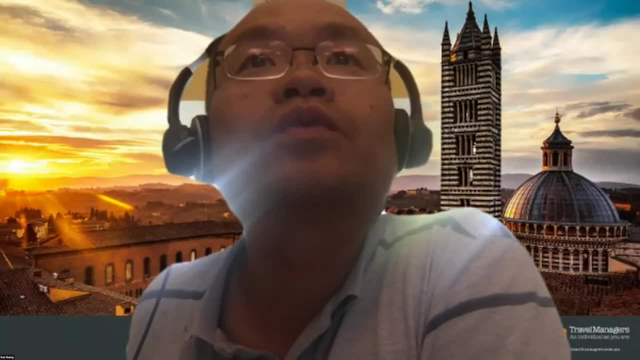 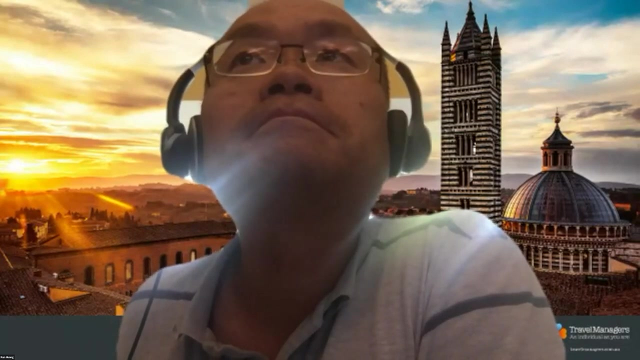 could be very tricky. And could Dr Kuber- I'm sorry, Dr Kuber, and to about can- if Dr Kuber can, elaborate more on the clustering method? Yeah, Yeah, so I'm going to refer you to our paper, but I agree with you, it's very tricky And I think. 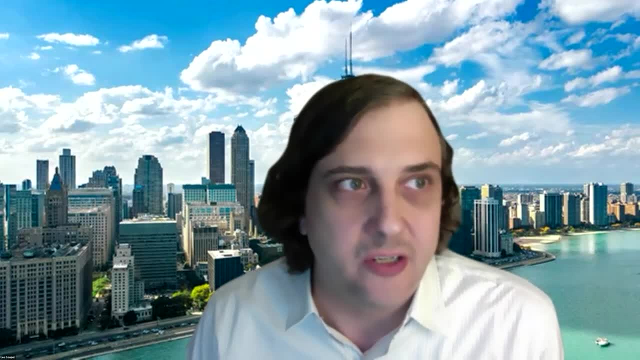 when we did our paper we did a lot of work on the clustering method And I think we did a lot of work on the clustering method. And I think we did a lot of work on the clustering method And I think segmentation project first it was more simple. we can just use like the same metrics people use. 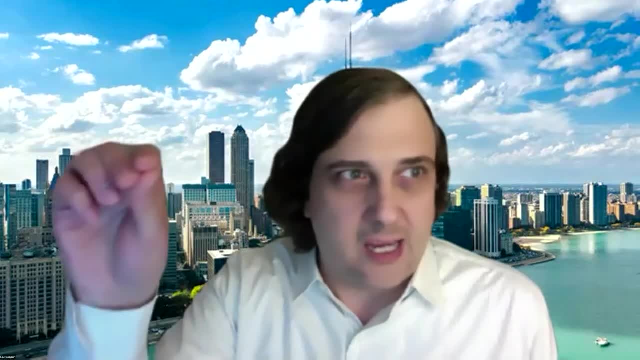 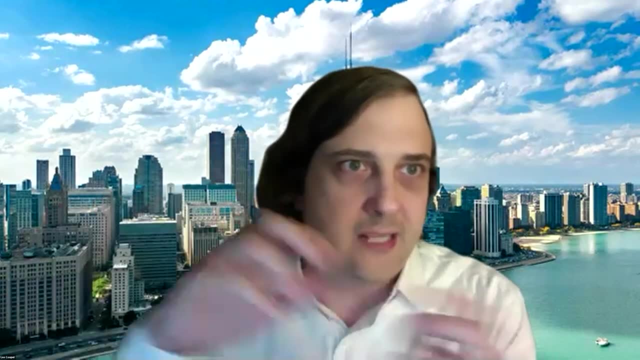 in radiology things like dice, But when you're talking about discrete objects there's a process of mapping. So if you have eight people looking at a single tissue area and they each have eight opinions, you have to kind of figure out, like for a given cell: are they talking about the same? 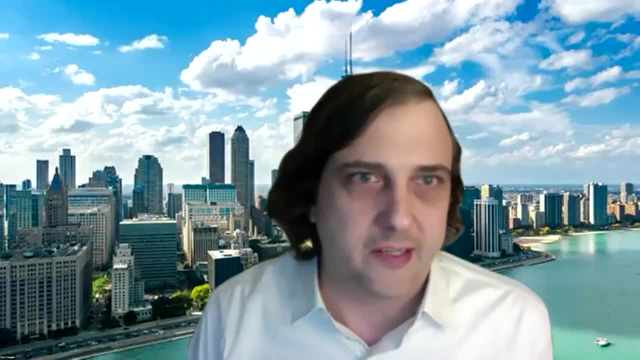 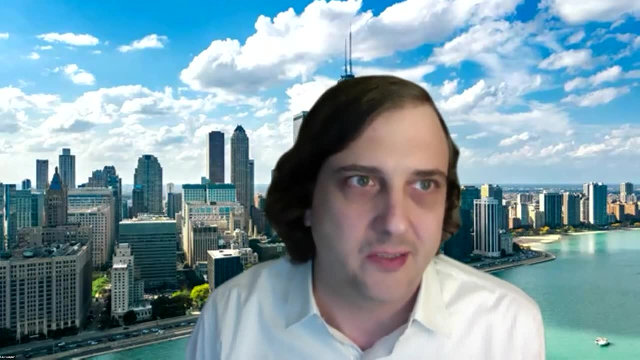 cell or different cells, And so that's really where the clustering is necessary. So I think if you take a look at our paper you'll see how we address that. But I think you know that's a big problem, For pathology is dealing with those discrete objects because there are many of them. 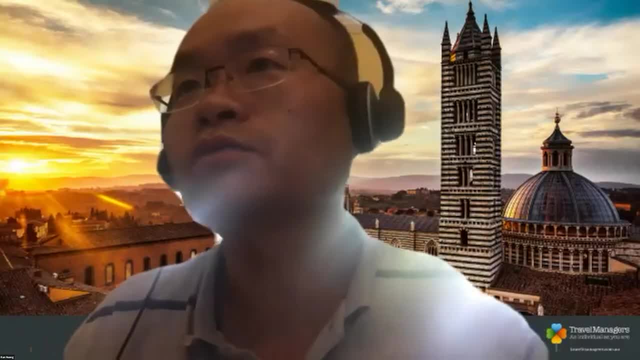 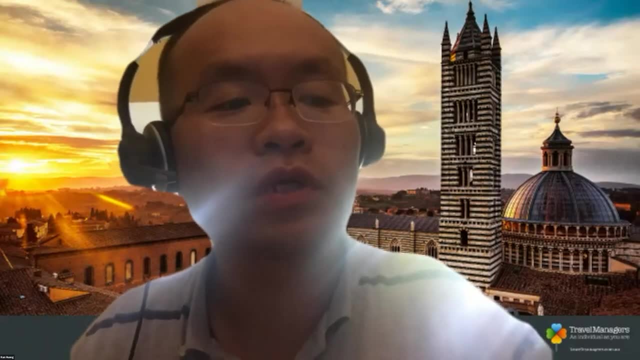 There is another question- Actually it's the same question- I would like to ask, actually for the panelist And because you guys give us such a wonderful talk today and with a clearly translational value and the translational applications. So then the question actually: 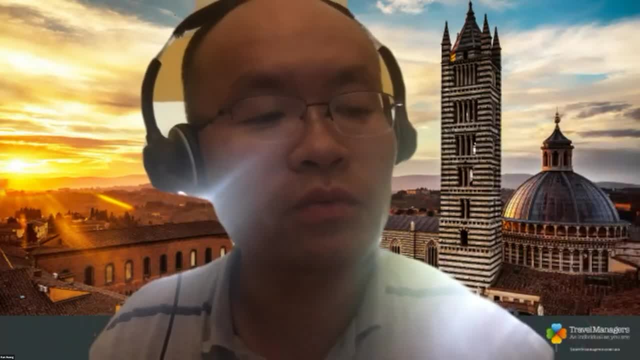 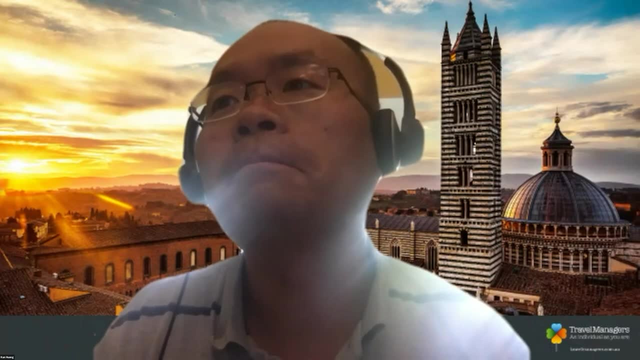 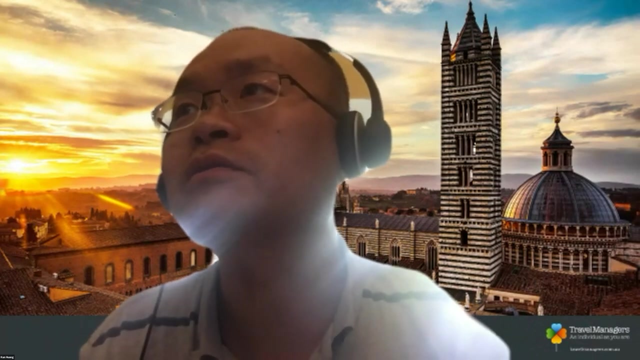 I think I have, but also the audience also have, is: what are the next steps And how do we really translate this into clinical practice or clinical? I think it's work flow. So I mean, since this is a common question, I think I'll just start with ask all the panelist members. so 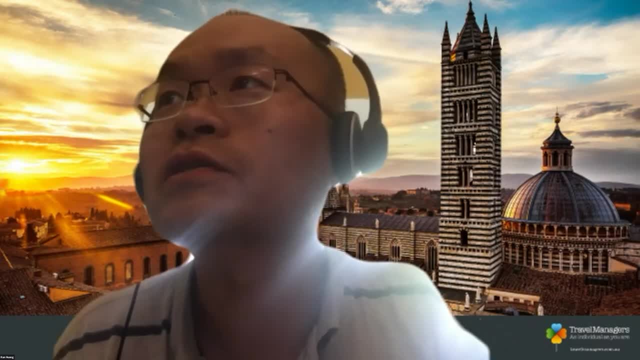 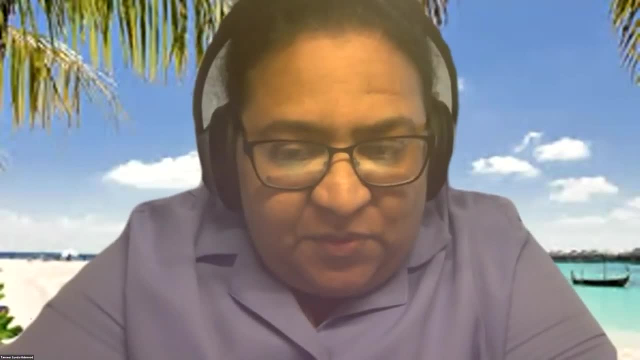 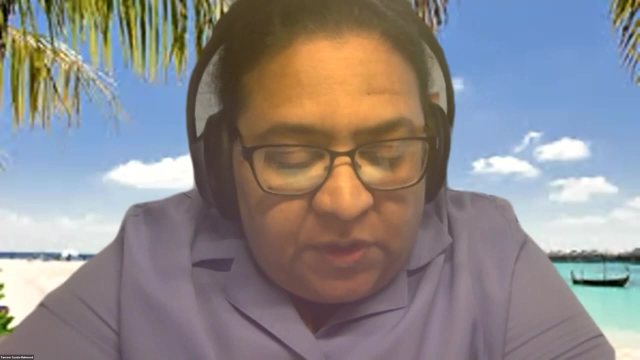 I'll start with Tanvir, Dr Syeda Mahmood. Okay, cool, I will answer that. I was also wanting to say that, in terms of the ground truth question, there was an additional point I wanted to make, if I could briefly comment on that before I get to this question. So, one of the methodologies. we had the difficult that each image would have multiple findings and we had to make sure all the findings were covered in the ground truth process right. so we use a triple consensus with adjudication as the methodology which is reasonably well accepted in clinical literature to do that. and 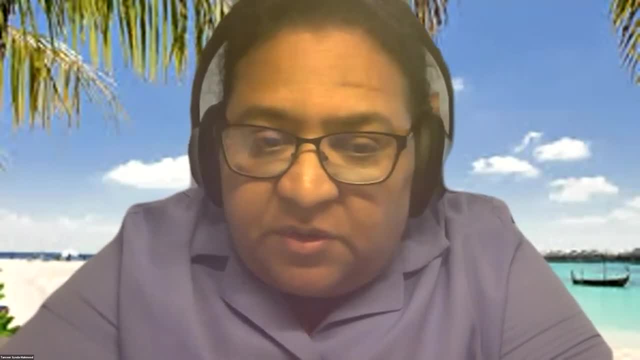 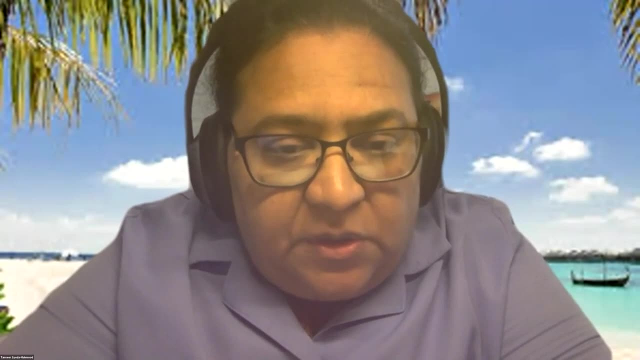 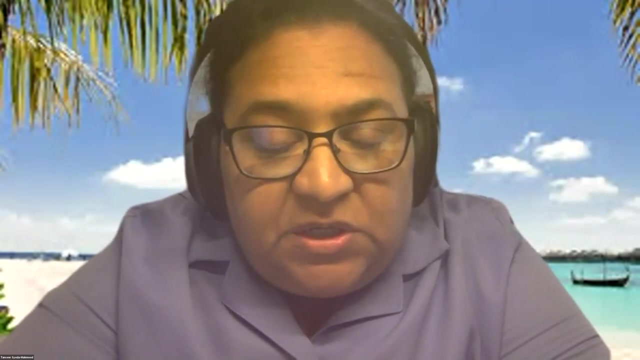 this requires having specialists with sufficient training and you know those sort of filtering, but having them do them independently and then come and get together in a room and hash it out until they are satisfied with the consensus they have achieved. so this was in discussion- adjudication process that you can do, for I mean, we were able to do that for about 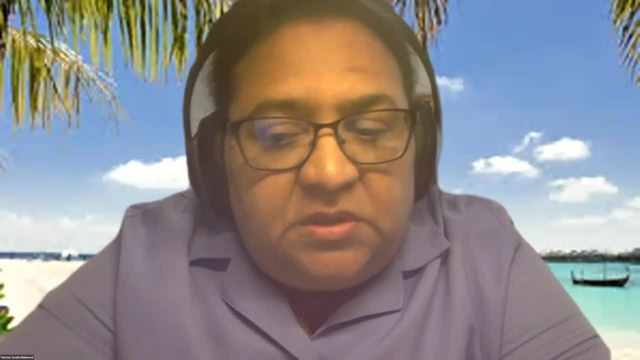 3,000 images, but the entire triple consensus adjudication process took us about six to nine months to achieve for 3,000 images. so this can give you a sense of how difficult achieving goal is The gold standard ground truth data set. problem is when you have multiple findings. 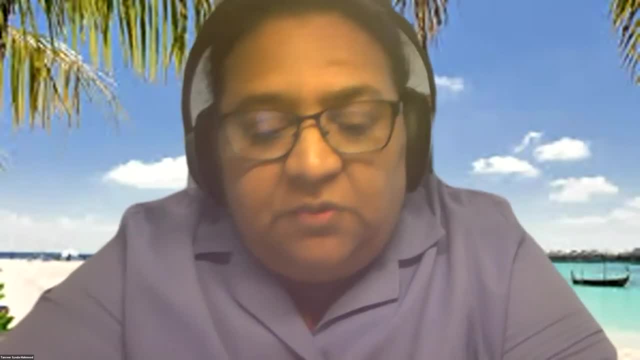 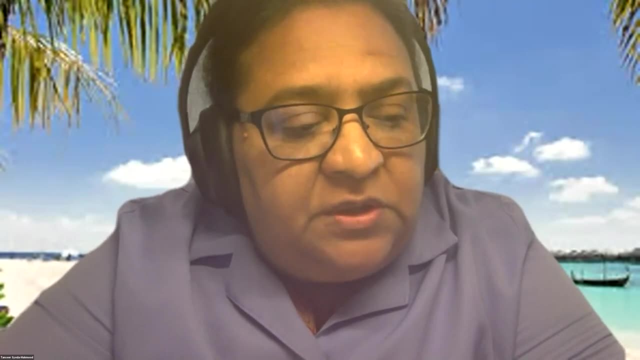 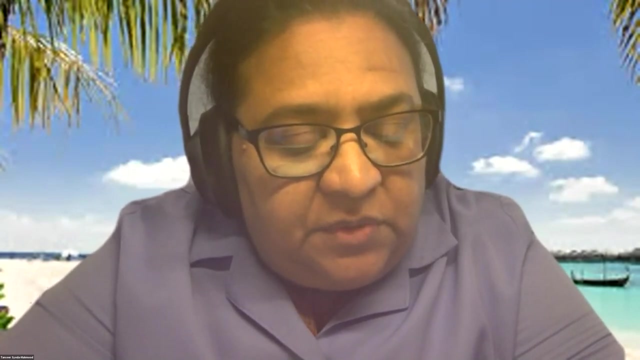 simultaneously present in one image. Now coming back to your question of you know how to translate into clinical practice. so one of the important things is to do clinical studies. I didn't get to fully describe these in my portion of the talk as we ran out of time. 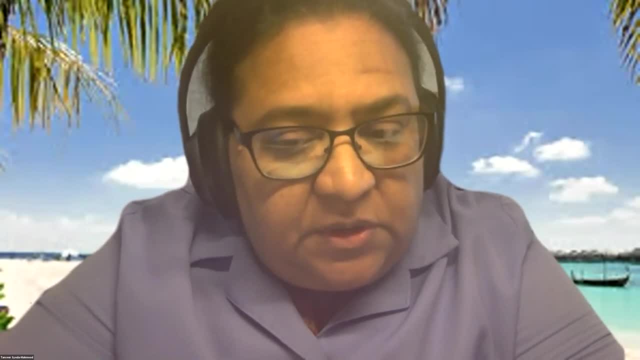 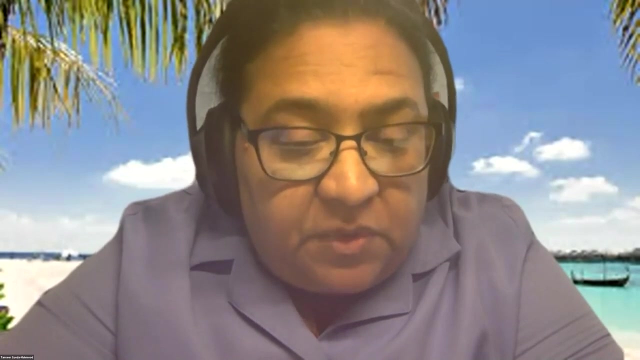 but doing clinical studies is very important in as part of the staging for this. Now, one of the difficulties with from a regulatory standpoint is to do this: clinical studies keeping the regulatory oversight in mind, like what would the FDA regulatory process would require, and doing the studies keeping those things in mind, which also means that the software itself 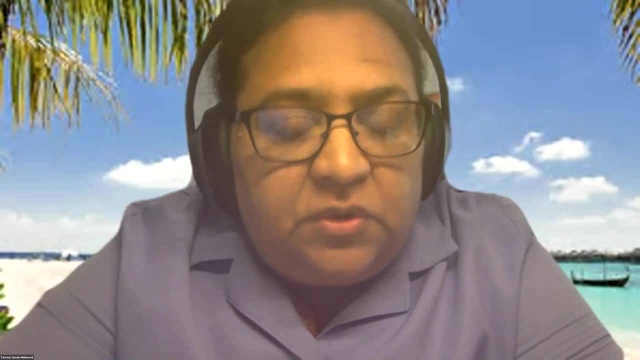 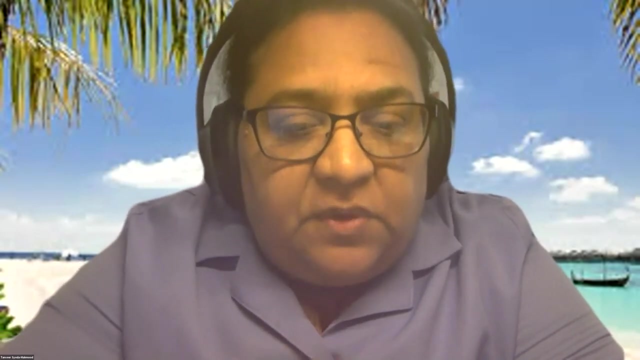 has to be produced using a QMS or those sort of operations. but once you are able to do that, you can conduct pilot studies. so one of the studies we've done is one such pilot study where you can. you cannot implement it in clinical practice, but it has to be a parallel workflow. 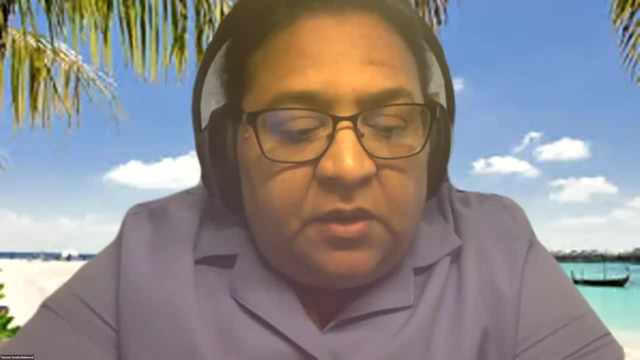 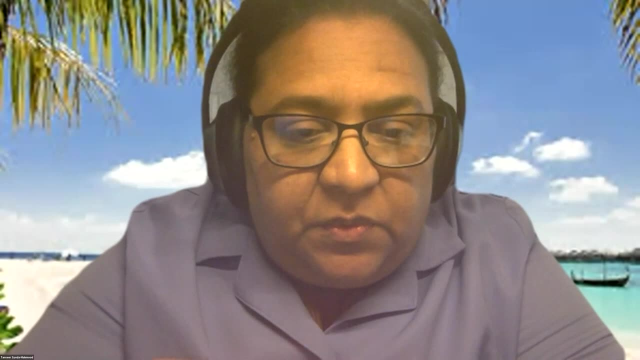 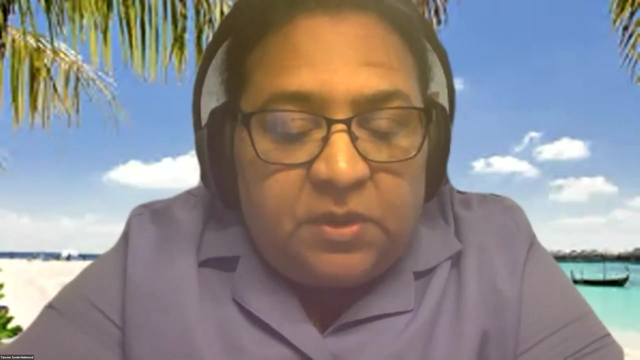 so the translational aspects of it go. first is a soft introduction where you can do this as a not impacting clinical practice but observation in a prospective fashion and then going into adoption phase. for if you are going for commercial then you have to follow the FDA regulatory process, but if your institution wants to adopt it for their own private use, 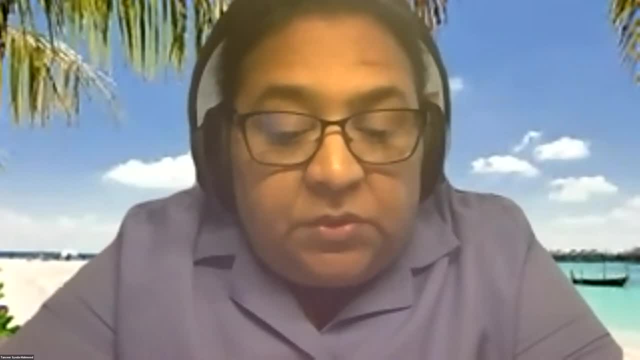 it may use a different process as well. so the translation to clinical practice certainly needs full-scale evaluation before you get to the pilot studies and then you go through the pilot studies as necessary for getting a regulatory oversight. I can tell you that FDA regulatory paperwork for AI algorithms has simplified. however, they still don't have a 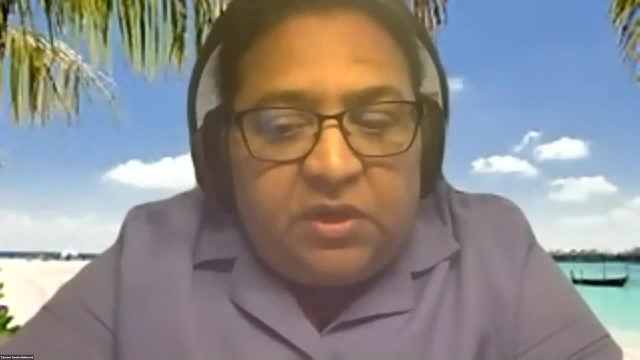 good way of treating multiple findings when the when the number of findings is in the hundreds, they just don't have the machinery to to approve such things at the moment. so this is one of the great difficulties in scaling AI algorithms. when the machine learning models are able to recognize 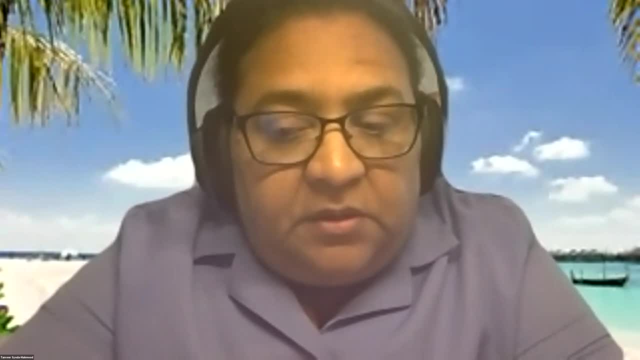 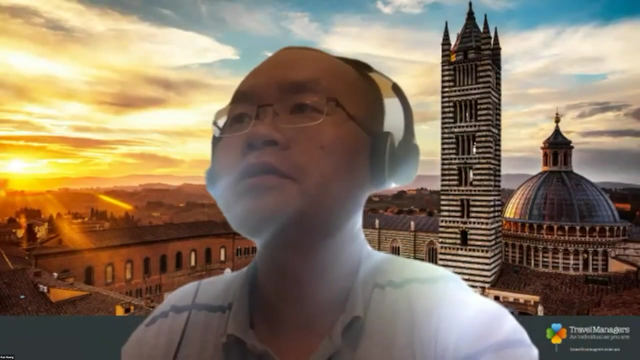 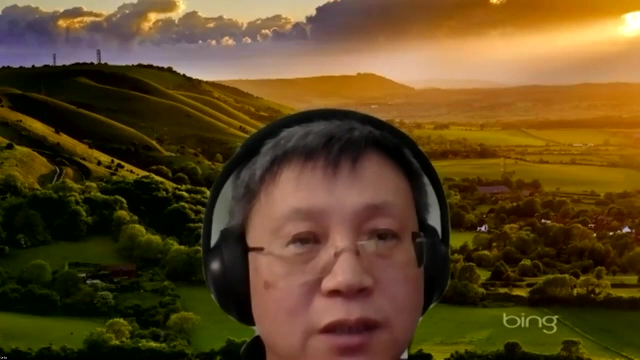 large number of findings simultaneously, but the evaluation and the methodology for you know, approving them for pre-market clearance is very difficult. all right. so, Dr Lu, you have got any comments? yeah, so I have a humble understanding. like you know, I work at Siemens. I, you know, we build FDA. 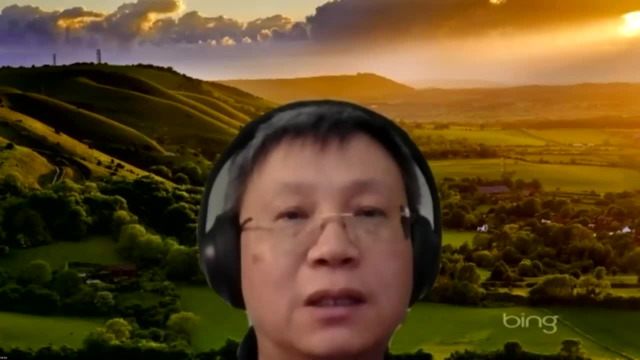 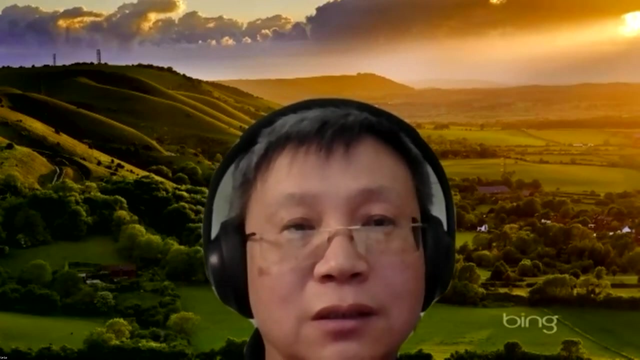 clearance stuff. right, and when I was at NIH we actually we have- we had meetings with FDA folks- that actually doing research they're not. they're not doing the approval work, but they are the backbone. they're doing research on deciding what can be approved, what cannot be approved, in a sense. 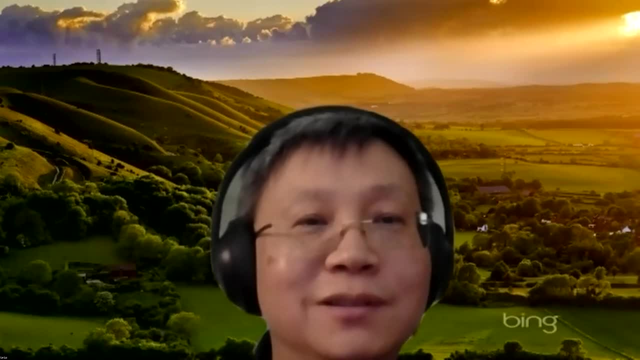 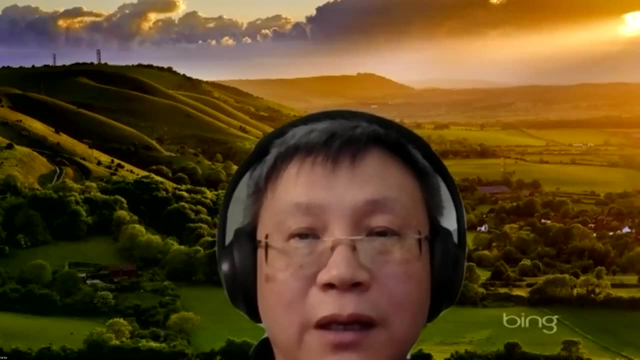 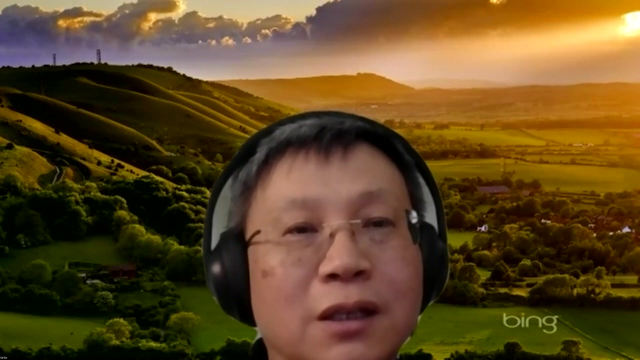 right. so they are doing kind of like counter research in a sense to figure out what's the real. what's real means what's really significant or not. so my hypothesis may not be correct, but I I think it's. the FDA clearance doesn't mean you are really helpful for the, for the clinics. 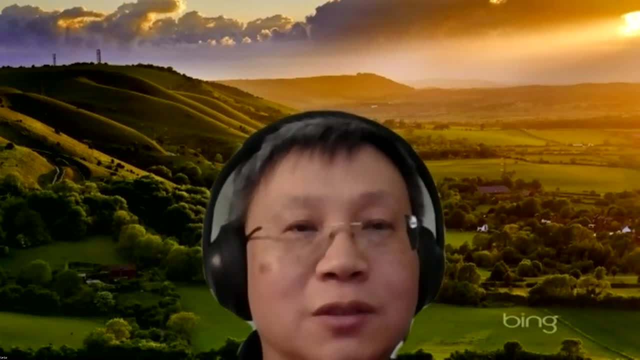 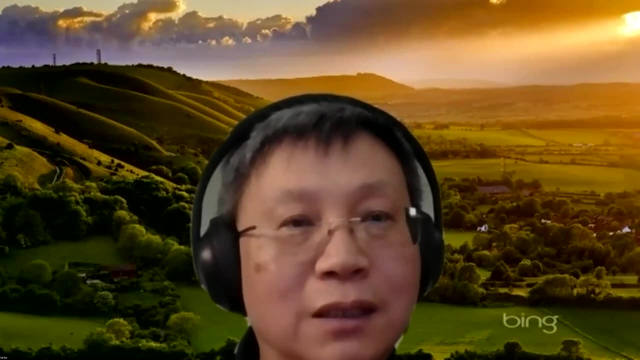 honestly, I think that from my own experience in, I see, when we do FDA present stuff, I don't feel like they actually help people like me or other people, but I do not feel that's really extremely helpful. so your understanding, the FDA clearance standard is between. you know you have to be safe, right you? 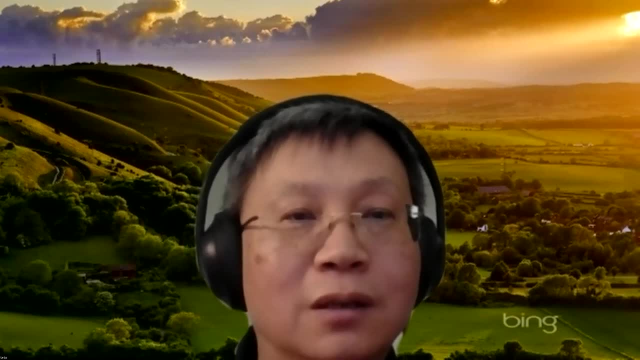 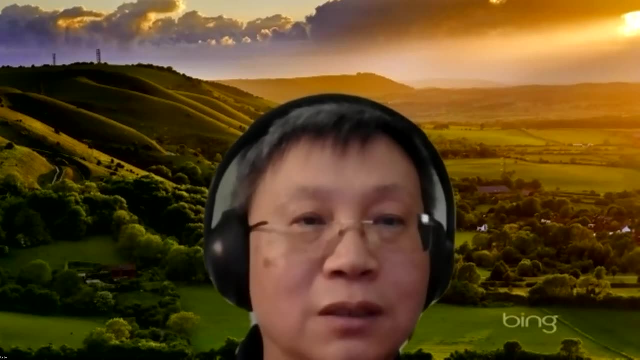 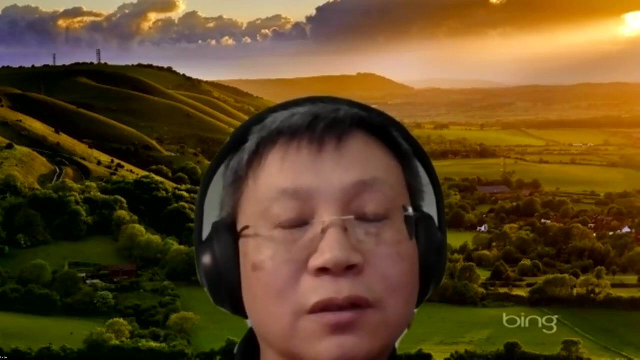 don't hurt patients and but it's below being very clinical useful. that's my assessment. you know you have a lot of FDA current stuff. they don't really sell well, they don't really help as you expected, you know, I I think I think this is one factor of doing certain things unnecessary. condition, but not. 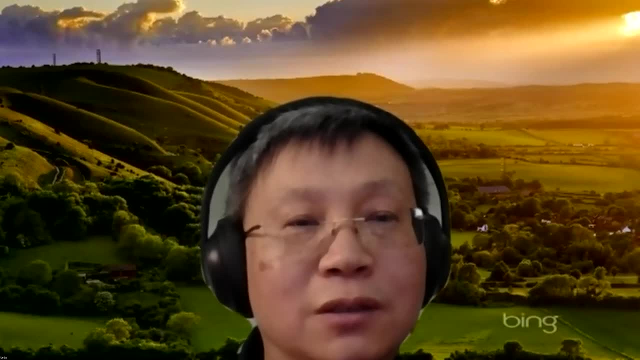 of the, not all thing you need to achieve in order to be clinically useful. you know, the goal at least i think we we should achieve is clinically useful. they need to help patients in health physicians. they need to make the way they can pay. they can, they want to pay for the, for the models or product. 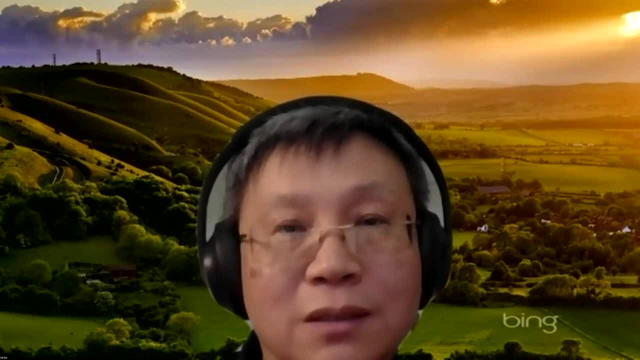 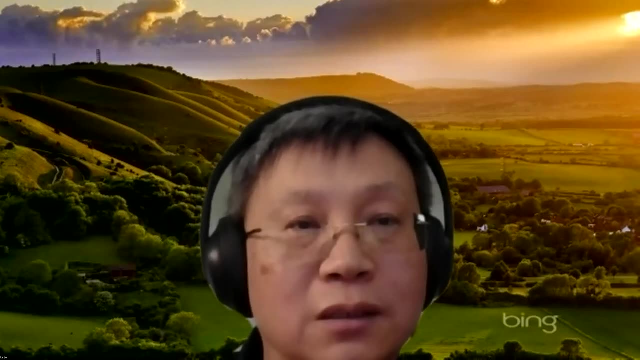 you. you are developing, because only if they are willing to pay means you really make a value. i think that's actually actually above, above the fda clearance standard. you know, of course, eventually we want something is that they cannot live without it. right, that's even one bar above. 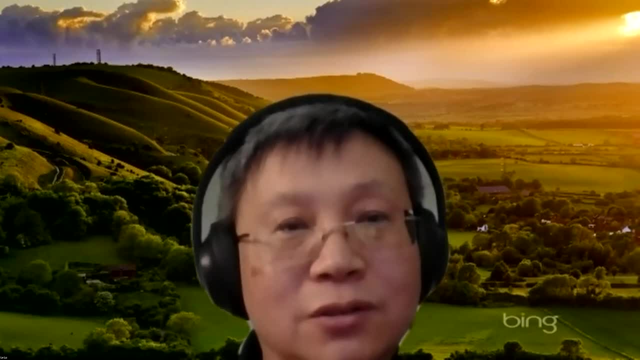 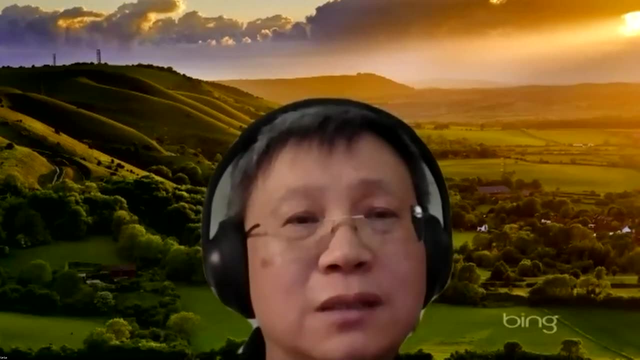 you know, i i think fda currency is nice, but it's not really end of the story. you need to do more things with more things beyond that. so, but also, you know one thing at least at all: today is like: once you, after you cleanse the substance, the thing need to be frozen right and 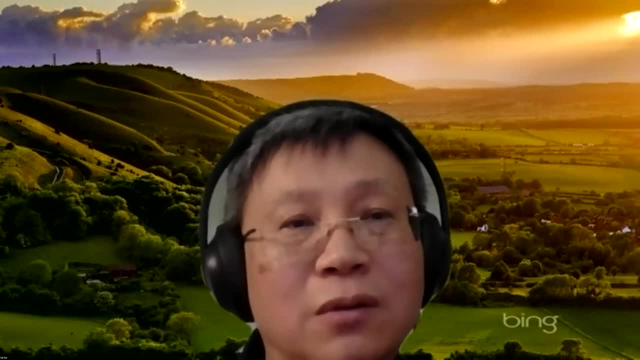 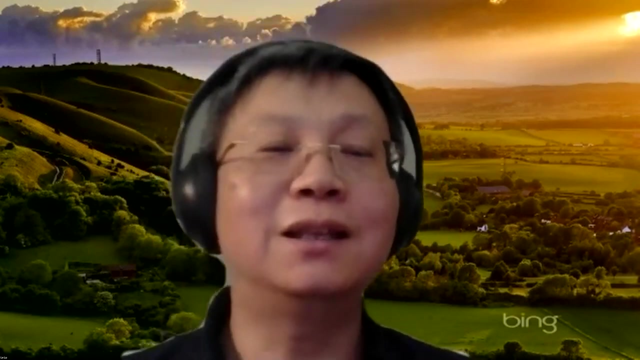 you at least before, and like at siemens, let's say, we have an old version which was fda clearance, but we have a newer one which is way more better, but we cannot afford to spend the next couple million dollars to do it again. you know, that's, that's. you know i don't know what to say. you know it's kind of silly. 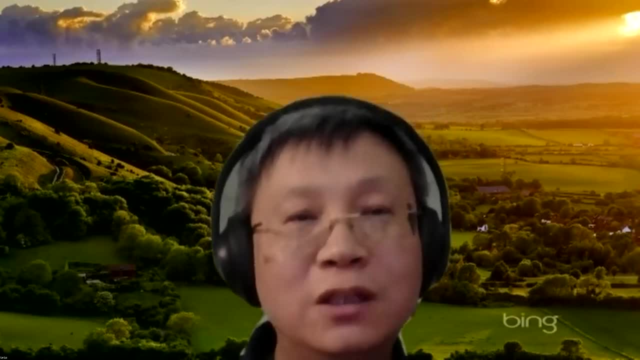 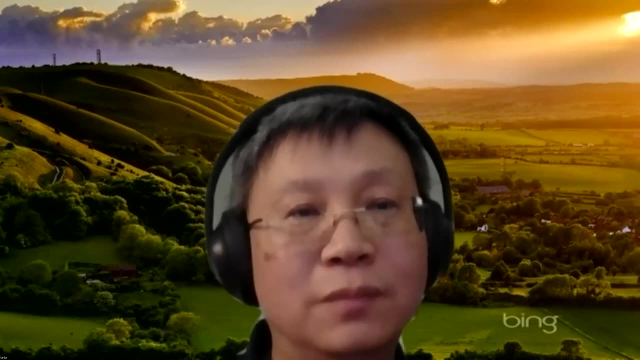 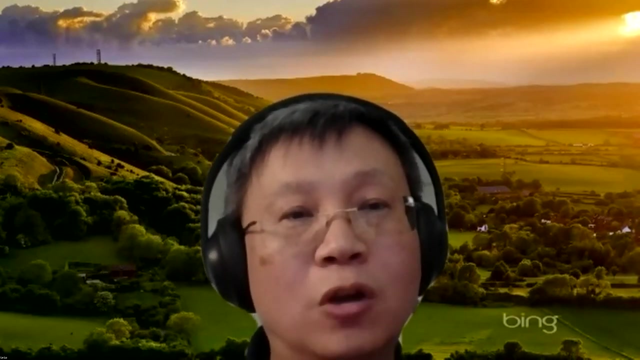 but you know, that's not just we need to work on, i think. i think i do need also looking into this issue: how, how to make this thing work, how to make something translatable. you know, somewhere they need to be less rigid and i think somewhere they need to be. 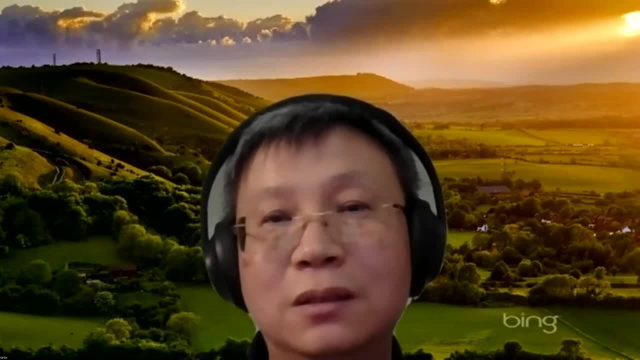 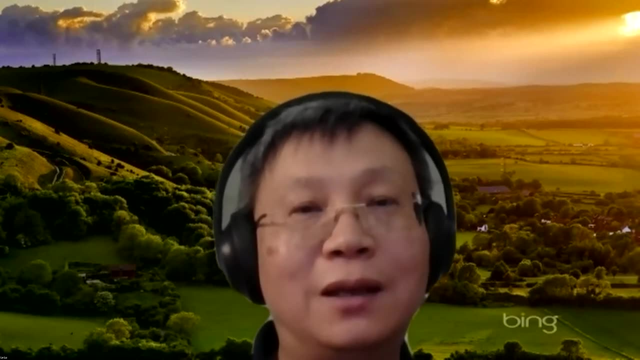 more rigid in a sense. we all need adjustment in a sense, otherwise it took too long. it takes too long to see patients i work in. actually that completely changed my life. i, i saw this- you know i'm mostly oncology. i saw many patients on the hallway and actually like really suffering and of course they 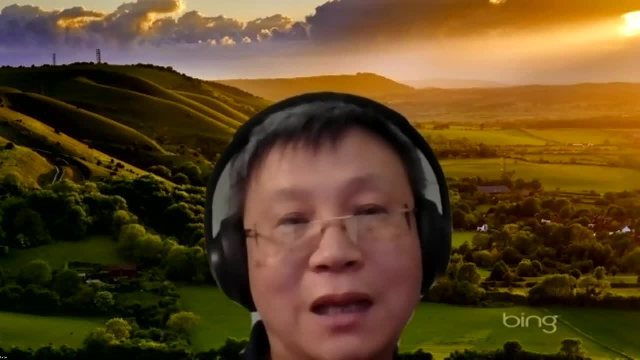 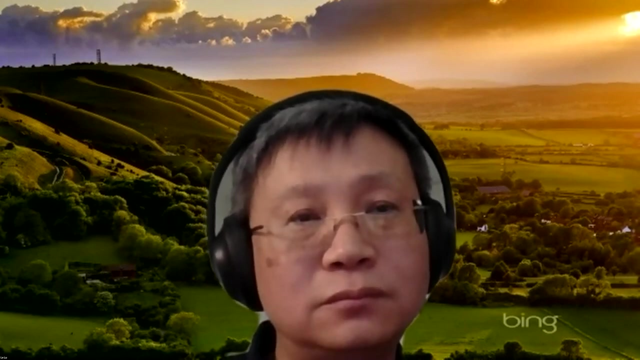 already had the best care ever possible on the planet. but i mean, really, it's limited patient can care anyways. so that's really the the best of the intuitive medicine and empirical medicine on the planet. but, um, you know, we need more than that. it's just saying so right now. our strategy is: um, i want. 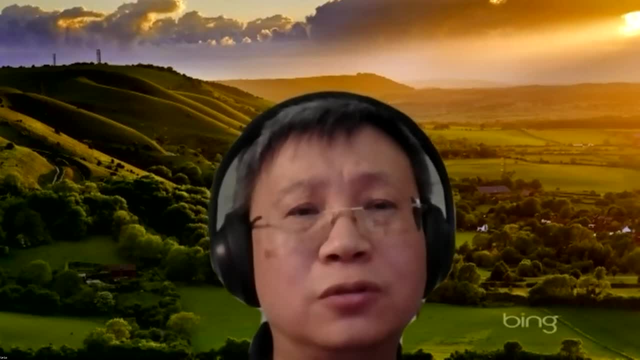 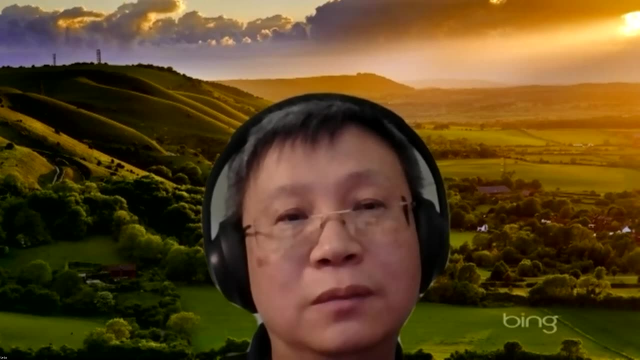 to first make sure everything are really really clinically useful before we go to fda, before we go to uh, before we go to clearance, that that that's something we want to uh make us we have one kind of scalable way to do even larger clinical trials, working with my hospitals, even open. 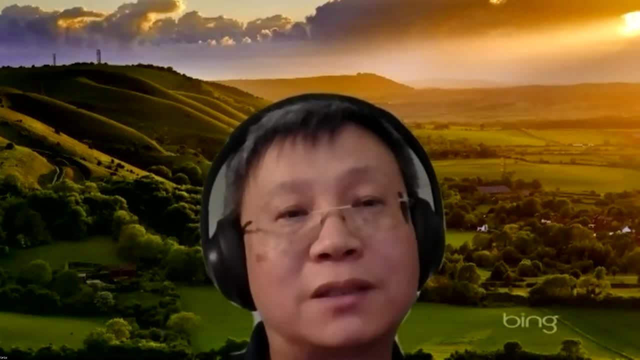 you know we doctorize the stuff, we build, uh. we work with past companies. they can help us to deploy uh. so really like a mock hospital can be used. that you know i want to. hopefully, you know i'm i'm working for a company. i don't make all the decisions right, but just think from a researcher. 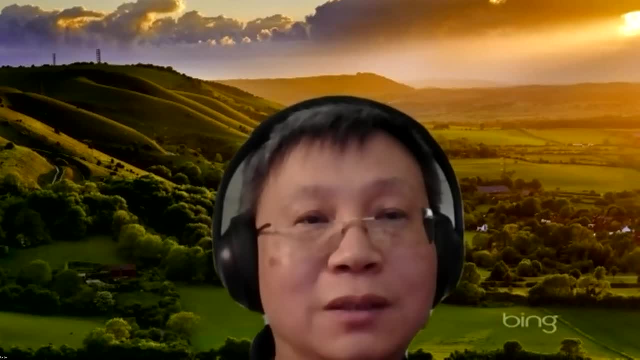 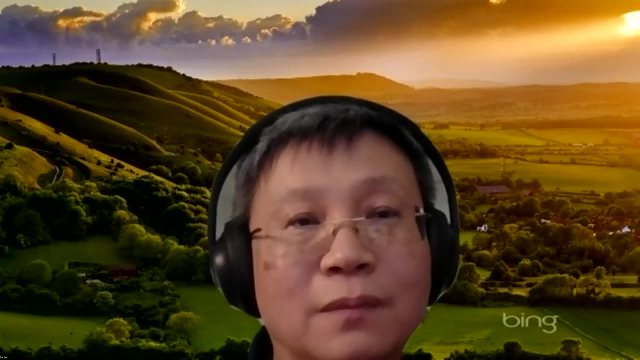 perspective, or from a person. i work with physician every day for the last eight years, really every day. i have a meeting with doctor every day, monday to friday. but i- i think it is- we really need to make sure something really, really useful. then we go to fda clearance, then we deploy to more places. 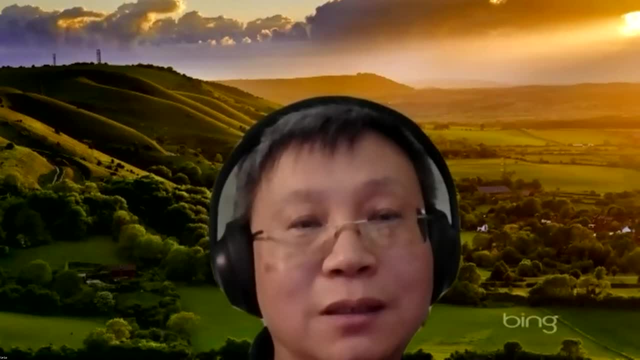 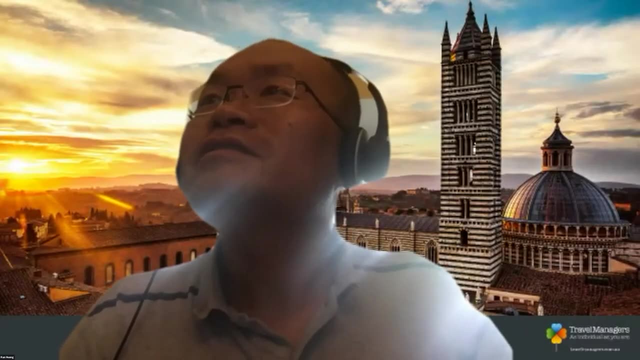 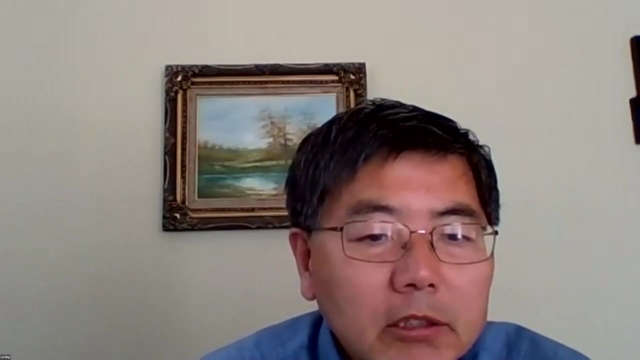 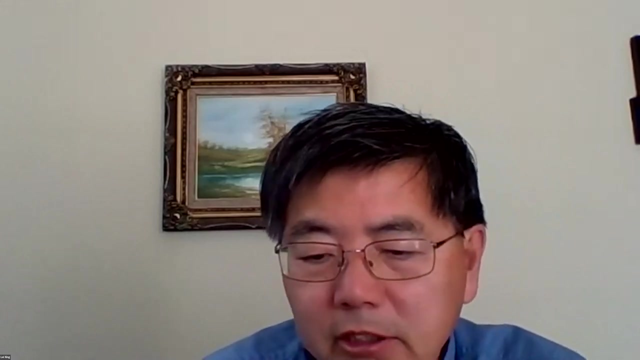 for money. yeah, that's basically what i want to say. yeah, thank you all right, thanks a lot, uh. so, yeah, well, this is a very important question and obviously we're working to change the healthcare. uh, you know, in my opinion, i feel there are two ways to translate your research into clinical practice. you know, if you're working in a clinical 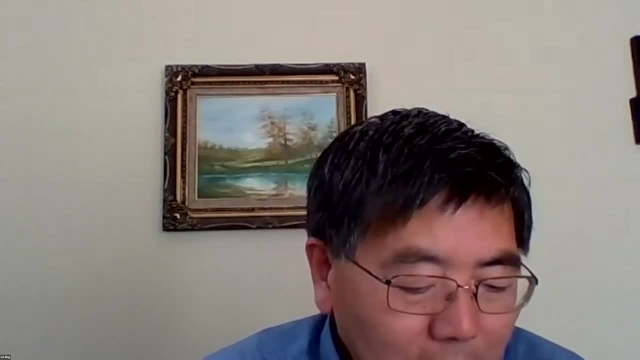 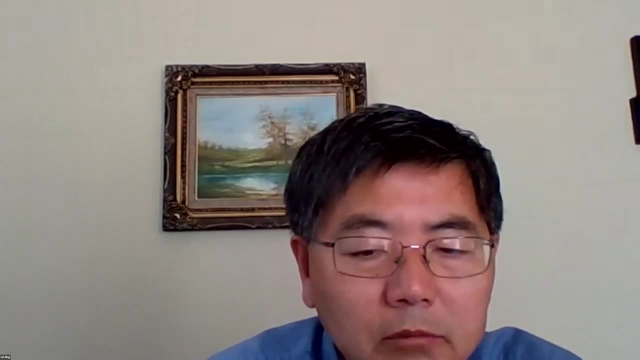 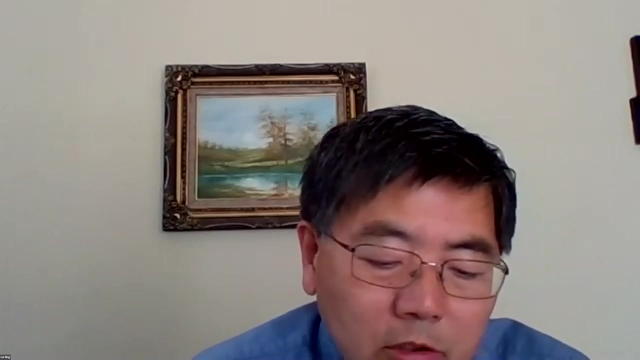 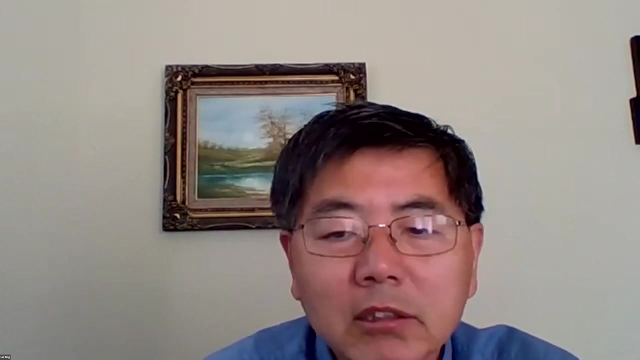 department, like me, or if you are, you know, having a very close collaborator in the clinical department, which i strongly recommend you, you do it. if you don't have one, uh, you know, it's possible and we actually did the translation something into our own practice. okay, because that's a diff. so there is a big difference, right. 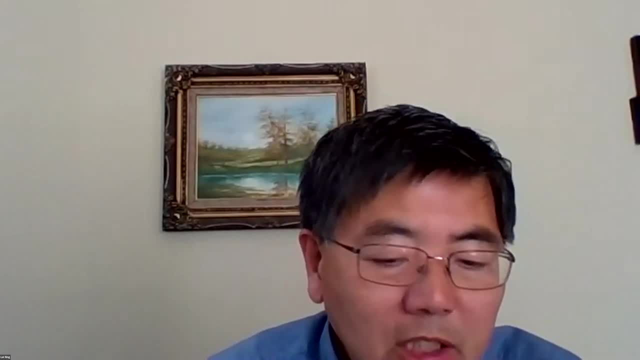 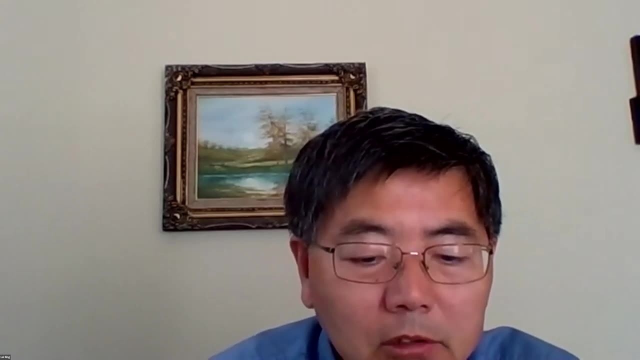 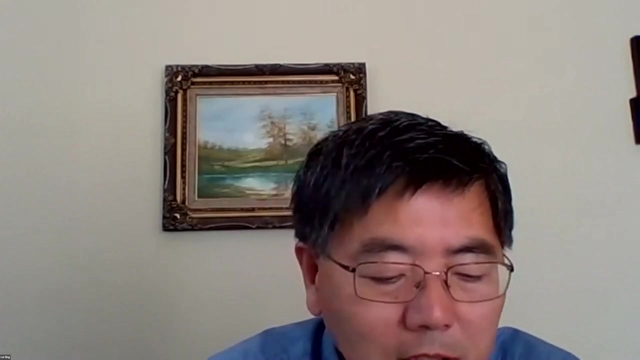 we. obviously, if you, if you do it in your own clinic, that's impact it's not huge, but you know it's a first step, uh. so i think it's an important step, you know, being able to test it in the clinical practice. i think the key issue is really the workflow. i mean just being able to, hey say, increase. 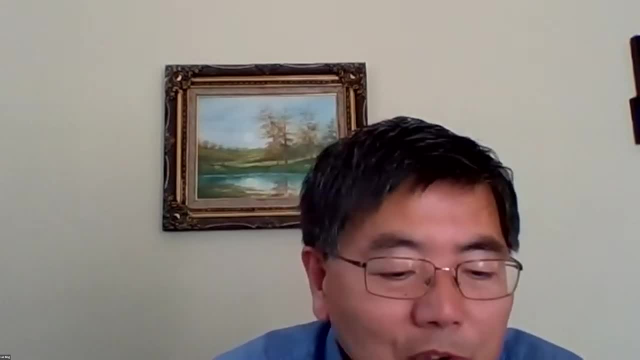 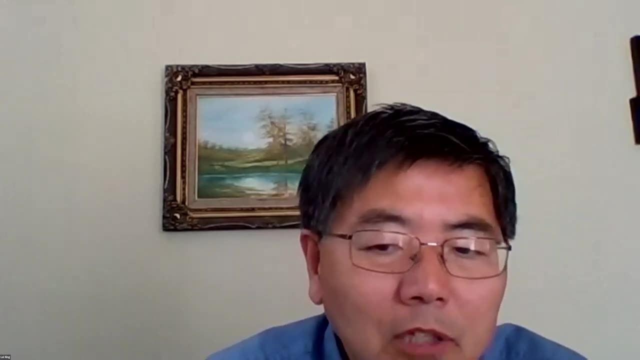 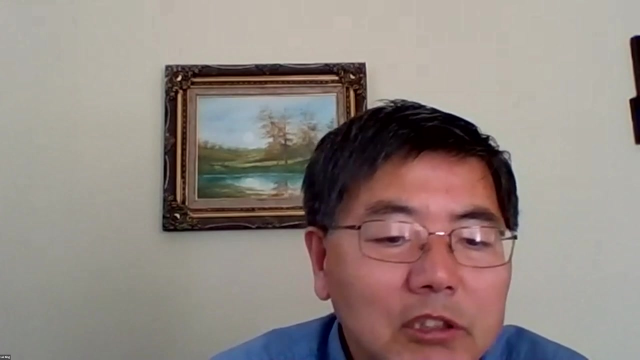 the dice of coefficient by point. you know, by a certain percentage it's not enough. you know you have to ask the question: at what cost? right, because uh, this day's, in the clinical environment, there are a lot, a lot of restriction. uh, i have to say that even you installing a software on a computer, 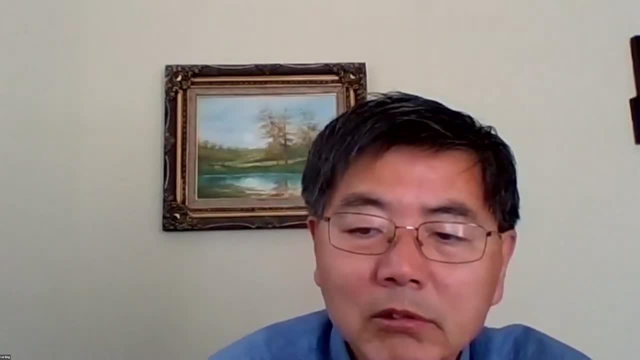 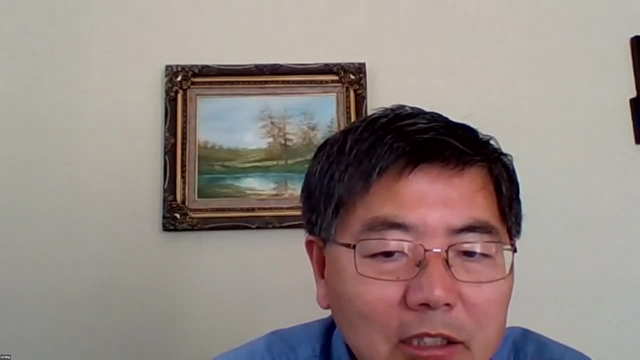 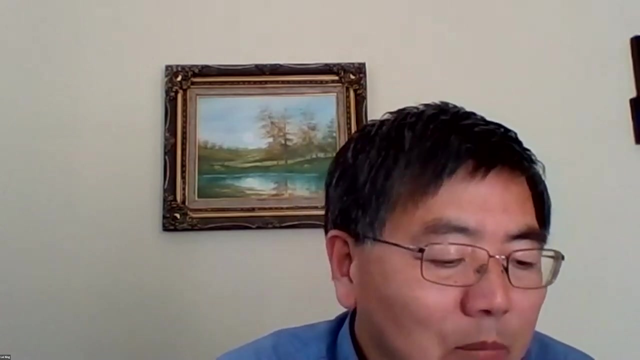 in the clinic. you know you have to go through the it, you have to- uh, you, you just have to go through a you know a long process. it may take longer than you know to to get that work in the clinic. then you spend time do your own research. so sometimes you have to balance, you have to. 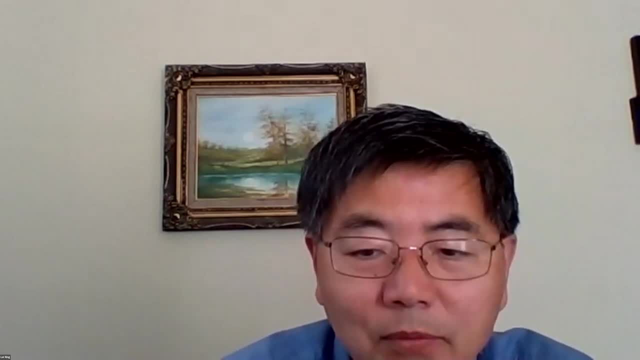 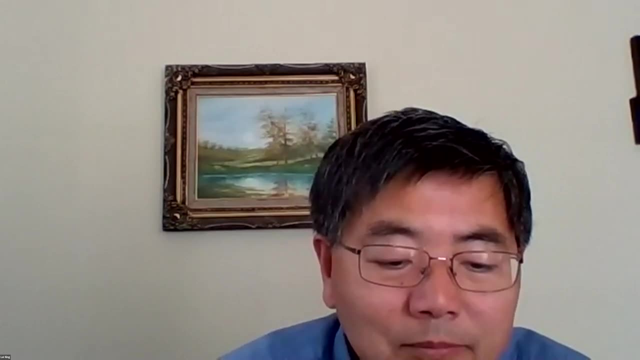 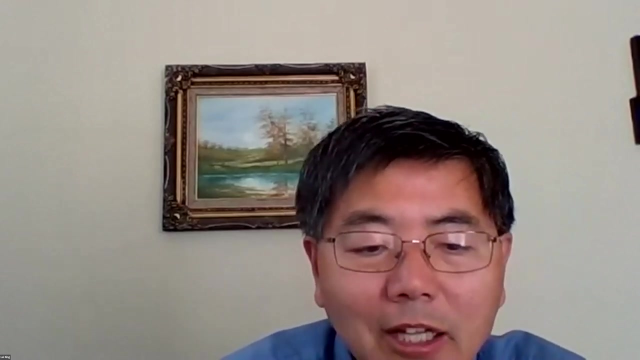 basically say, hey, is it? is it worse for me to really go through all the hassle, uh, to make it work in in the clinic because you say maybe i can spend my time better to do more interesting research and then let other people, let other company to take over and to translate into the 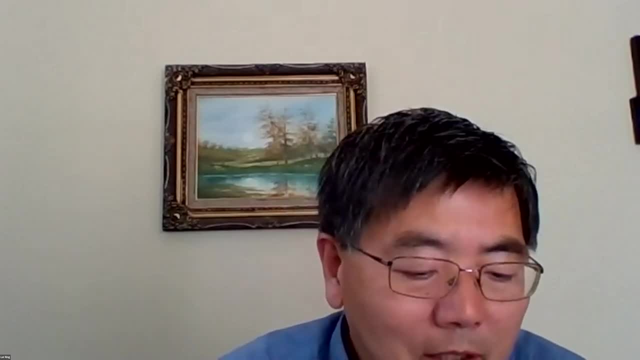 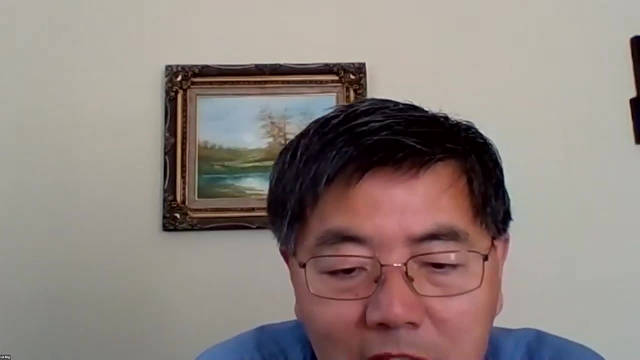 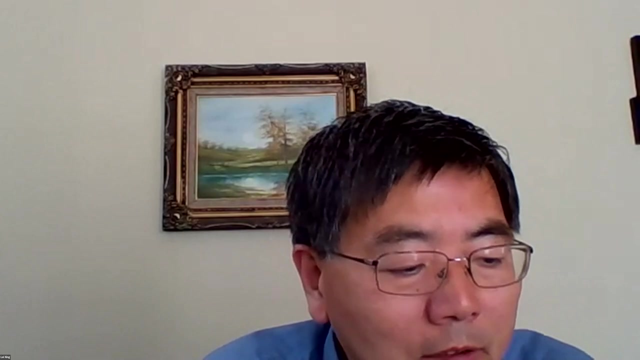 into the practice and i think it's all in the end. it's, all you know, a trade-off. so the other path is really license your technology to company. we, actually we, we were successful on that, uh, uh, you know, in some technology i actually get licensed through. 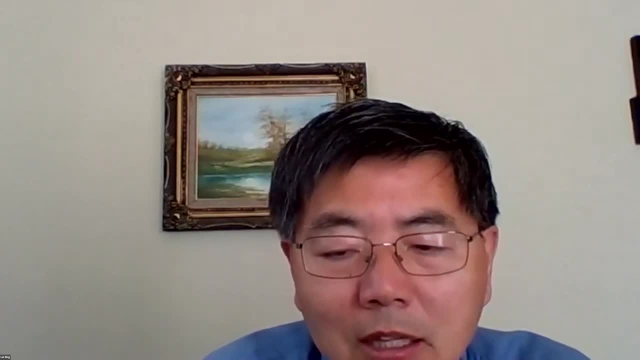 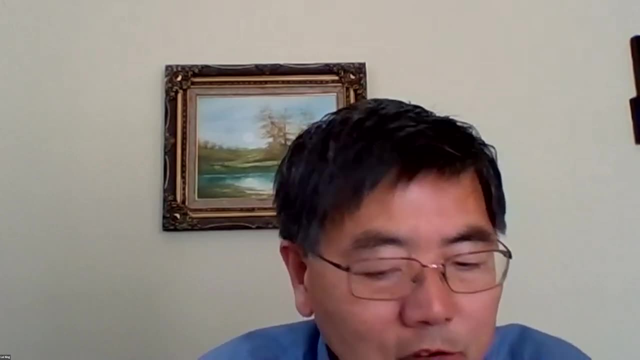 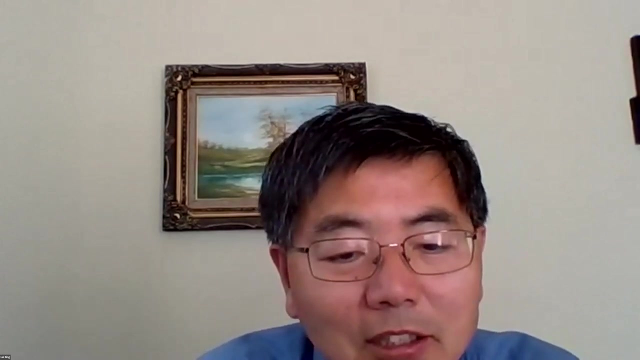 the university to some companies and they are obviously professional and so they can make the software, you know, robust and then industry great and uh, and then they have, uh, the marketing team, or you know, really to sales team, to really, you know, penetrate to the, to the individual. 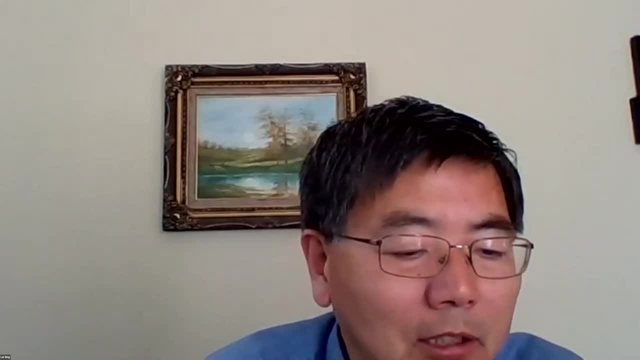 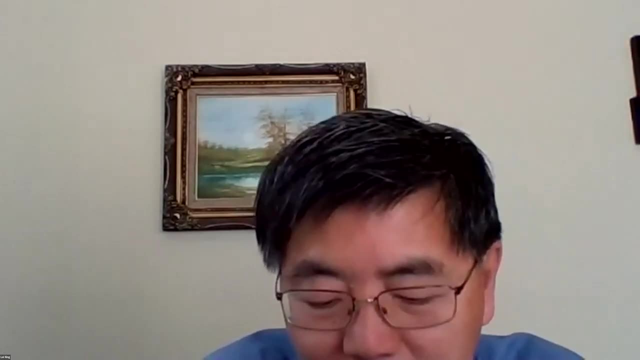 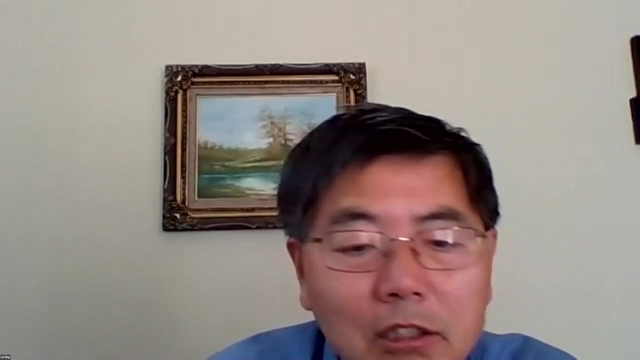 hospital, because that's not a trivial. i mean, i think, uh, it's, i would really if you- if it's not a huge technology and maybe that's a good way to go right- just license to somebody who is good at it and led them to to finish the next few miles. i mean really, uh, i think those are. 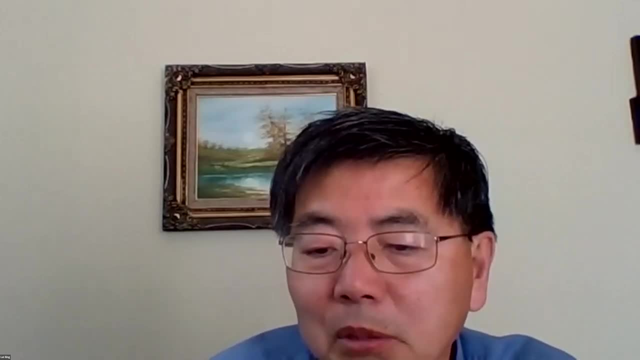 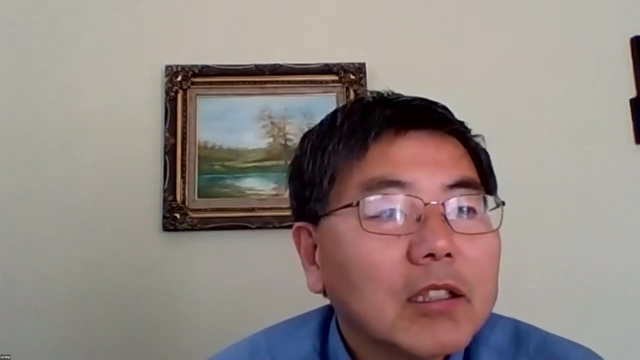 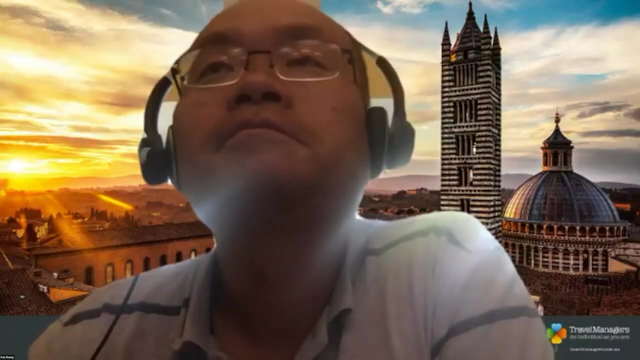 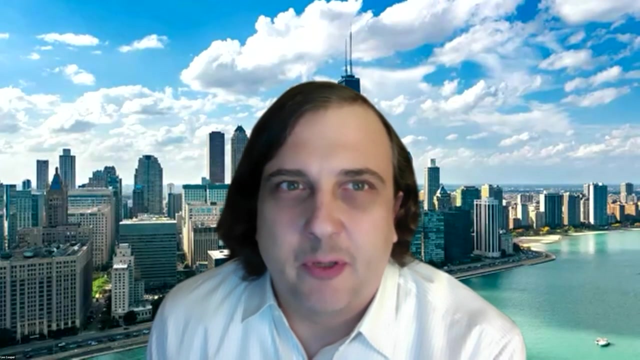 those are the uh important things that the people need to keep in mind. you know, licensee is actually very useful. yeah, that that's great. that's a wonderful point. um. so, lee, do you have any comments? yeah, you're also working in clinical departments, so right, i think the opportunity is in um, the opportunities in clinical trials, right, and i think the first. 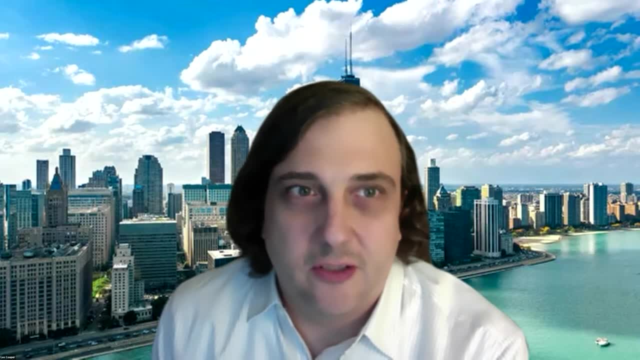 thing to do is just to sort of build the operational capabilities to do those things, which is really challenging in academics, right? so you know, before you use the predictions to influence any kind of treatment, i think you need to show that you can generate them and provide them. 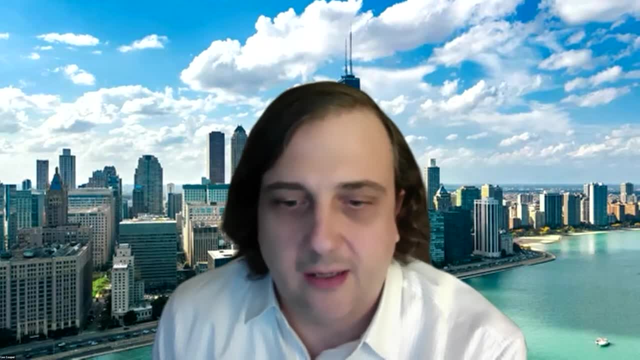 um, you know the clinicians in a you know quick, uh manner, that you know where they appreciate them and they can visualize them and that's, that's not trivial. so a lot of those operational pieces i think you know it's hard to accomplish in academics because we have like post-docs and